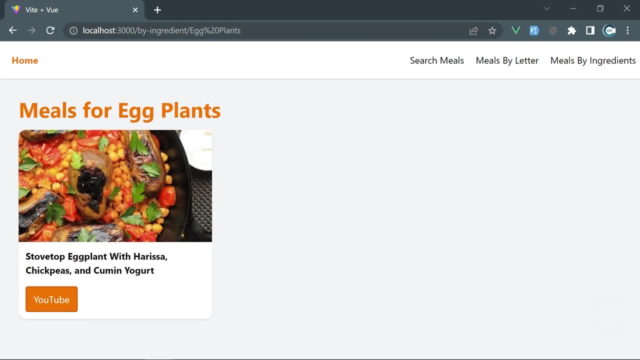 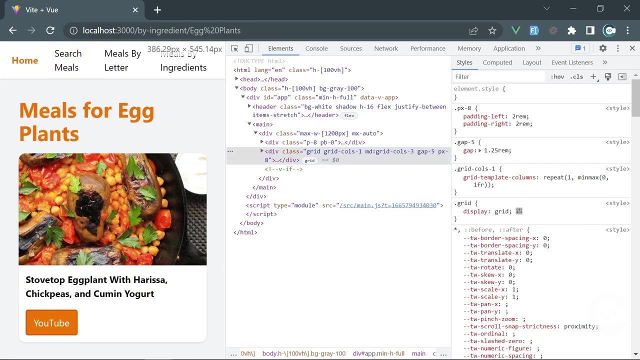 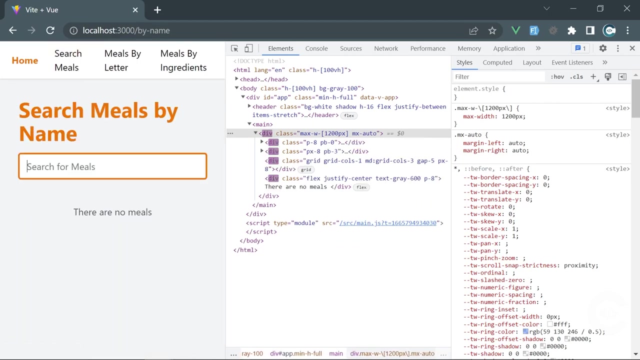 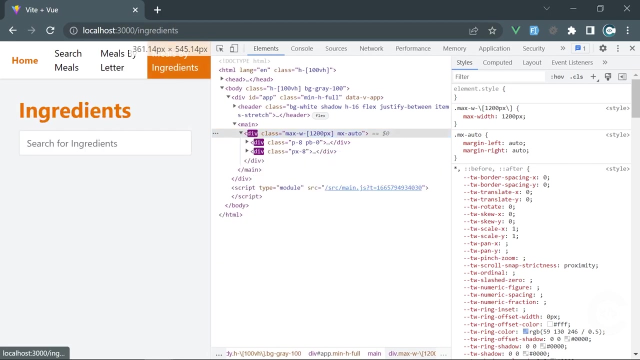 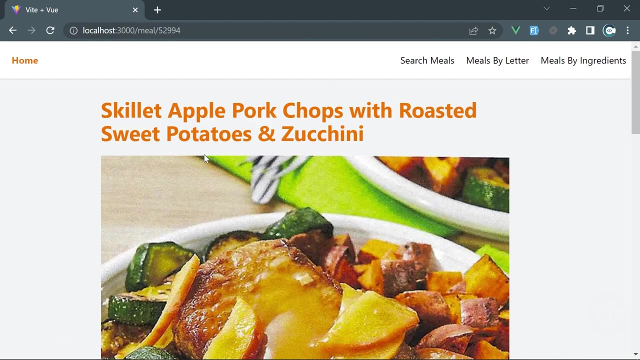 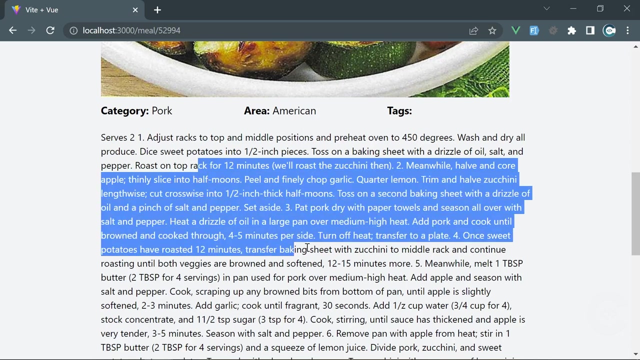 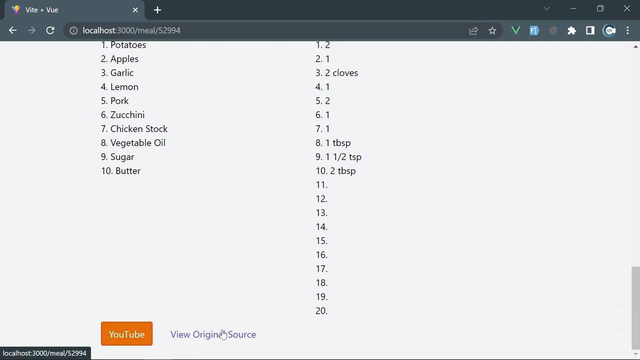 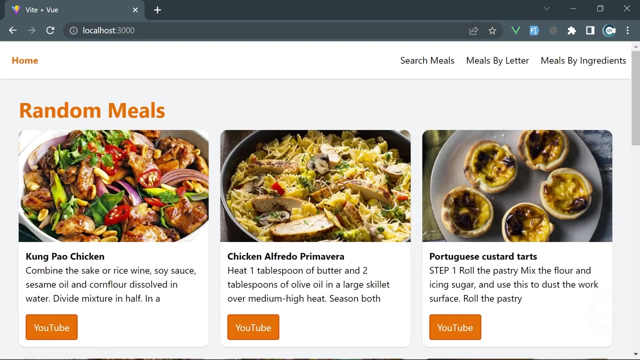 Okay and right here we see also the ingredient name and we're going to use Vuex for this to display this specific text right here which basically was loaded on a different page but now we need this on this page as well. And everything is responsive so if I just reduce it go on the home page we see them as cards single item in a row. If we go on the search page everything is fully responsive. Right here we see that the letters are going on a next row. This is how it's supposed to do. And we have meal details page as well. Whenever we click any meal it's going to open the inner page where right here we see the title, we see the image and we see category, area, tags, instructions and ingredients and measures. And down below we have this YouTube link and Vue original source as well to see the original source from which basically this was taken. All right now let's understand what are we going to learn by building this application. We're going to learn how to create Vue 3 project with a vite and how to add Vue router right there and configure that. How to add Vuex and configure that. How to add talent CSS to our project. How to structure our files and folders so that it should be scalable. How to create scalable Vuex structure as well. How to create multiple layouts in your Vue 3 application and there are many many others. So let's get started. 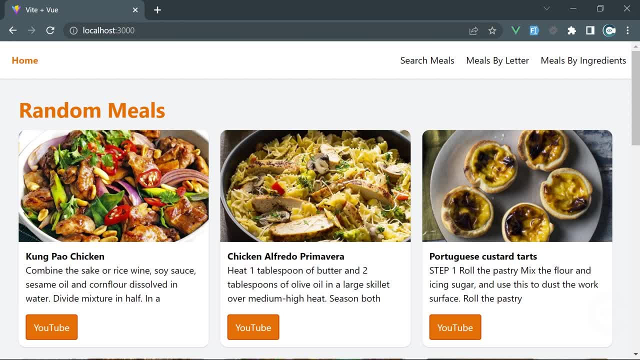 So I think it's good time so that if you're new to my channel hit the like button and hit the subscribe button and enable notifications. All right let's jump into this video and build this 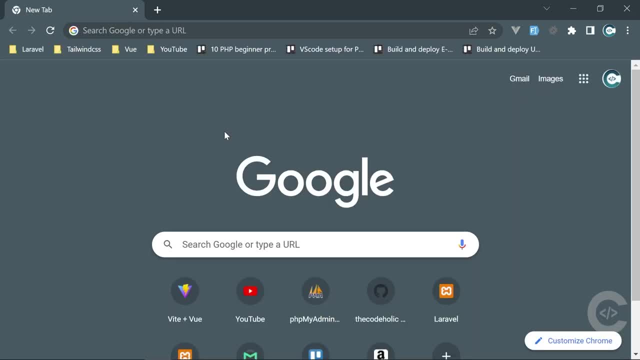 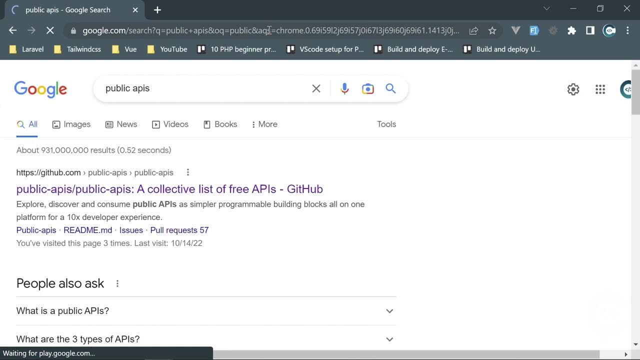 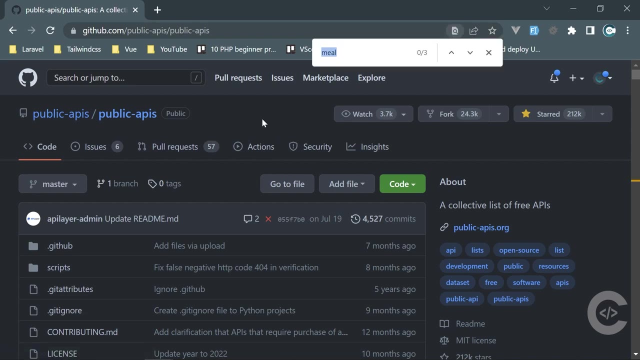 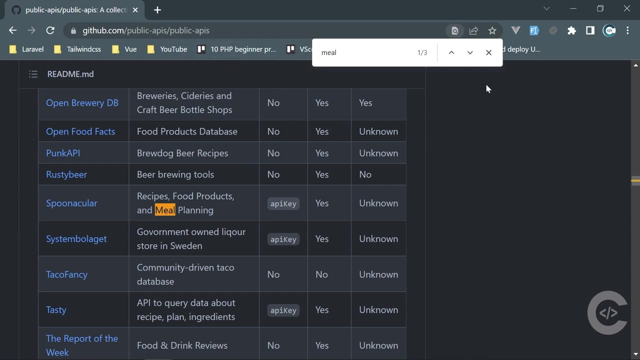 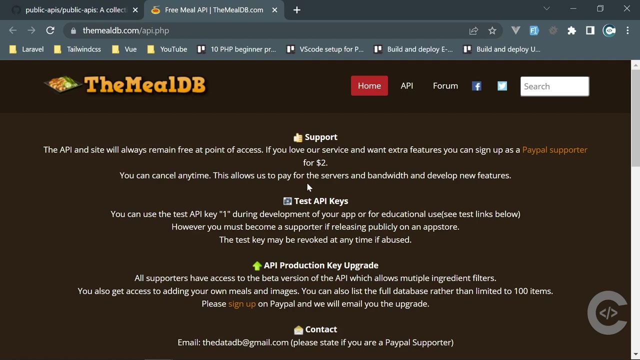 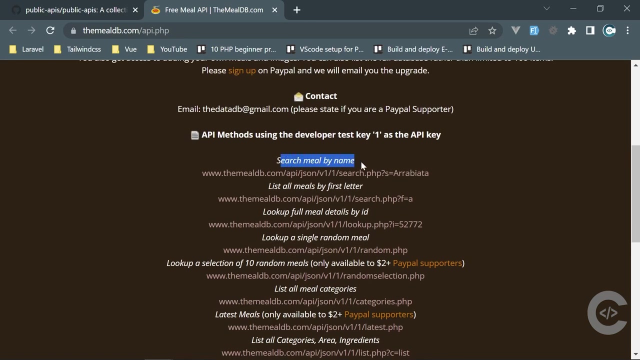 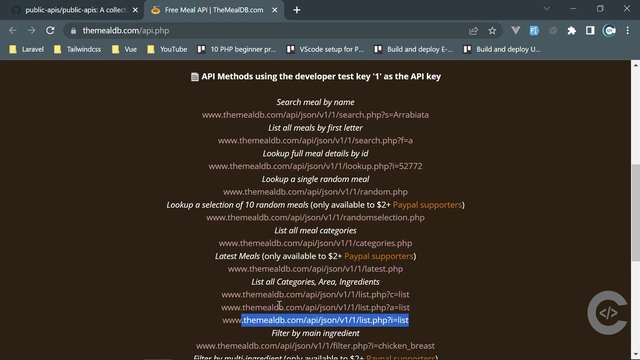 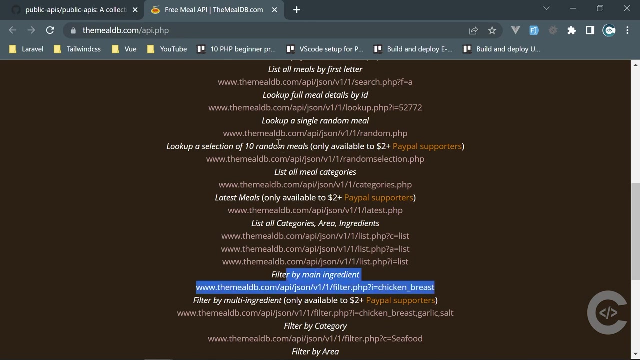 nice Vue.js application. Now let's start building our Vue.js application but first let's have a look at the API we are gonna use. Let's search in the Google public APIs and the very first link which is the repository is what we need. So right here inside this repository we're going to search for meal. This repository is an excellent repository for public APIs. Let's search for the meal db and this is what we are going to use and this is free API for searching meals and we need the following endpoints. We need search meal by name. We need to list all meals by first letter. We will need look at full meal details by id and we will need to list all ingredients which is the following endpoint and we will need to filter by main ingredient which is the following endpoint. Okay all of them are free however it has a couple of other endpoints which supports two plus dollar paypal support. 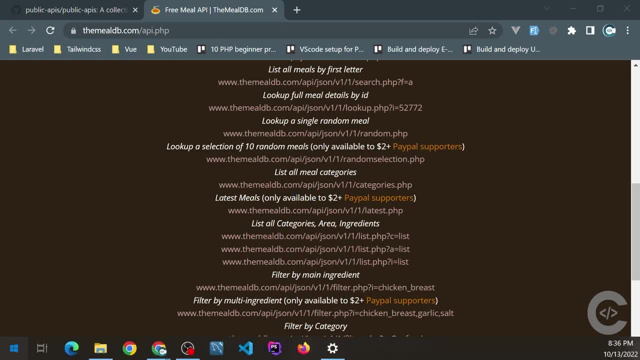 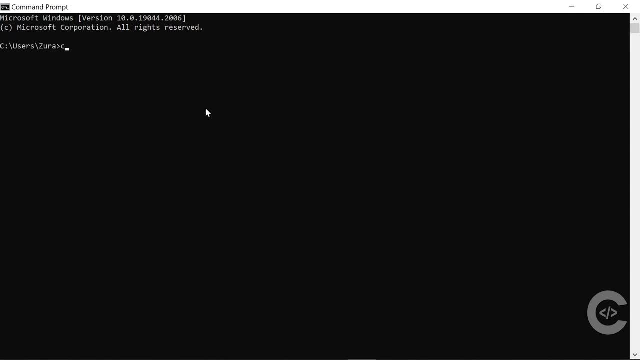 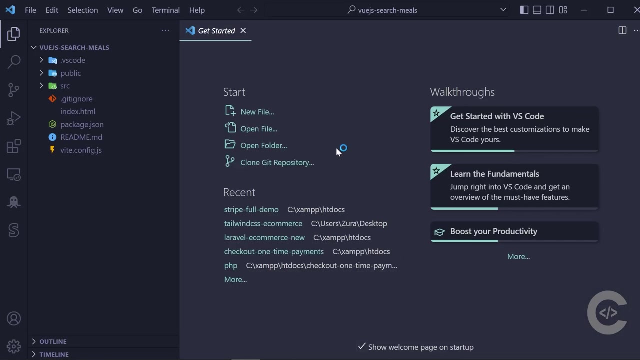 All right now let's create Vue.js application. So for this I'm going to bring up cmd and navigate into www folder and create my project right here but first make sure you have node.js and npm installed and available. If you don't have go node.js.org and download a node.js for your operating system. I already have them so npm command is available in my terminal and I'm going to create new project by executing npm create write at latest. So I'm specifying the latest version for white to create new project and let's give it name Vue.js search meals. Let's hit the enter. I'm going to choose view javascript and now I'm going to navigate inside Vue.js search meals and open this using vs code and I'm going to close the cmd completely. 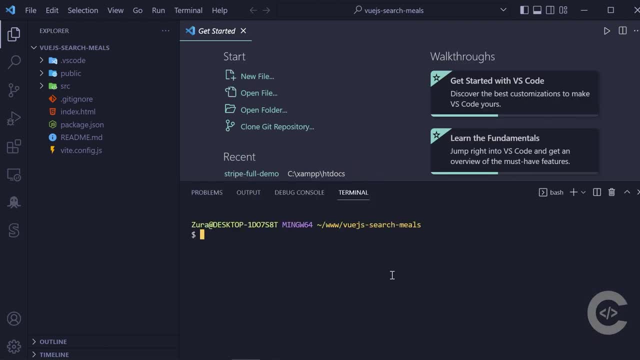 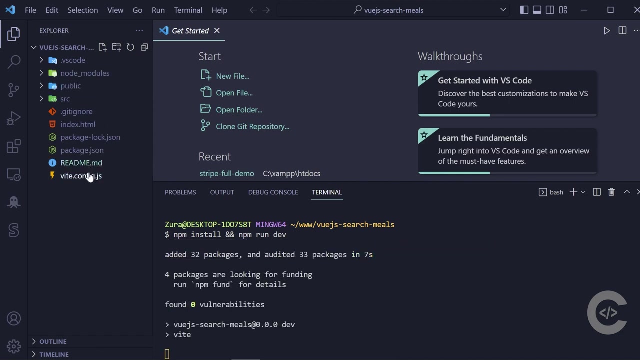 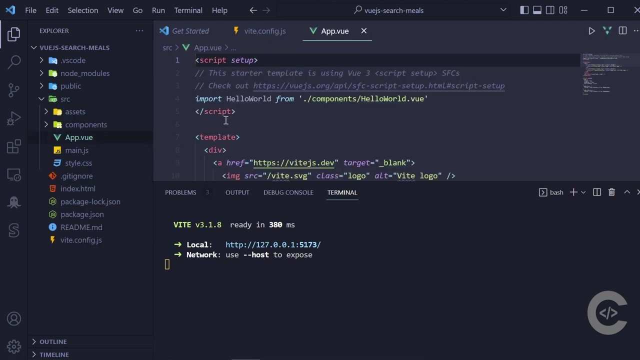 Okay now right here I'm going to open terminal and run npm install and npm run dev. It's going to take few seconds until this is installed meanwhile we can have a look at the repository we have package.json we have white config file which contains white configuration options we have source inside there we have the main component file which is app.vue we have main.js css and inside the components we have hello world component. 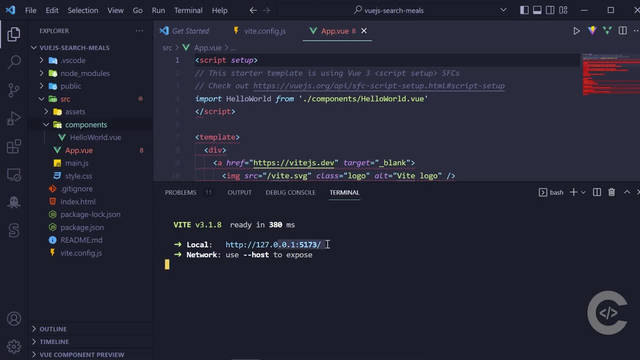 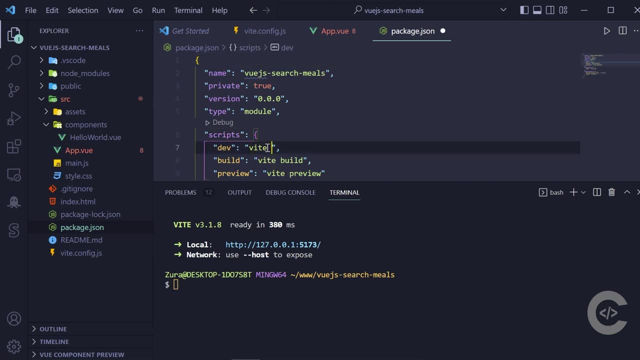 All right this was already started. But I want to start this on port 3000 so I'm going to kill this. I want to open package.json and specify right here dash dash port equals 3000. So I save this and I'm going to run npm run dev which will now start the server on port 3000 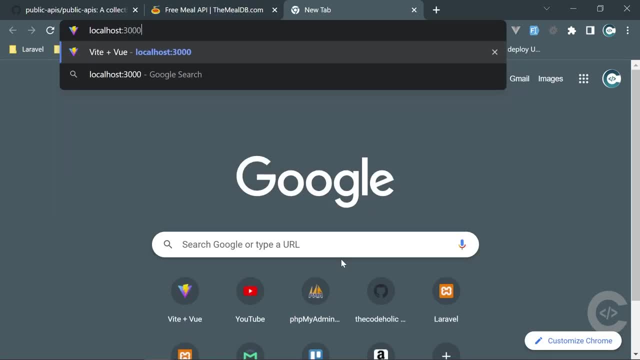 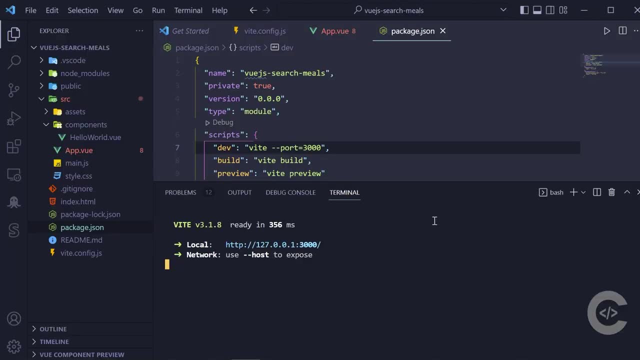 and in the browser I'm going to type localhost port 3000 and this will show me byte plus Vue.js application running and this counter also works. All right let's clean up a few things. 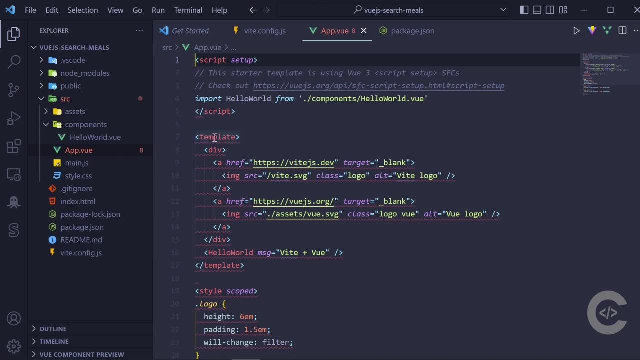 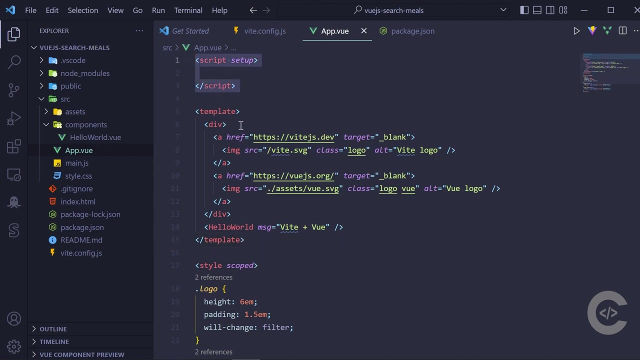 If you go in the app view first of all we see the errors the errors are coming from the Vue.js extension it thinks that we have JSX expressions which complains that we need to have only one element inside this template so but surprisingly if I just remove this if I just yeah if I remove this everything is basically okay and if I just put this script down this is I how I prefer okay. 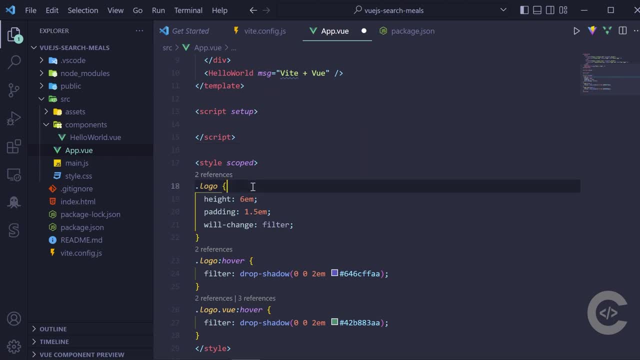 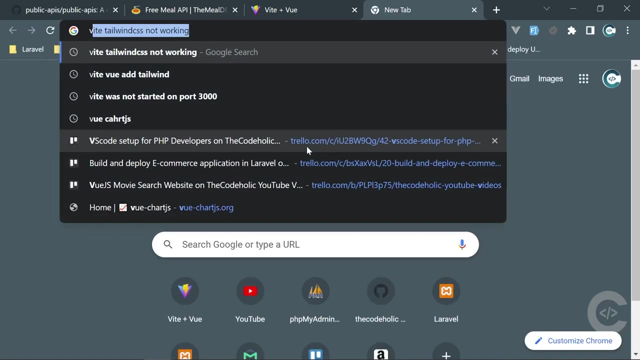 have i prefer to have template and then script and as for the styling i'm going to remove everything from here and let's remove everything from here as well this is now a plain component absolutely empty component and we can just type app.view and save that and we see app.view let's clean up some css as well from style css and let's remove this hello world component as well all right now let's add tilewind css so i'm going to look for vite tilewind css and let's 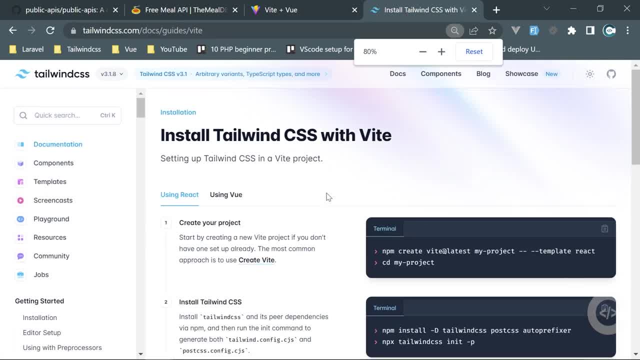 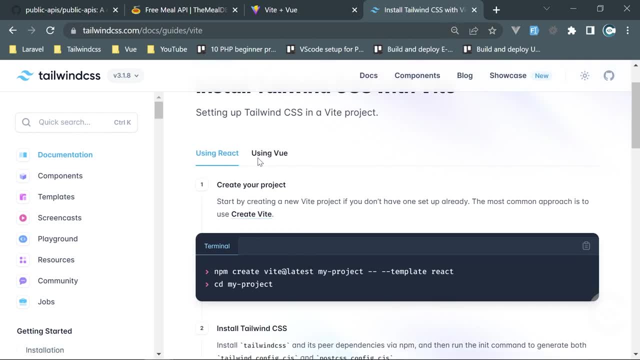 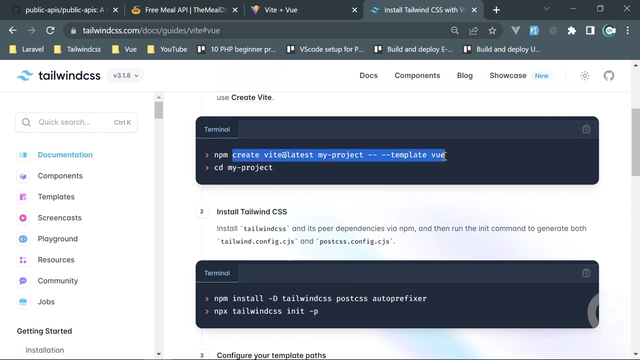 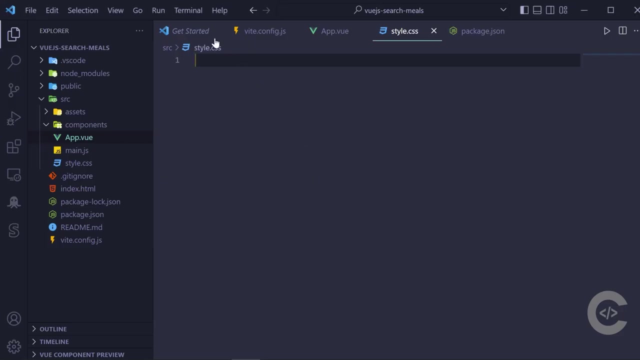 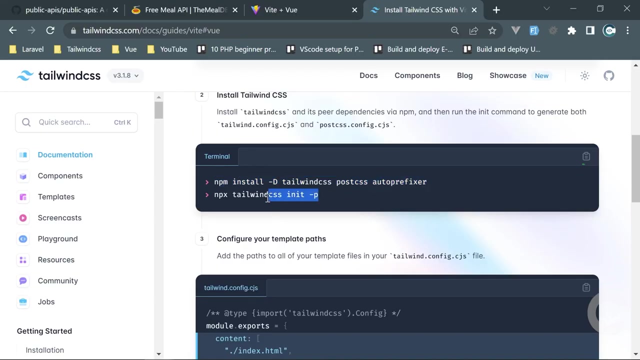 install tilewind css with vite and this is the official tilewind css documentation here we have the using react section but we are using view so we're going to click on this using view and let's scroll down below we already have a project generated so down below we're going to copy this to install tilewind css and we're going to copy this to install tilewind css and let's see what we're going to do here so i'm going to copy this to install tilewind css post css and auto prefixer so i'm going to bring up a new terminal and install that actually i can delete this and open the existing terminal just kill this process npm run dev install that and hit the enter and then we need to initialize the tilewind css configuration file but make sure you have 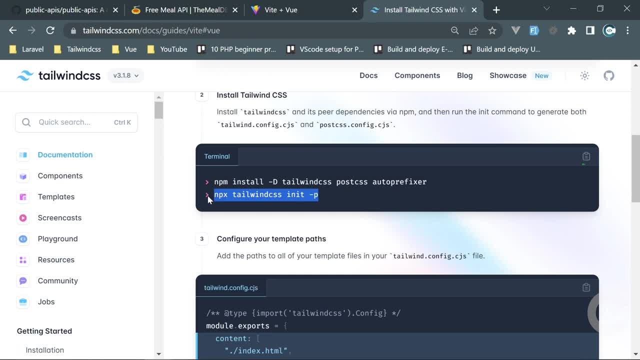 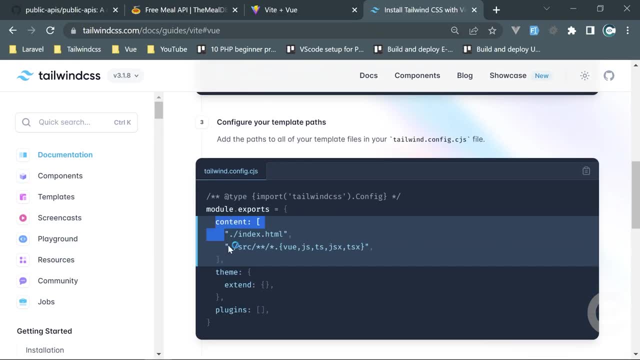 specified dash p as well because we need post css file as well otherwise it might not work so let's this and hit the enter and down below we need our content to be modified like this so i'm going to 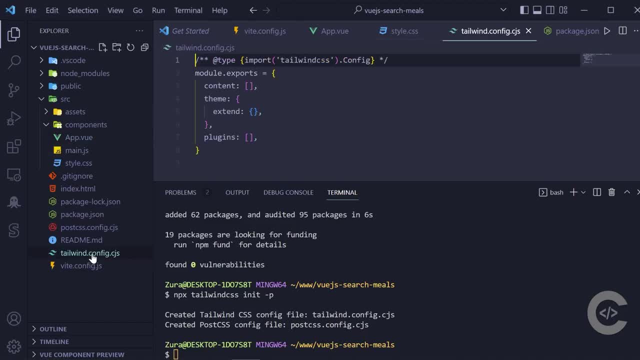 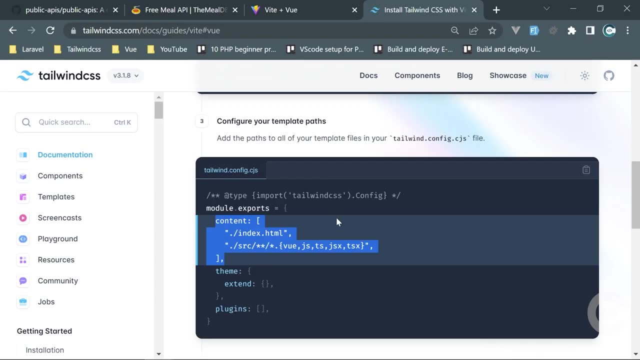 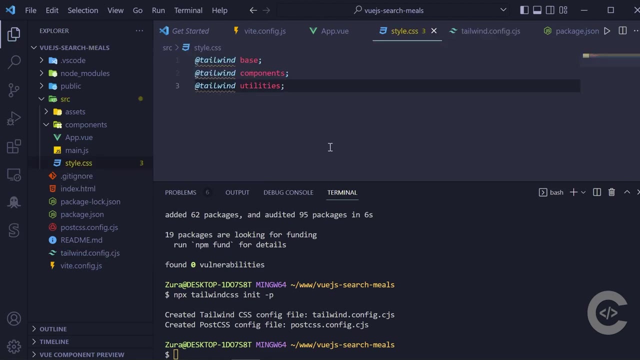 copy this content and open tilewind css config file and replace this content with our specified content so we save this and the last thing we need to do is to copy these directives open style css and paste them right here and now we can already add run the server and edit tilewind css classes so if we open 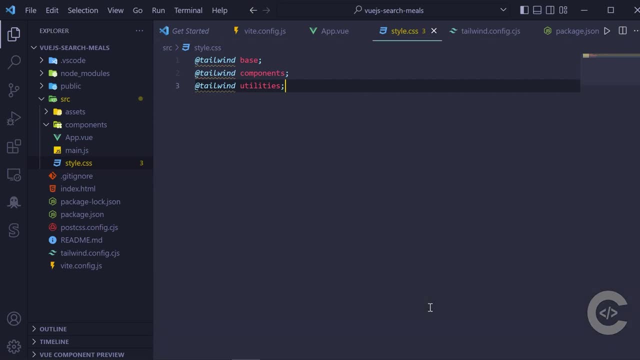 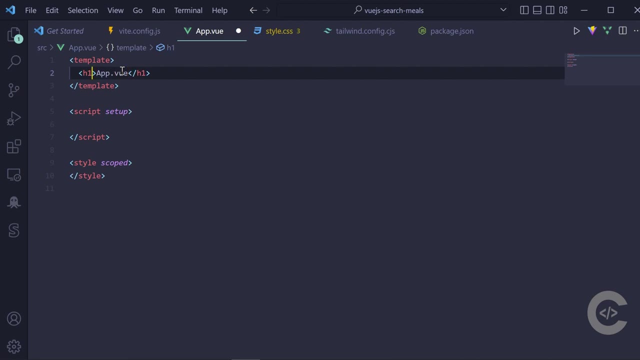 let's start the server npm run dev and now i'm gonna open up view and put this in h1 maybe and let's give this class bg blue 500 for example so we save this 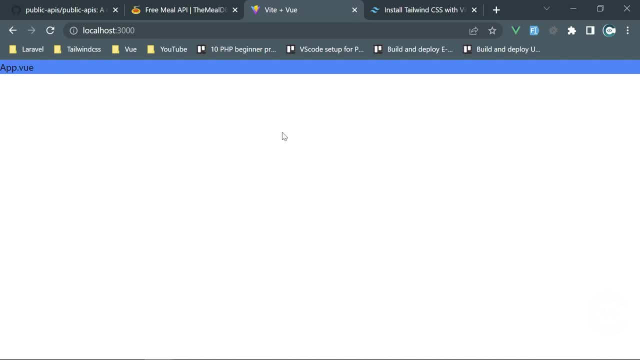 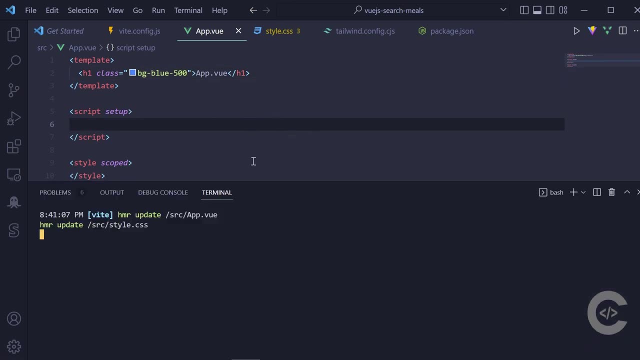 and have a look in the browser and we see this this is blue all right so tilewind css is installed now let's install view router for this i'm going to bring up the terminal 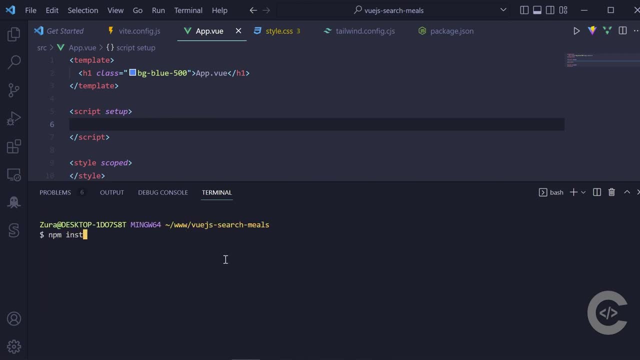 let's close this and i'm going to run npm install view dash router and we're going to specify a version right here if i specify next this can install the latest version at the moment while i'm recording this the latest version is four point something if you are gonna watch this 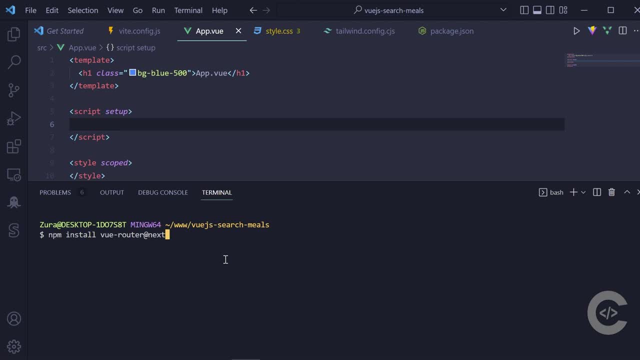 tutorial after one year the next version might be view rotor six and if you install sixth version it is going to have some problems so basically uh i prefer to run a specific version like version four in this case and let's hit the enter 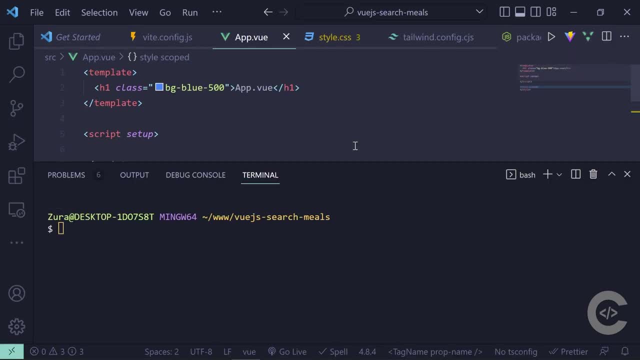 all right so that was successfully installed actually i can't even zoom in and for like 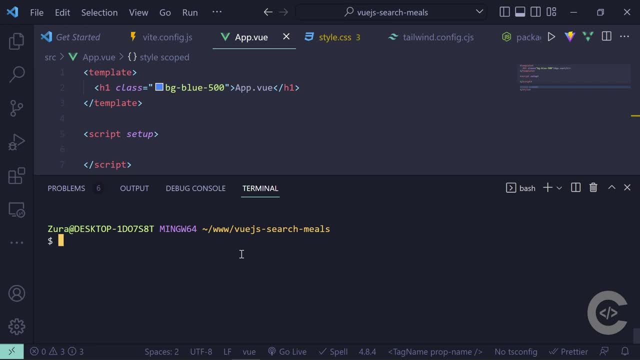 for viewers who are watching this on mobile so we have a view router installed and let's start the server now 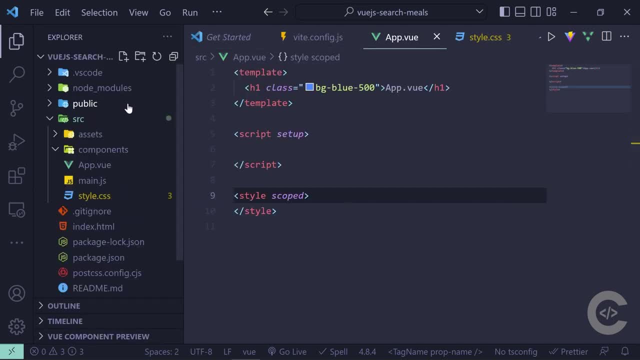 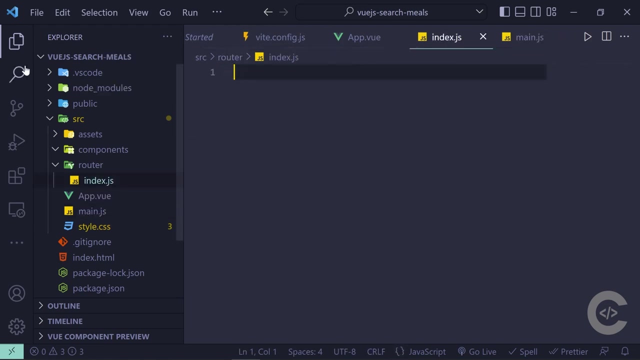 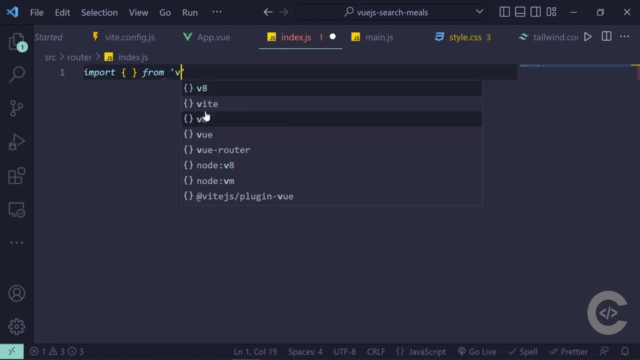 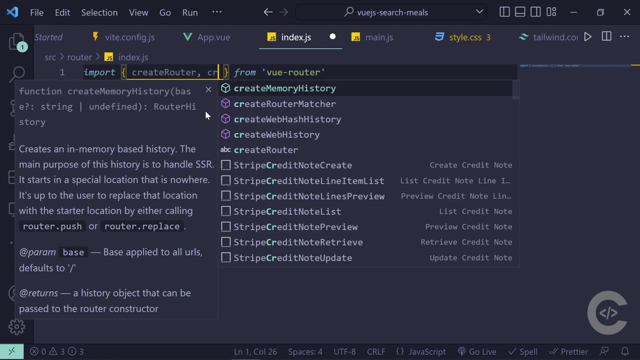 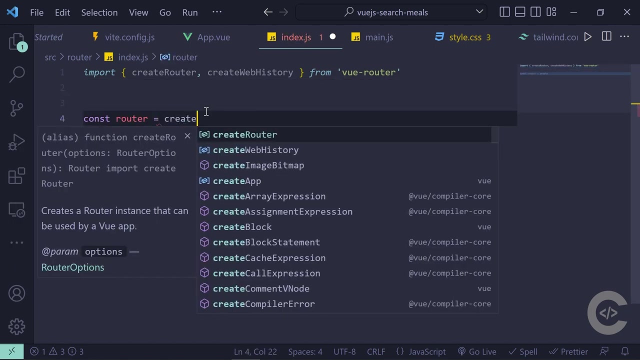 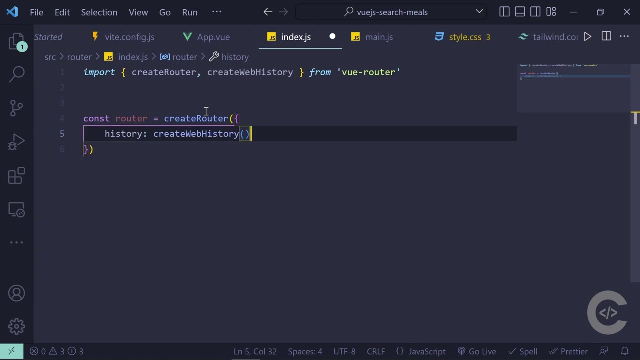 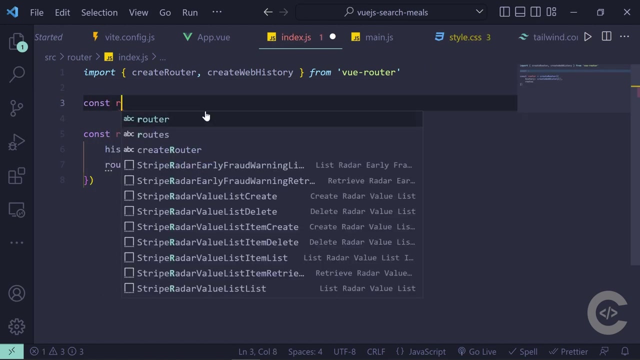 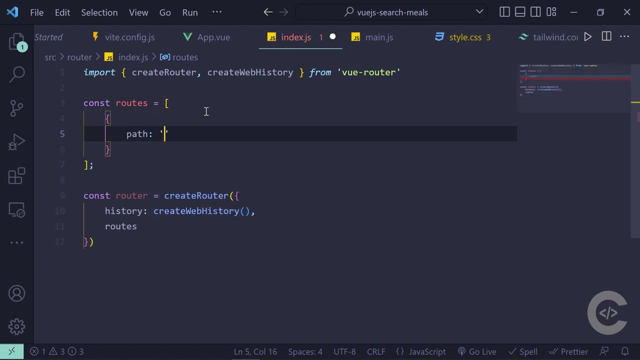 let's go to the terminal and we're going to create the router file under source folder i'm going to create new file which will be under router folder index.js let's hit the enter and right here we're going to create router and then export it and then we're going to import this in the main js so let's go in the router index and we are going to import uh from view dash router and we're going to import create router and create web history okay then down below we're going to create router equals create router we're going to specify history right here to be create web history and we're going to specify routes right here as well okay but let's define those routes const routes equals an array okay and we will need to define right here path to be slash we need name to be home this is the first route and the component needs to be home component which doesn't exist yet but we're going to create that soon so we have routes variable and we're providing routes right here and finally we're going to export default router from here all right so the indentation is set to four spaces which is i'm going to quickly fix i don't like 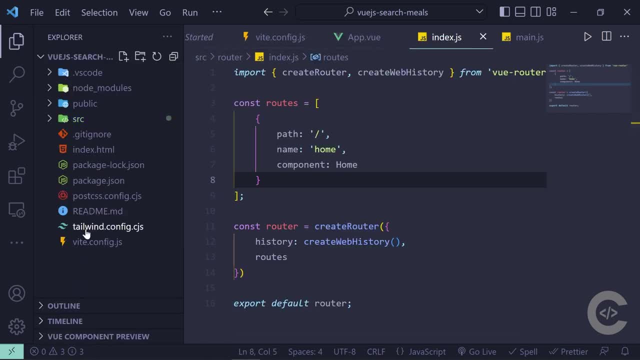 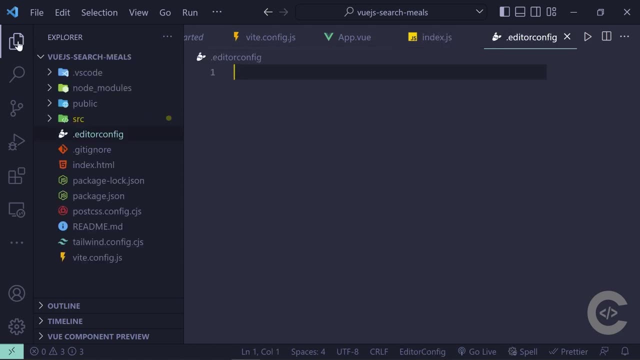 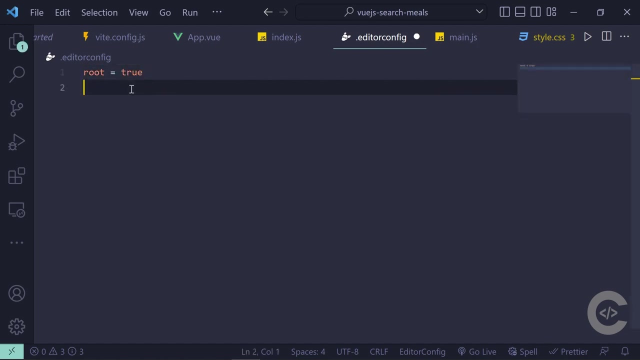 four spaces so i'm going to open the project explorer and create new file called editor config file if you don't know what's editor config file check my video which will appear in the top right corner and we're going to set route to be true we're going to set for every file basically indent size needs to be two and tab size needs to be two as well and we can set a chart set to be utf-8 as well 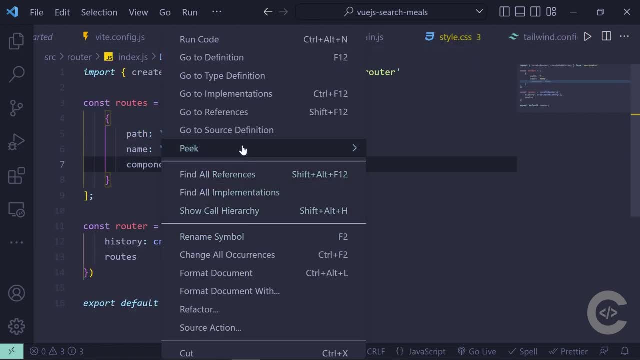 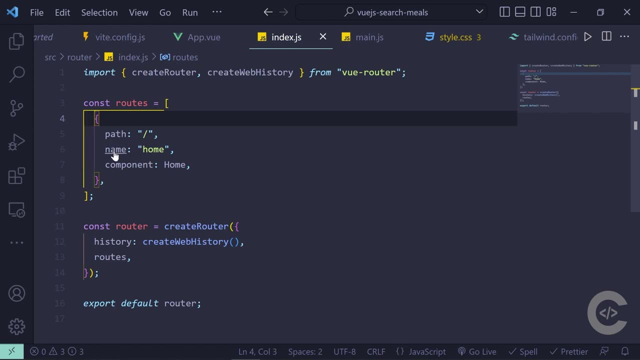 so i save this and now if i format the code where is format okay now that was formatted nicely and now tab is for set into uh two spaces all right so we exported router now let's go in the main js and i'm going to import router right here import router from router and after we create our application we're going to use our road 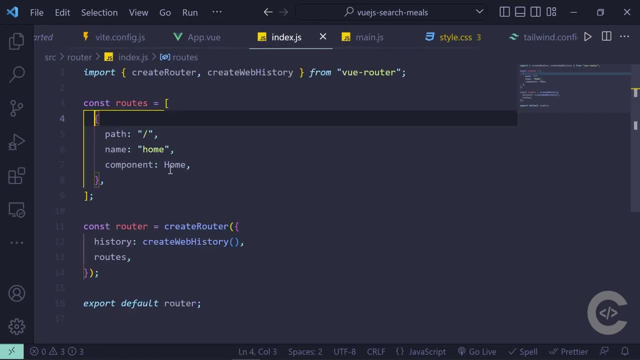 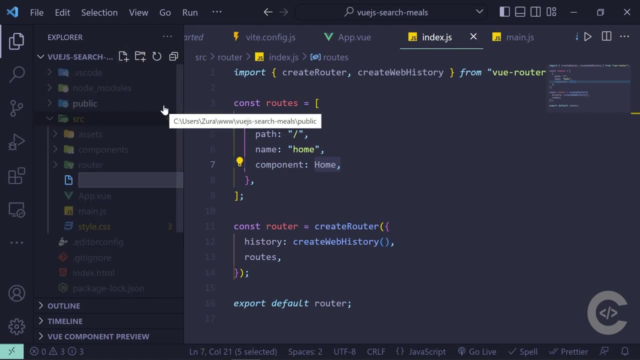 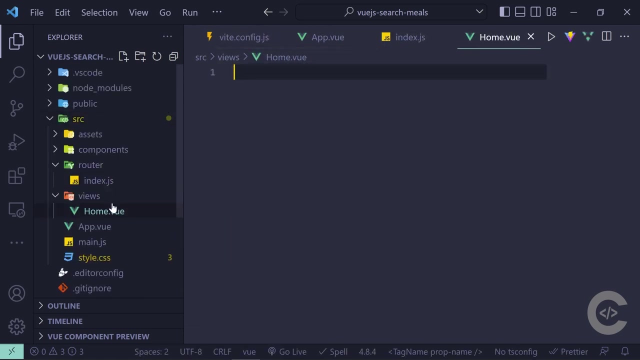 router as well okay now everything is set up except this home component which doesn't exist in the source folder i'm going to create new file but i'm going to create this inside subfolder called views home.view okay so basically i create separate views folder for those components which are associated to a route okay and inside the components i have more like smaller components which are used in the home component so i'm going to create a new file and i'm going to create a new 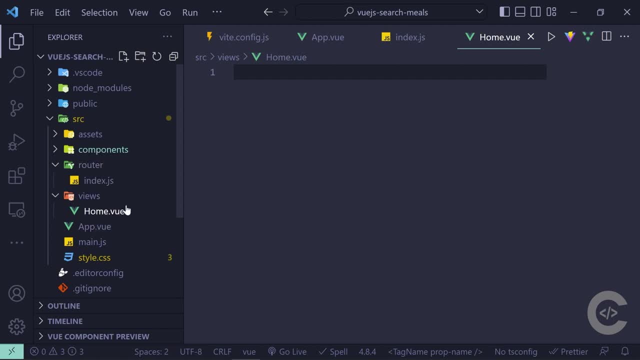 file inside the views or in another components all right now i have this home and i'm going to 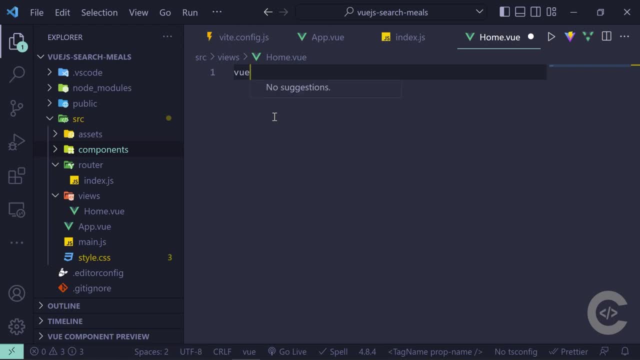 generate the template let's actually quickly create template we will need script tag and we 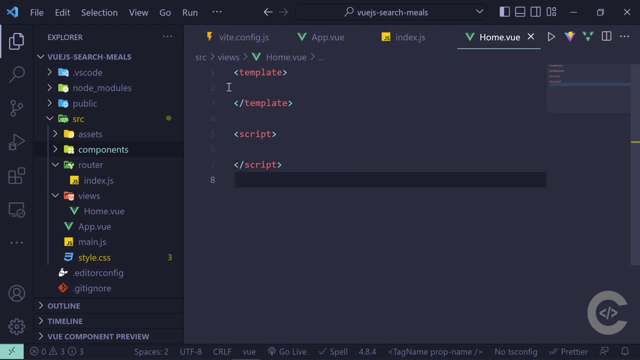 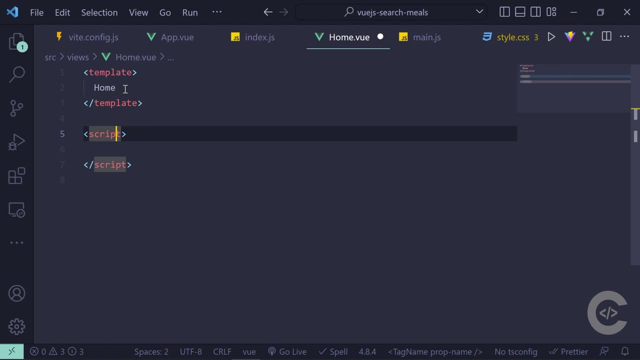 will need style no we can leave this style we're using tile on css we might not even need that and right here let's just write home for the script i'm gonna 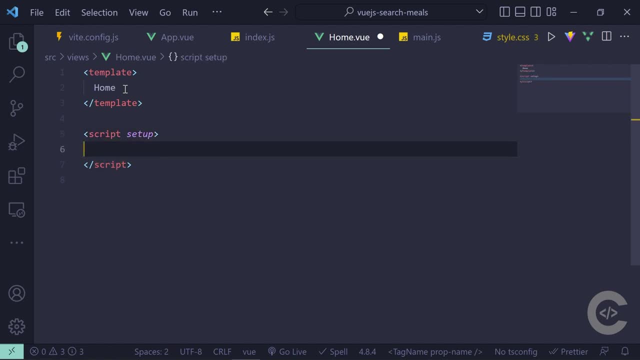 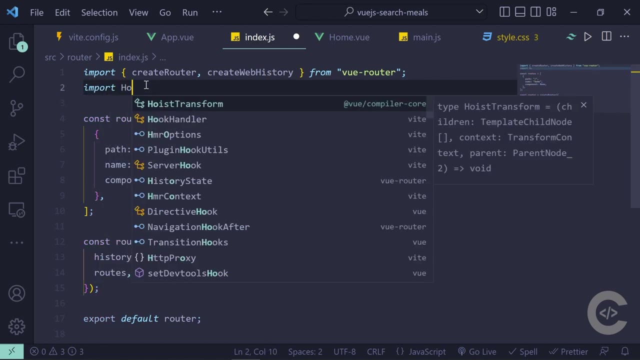 give it a setup attribute because i want composition api and now if we go in the router we're going to import this home so import home from let's go one directory back under views 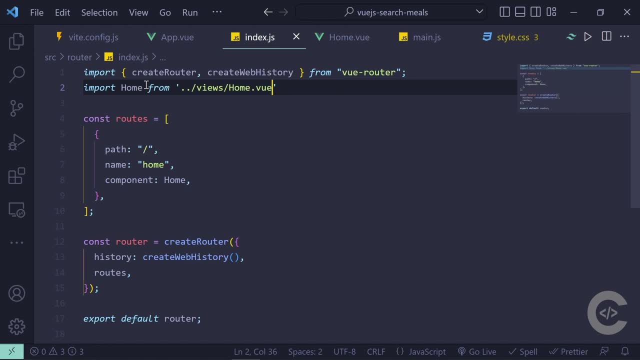 folder and the component is called home.view so we save this and the last thing is to go 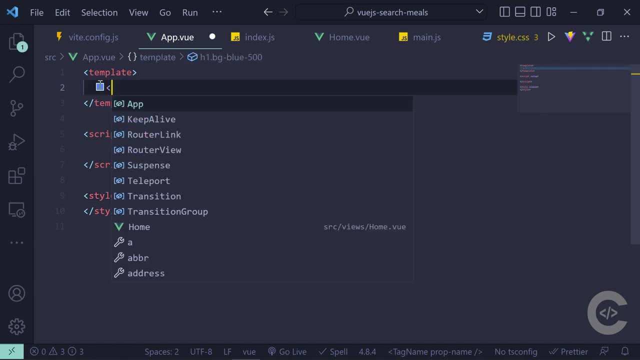 in the app view and remove this and we're going to use router dash router view router view all right so we have this router view let's save this and now let's have a look in the browser and we see home right here okay so this is coming from this home component now let's remove 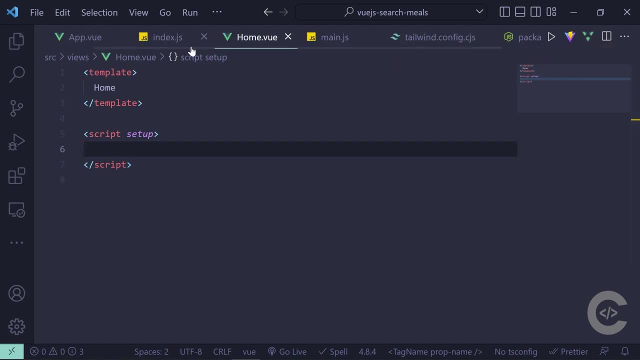 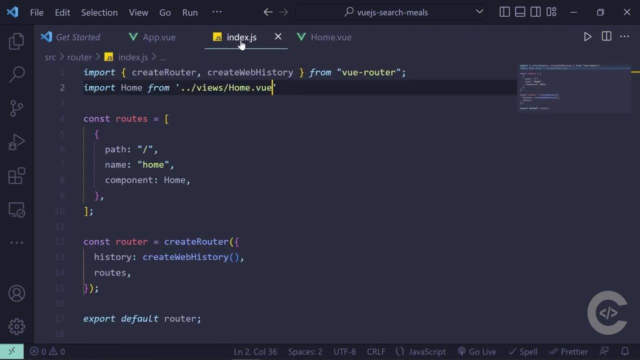 a few things i'm going to close this style uh white config tile resistance config as well we don't need main js yet and the package json as well okay and getting started as well nice so now 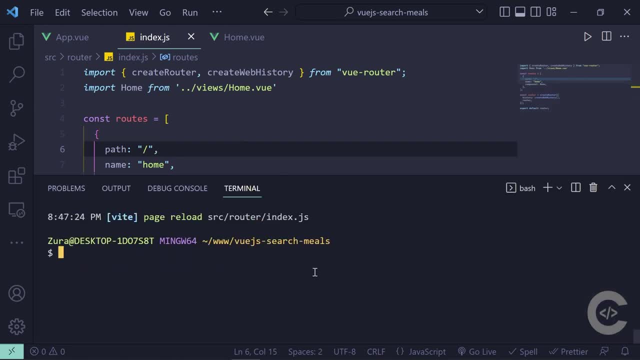 let's install viewix let's bring up the again cancel this server and we're going to run npm install view dash view x excuse me view x at 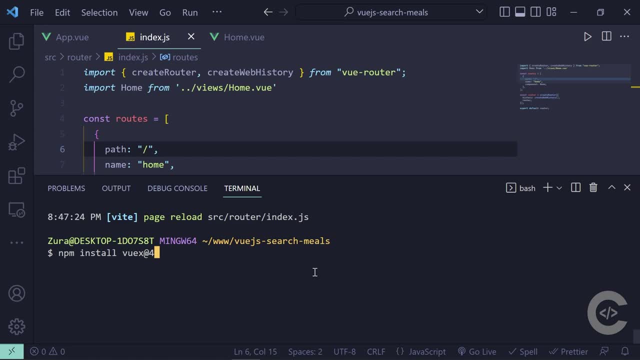 and we're going to again specify right here version 4 and i'm going to specify dash s not sure if i specified this when installing the view router but i'm going to check this so view x was 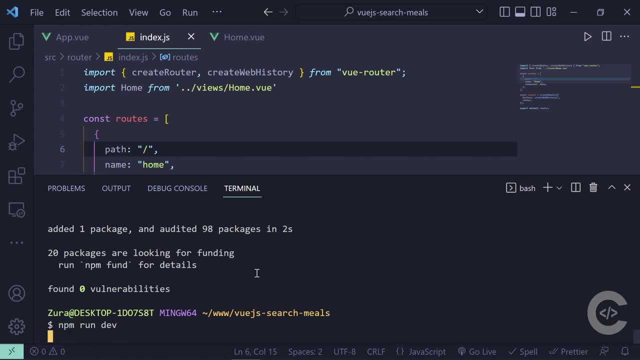 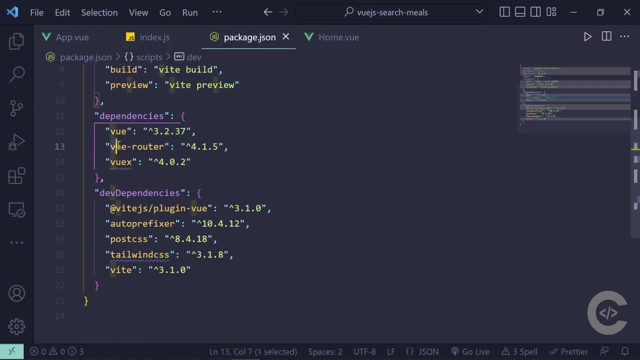 installed now let's run npm run dev again and close this terminal and now let's open package json and have a look view router is added right here which is fine okay now view x is also 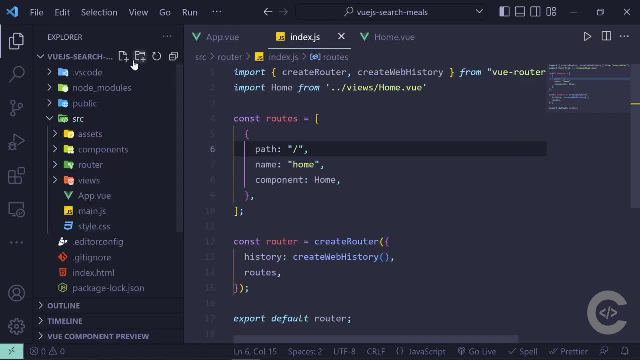 installed and i'm going to create now store in the source folder i'm going to create a file called index but that's going to be under store slash index.js and in this case we are going to run npm run dev again and close this terminal and now let's open package json and 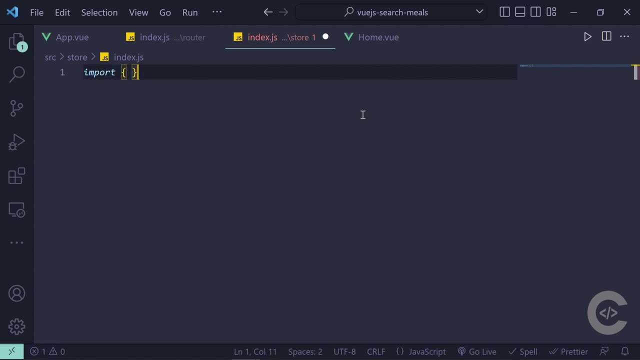 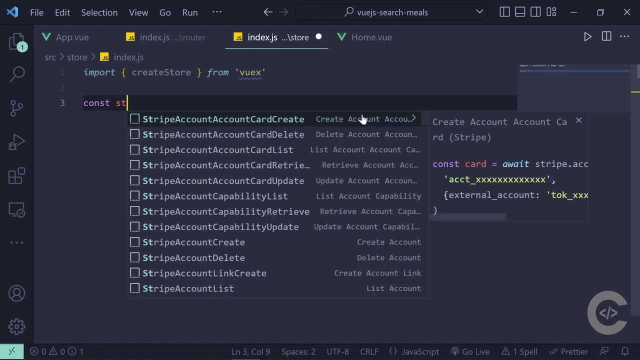 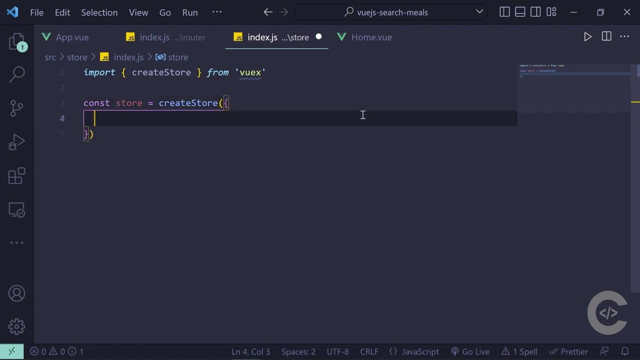 going to import from Vuex, and what we are going to import is called createStore, not logger, createStore, okay? And we are going to create the store, const store equals createStore, and we're going to specify right here actions and mutations, so let's specify all of them, because I'm 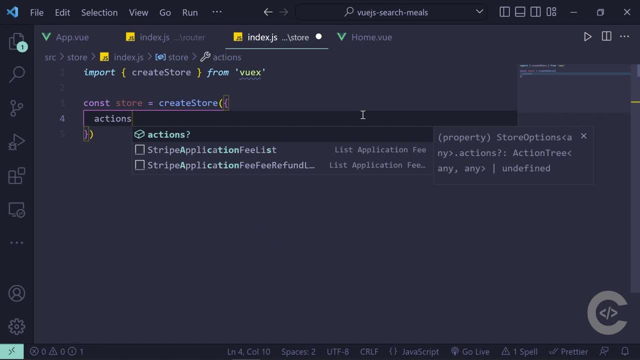 going to create a modular and flexible project structure which will scale up, scalable, that's the word I wanted to say. 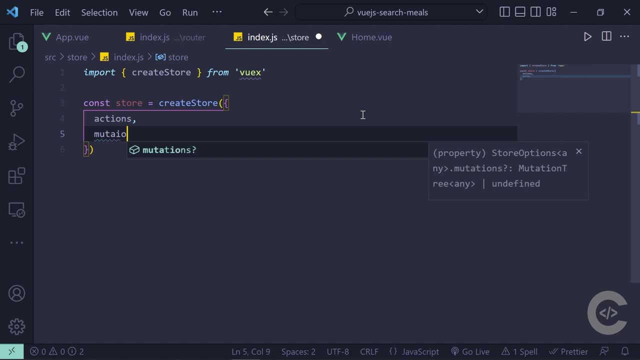 So we're going to have actions right here, we are going to have mutations, we are going to have getters, and we're going to have state at the very top, okay? 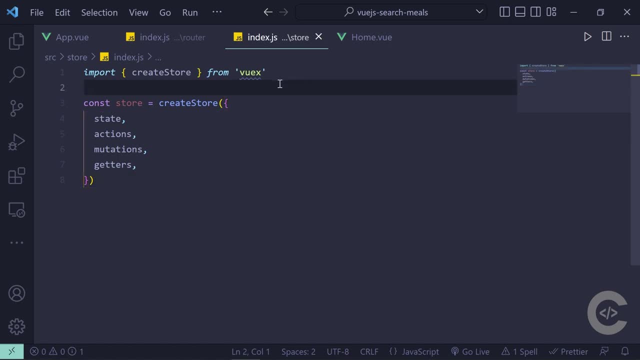 So these four properties, but we have to define those properties, so basically I'm going to go inside store and create. 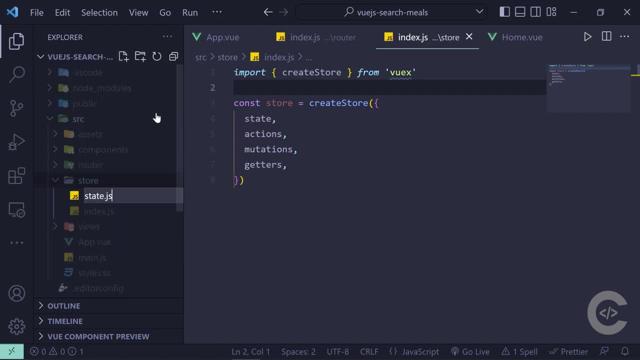 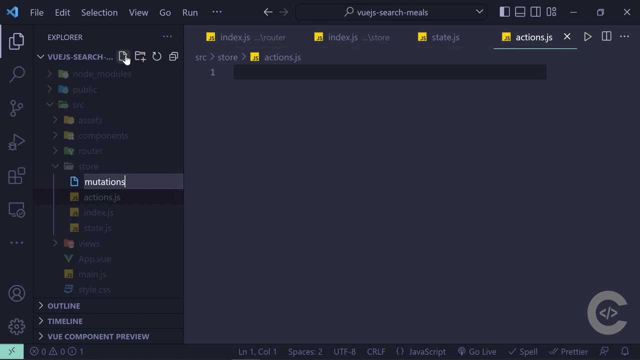 Those files, state.js, we are going to create actions.js, we're going to create mutations.js, all right? 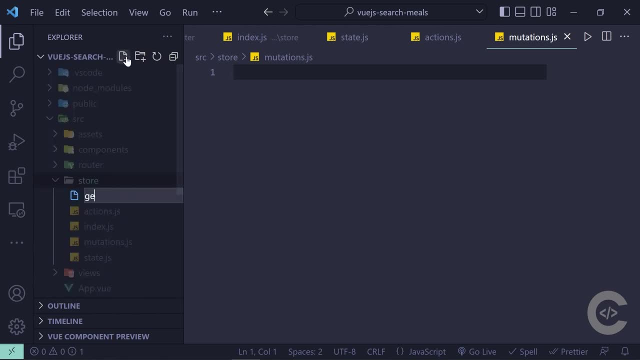 And what else? I think we need getters, getters.js, all right? 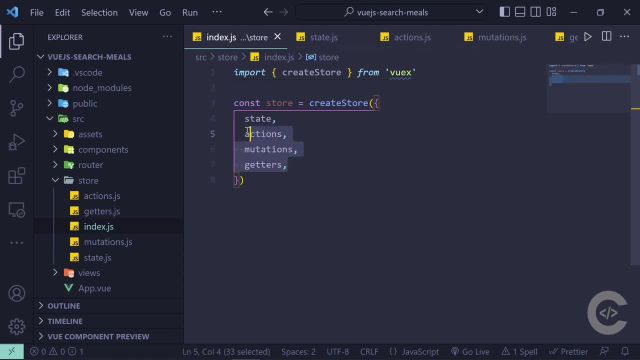 We can have everything inside the index, but the reason is that we're going to create something scalable. 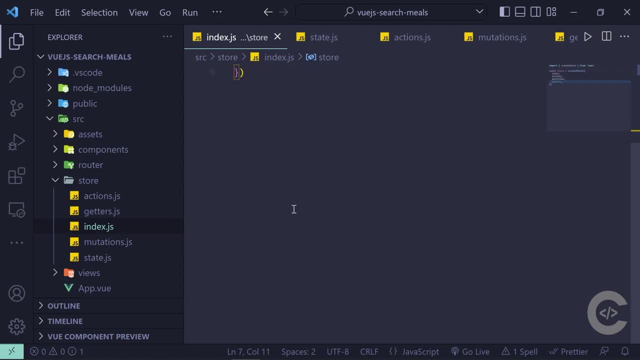 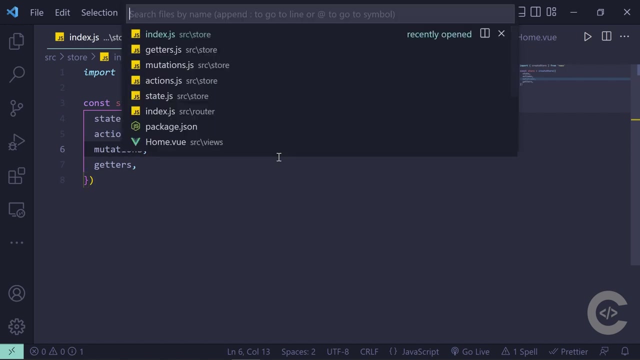 So if our application grows, we're going to have a lot of things inside the index, and we're going to have hundreds or maybe thousands of lines inside a single file, but right now we are separating these into multiple different files, and it's going to be also very easy to find them, because whenever you have the left side collapsed, you're going to bring up the search files using ctrl and p and search for actions or mutations or getters, whatever you want, right? 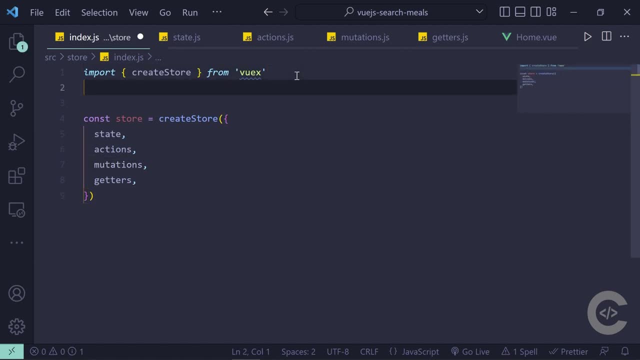 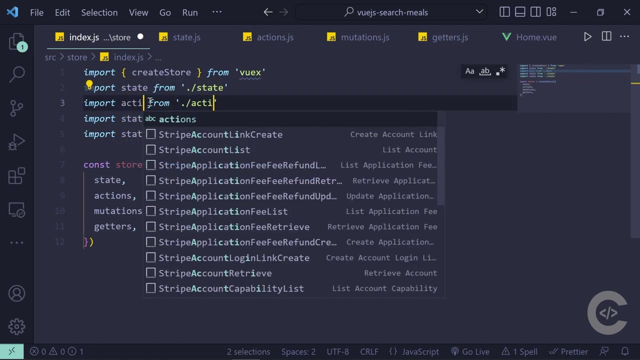 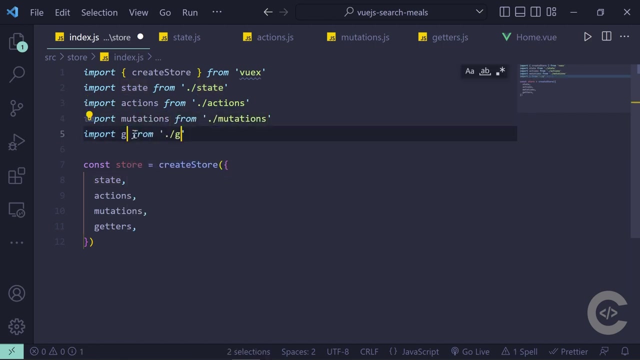 So now let's import those files, state and actions and mutations and getters. So import state from state, and let's duplicate this, and we need import actions from actions, we need import mutations, and we need import getters, all right? We have all of them. 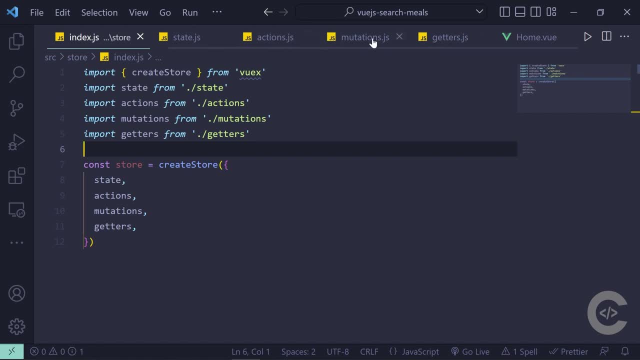 Now I save this, and let's see if we can close a couple of files. I think we cannot close. Finally. 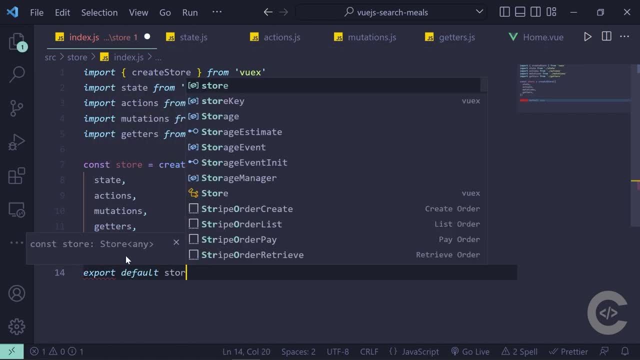 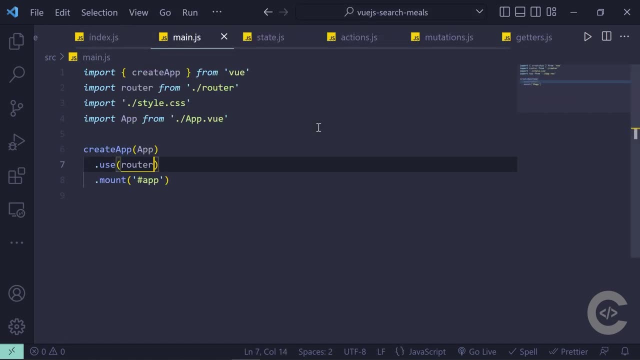 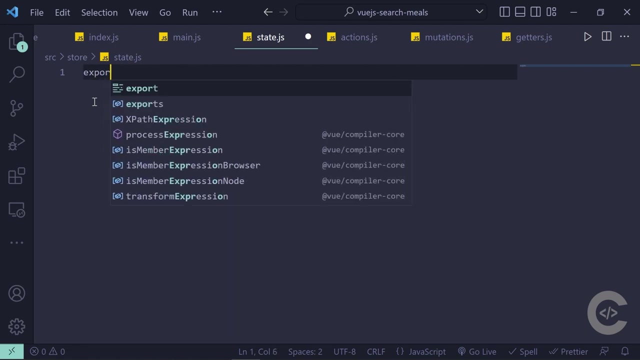 So I'm going to export a default store from here, and then I think I can close this file and go in the main.js, and we are going to import store from here, and just like we are using router, we're going to use store, all right? Now let's go in the state and define state right here. We're going to export default object from here, and that object will have some state, for example, meals, which is going to be an array, and let's say right here, salmon. 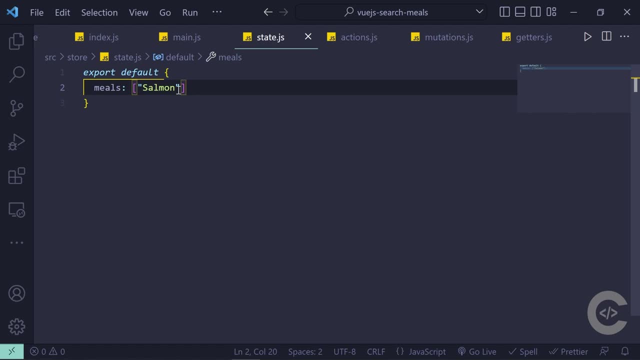 I know this is not a meal, it's an ingredient, but let's put it right here. 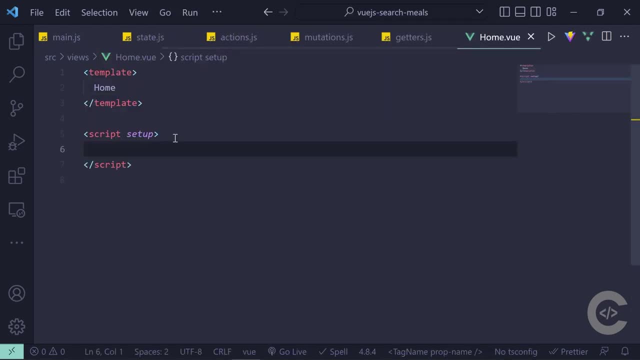 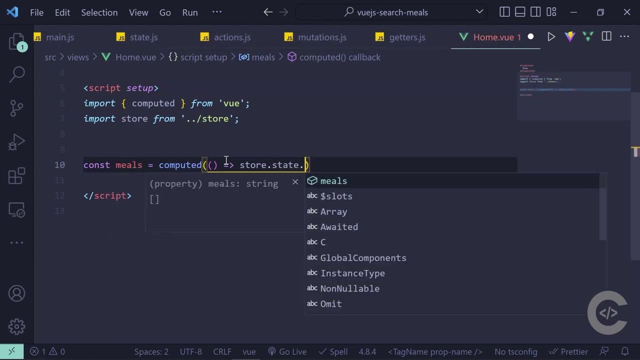 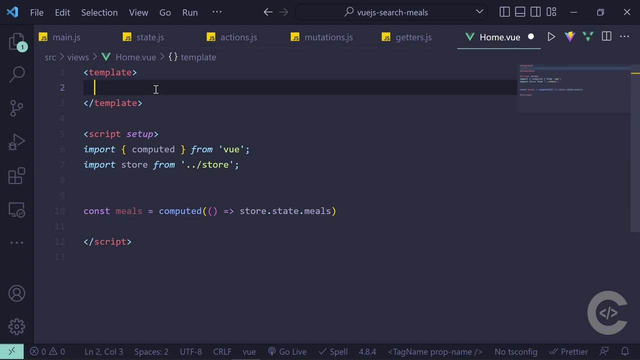 Now if I go in any components, like home.view, and I'm going to create right here computed property, computed variable called meals equals computed, let's hit the enter. That was imported from view reactivity. But I think it should be imported. It should be imported just from view, okay? Now we have this computed, and right here, we need callback, and we have store as well. So from store, we are going to take state, and from that state, we're going to return meals, all right? Now these meals will be outputted in the template, and let's actually create pre-tag and output meals right there. So I'm going to save this. And let's have a look in the browser. 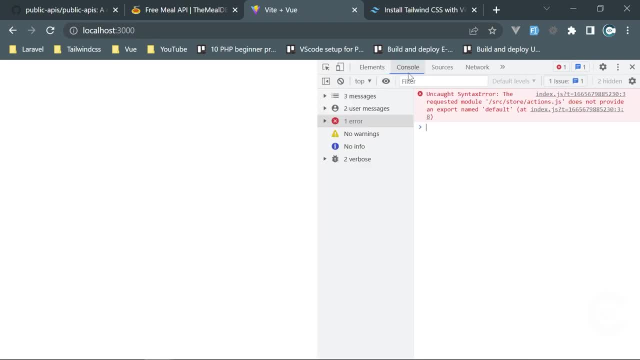 Okay, we have some kind of error probably. If we go in the console, we see store, source store actions, JS doesn't provide an export name default. That's correct. 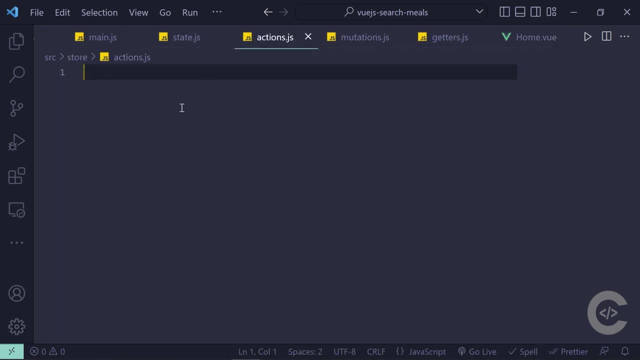 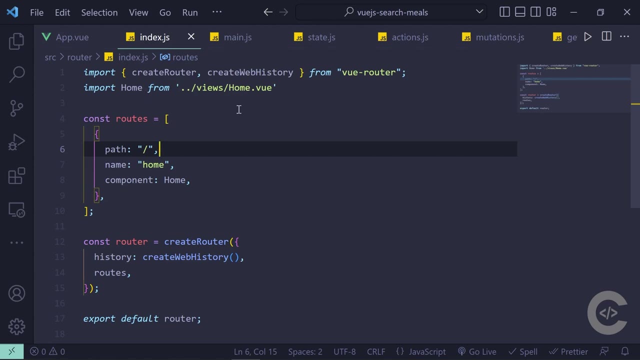 If we go in the actions, nothing is exported from here. What we need to do is to go in the index and go in the store slash index, and we need to import them. 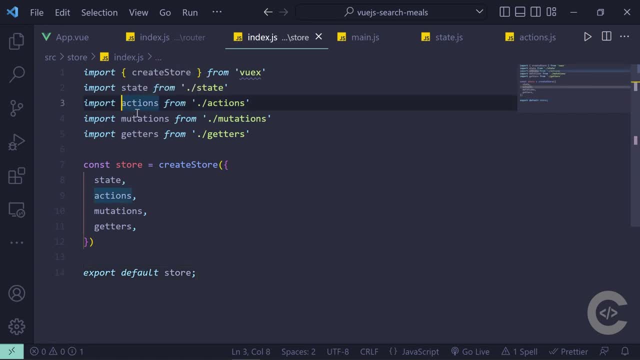 Like in a different way, okay? So we're going to import everything as actions, everything as mutations, and everything as getters. 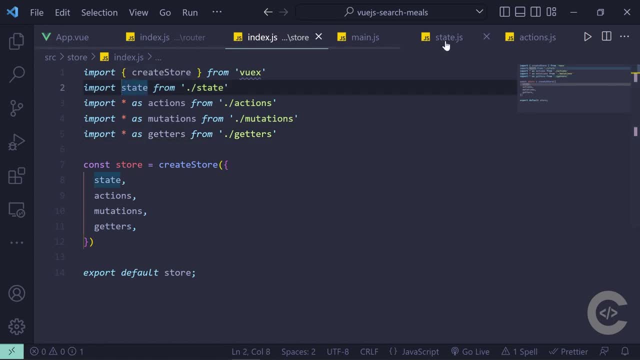 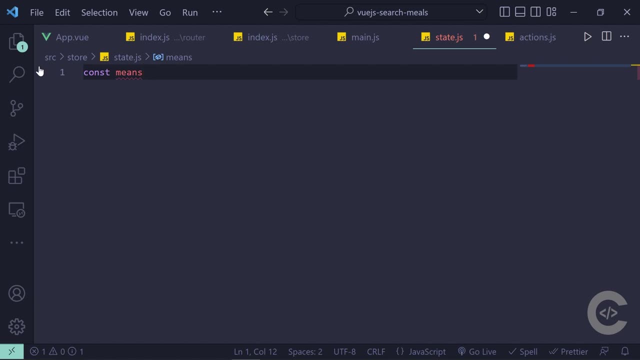 Like we can do the same approach, everything as a state, but in this case, we have to create separate objects. Like we can do const meals, for example, or export const meals. Oops. A lot of them. Okay. Hold on. 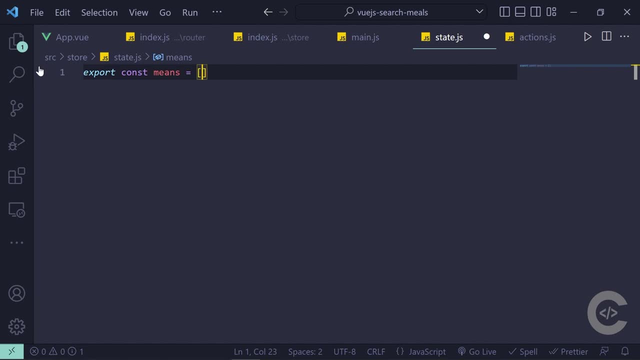 Export const meals equals the following array, and we have Salmon right here. Okay. We can do even like this. 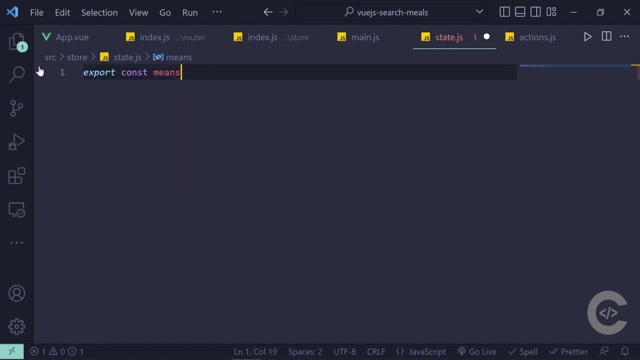 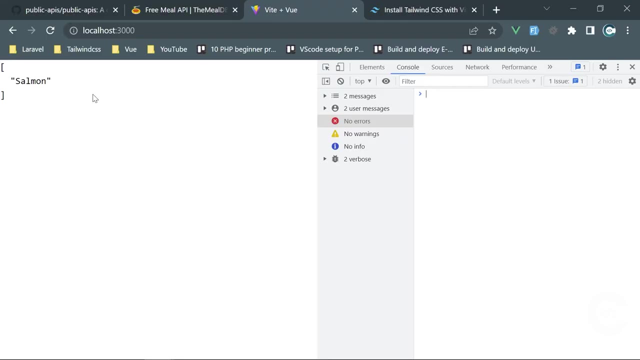 But I prefer to have export, let's undo actually, export default object like this. All right. So now we have this, and let's check in the browser, and here we see Salmon. Okay. This is coming from Vue X. Okay. 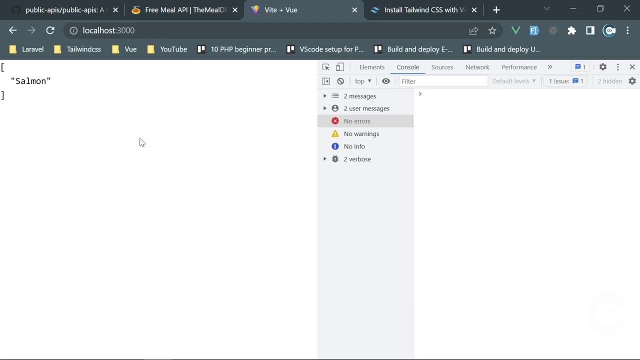 We installed Album CSS. We installed Vue Router. And we have Vue X also saved. 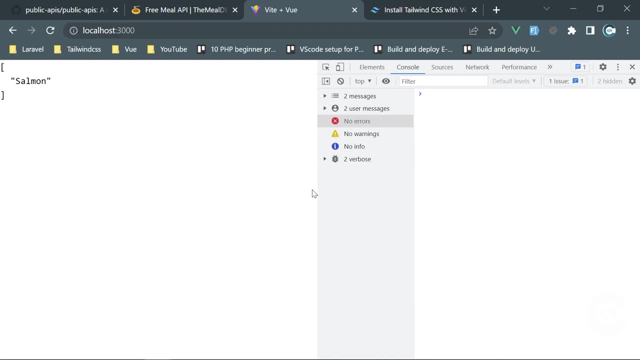 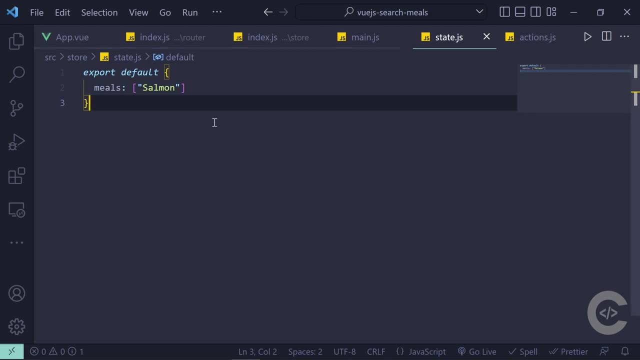 Now we can start building an interface and making requests into this API. Let's go in the, let's go in the home and build up some interface right here. 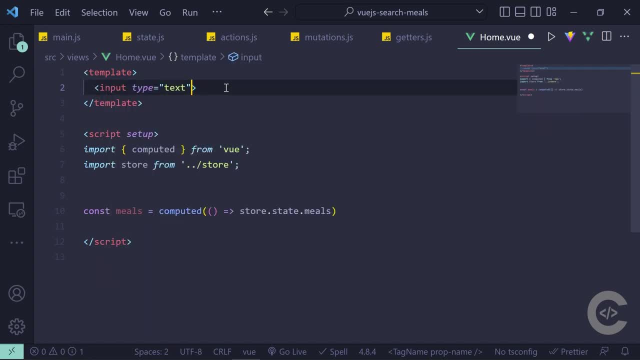 So first we're going to have input type text, which will be for search. Okay. 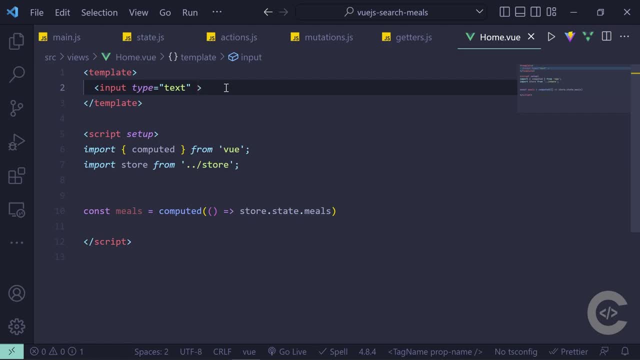 And for this, we're going to also install Tailwind CSS forms. 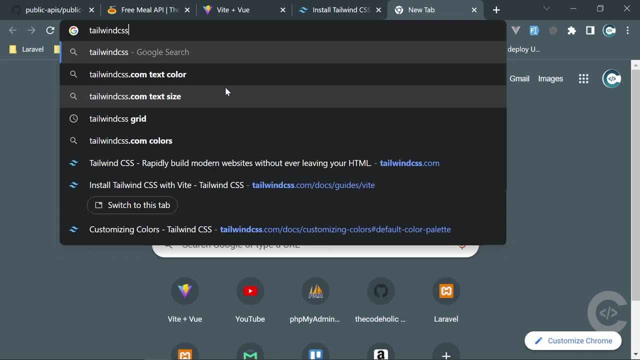 Let's go in the browser and search for Tailwind CSS forms. And this is the package. 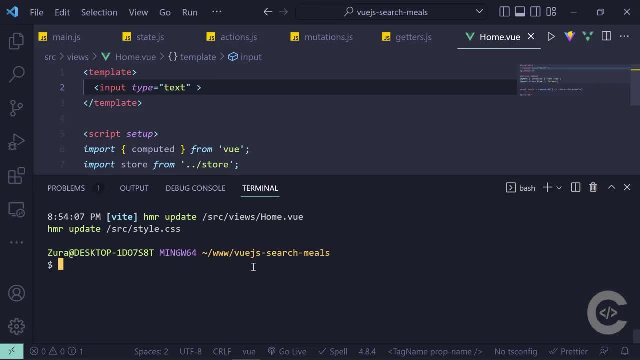 We're going to run the following command in the terminal. So let's kill this and paste. And then finally, we're going to put this in the plugins. Okay. 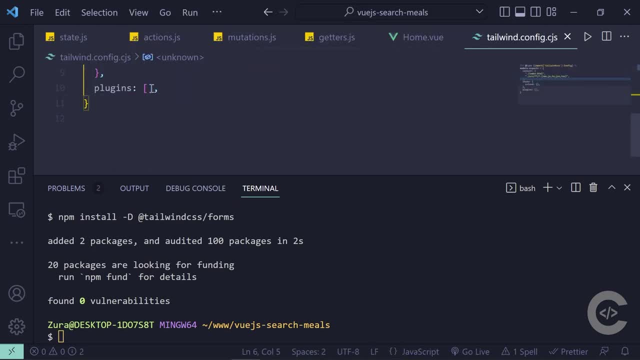 So let's open Tailwind config.js. Let's scroll down below in the plugin section, and I'm going to put this right here. Okay. And then run npm run dev. Okay. 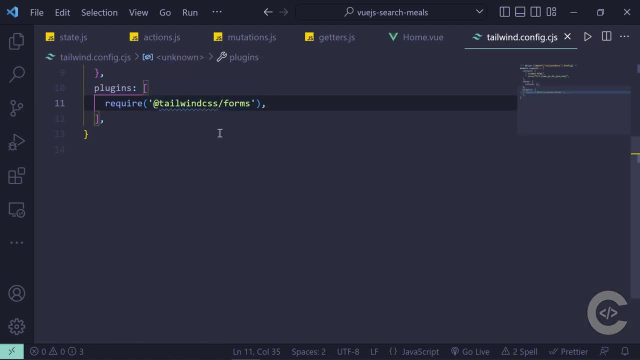 We have our application running. And basically inputs now should have a name. Okay. 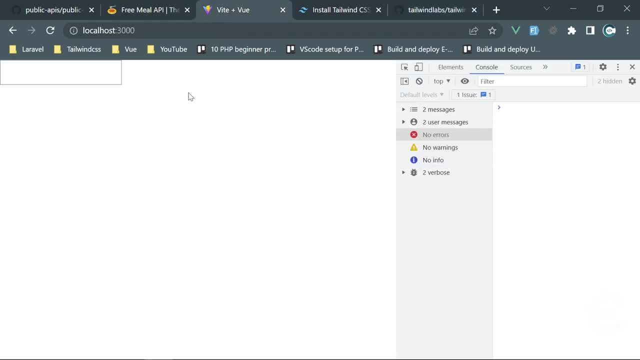 We have basic styles. So if we go, we see this basic style and we need to add more styles right there, of course. So let's specify a class right here. 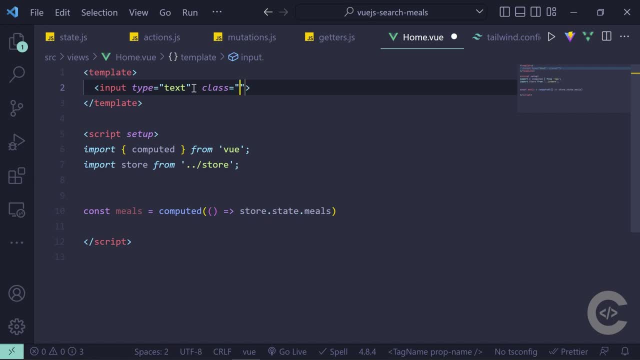 I'm going to give it, I'm going to give it like rounded. 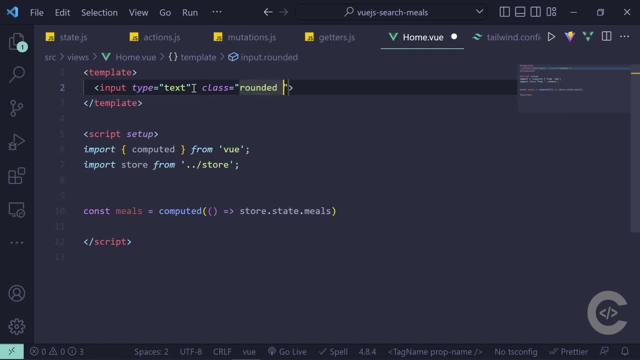 Let's give it rounded. Let's give it border, border two. Let's have a look. 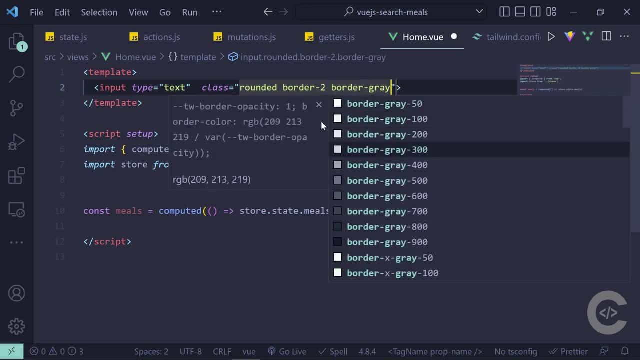 So we have it border gray, maybe 200. Okay. 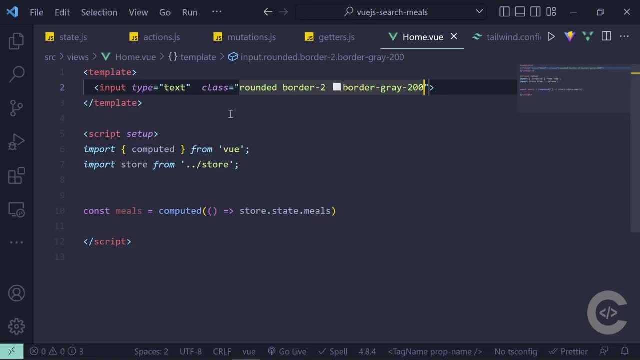 That's, that's good. And let's put it in the center. So because this is the home component, I'm going to wrap everything inside and let's put right here. 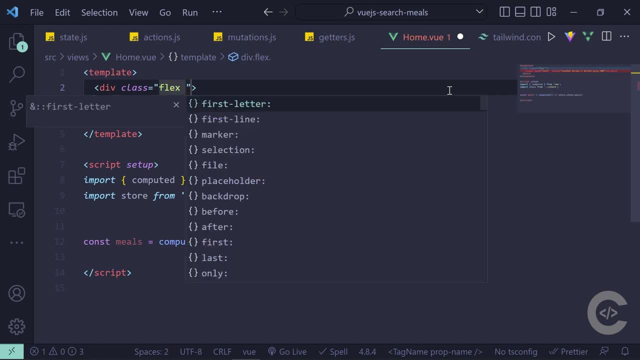 Let's give it flex as well. Let's give it also padding eight, maybe. 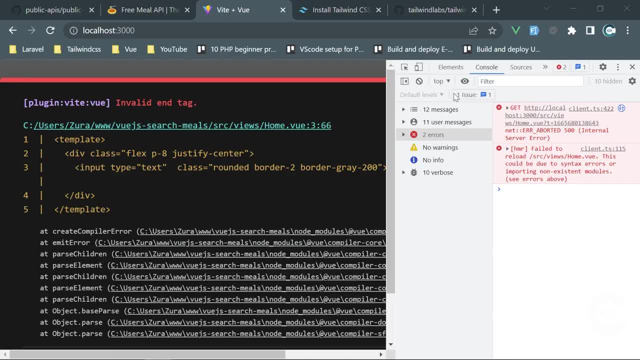 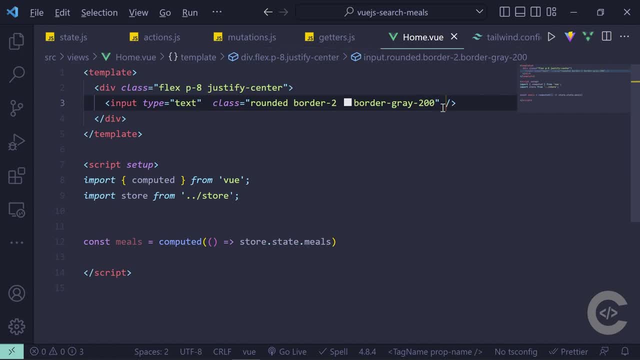 And let's give it also justify center. We save that. And slash right here. The input closing tag is not necessary. So we save that and we have input right here. 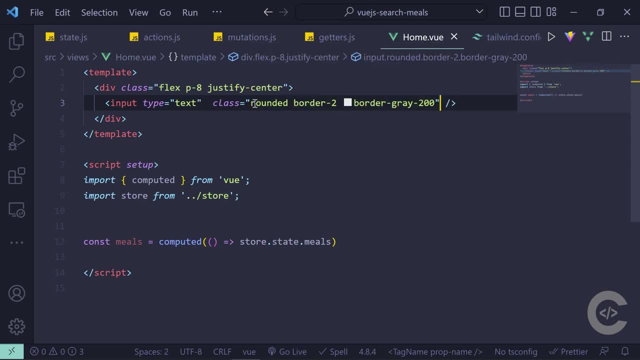 We can give it all also, uh, with like w like 64, maybe it should be large or maybe 72. Okay. 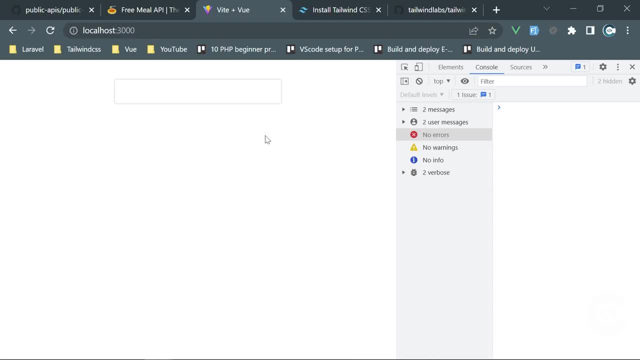 Now we have this large search input field. We can even stretch this on a full width w full. 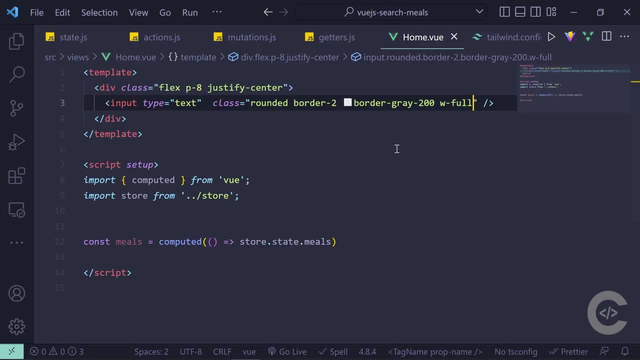 Okay. Okay. Okay. That's more like it. 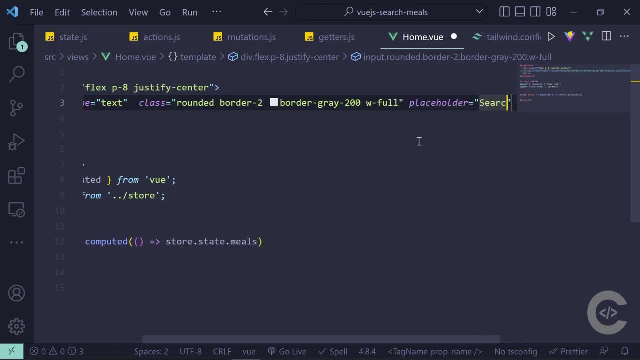 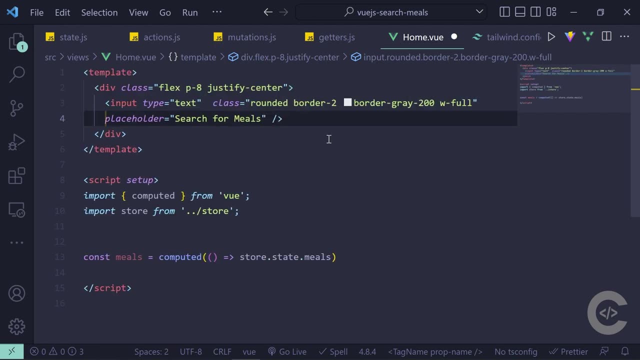 And let's give it also placeholder, placeholder search or meals, meals, and let's move this on a second line. 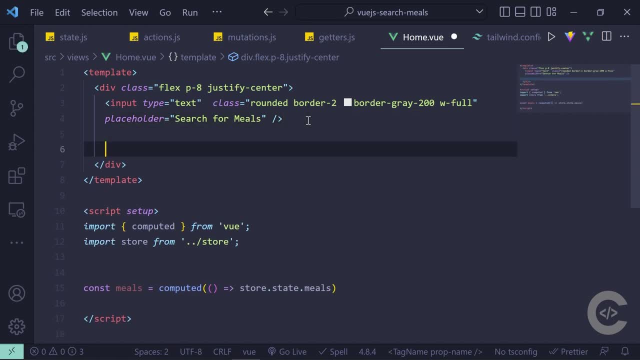 Now we have this input and we're going to also display letters from A to Z. So let's create div right here, which will have a display, display flex, maybe, and let's give it a gap one. Okay. 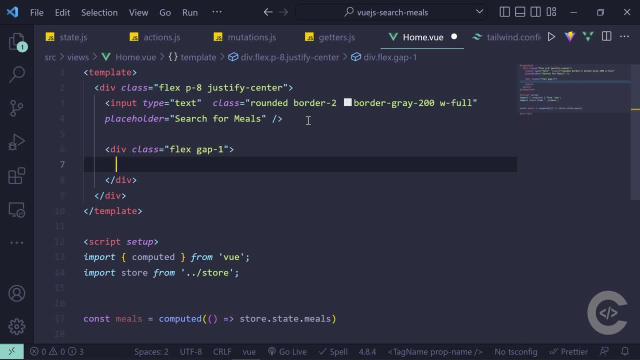 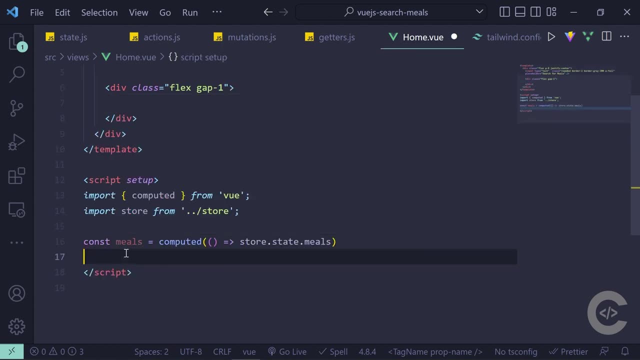 So we're going to create right here, span elements, uh, or they should be rotor link elements. Not quite sure yet, but I know for sure that we have to generate right here, an array of elements from A to Z. All right. 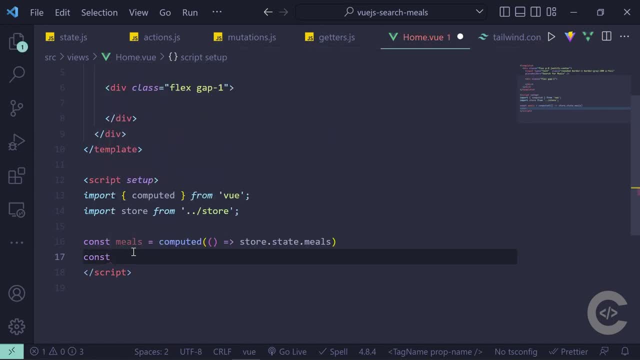 So let's create, um, an array, or maybe I'm going to create a string value, uh, letters. Um, AB, I can generate, of course, this, uh, from ASCII codes. Um, but why? To overcomplicate things. 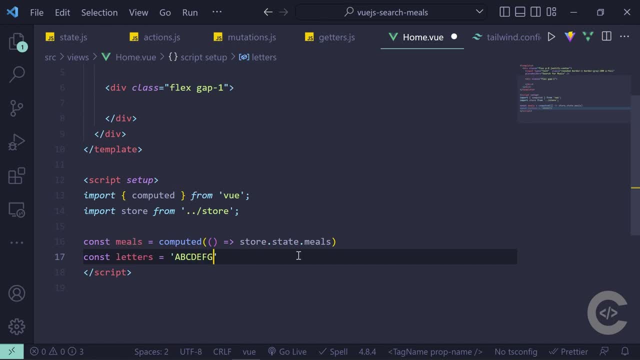 I'm just going to type A, B, C, D, E, F, G, H, I, J, K, L, M, N, O, P, Q, R, S, T, U, V, W, X, Y, and Z. 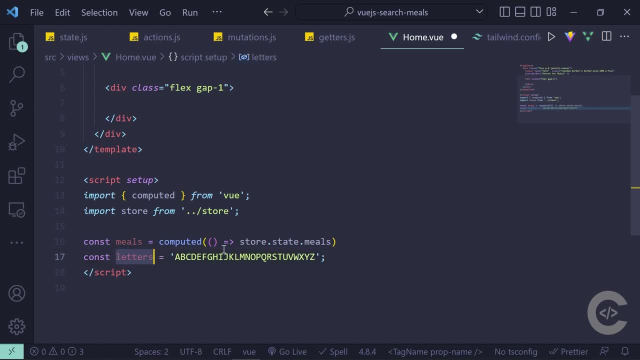 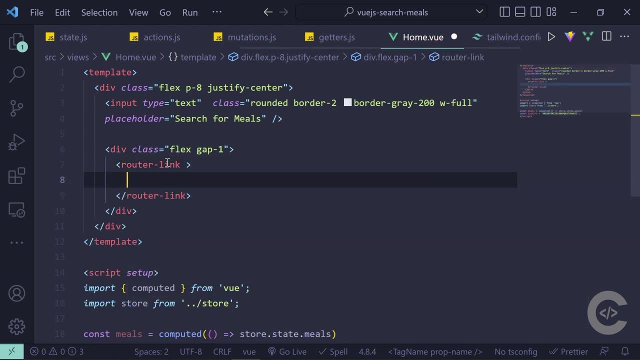 All right. So I have letters right here and I'm going to iterate over my letters. Let's actually actually use rotor link right here. Okay. 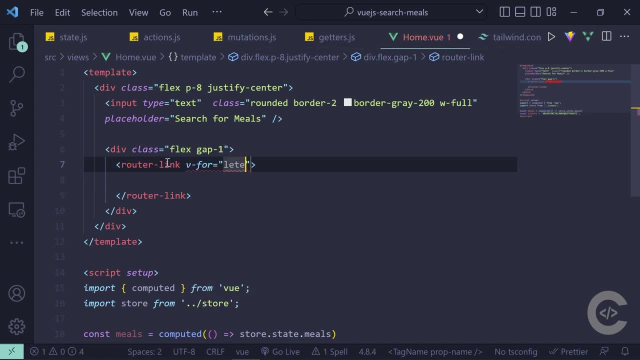 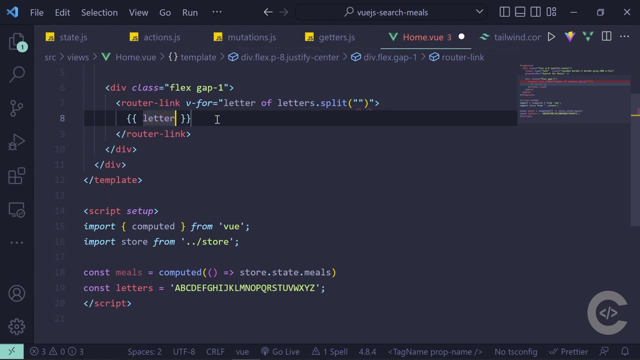 And we're going to use V4 letter of letters. Splash. Split. Okay. I'm splitting the letters with an empty string. That's going to give me an array and right here, I'm going to output a letter. 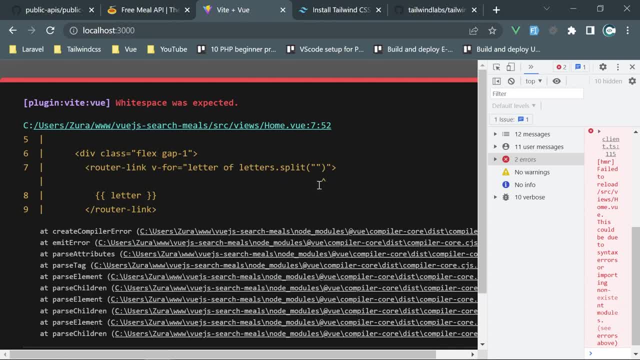 So I save this and let's have a look. All right. 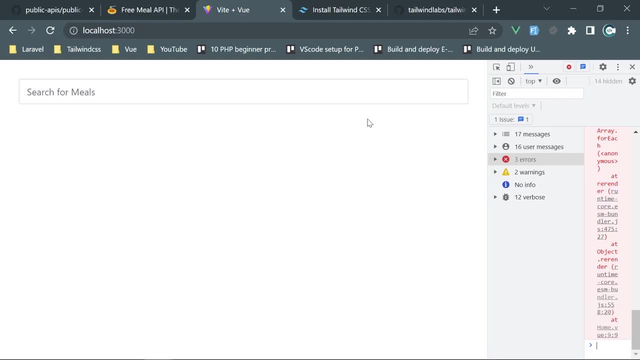 Split. Let's use single quotes right here. 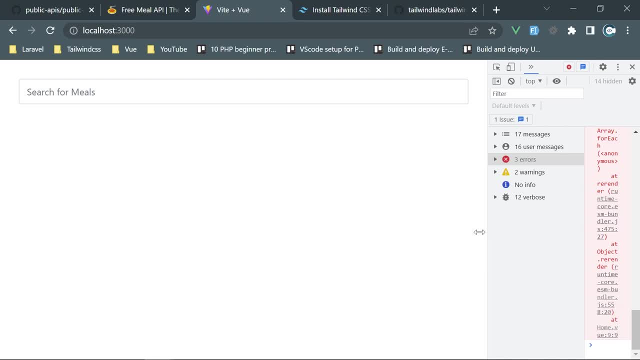 Save this and have a look. We probably have an error. 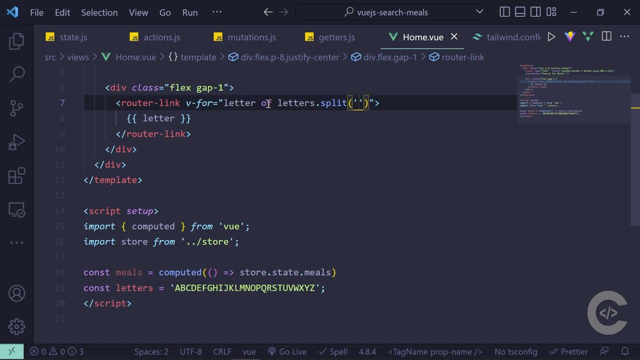 It doesn't seem to be working, uh, letter of letters. Oh, let's actually. Okay. I'm going to print. 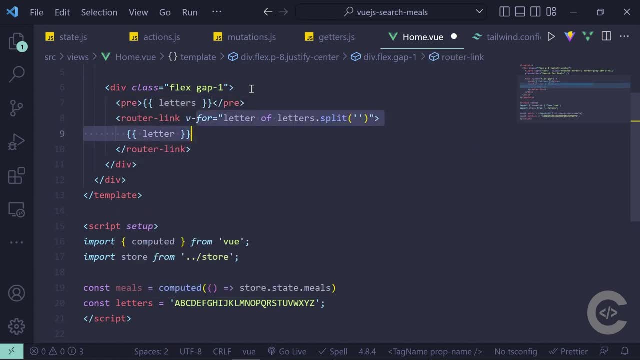 What is the whole letters inside pre-take maybe and remove this. 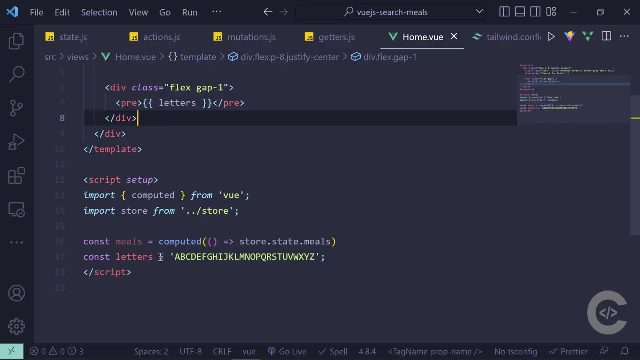 So we have those letters, which is string. Okay. 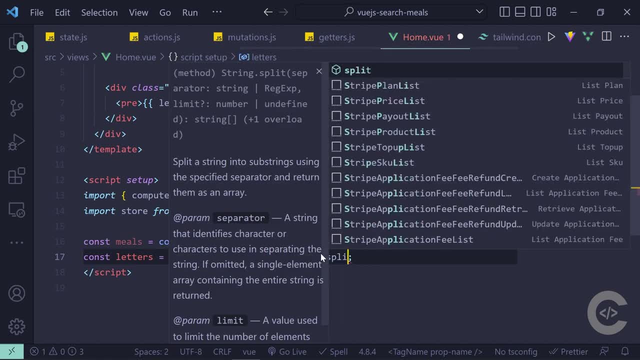 Let me split it right here. Um, split with an empty string. Now there should be an array. Okay. 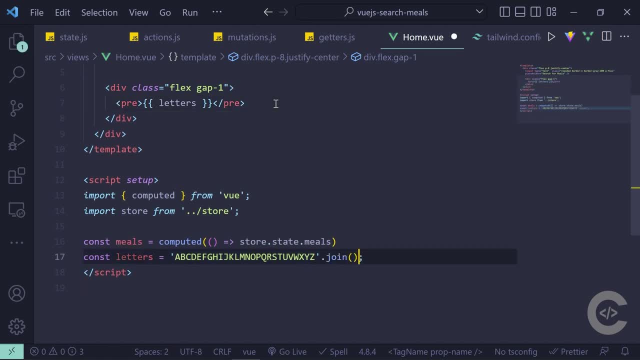 And now I should be able to iterate. Oops. Let's revert my change. I should be able to iterate over my letters. Okay. Now I should be able to iterate. Oops. I should be able to iterate over my letters. Okay. And let's put split right here again. And if you scroll down below, we don't see that. Okay. 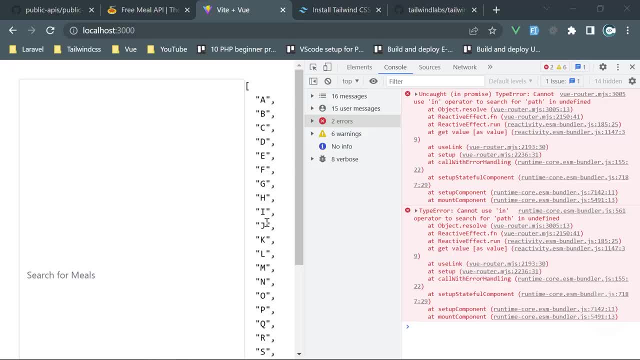 V4 letter of letters and we output letter. I think we have to specify right here, uh, two. 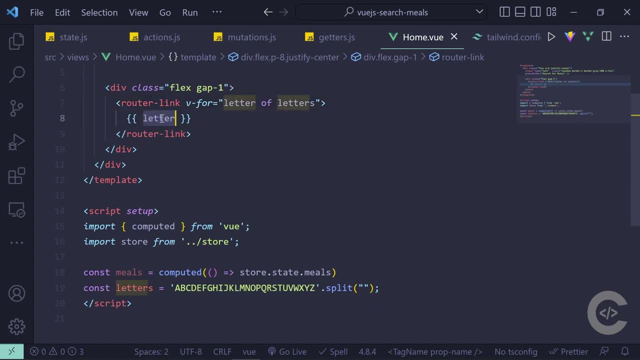 Let's specify slash at the moment. All right. Yeah, we have the letters. Awesome. 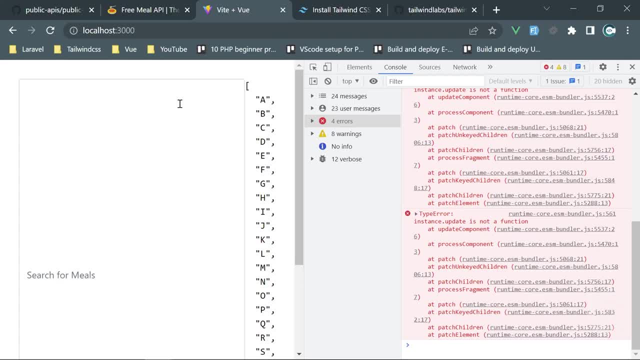 So this has 5 letters inside pre-take. So we can see that now we have an array of letters. Awesome. 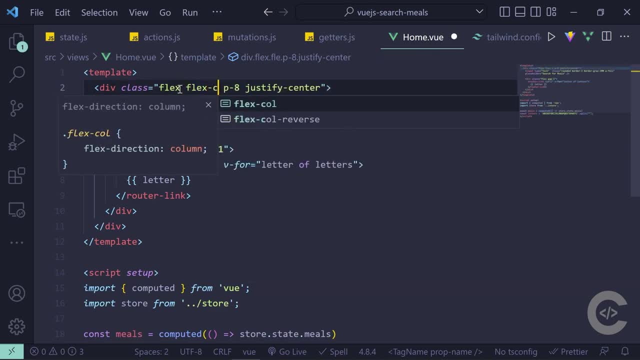 this has flex let's give it flex column and let's give it items items center 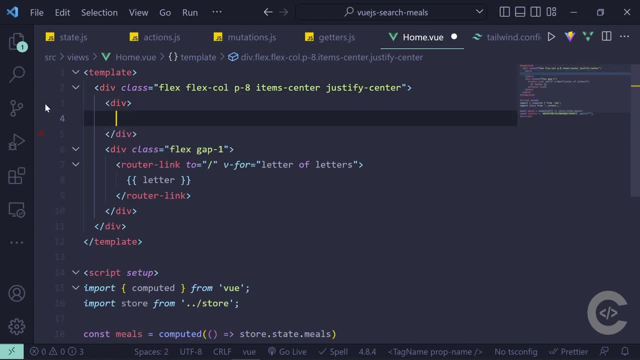 well i think we should wrap this in another div which will have or just remove this 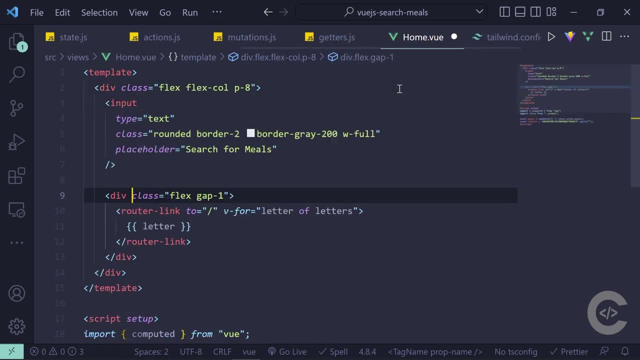 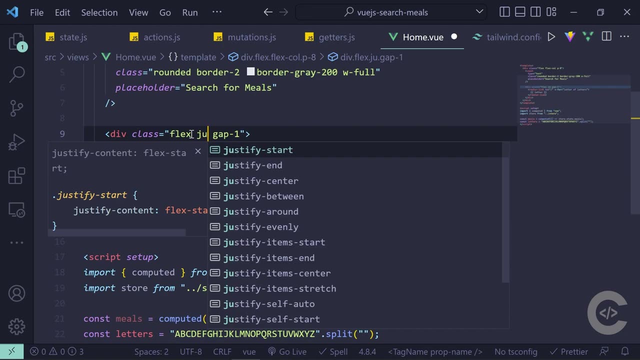 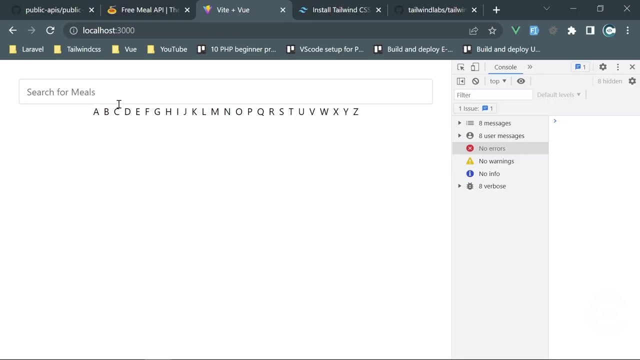 like this all right that's good so we have display flex let's give it justify center so that we have them in the center let's increase gap slightly this is good let's give it margin top 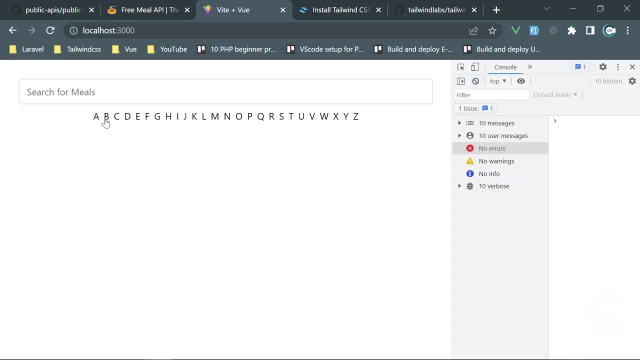 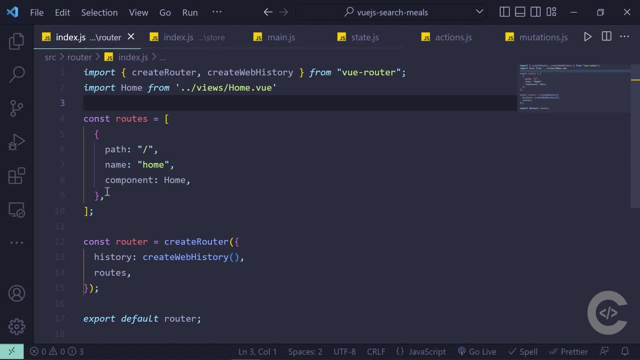 two and i think that's that's really nice now let's define a new route so let's go in the router slash index and create new route oops new route right here and that's going to be 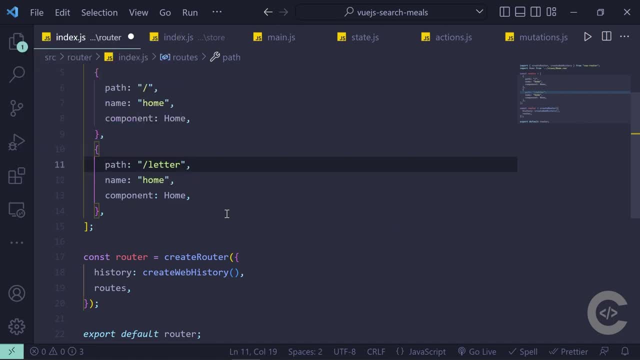 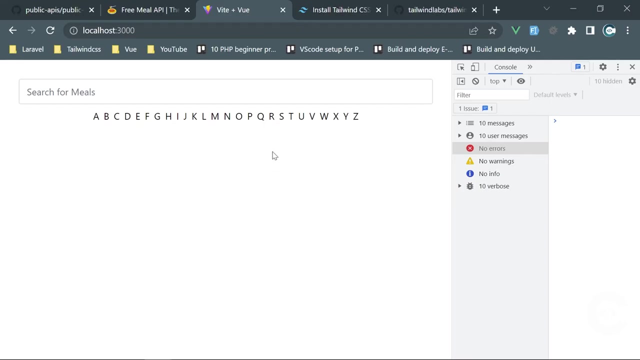 letter the road path will be letter slash and then the actual letter which i'm going to call it letter all right and the name of this road will be by letter all right and the component will be what component can we use so i think we can use 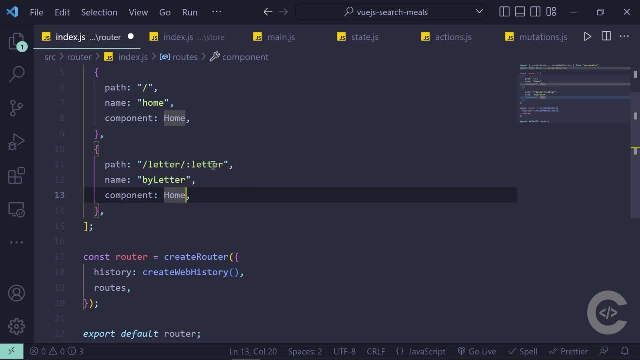 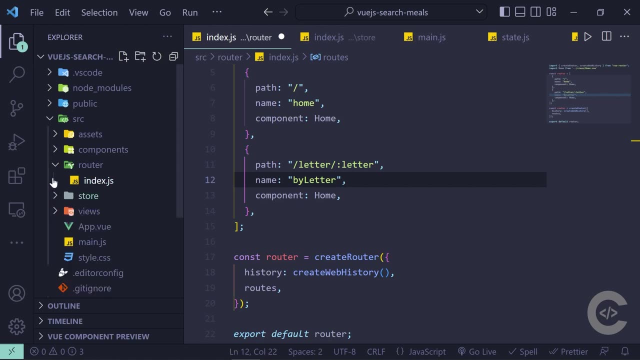 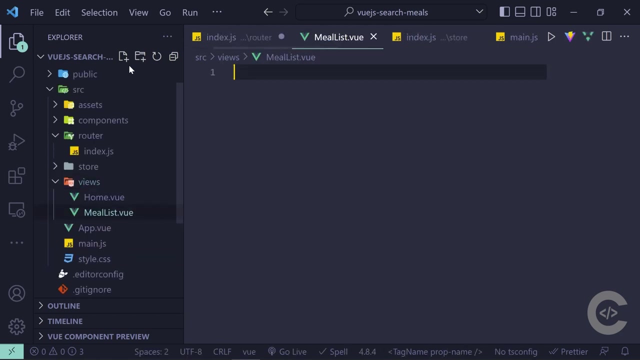 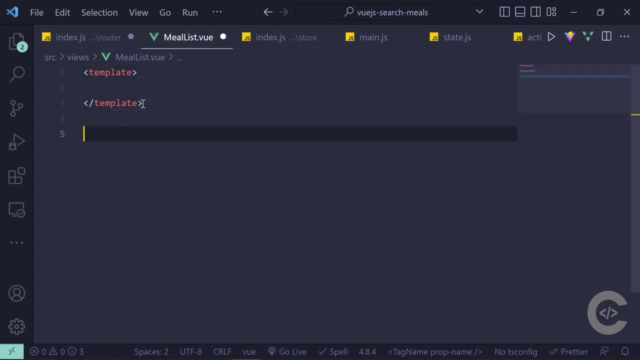 a new component and let's call it a meal list component maybe so i'm going to go under views again and create new component right here meal list dot view component all right and now let's generate template right here and we will need script with setup attribute and right here i'm going to create a div 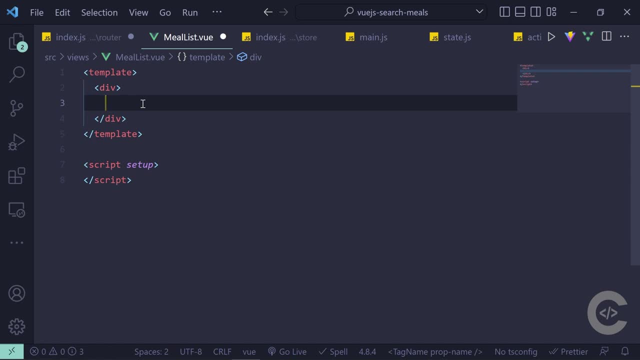 i'm not sure if i need this div but let's have it and we are going to display now items right here 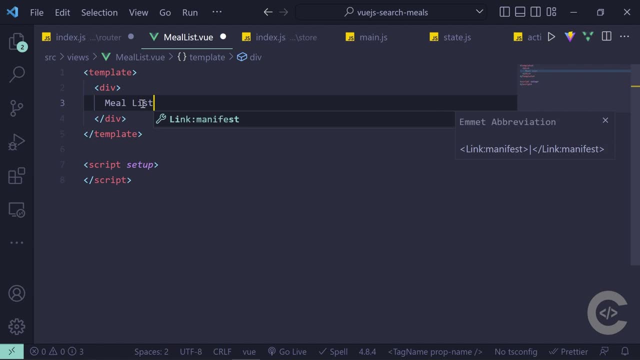 okay let's just type meal list at the moment and if we go in the router i'm going to use meal list 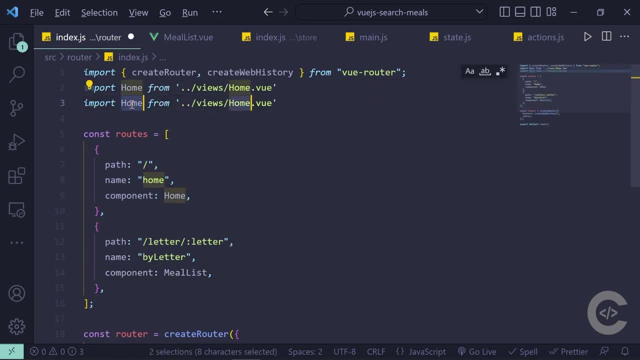 meal list which needs to be imported right here so meal list if we say this now and go in the 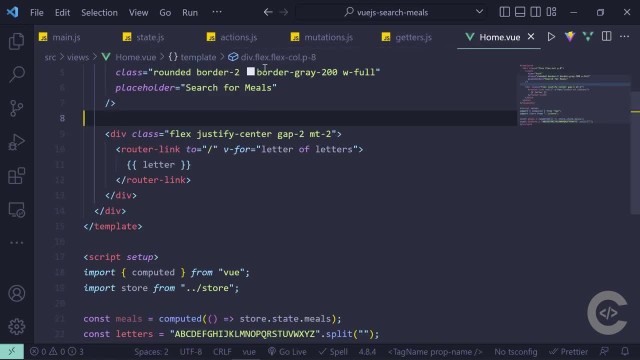 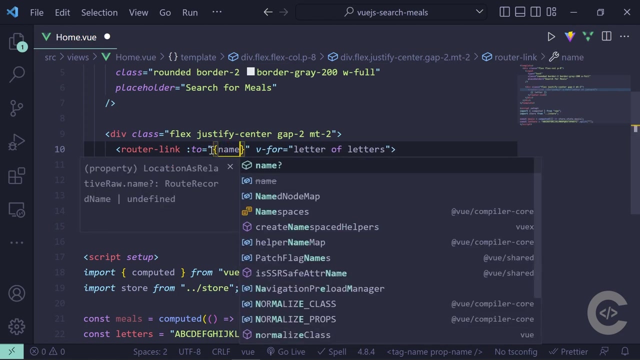 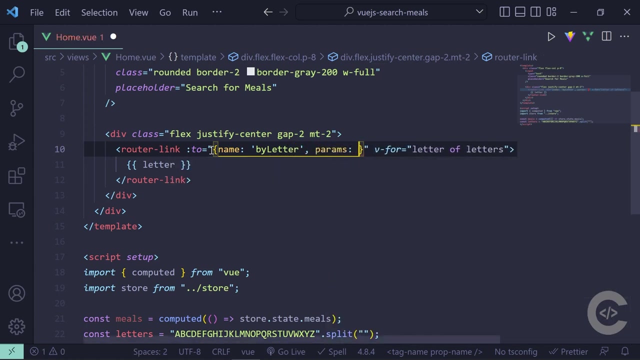 go in home let's actually close everything close all and just open home and right here i'm going to specify a root and i'm going to use now binding of fruits and i'm going to specify by name and i'm name is by letter, and I'm going to specify params as well, and in this case, params 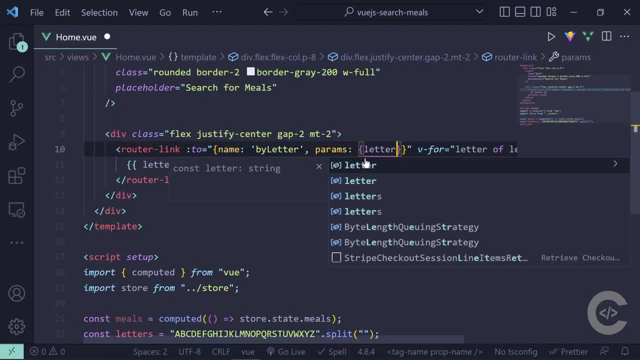 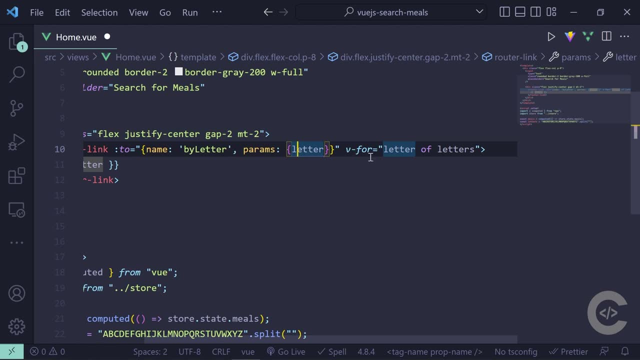 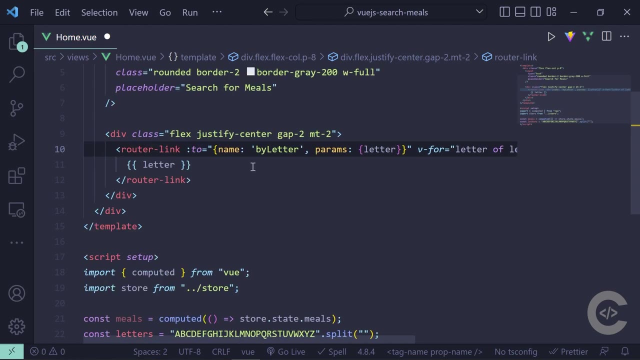 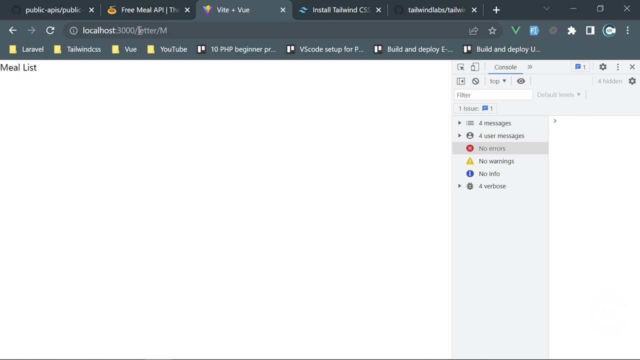 will be letter, we have only one param, and that is a letter, all right, this letter will be bound as parameter letter right here, and let's also use right here key to be letter, all right, now we have wrote configured, if I click now any of the letters, we will see in the url letter m, all right, if we go back and click something else, we will see letter p, and we see meal list right here, okay, we are going to have also display, we're going to display the categories, sorry, ingredients right here as well, and whenever we click on one of the ingredients, it's going to open a similar page of this, it's going to use, we will try to use the meal list component, and it's going to render items right there, and if we just search something, salmon right here, it's going to open also something similar component, or we're going to display it right here, so we're going to think 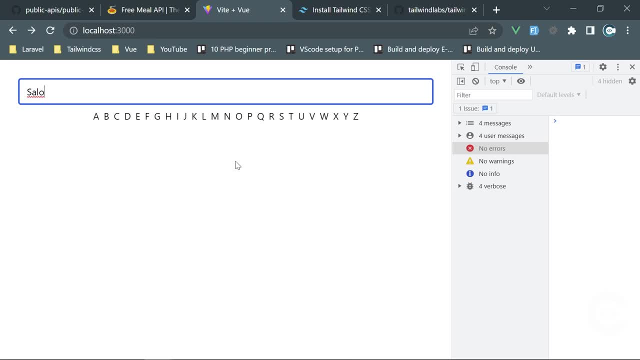 how we're going to do that, but in any case, we're going to try to reuse everything, okay, so I'm 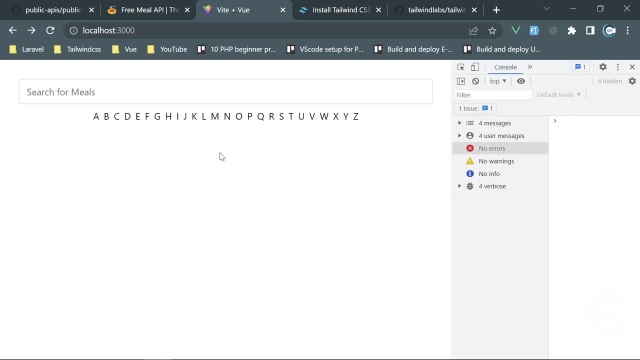 building right now, this is the first time I'm building this particular application, so 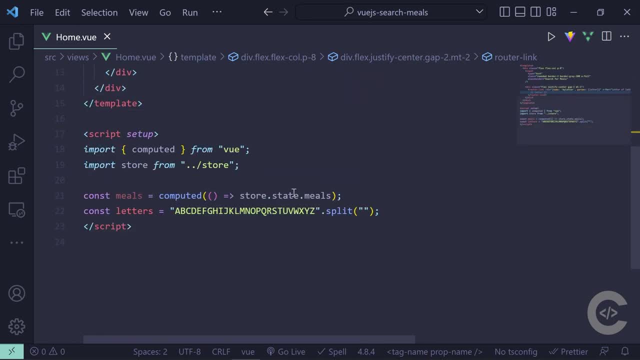 all right, so let's now make request to list all the ingredients, we don't need these meals right 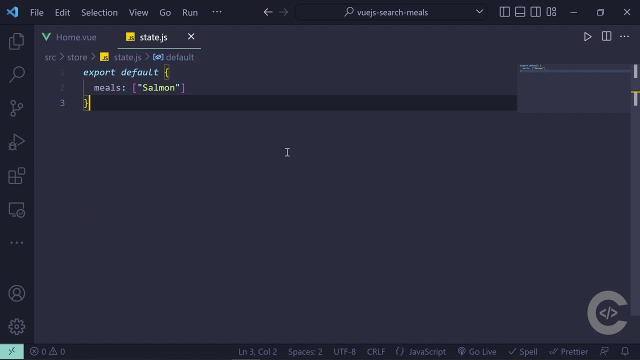 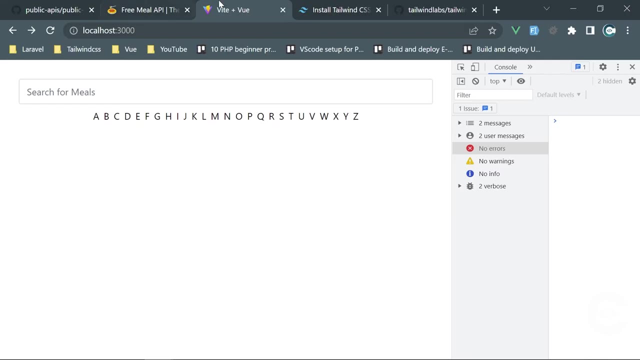 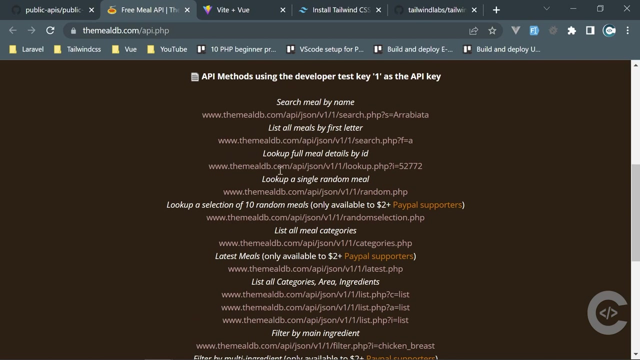 now, so I'm going to remove this, we can open event state, and remove this from here, we don't need them at the moment, however, now let's get those urls, so we need, we need to list all 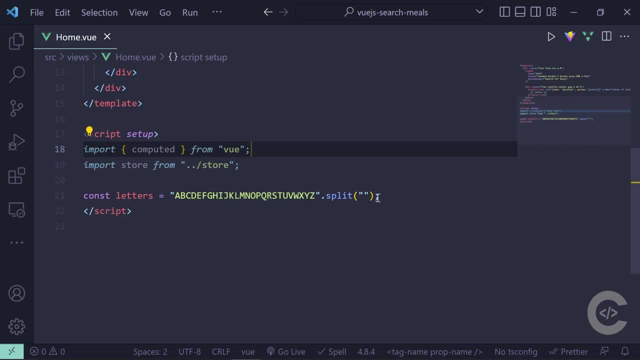 ingredients, so let's use the following endpoint, so right here, I'm going to make requests on the following endpoint, and I'm going to make requests using Axios, okay, so we don't have Axios installed in the system, so let's install 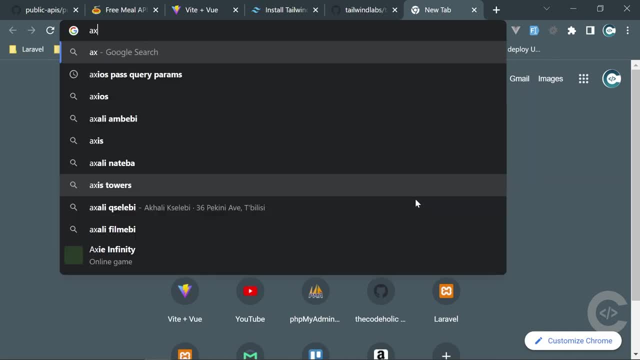 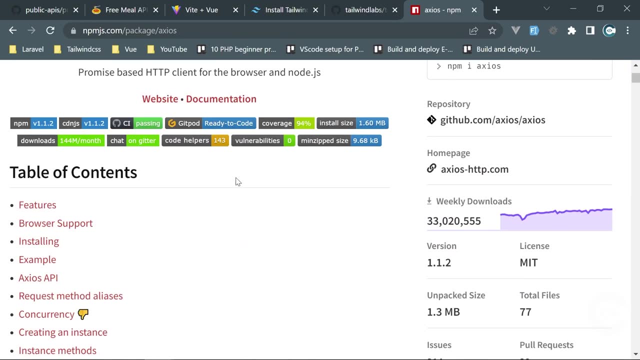 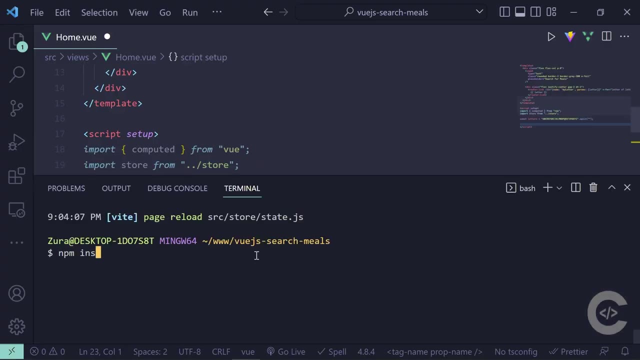 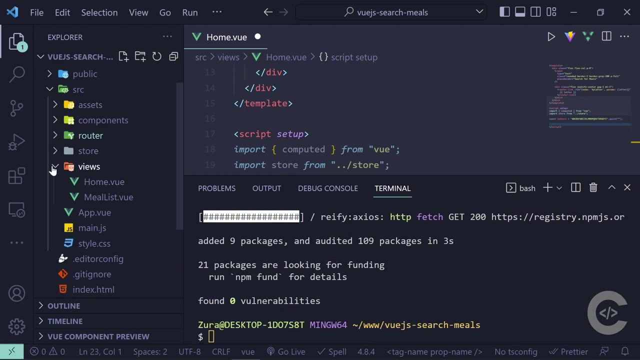 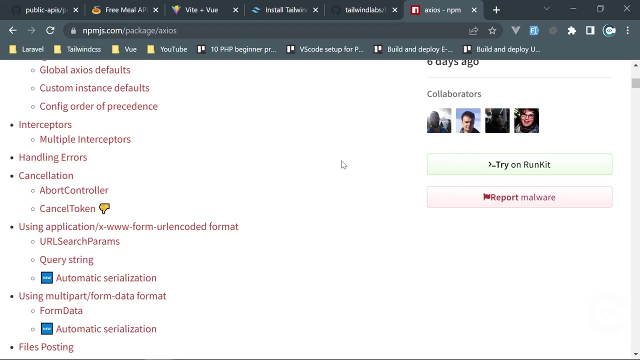 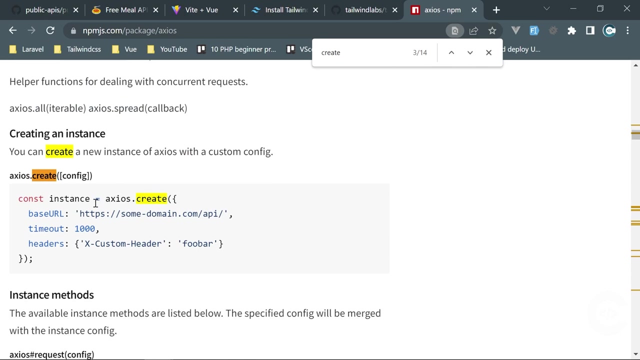 that, I'm going to open now browser and search for Axios npm, the name is Axios, I know how to install, just I want to find the configuration file as well, how to create the config, so actually, let's install npm install dash s Axios, and then I'm going to create, under source, I'm going to create new file called Axios client dot js, and let's start the server, and I'm going to create now client right here, and let's search for create or something like this, yeah, this is what I want, 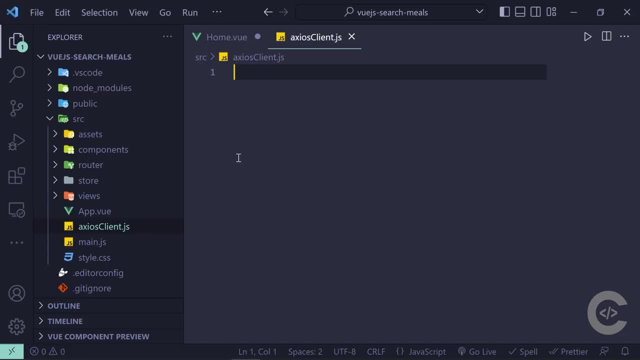 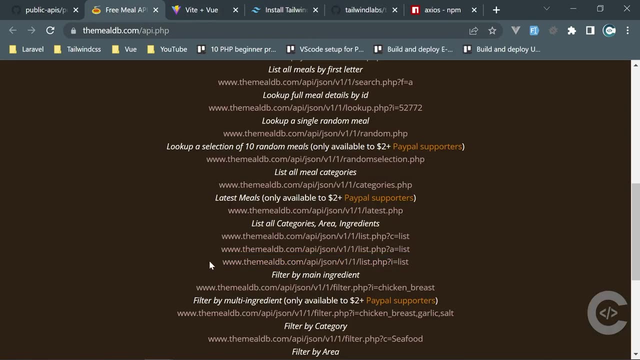 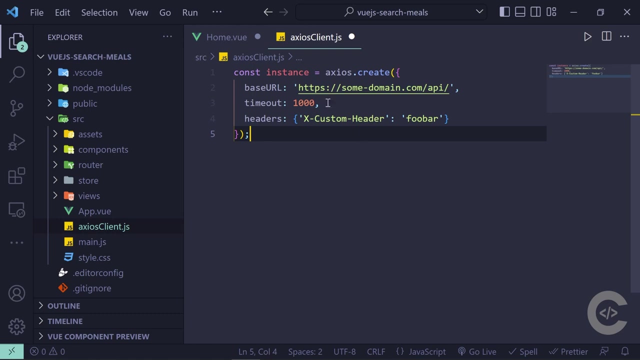 so I want to create an instance, so let's specify it right here, the base url will be the url base url of the api, and it is the same in all cases, okay, so this is going to be base url for every endpoint, okay, we have timeout right here, which we don't need probably, so we can remove that, for custom, 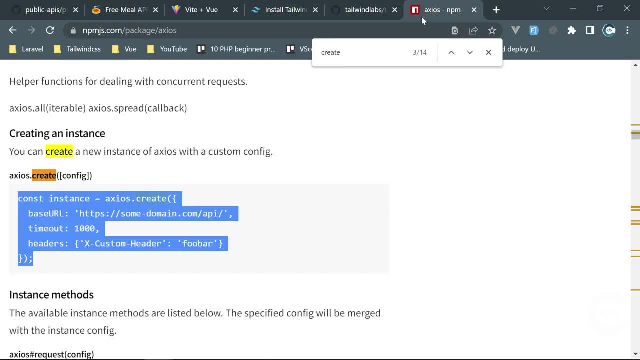 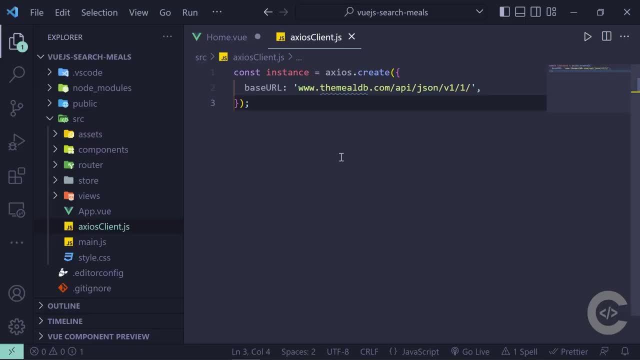 we don't need these custom headers as well, let's have a look right here, what else do we need, we, whenever you're building something, which needs authorization, we will need 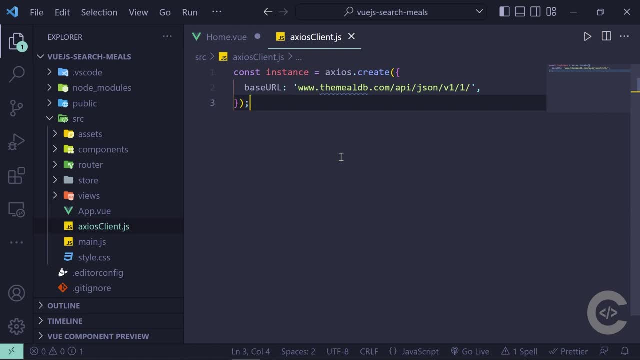 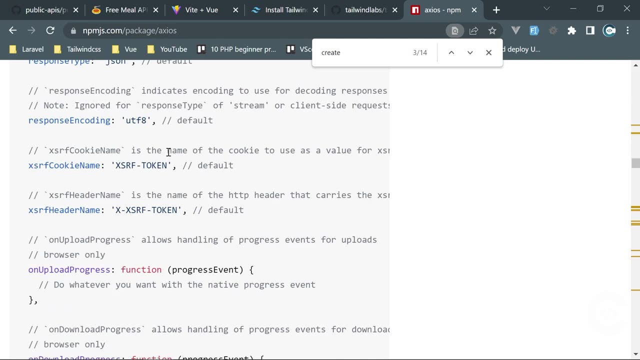 interceptors as well, but in this case, we aren't building anything like this, so we probably don't need that, yeah, I think we can directly export, directly export this instance from here, okay, 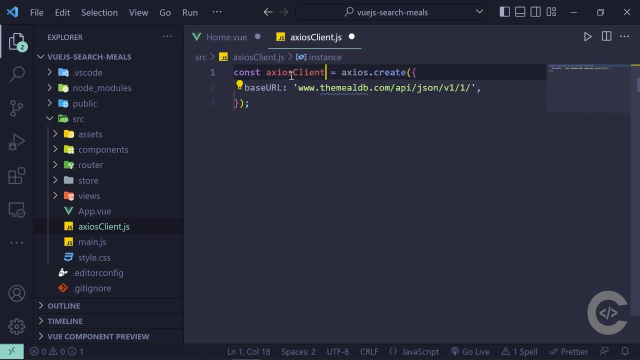 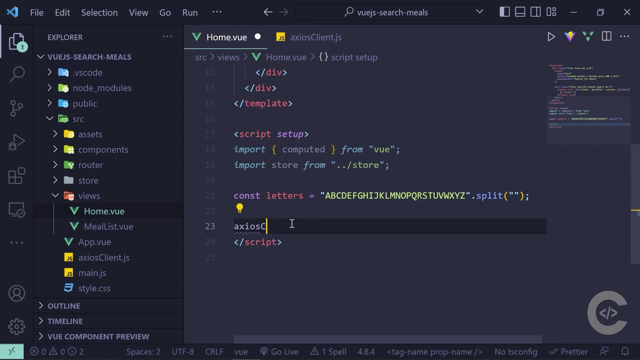 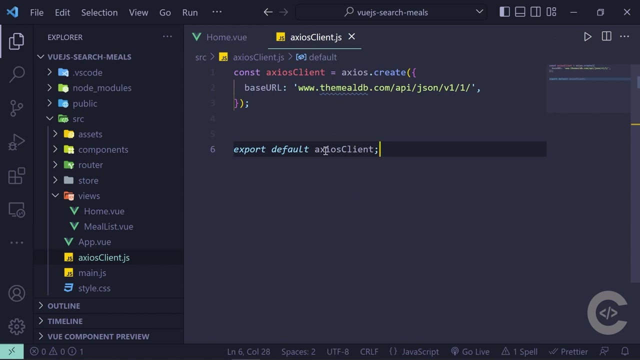 actually, I'm going to call this instance axios client, and then we're going to run export default axios client, all right, let me save this, and if we go in the home, I'm going to use axios client, the autocompletion doesn't work in this case, we have axios client, and we're exporting that, so that should be visible right here, okay, 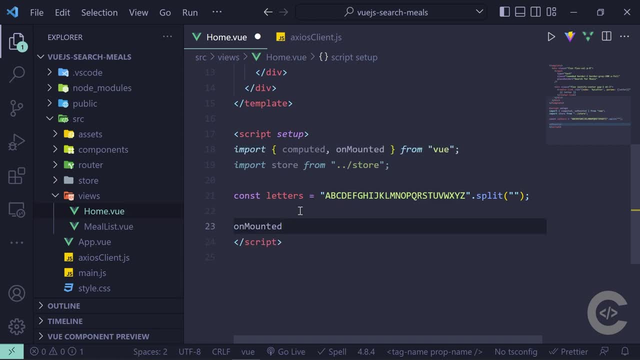 let's first use unmounted hook, let's hit the enter, that unmounted was automatically imported from view, this is what we need, unmounted, we are going to use axios client, and run get request 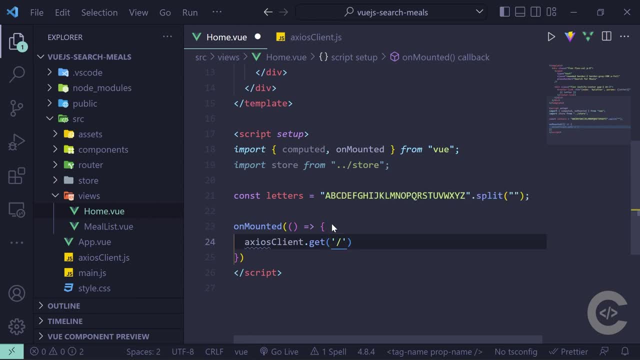 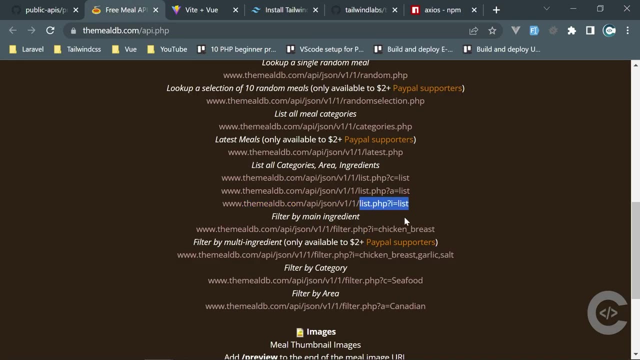 on the following url, and the url is basically, let's have a look in our api, the url will be this, to get all the ingredients, so let's put this right here, 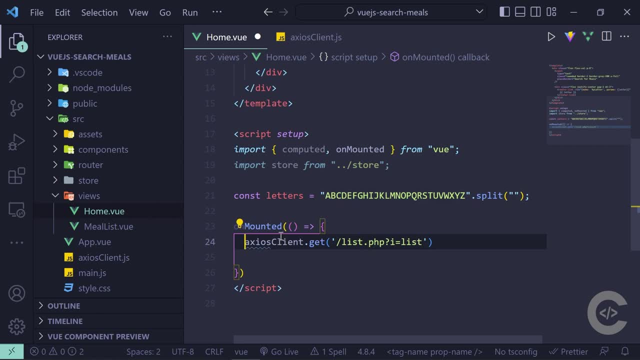 all right, and we first need to import axios client, so let's just type import axios client from, from go one directory back, and from axios client dot js, well, I think we should call this 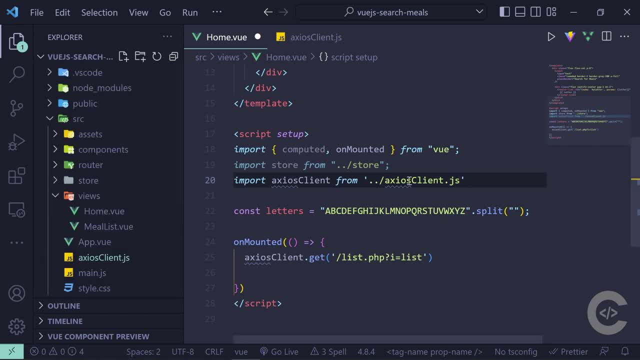 in, also, the VS Code complains about that, axios unknown word, that's okay, I think we can call this with, 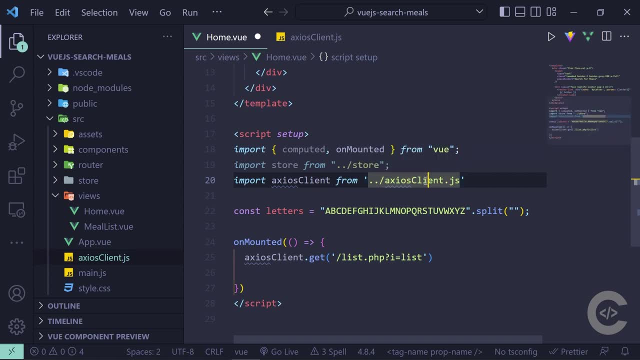 and i'm not sure what is the best standard to name this file so i'm going to leave this as this and we have it imported and we need a then right there or we can turn this callback 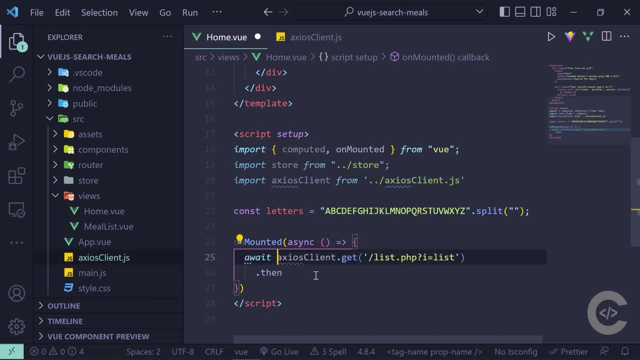 asynchronous and we can use await here and we can get the response response and then we can just print the response console.log response.data okay so we save this and now let's have a look 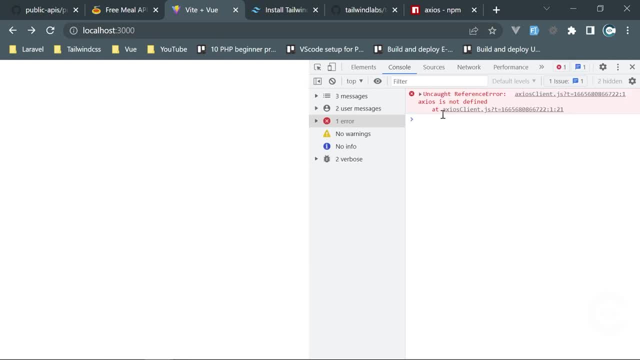 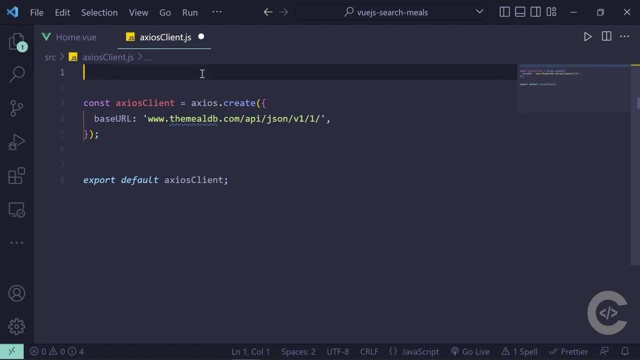 so on home if we just reload we see axios is not defined that's because in the access client we don't import axios so import axios from axios so we save this 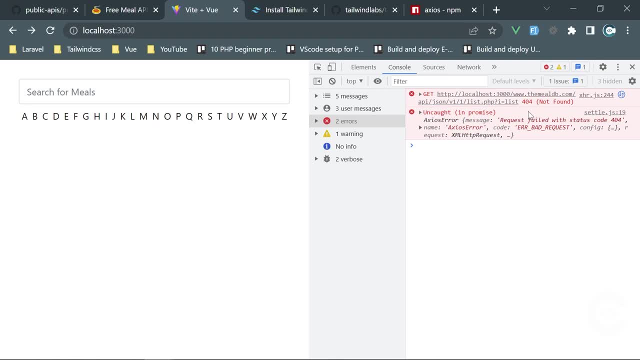 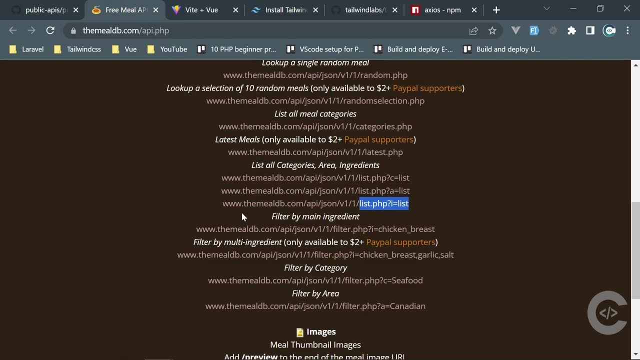 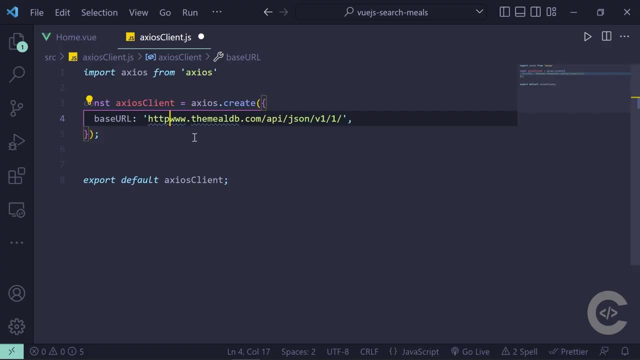 and let's have a look so we have error not found because http or https let's test this it is https so https colon slash slash we save that and now have a look 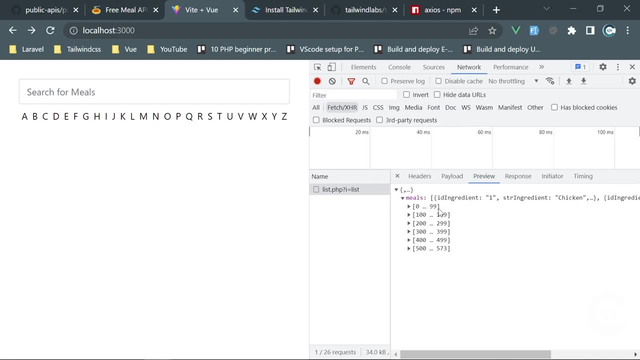 and i guess the request is made here we see that and we have meals well actually we have ingredients and we have almost 600 ingredients right 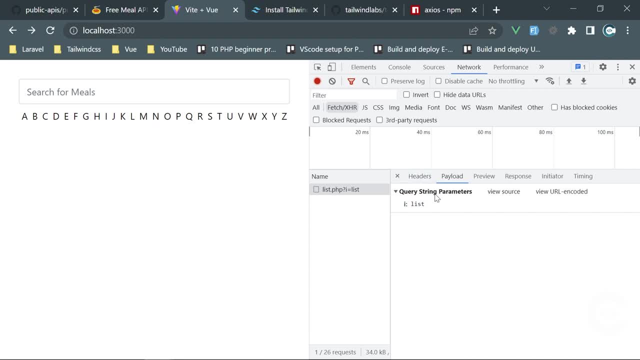 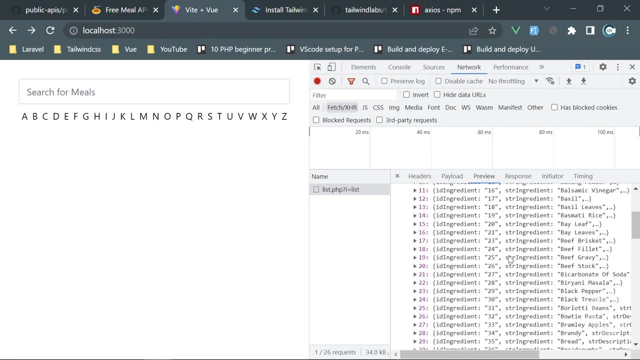 we made a request to the ingredients list all right we can display all of them so we probably need to display like first first 20 maybe 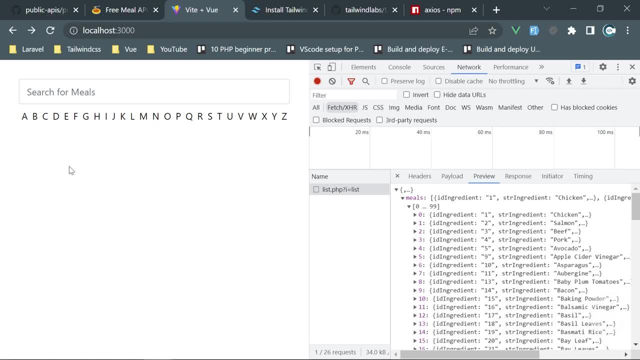 yeah we can't actually display all of them or we can display them and have ingredient search as well like client-side search 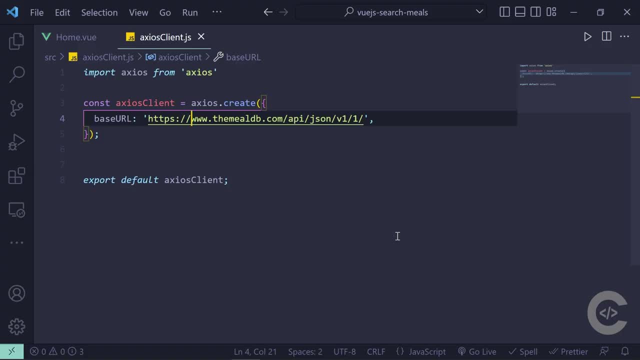 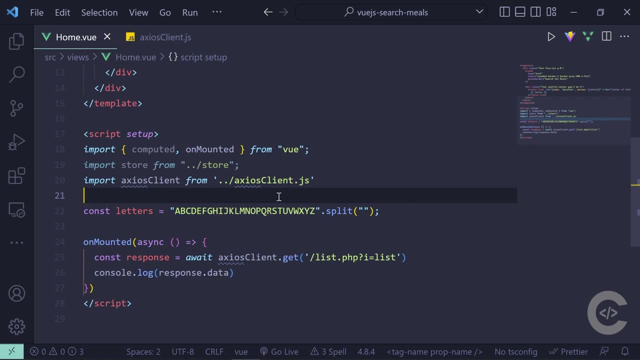 like i'm thinking while i'm building this all right so let's go in the home and let's create right here okay here are a few things i want these ingredients 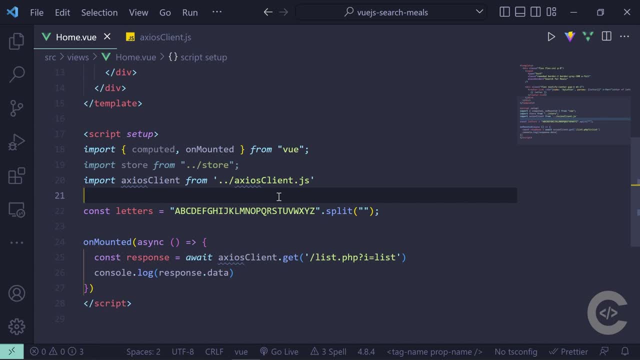 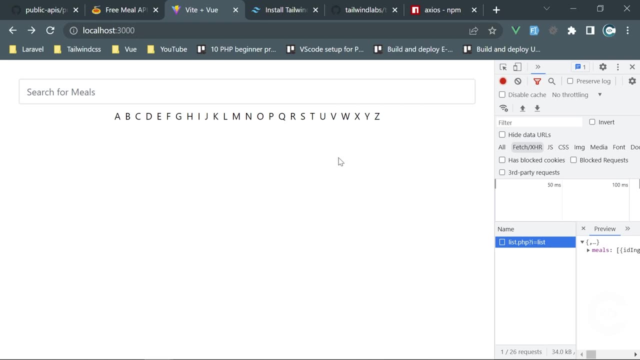 basically to be saved inside inside viewix and then retrieved from there okay but to make this happen we need navigation so we need like a couple of pages search maybe a search meals page 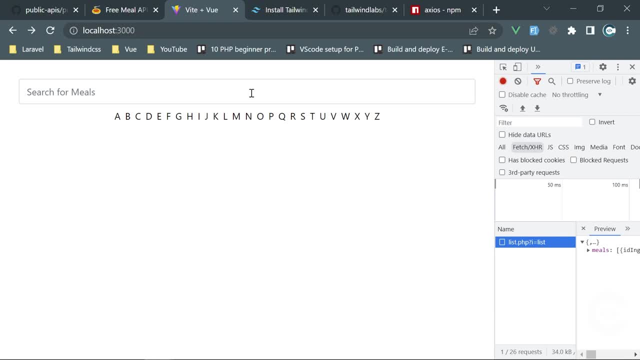 meals by letters or and meals by ingredients if we have those three pages then when you go in the meals by ingredient page and the content is loaded that content is saved in the viewx and then you go in different page search meals 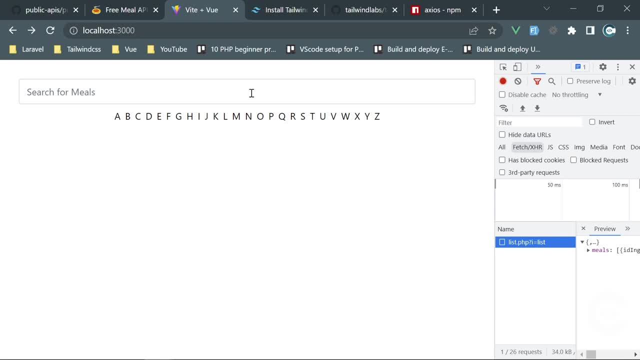 and then you save it in the viewix menu and then you go in the different page search meals and then when you go back into the search by ingredients then you're gonna have that 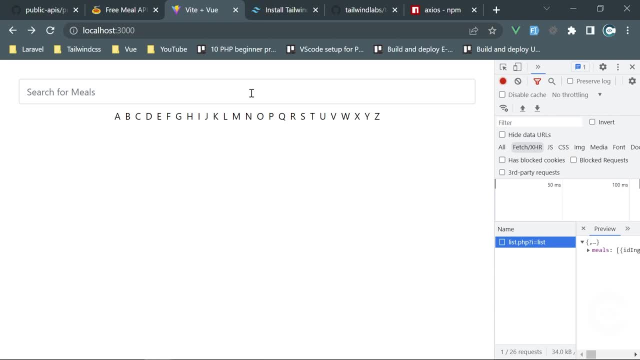 data coming from the store because you received it once and that is basically 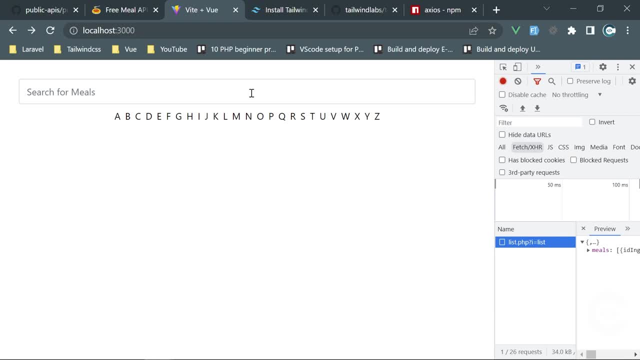 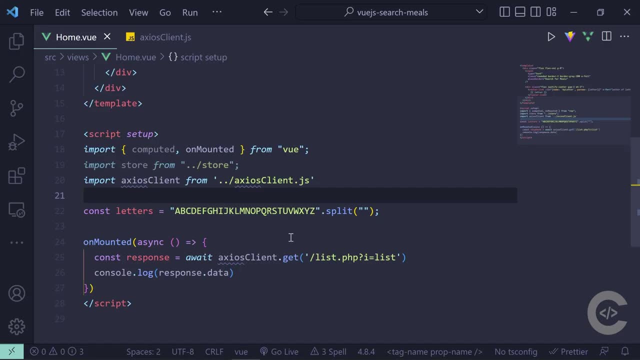 available as much as you want in the entire application right all right let's try to use store without store in Vuex this is very simple so at this moment we 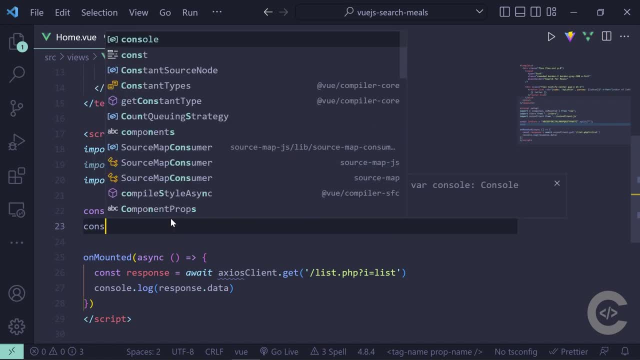 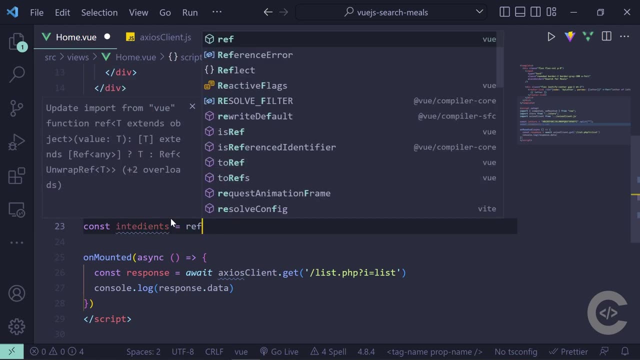 can right here create a constant variable const like ingredients and that's gonna be using ref let's create that's gonna be an array all right 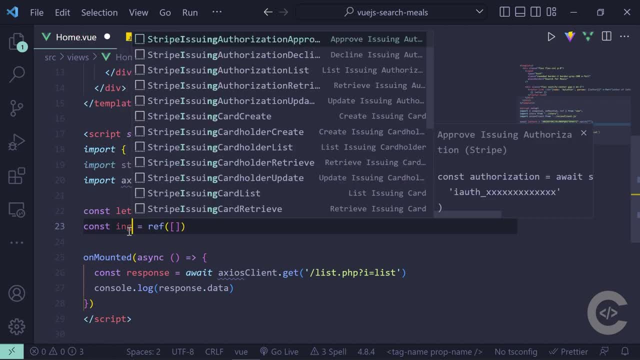 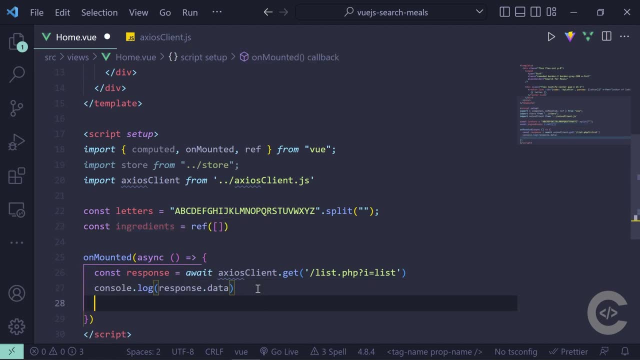 what did I wrote there ingredients not sure how this is written ingredients I think this is the correct one so I just type ingredients dot value value value equals response.data, and right here in this template, I can just type inside pre-tag 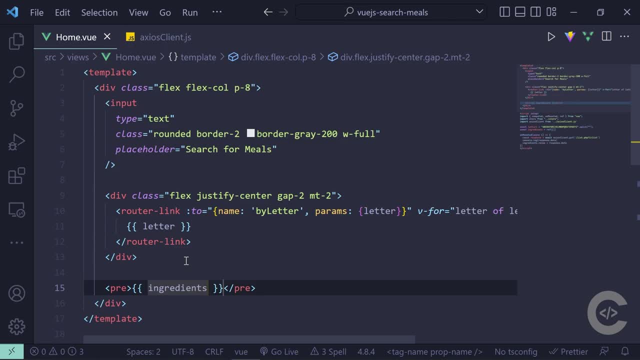 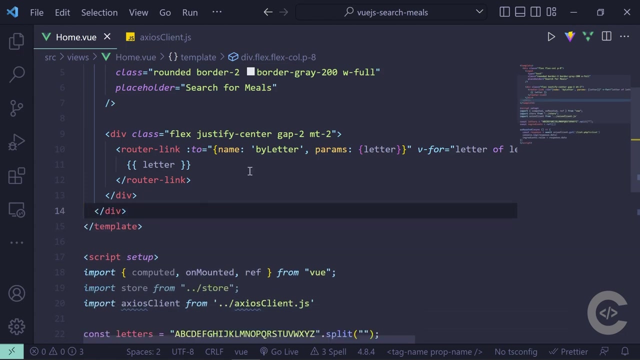 ingredients, so I save this, and here I have all the ingredients, okay, like those 600 ingredients, and displaying this is very easy, okay, I want to use Vuex as well, so for this, let's create a layout as well in our application, so I'm going to go in the app right here, and we're going to 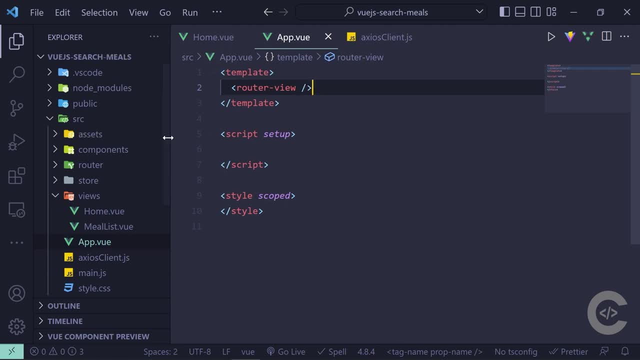 define layout, this layout can be defined inside the app view right here, if we have a single layout, we can define right here, so for example, we're going to have a single div inside there, I'm going to have like a header component, and then I'm going to have main, and inside main, I'm going to put 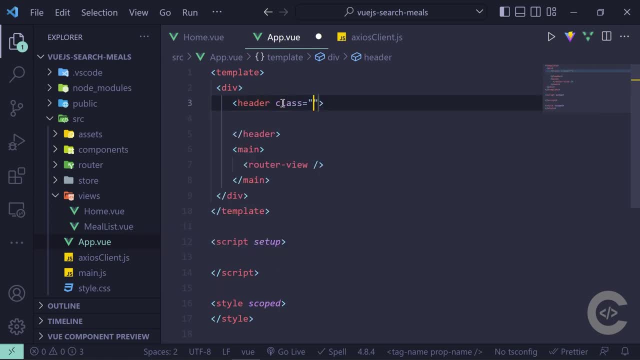 this router view, however, in this header, I'm going to give it some classes, like pg white, let's give it shadow, shadow md, let's give this one also 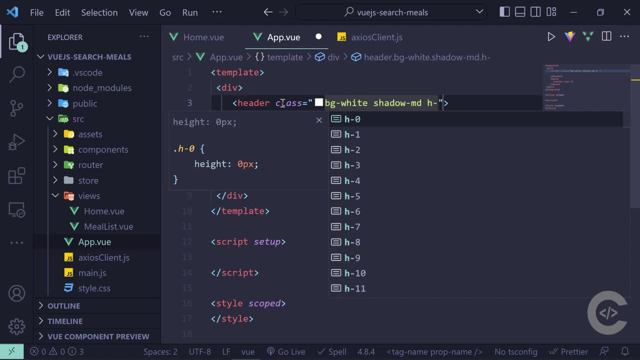 height of like 24, maybe, and let's give the parent one pg gray 100, so if I save this, now look at this, so we have by default, 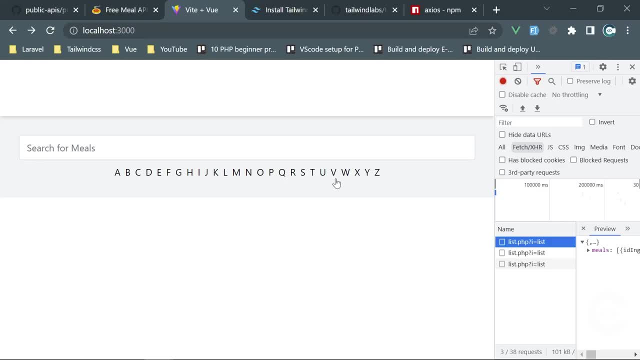 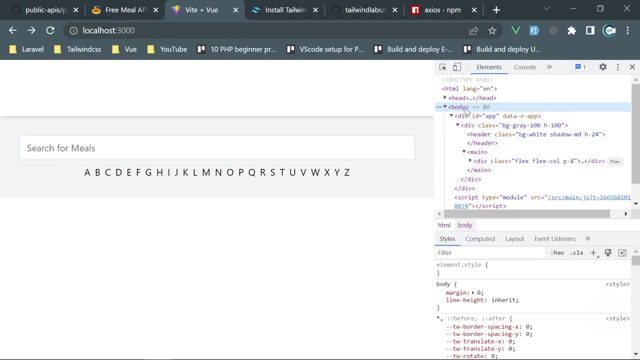 gray background, and let's give this also h100 to give it full height, and it doesn't have full height still, because the html doesn't have full height, and body as well, so if we go in the public, 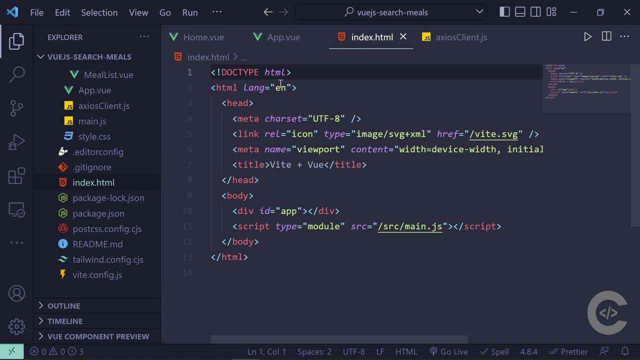 where's the index html, here it is, and if we give html and body class h100, we should be good, 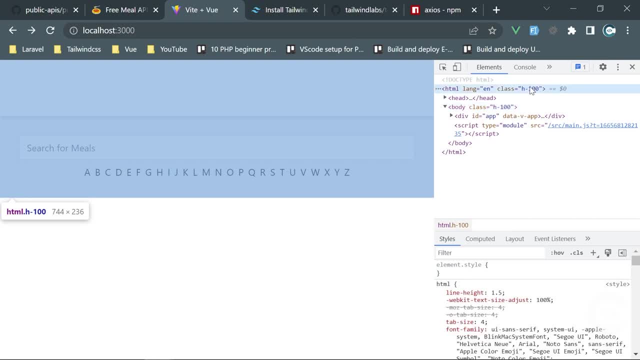 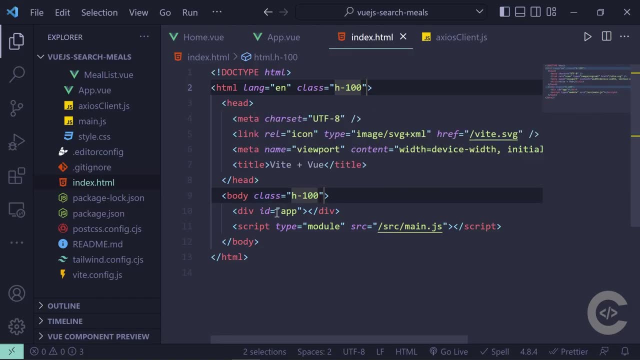 okay, it doesn't seem to be working, so talent css doesn't seem to be working there, because we don't probably watch html files, not sure what is happening there, 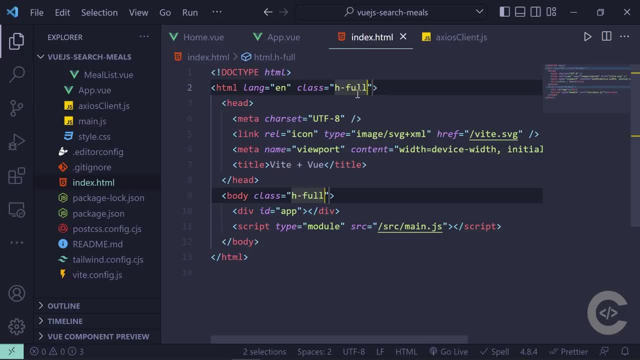 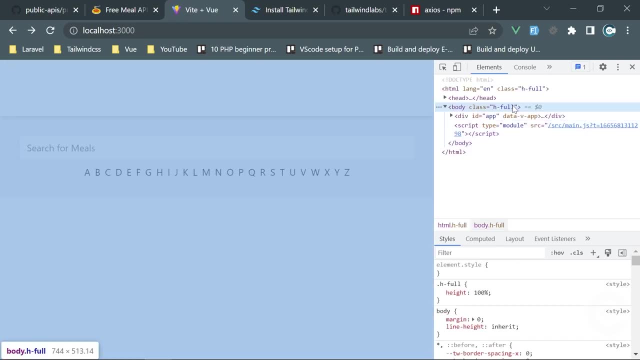 h100, no, it should be h full, it should be h full, and we need h full here as well, okay, now this has full height, 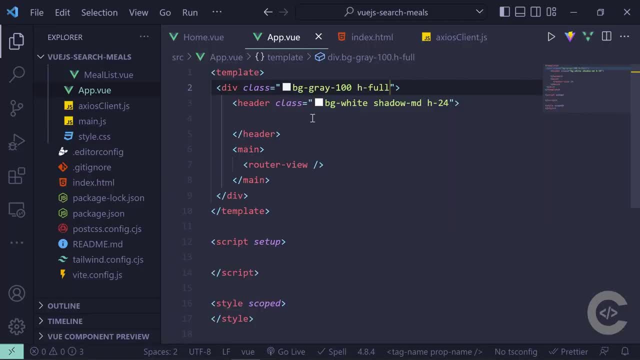 and this one doesn't have full height, because we need to give that h full to this up element right 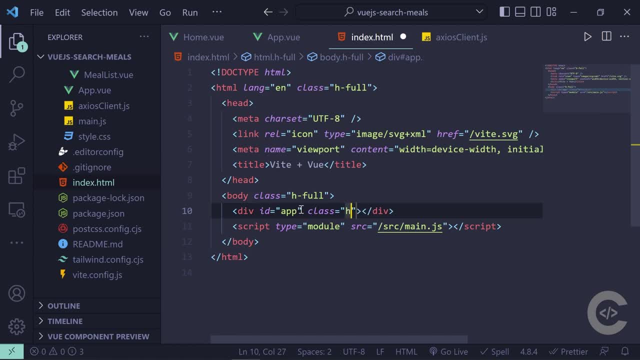 here, h, h full, so we save this, and this is our header, let's reduce it slightly, let's give it height of 16, oops, here we have this header, 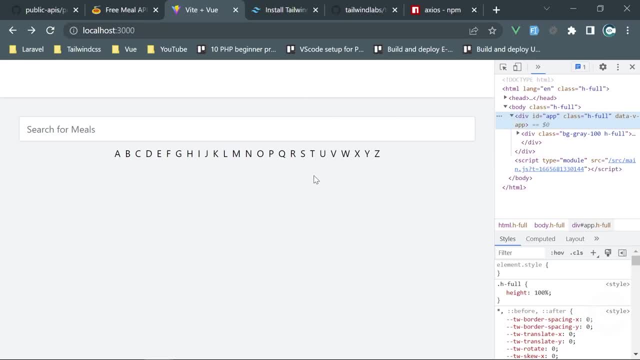 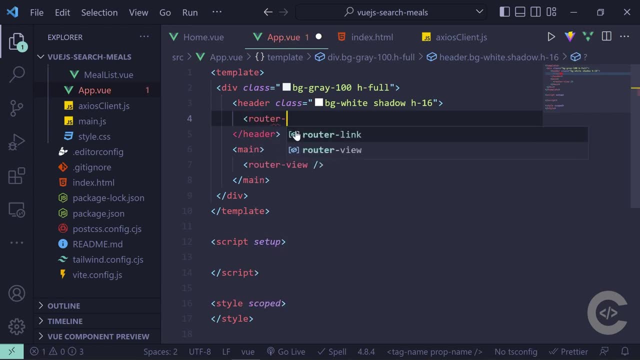 we can reduce the shadow as well, that's nice, that's nice, and we can give it also on the left side, we're gonna have rotor link, probably, which will go on the home page, that's gonna be home, and let's specify right here, two, I always, like, one good practice, I don't know if it's good 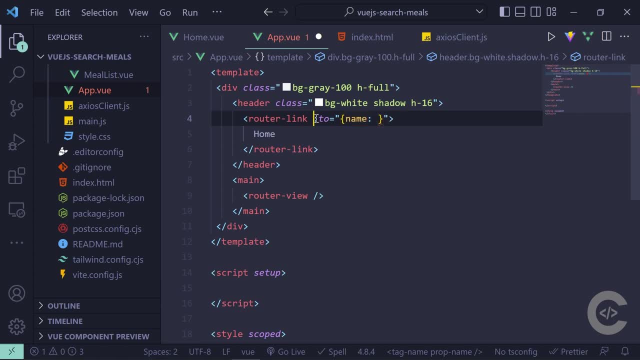 or not, but one standard I have, I always specify, 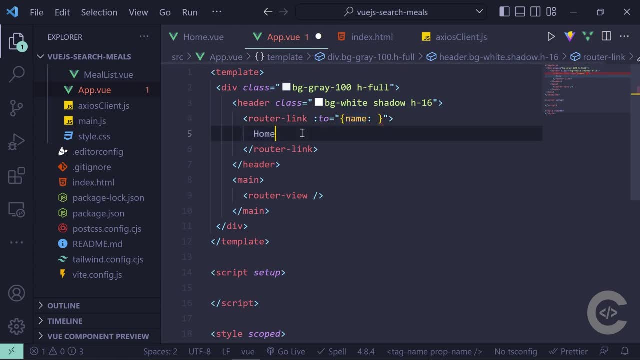 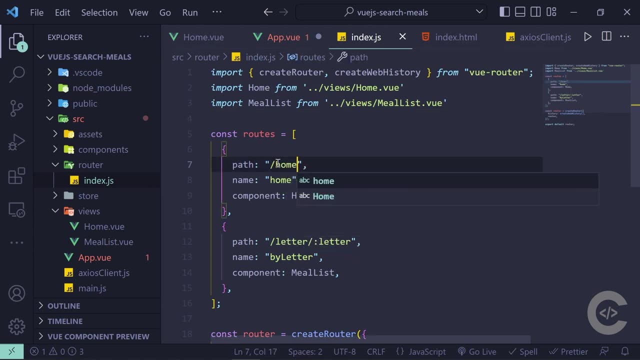 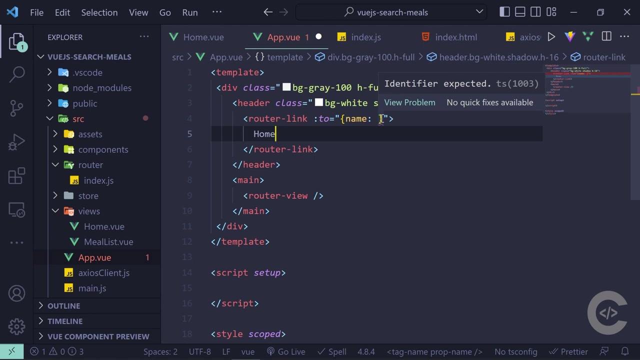 okay, in the future if I want to change the path, and call this home, imagine that I am using, right here, slash, and later, and I use that in 10 places, later I decided to change that slash into home, I have to go and replace all the places, okay, and specifying the name is kind of a safe way in this case, so the name will be home, and let's, by the way, 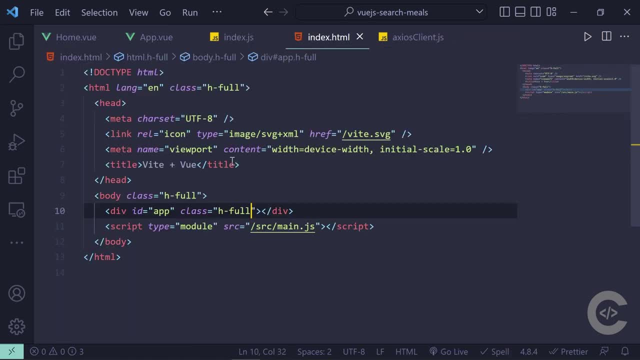 this into slash and we have this in the app we have this rotor link and we can create now a 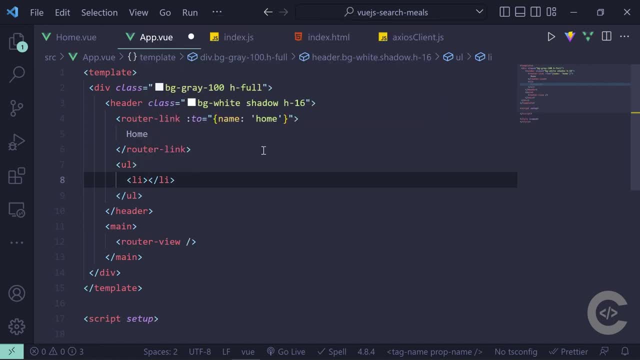 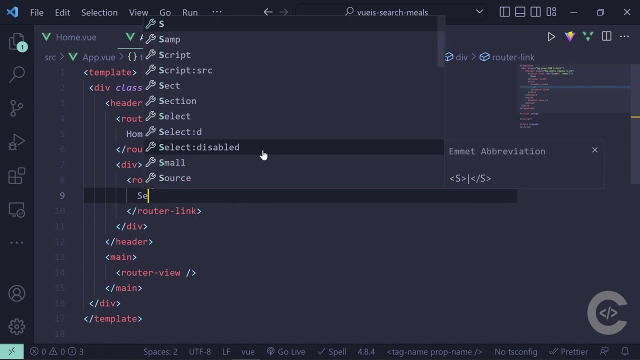 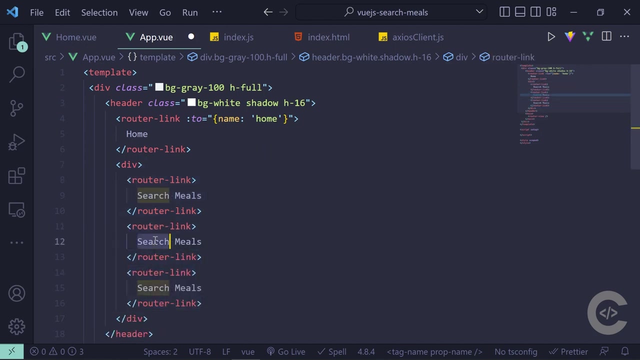 navigation an order list inside there we have uh lee or we just can't have normal links they can be inside div probably let's put rotor rotor links and we're going to have search meals one will be search meals second will be meals by letter and third will be 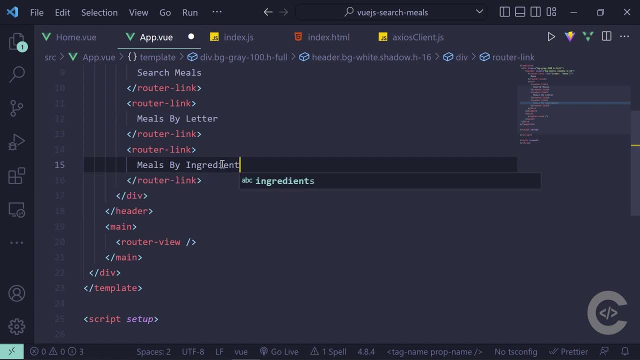 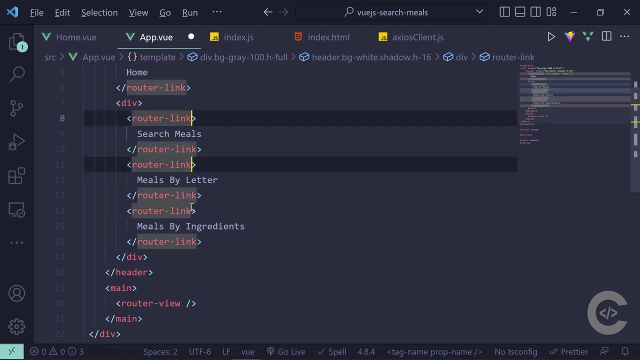 meals by ingredient ingredients all right we have to specify paths right here as well so at the moment i'm going to specify 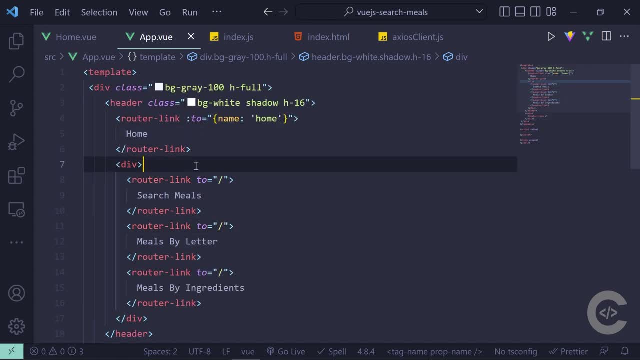 to slash to all of them and let's apply some styling so for this header i'm going to give it flex i'm going to give it a justify between 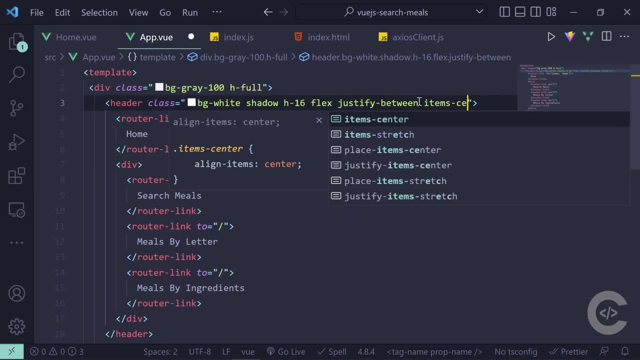 that's good we need to specify items center as well 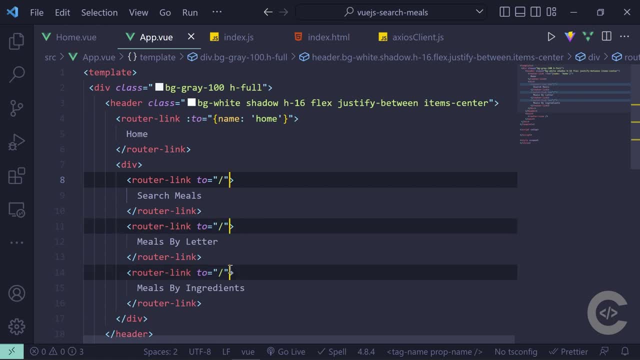 okay not so bad and for these rotor links i'm going to specify class uh we need padding horizontal padding uh we need 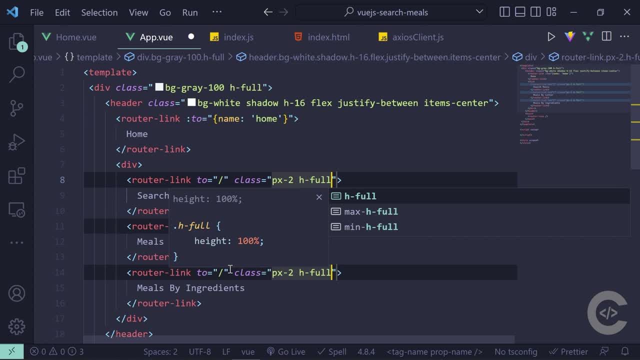 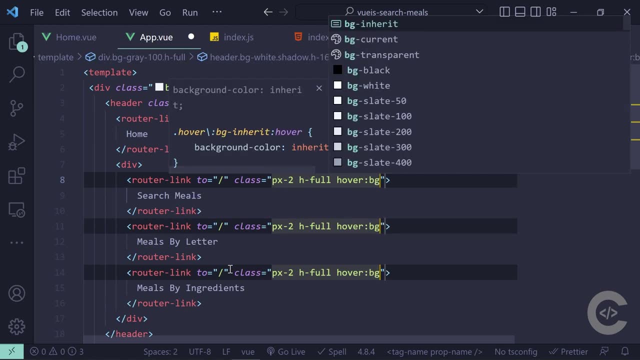 um we probably need full height h full and let's give it also on hover we're going to give it BG purple 200 something like that 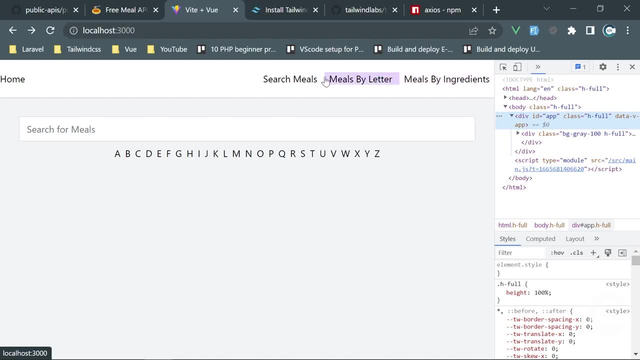 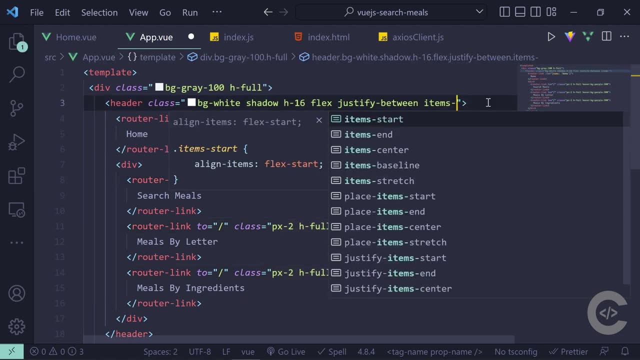 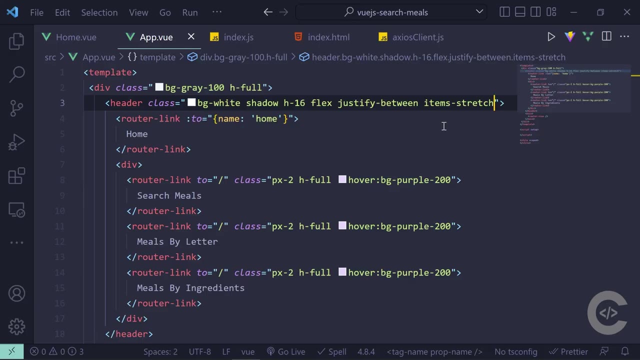 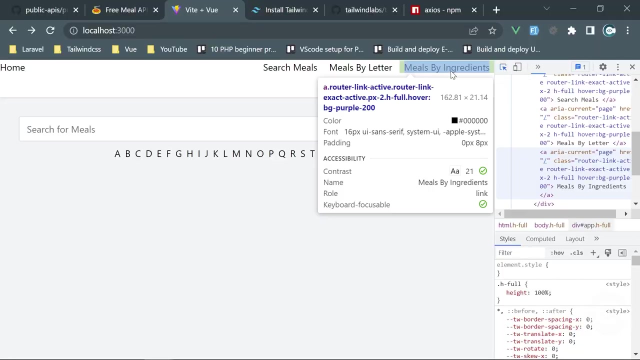 like this let's test this functionality okay this is not what i wanted now items center maybe that should be items stretch okay this is this doesn't work as as i want so if i inspect this 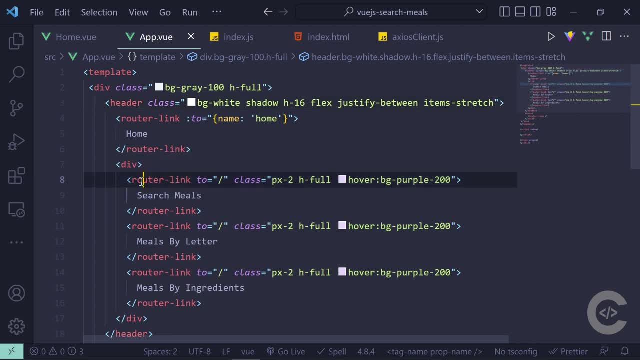 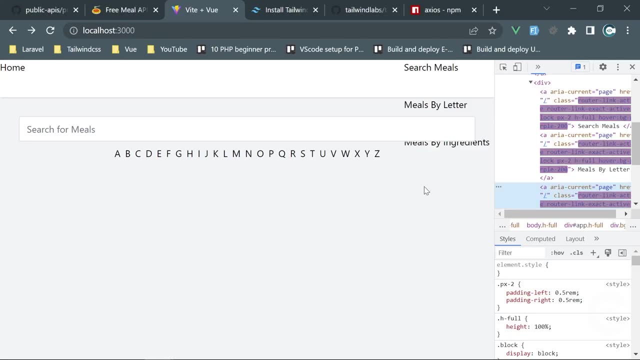 i have the router links i think because they are a elements uh we have to provide like maybe block to make them block level elements or inline block probably inline inline block 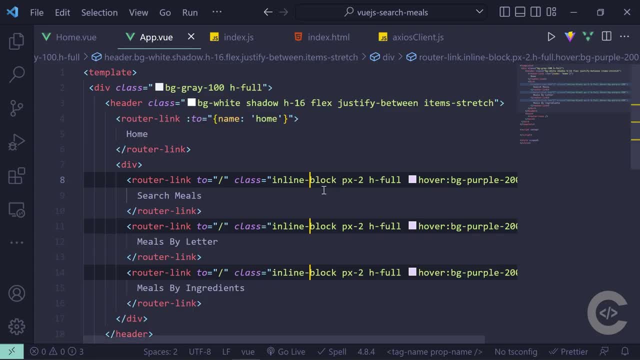 okay that's more like it and let's give this one also flex items center and let's give it gap of 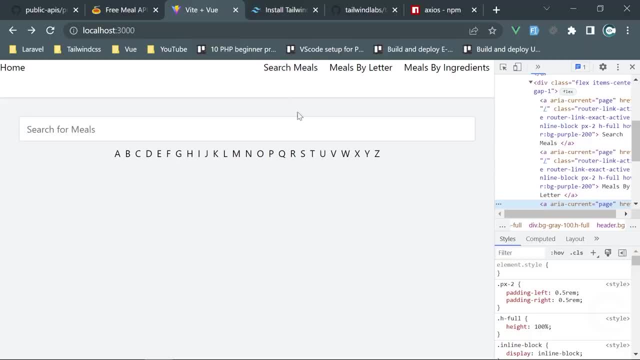 one probably and we need them to be displayed 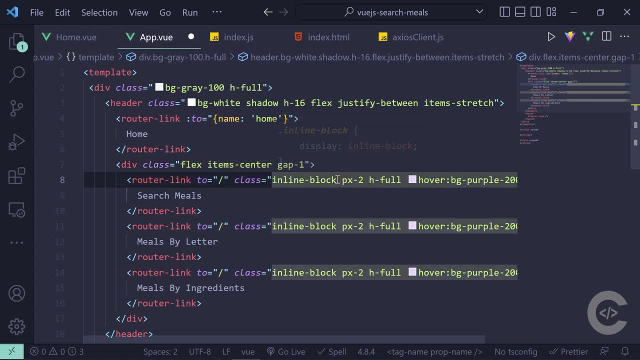 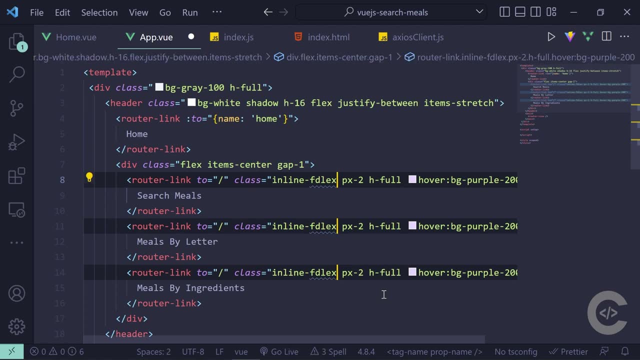 well those block elements those should be probably changed into inline flex flex and items center all right here we see that let's give this one also 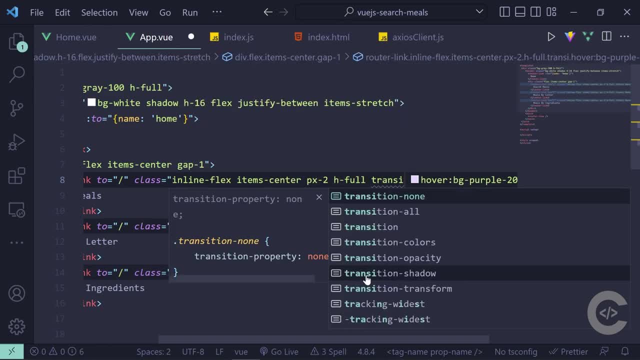 a transition transition transition on colors and let's change this into 100 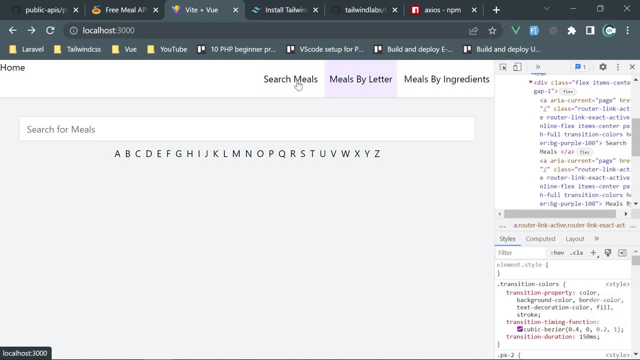 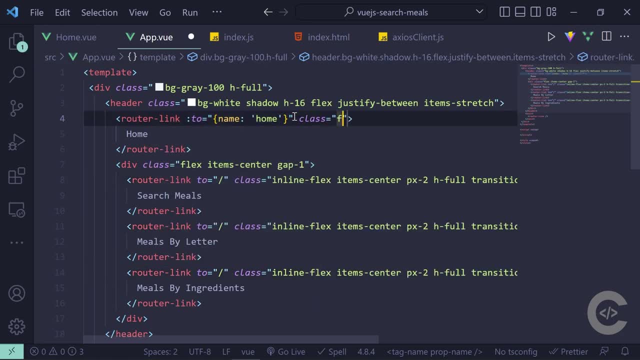 okay we have them and let's now apply some styles to home as well so this should have also class flex uh not flex maybe but inline flex inline dash flex let's give it also items center and h full uh padding x five 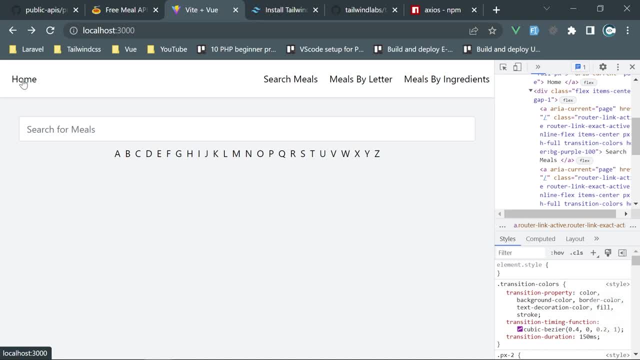 okay this is our home whenever we click we go on the home page like this and we have search meals and meals by letter and the meals by ingredients and i'm going 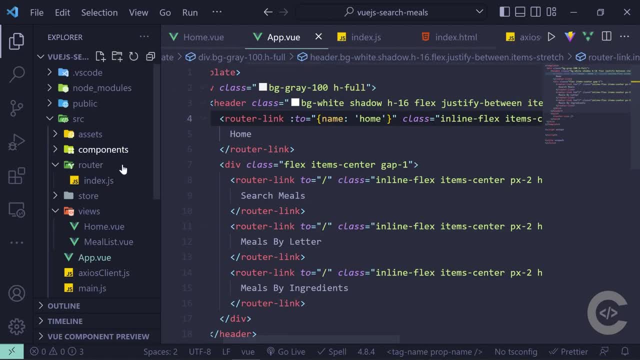 to create now three different views for those files and let me actually duplicate this meal list 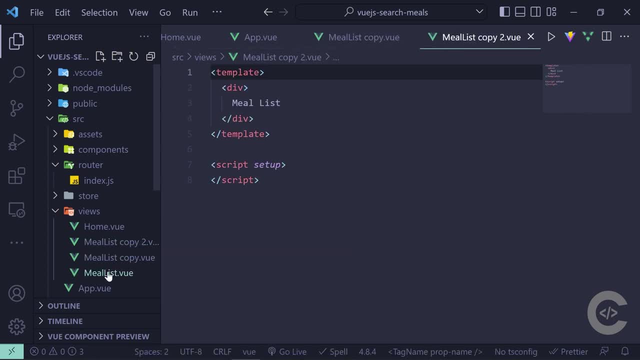 two more times and this one will be search by search by name 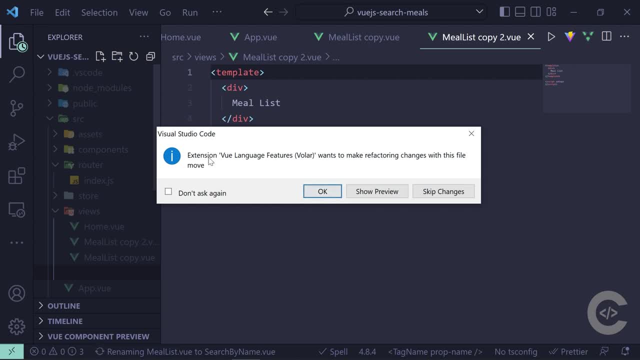 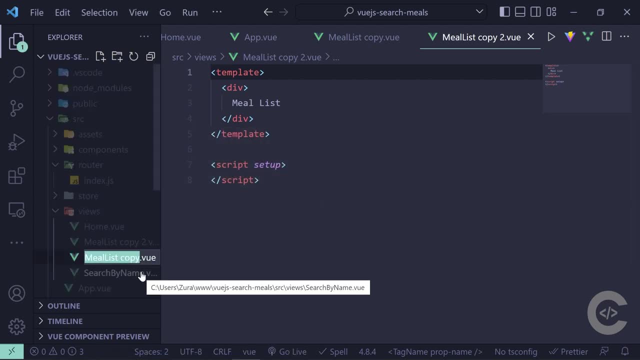 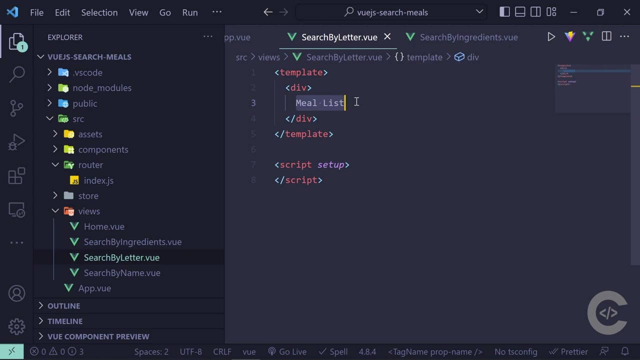 extension view language wants to make refactoring changes with this file okay let's do refactoring the second one will be search by letter and the third one will be search by ingredients all right we have all three components let's give them corresponding texts by search by letter this one will be by name and this one will be 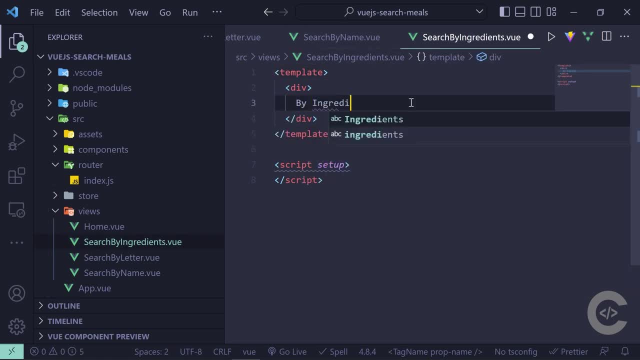 by ingredients all right we save this and now we have 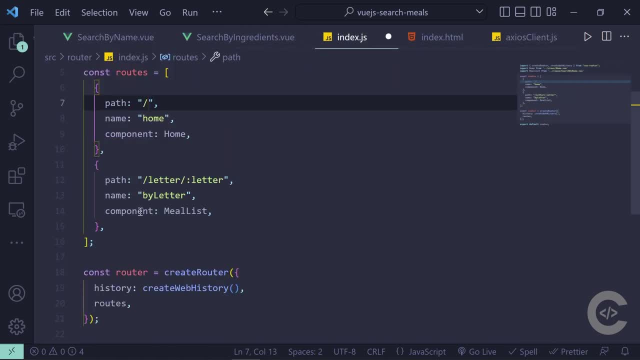 to open rotor and let's configure those routes let's duplicate these two more times it's going to be by by name probably or by keyword whatever and we can specify right here name of the meal and let's give it also by name as a name and that's going to be what's the name search by name 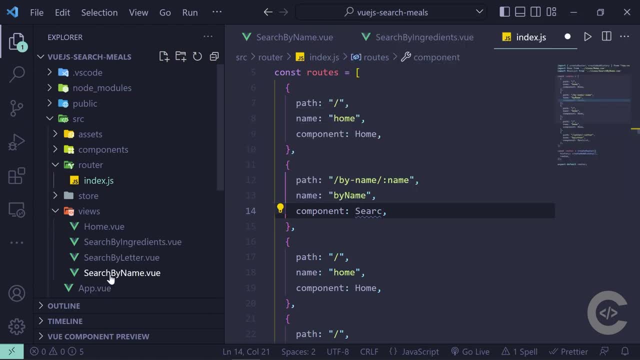 okay search or probably probably we should call it meals by name meals by name let me quickly do this meals by ingredient and meals by letter all right so we have this 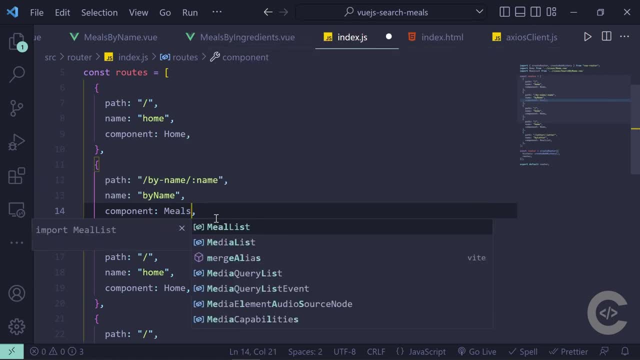 and there's going to be meals meals by name let me copy this oh let me actually delete these two rules and copy this one because modifying this one will 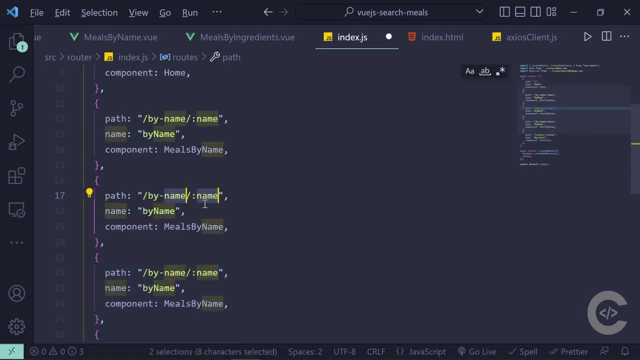 be much easier okay this should be by letter right here we will need 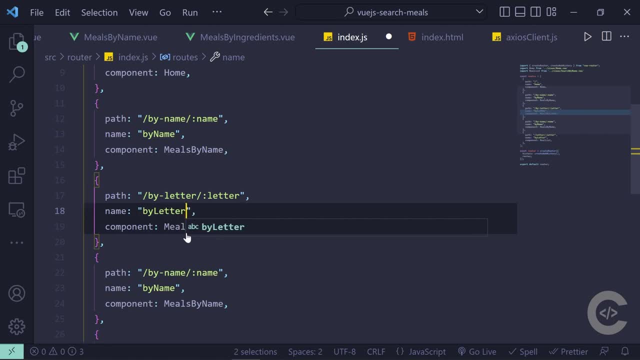 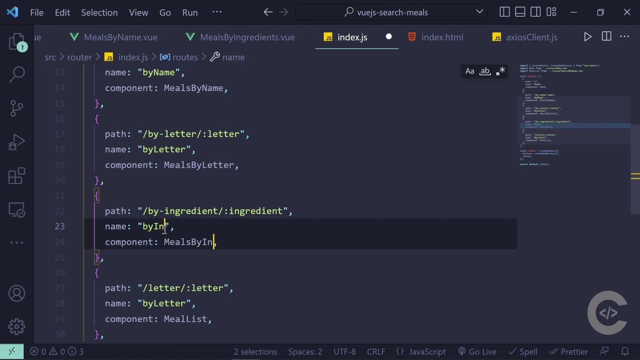 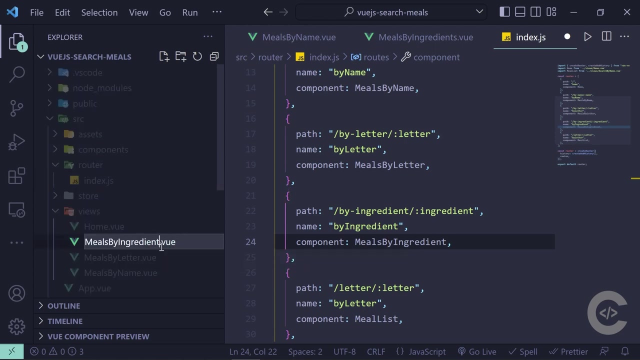 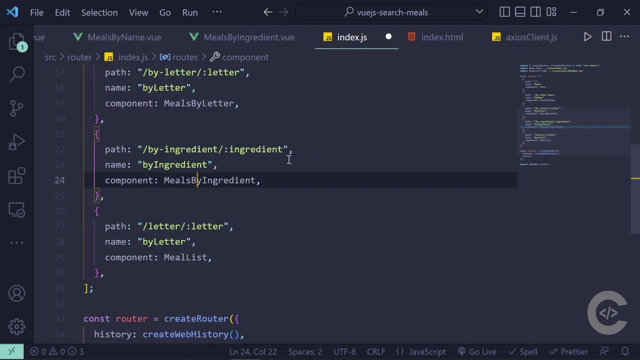 a letter and down below we're going to need ingredients or ingredient and here we will need ingredient as well meals by ingredient let's change this into singular form meals by ingredient meals by letter meals by name all right we have those view files ready and let's now import them 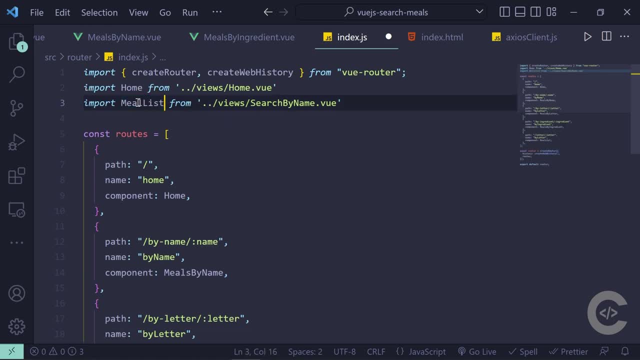 and meal list doesn't exist so we should call this meals by ingredient for example and let's now import them and let's change this to singular form meals by ingredient 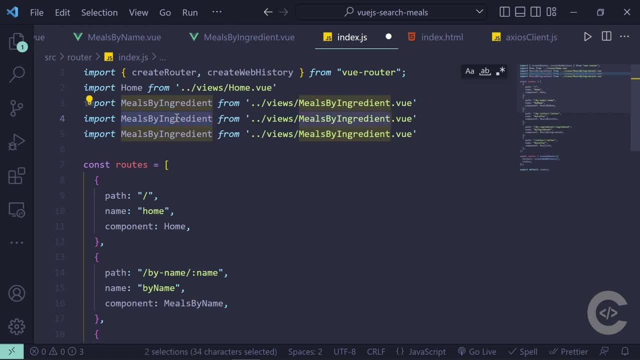 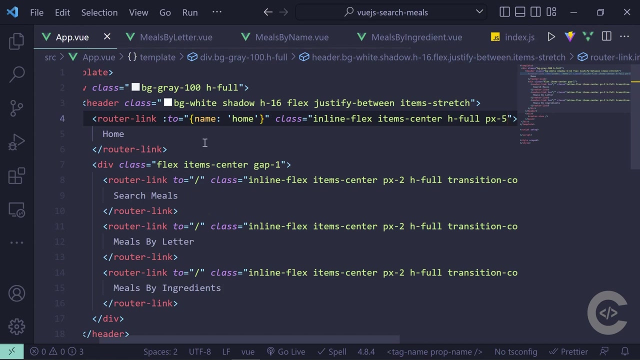 here we go and I'm going to duplicate these two times and that's going to be meals by later and the second one will be meals by name we have all of them created and imported right here and if we go now in up dot view we have to adjust these rules so 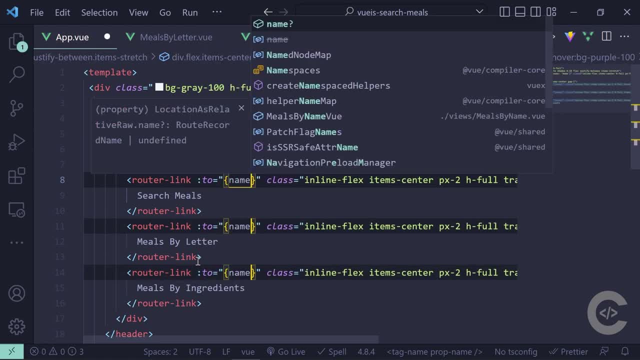 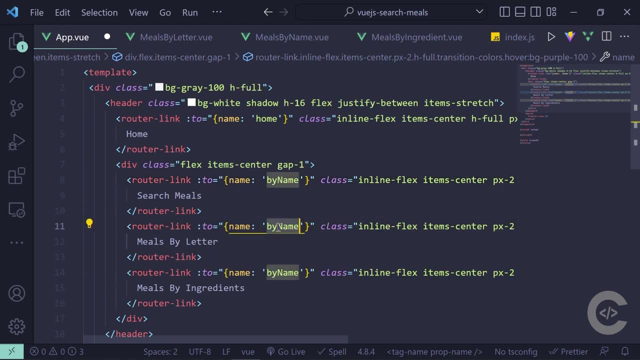 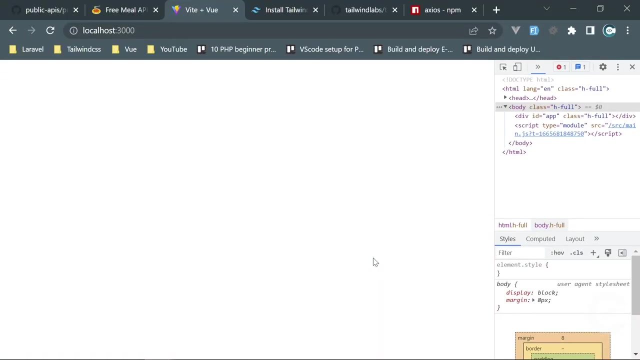 I'm going to change this into two-way binding and I'm going to specify name right here to be by name this will be by name this will be by letter by letter this will be by ingredients all right so we have this now let's reload the page we probably 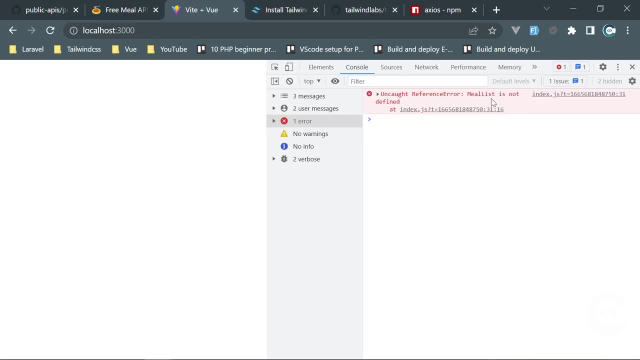 have an error let's see mail list is not defined and it is used it is used in 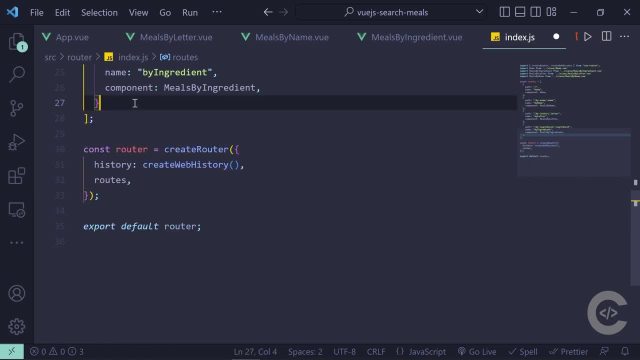 router okay let's remove this let's quickly remove that and we just reload 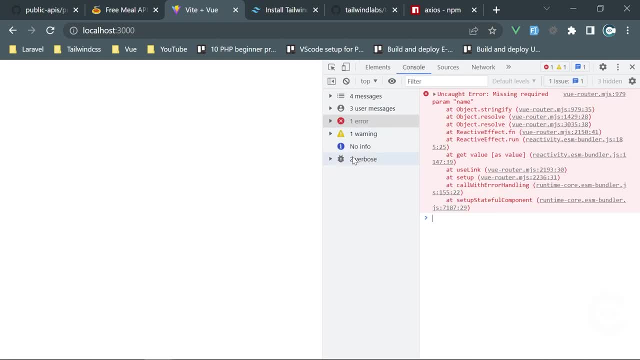 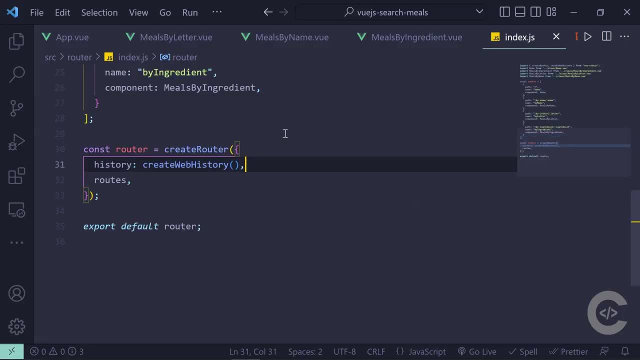 the page and we still see an error missing required param name where is that coming from from up view we do have name here 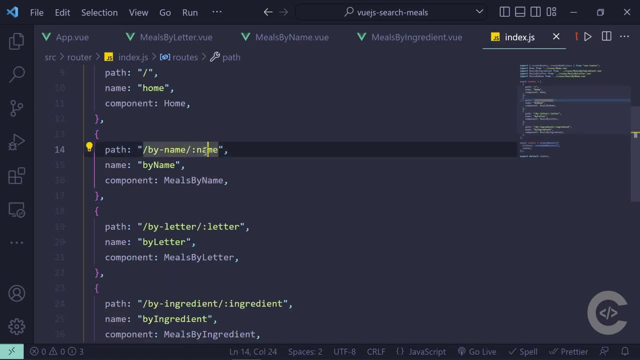 aha so this is this is required params all right i think they should not be required they should probably be optional arguments so if i'm going to put question marks right 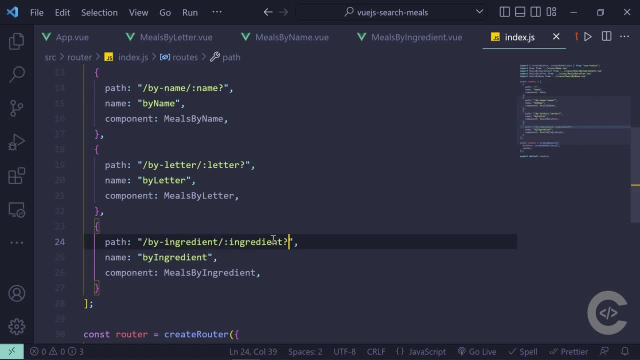 here so all of them will be optional so we just reload the page let's see no match for name by ingredients i think that was used somewhere so if i just 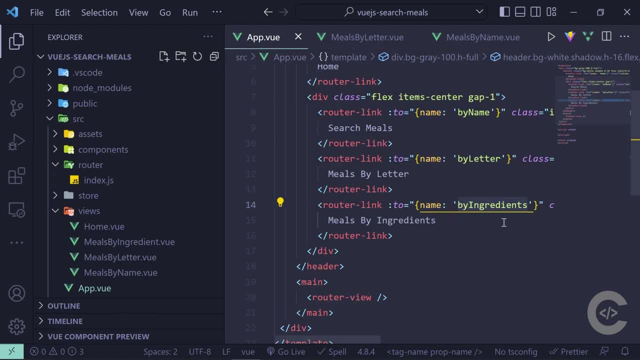 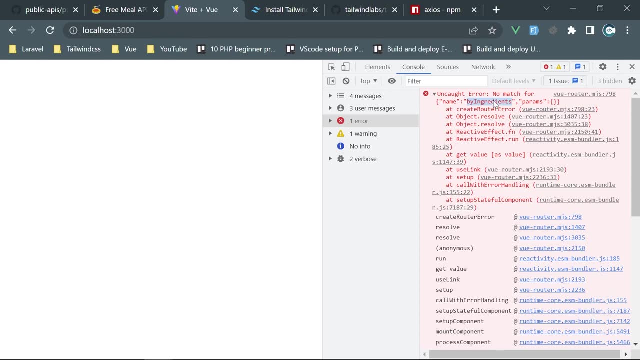 search for that that was used where right here the params is empty no match for name by ingredients should be probably in 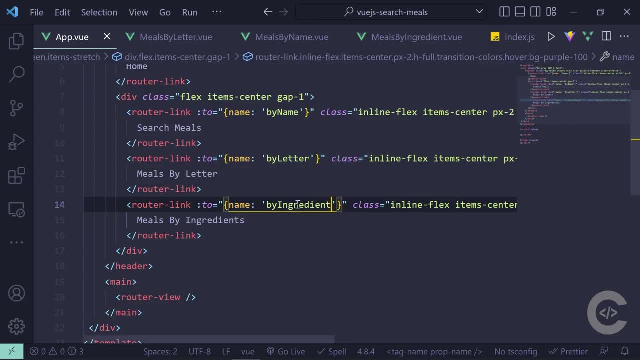 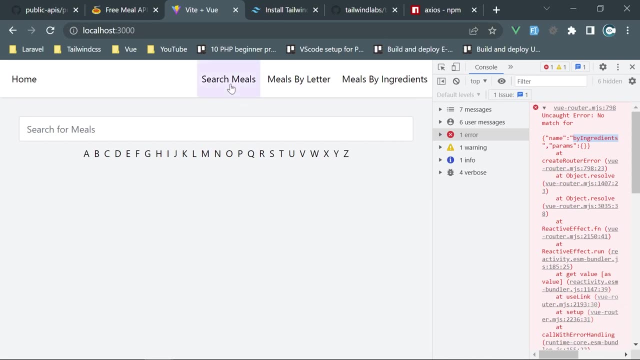 singular form yes it is so we have wrote named called by ingredient all right now we have this layout as well as we have different pages okay we navigate between these pages if we go in the home we're going to move this search right here and this this letter 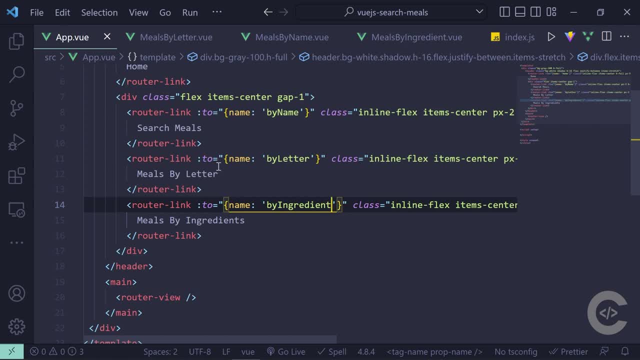 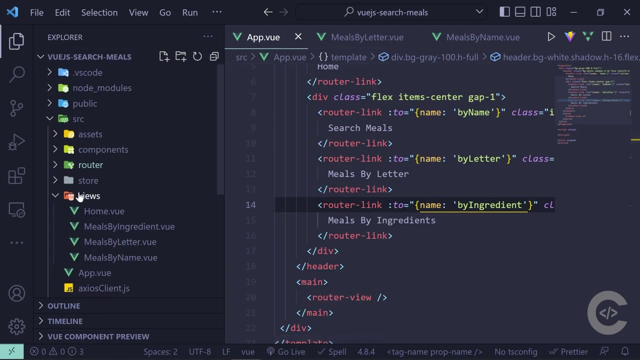 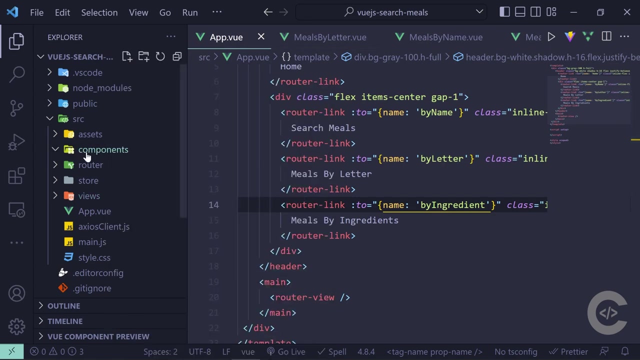 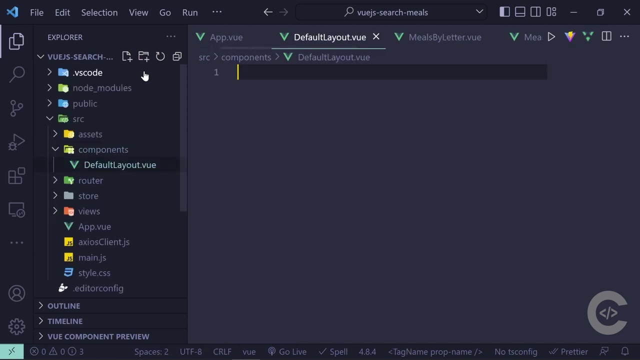 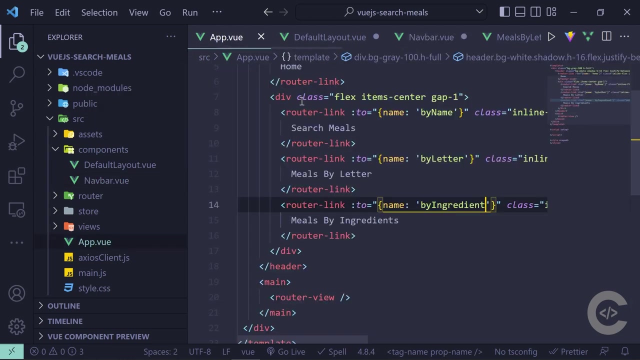 right here but i'm going to also define a new layout like when you are building an application you might have multiple layouts you might have a layout for authorized users you might have layout for guest users even though we are not doing authorization at this moment we will see how we can have multiple layouts and in this case in the components folder i'm going to create default layout layout dot view which will be a normal view component however this one will have another component used inside so i'm going to create now navbar dot view component and this will be the header this header will be navbar so i'm going to take this 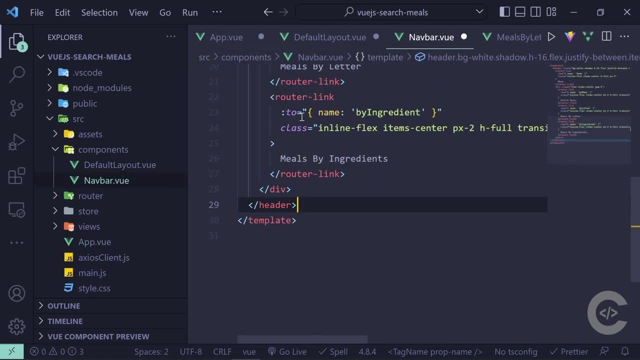 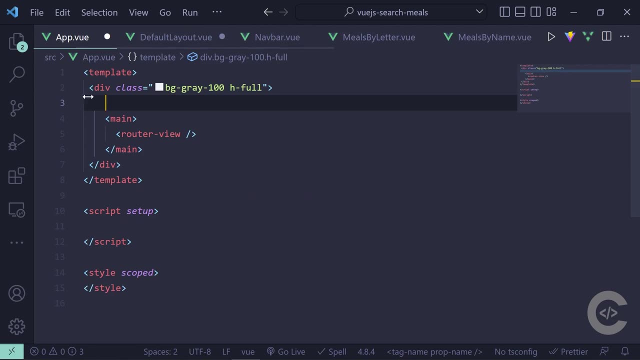 navbar and put this right here okay and we format the code we have this navbar and if we go now in app view i am going to basically 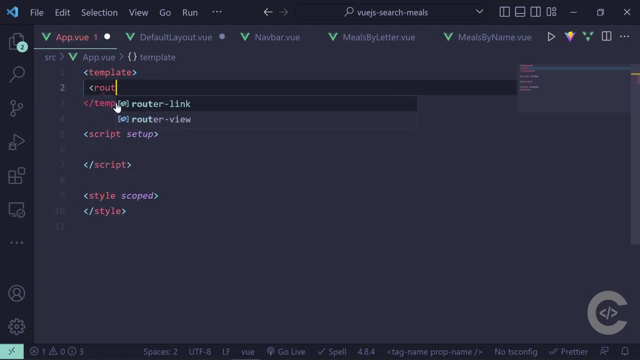 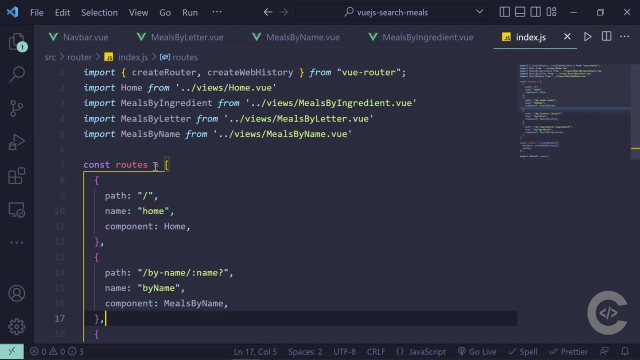 change this and just use again rauter link sorry router view all right however we are going to have however we are going to have layouts and if we open router and i'm going to confirm that it works 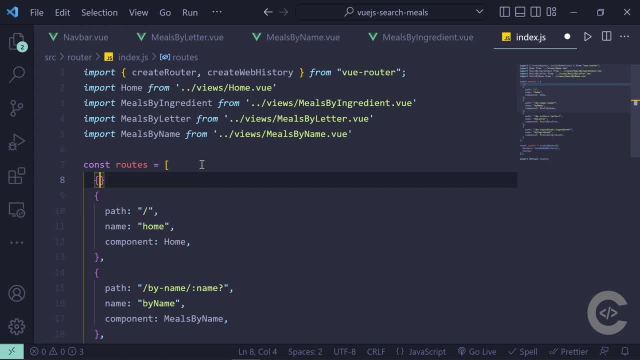 going to configure right now default layout so let's create new route right here we need to specify path i'm going to specify it slash all right we have slash i know down below but we're going to modify this so we are going to create right here we're going to use component 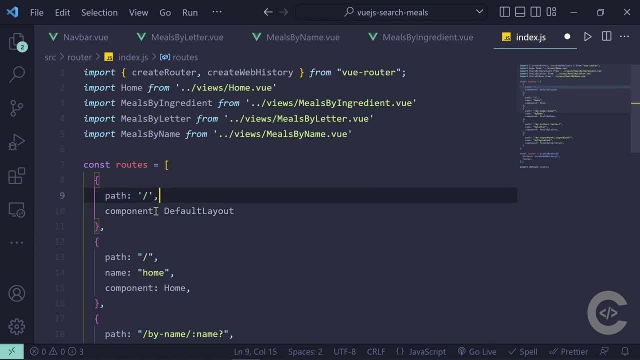 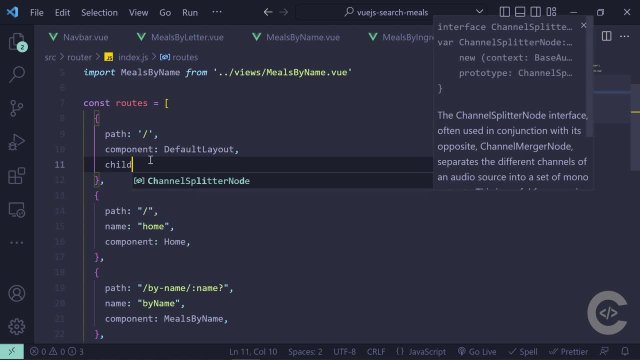 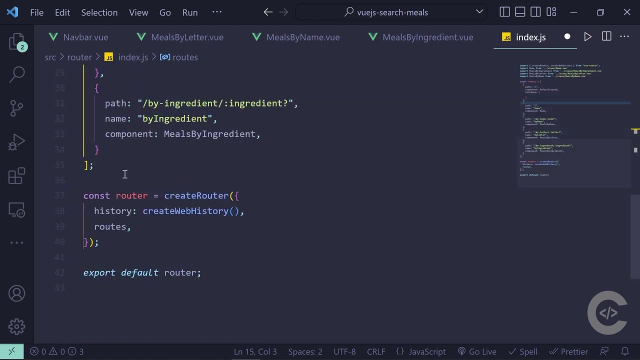 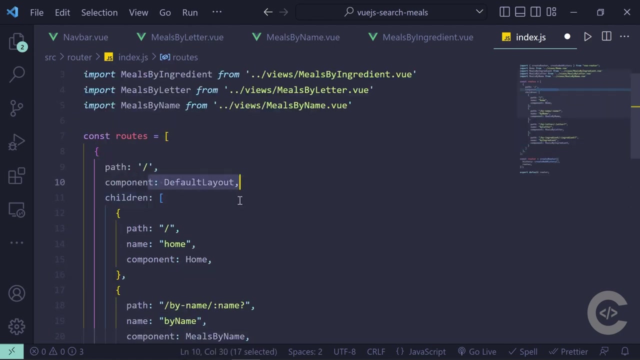 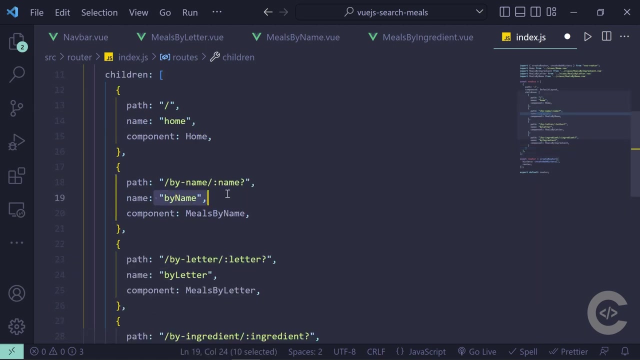 default layout all right and then these views will be children of this default layout so let's put them as children and let's create an array and let's cut everything all right and put them right here okay so we have now wrote slash and we have children they will work in the same way as they were working before we have um we have uh accessing to roads by name so it's gonna work in the same 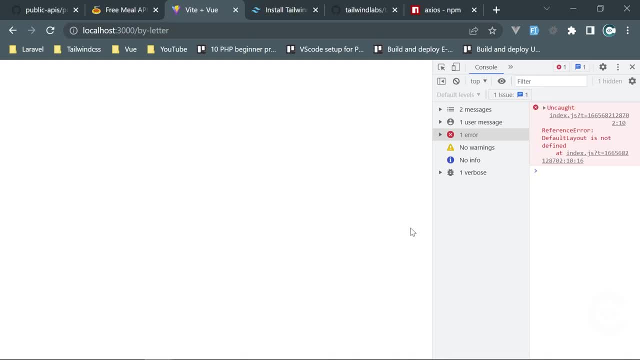 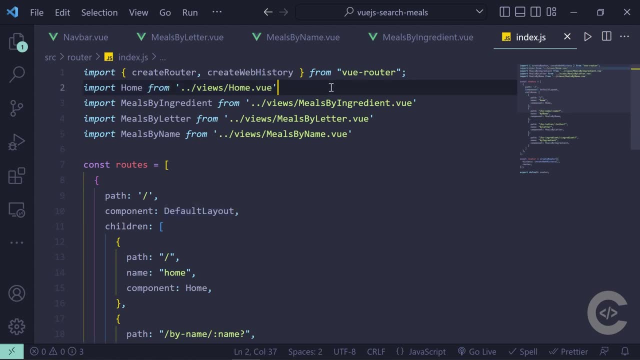 way however let's have a look in the browser we're gonna have an error and we're gonna fix that default layout is not defined yeah we have to import this default layout and that should come from components import default layout from go one directory 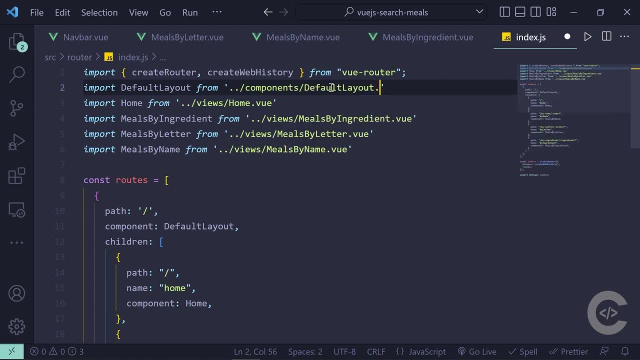 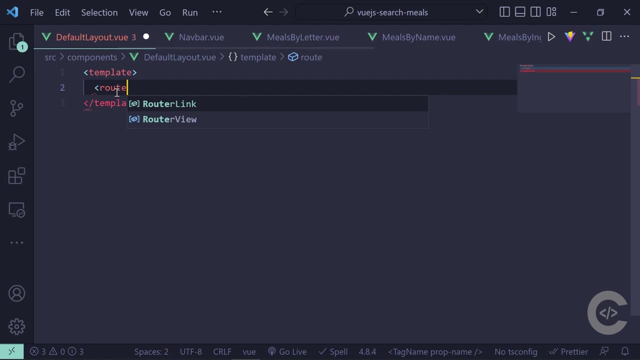 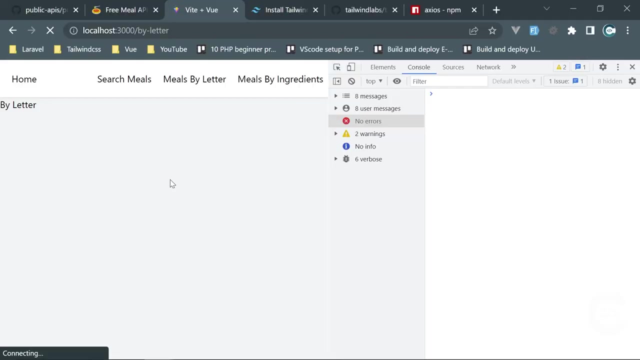 back go in under components and paste this dot view file so we have default layout let's reload the page we don't see anything because in the default layout right here we don't have a router router dash view all right we need router view right here as well but we need the router view and navbar here as well basically i think i copied something from the app so let's actually go in the app and i'm going to quickly undo and i'm going to copy this and then redo and then go in the default layout and paste this right here and in this section we will use navbar okay which we just created and we have to import this navbar here as well in this script let's give it setup and let's import navbar from we go one directory back go under components and we use this navbar so we save this and now we have the exact same layout as well as the default layout as well as the default layout that we just created so we can the implementation is the exact same however now we have default layout and in the same way 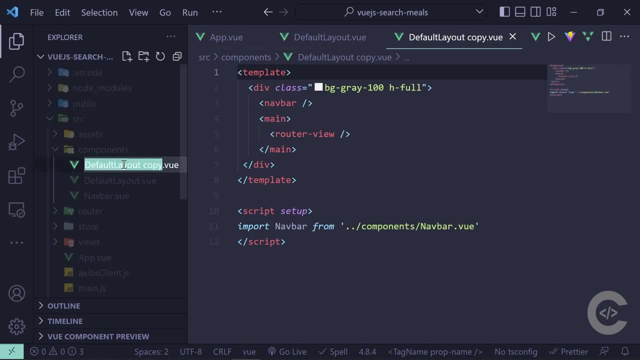 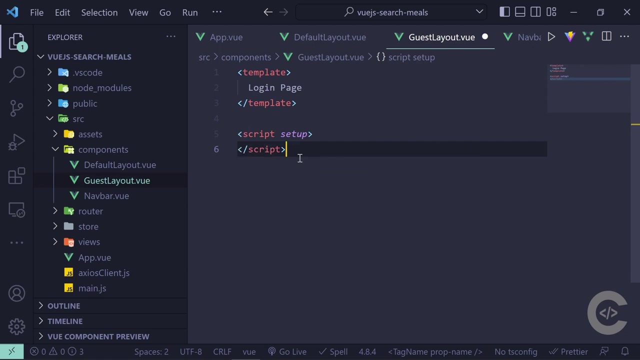 i can create now second layout let me copy and paste this and call this guest layout let's skip the changes it will be just guest layout however i'm going to remove this and just type login page as an implementation i'm not going to actually do login or something like this but we see login page right here and if we go in the router 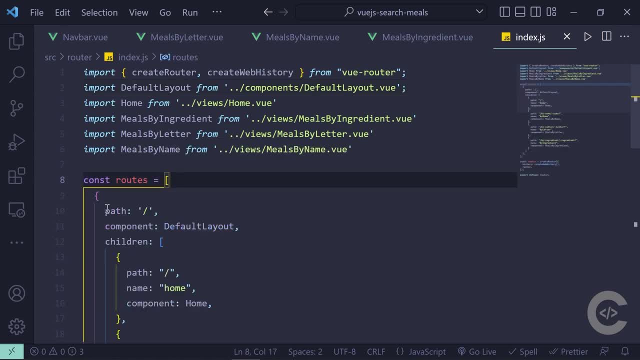 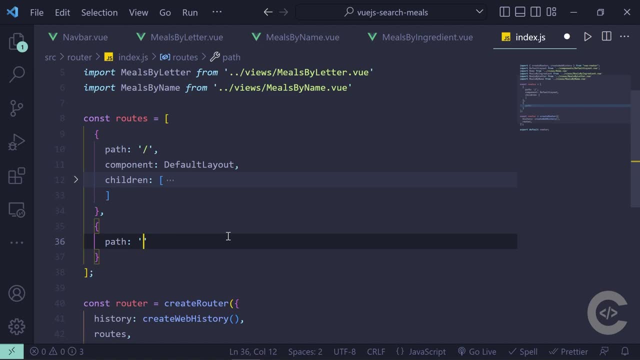 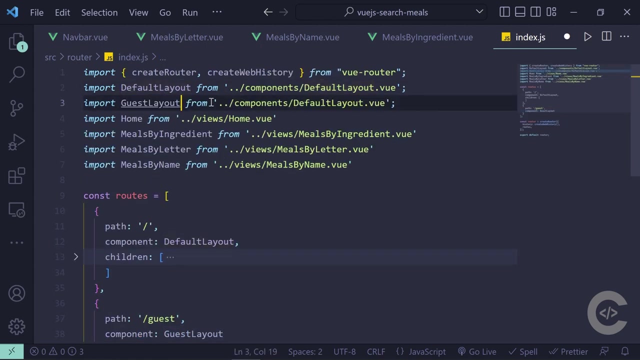 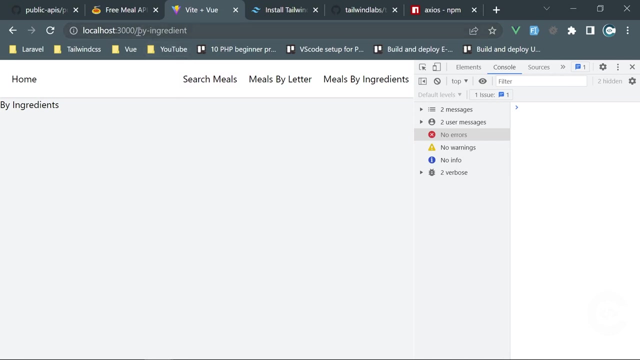 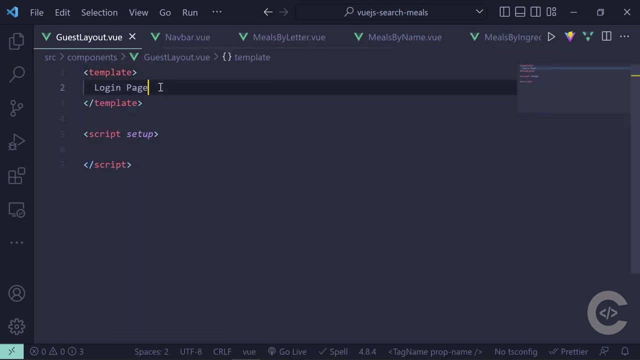 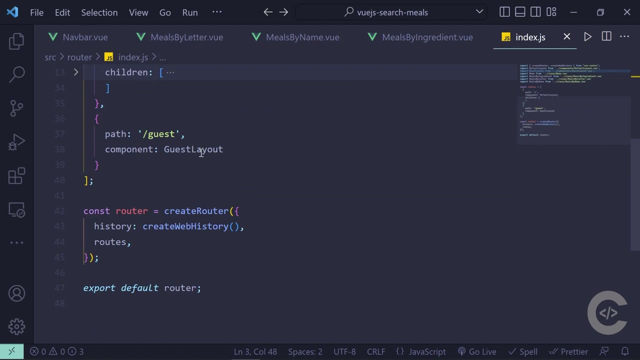 and and we're going to create right here an additional new route which will be for example slash auth or slash guest all right because we have guest component so component will be guest layout and the guest layout needs to be imported here as well and imagine that now we have a guest layout and the guest layout will be displayed basically when you access slash auth and at the moment i think there's nothing in the guest layout uh no there's a login page and it should be displayed we have the guest layout 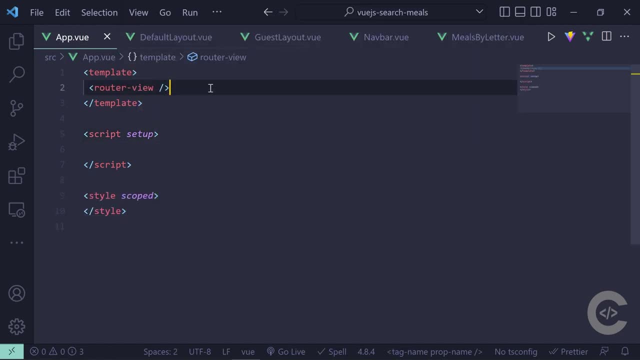 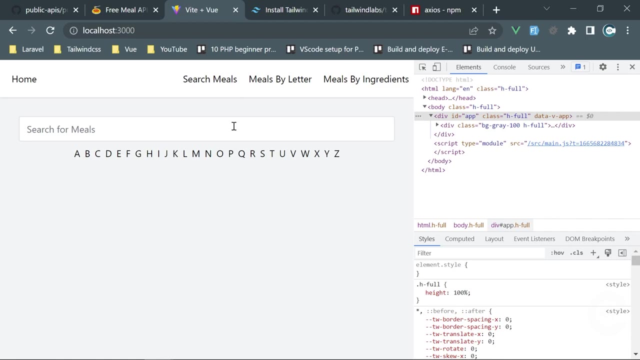 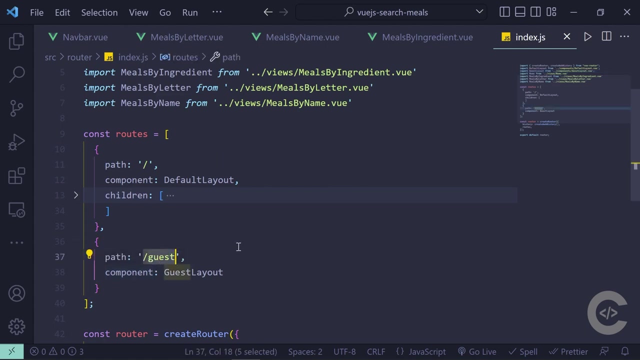 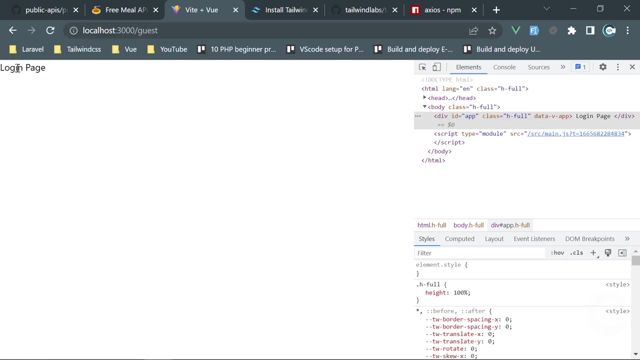 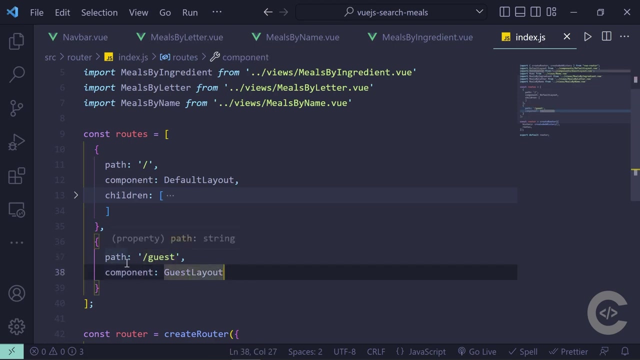 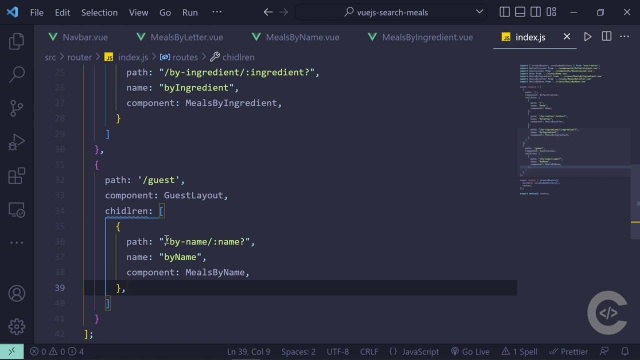 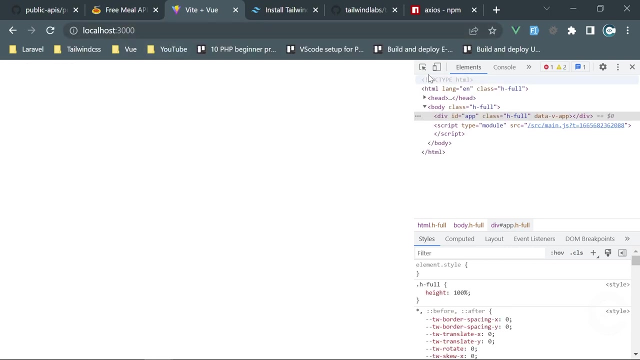 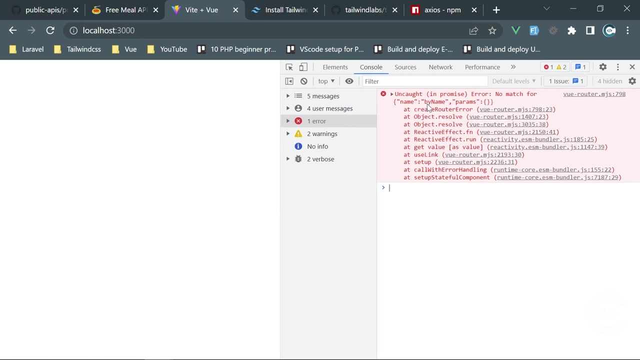 okay let's open up view we have router view here if we access to slash that is displayed okay and this is displayed we have slash path here we have slash slash guest we don't have slash auth we have slash guest let's hit the enter and here's the login page okay and this login page does not have this navbar it's a different layout at the moment we have this to be a layout we can define children right here and if i just take any of the routes let's take this one cut from the default layout and put it in the guest layout now that by name we'll use guest layout okay if we go now on home page we are going to see an error okay and no match for name by name params okay what just happened 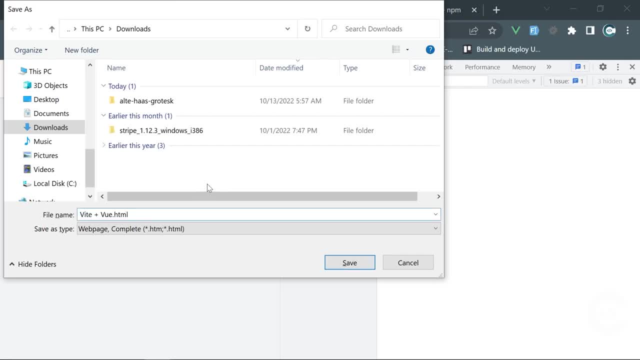 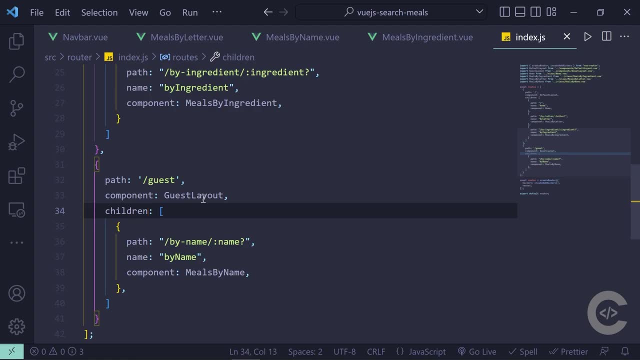 uh here i have this type of children all right so i just reload the page and we see now all the many items right and by name has now guest layout it doesn't have default layout the home page has 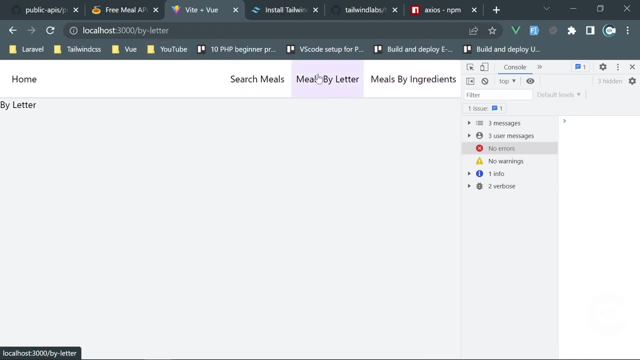 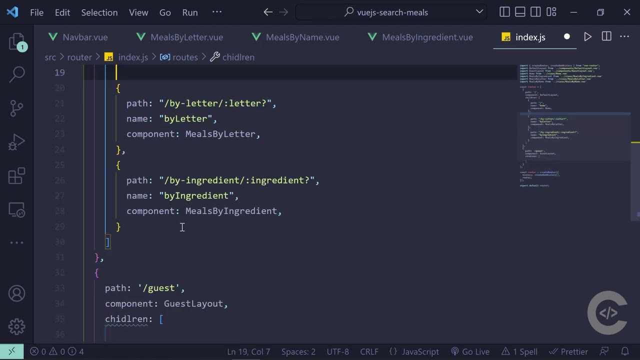 this now bar meal by ingredients has this now bar meal by letters search meals has different layout okay this way you can create multiple layouts in your application if you need even though we didn't need i'm going to leave this guest layer right here just i'm going to move this uh right here so 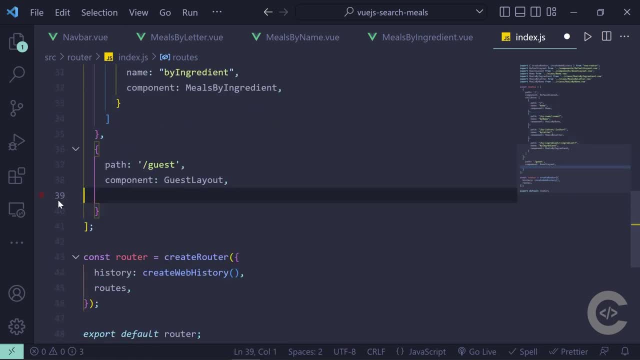 whenever you get this repository or you're going to create a new repository or you're going to create on your local machine you're going to have this guest layout right there and you can experiment 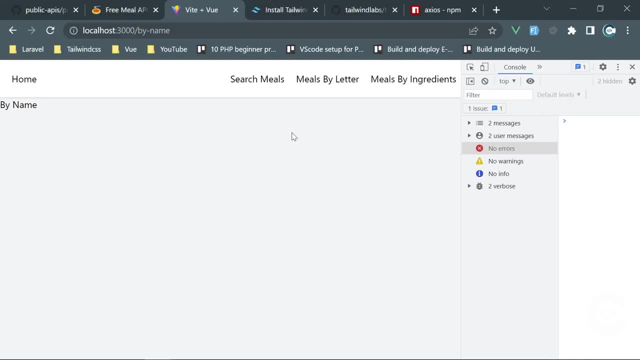 with that all right so we have layouts implemented now i think we can move this input search into this search meals and render ingredients and basically start finalizing our project okay 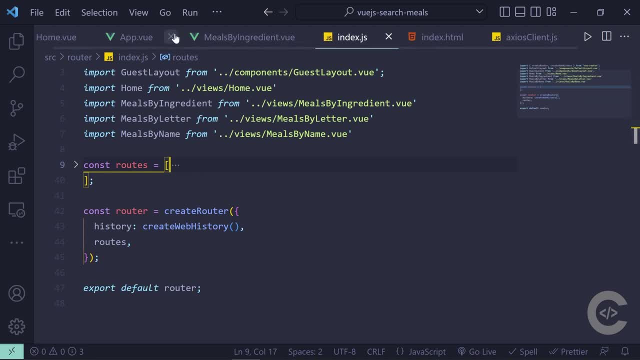 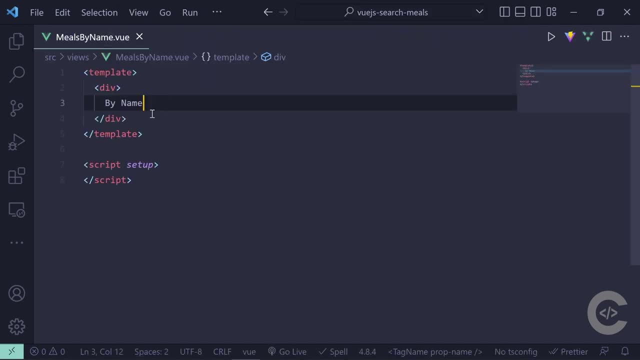 so let's implement the first one let me actually close all of them okay and open um it's called meal by name all right and i'm going to put this search field right there but i'm going to take this from home 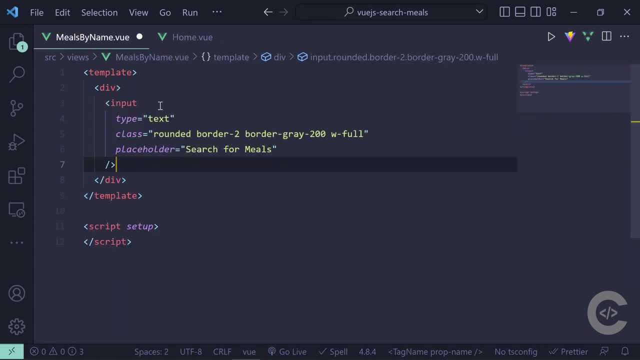 so let me take this and put this right here okay so i save this and if we go in search meals we have this input let's give it some classes padding six and i think that's it 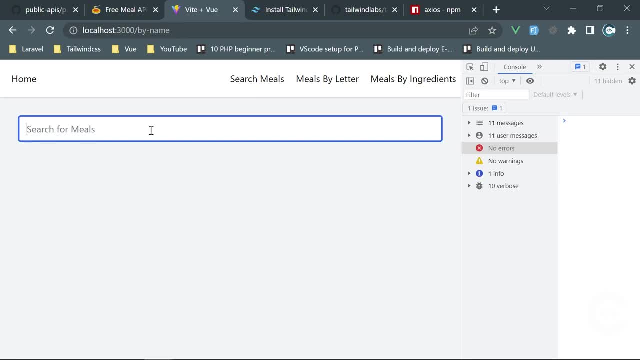 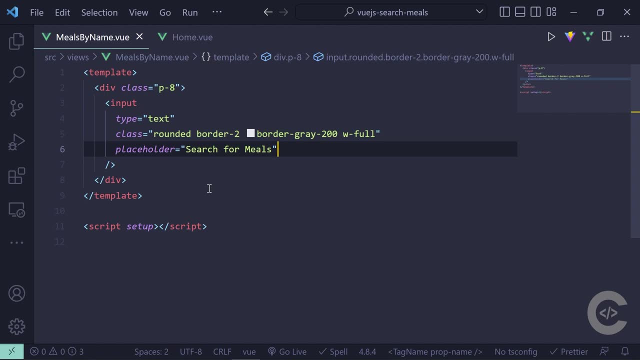 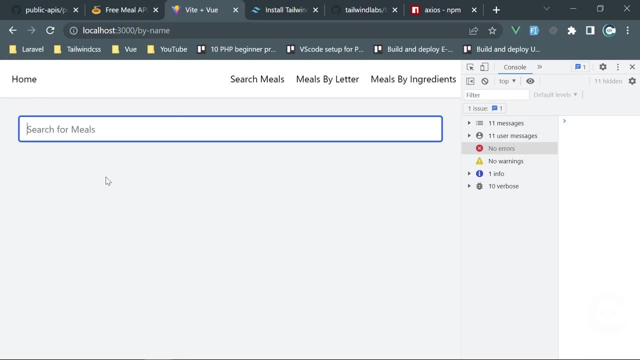 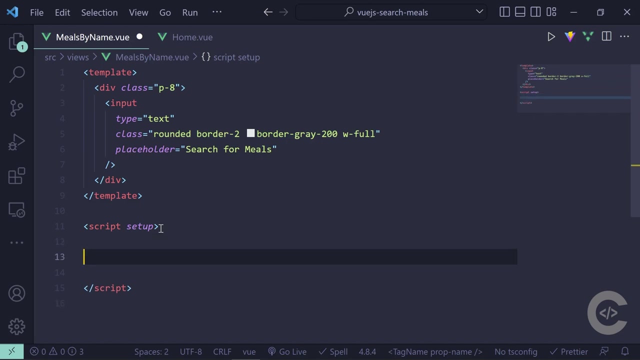 can even increase this into eight okay we have search by meals and let's now listen let's now listen to change of this input field and make a request and to fetch those meals but we're going to save those fetched meals in the view x for later usage okay let's start step by step we already have axios client so on uh on what so basically i'm going to create a function 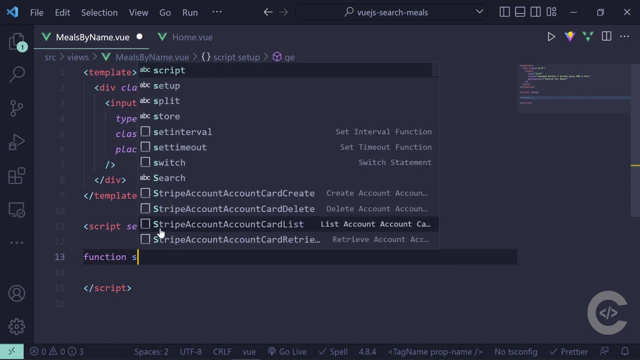 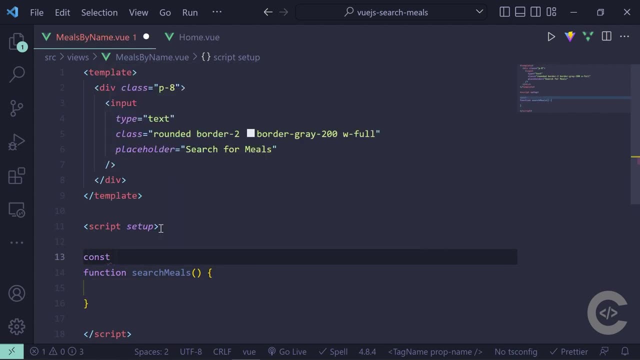 get or search meals okay and let's create right here also a constant field called keyword maybe using ref we're going to give its default value empty string uh keyword and then on this input we're going to give it v modal keyword all right now whenever change event happens on that input we're going to call search meals quick pause right here the 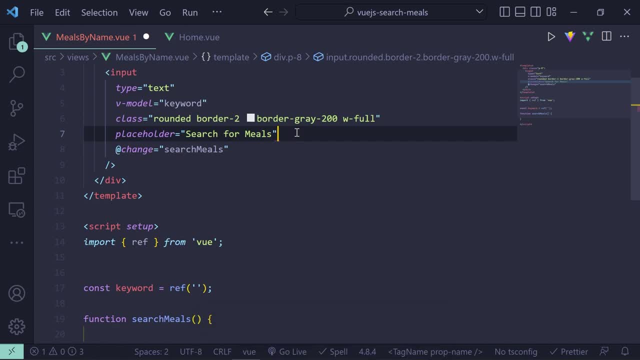 only thing i ask for is like subscribe and cheer but if you really love my content and want to do something even more check my donation pages patreon and buy me a coffee i really appreciate it and i'll see you in the next video bye bye 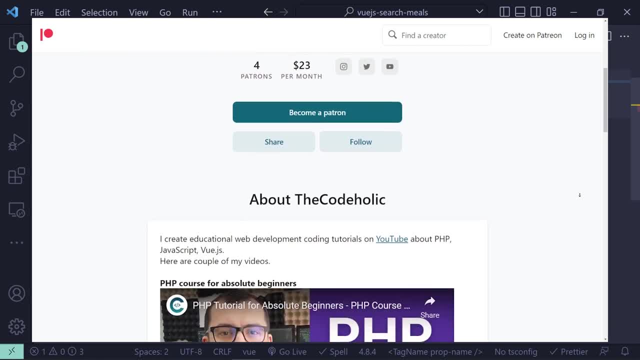 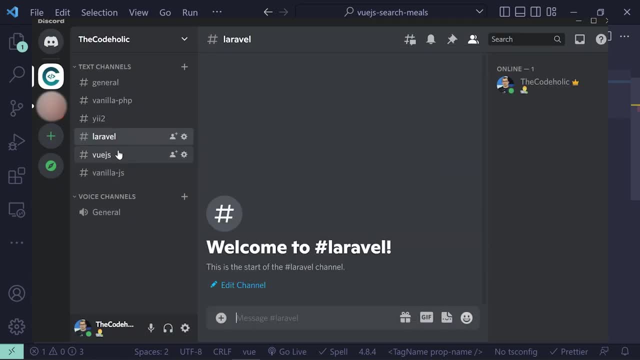 appreciate every single cent you donate and it's going to give me much more motivation to keep creating free educational content i also created discord server which is at the moment only available for my atreons so as soon as you become a patreon you will have access to the discord 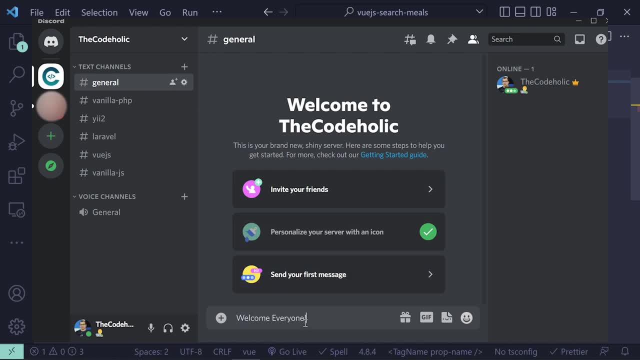 server on which you can ask your questions post your problems and i will personally assist you 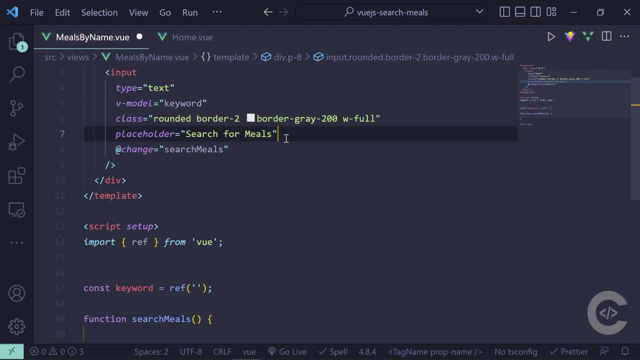 there sorry for interruption let's get back to the video comma is not necessary here search meals will use axios client 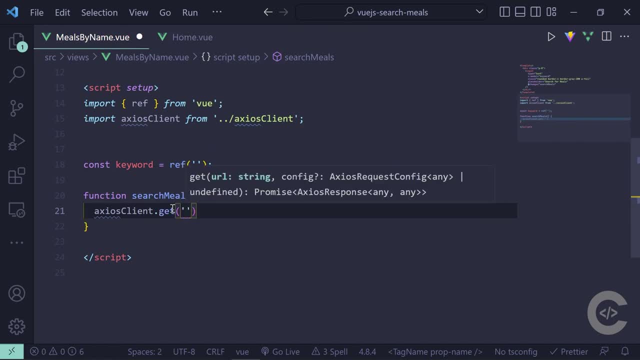 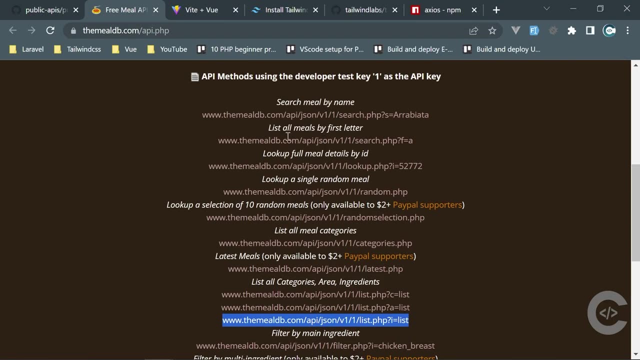 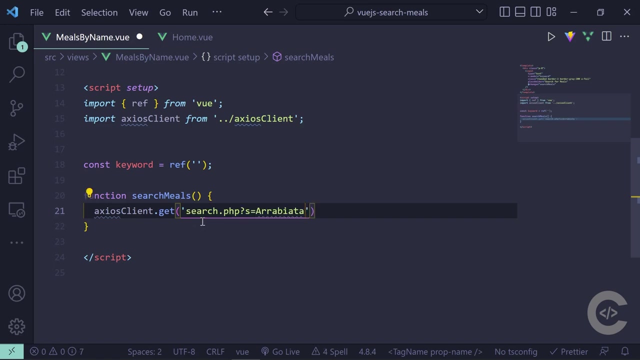 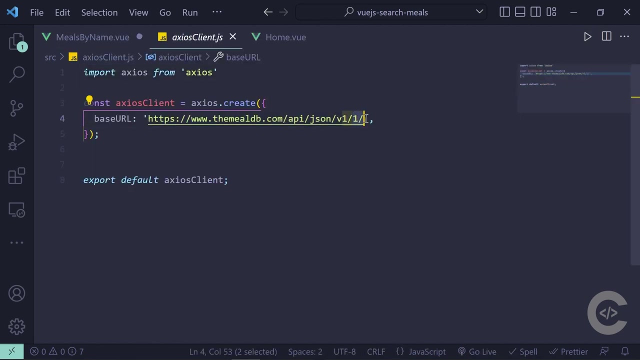 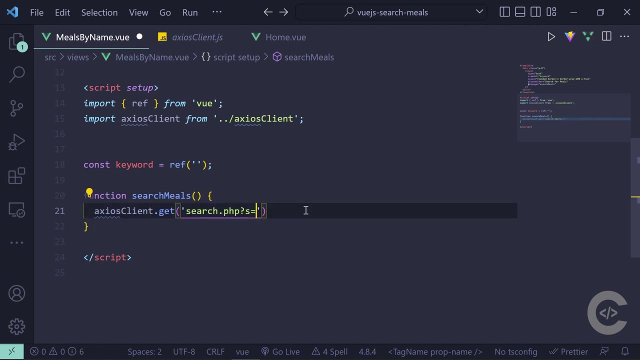 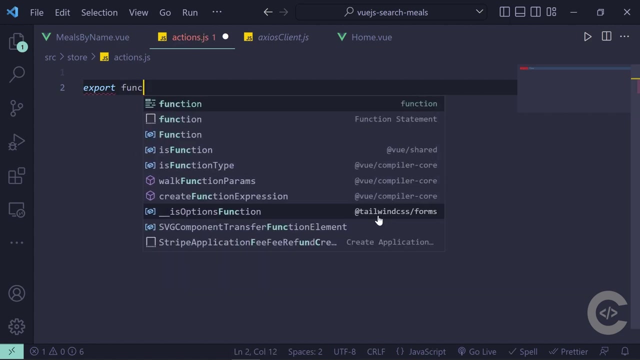 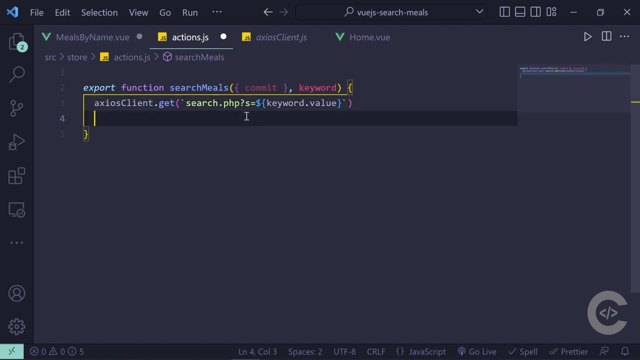 get and we're going to specify right here now an end point to search meals and search meals by name so this is going to be the end point all right so let's specify it right here by the way do we need slash here or not let's check axios client at the very bottom we have slash so we don't need slash here okay and this equals right here we need this keyword so let me change this into back ticks and i'm going to use right here keyword dot value all right so we're making request and we are going to save that information in the store and for doing this the best way is to use actions and now i'm gonna open up actions.js and i'm going to create a function here export function search meals this one accepts an object which whenever we destructure we take commit from there and then it will accept keyword right here okay and that axios client get will go inside here we're making request to that 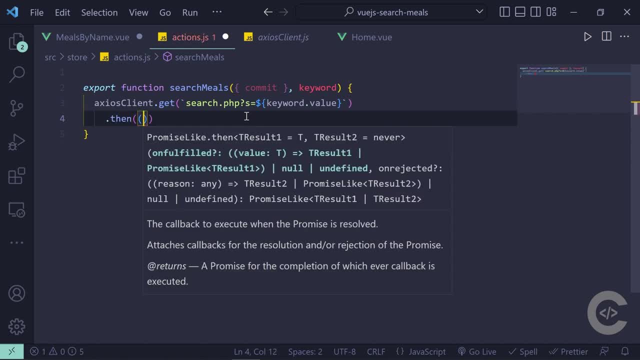 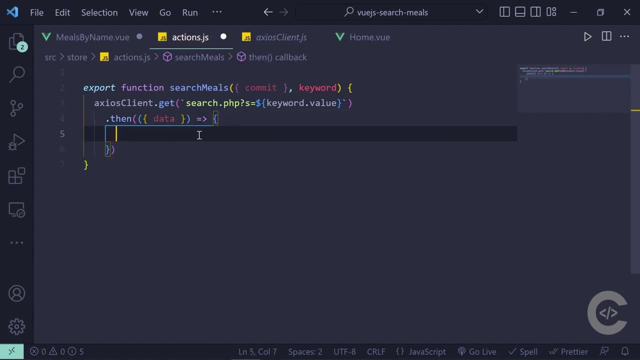 and on response we get the response we destructure the the response and take out the data and then we're gonna commit the mutation to save that received data inside store so for this i'm going to call commit and we're going to specify right here mutation name now let's create in the uh let's create the mutation let's open mutations.js export default set 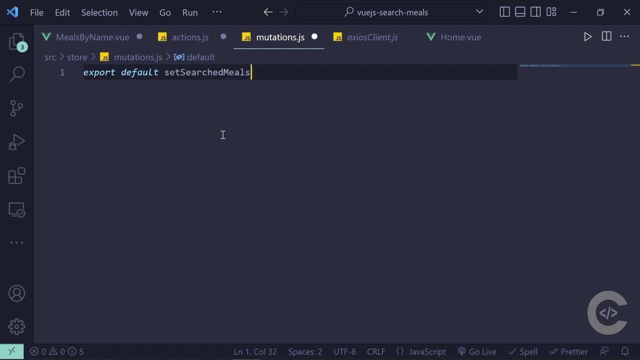 search meals okay and right here we accept state and we accept also we are going to accept meals which we are searched and found right so and inside state we are going to set these meals now let's open state inside state we don't have meals and in this case we're going to create 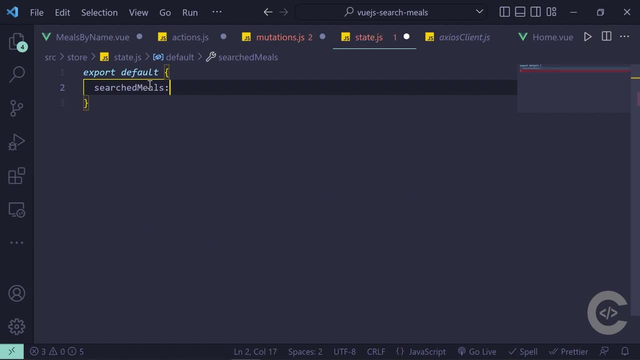 search the meals and this will be this can be an array and we're we're we're going to directly assign something to it or we can have kind of like loading indicator right here okay so this will have loading indicator false and data as well 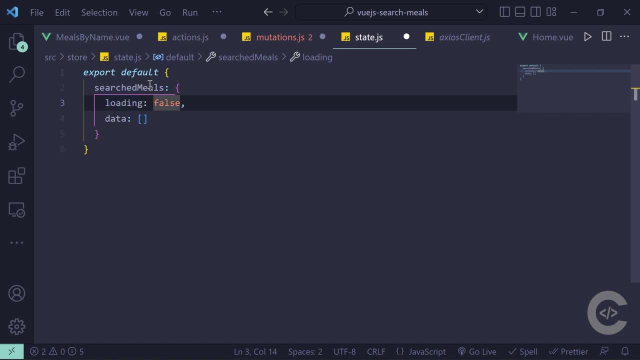 and this loading whenever this loading is true we will see a loading indicator on the client side right here that the searching is in progress okay we can do it like this however these kind of things are um 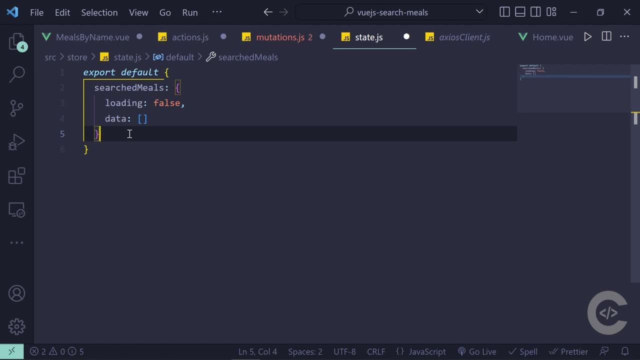 makes this project more complex and it's for a more like complex application so this is how you can do if you want to have loading in the view x but in this case i think just having the data 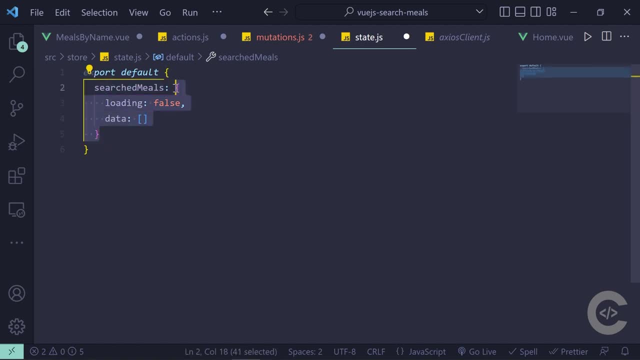 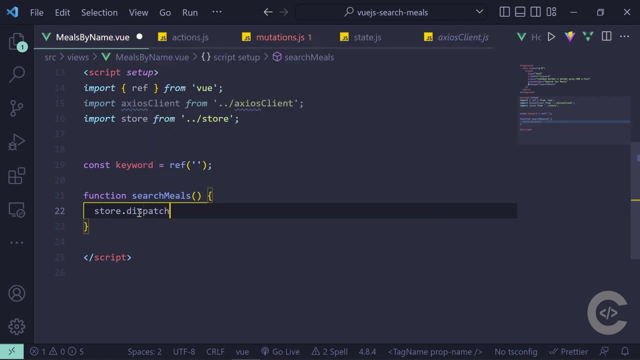 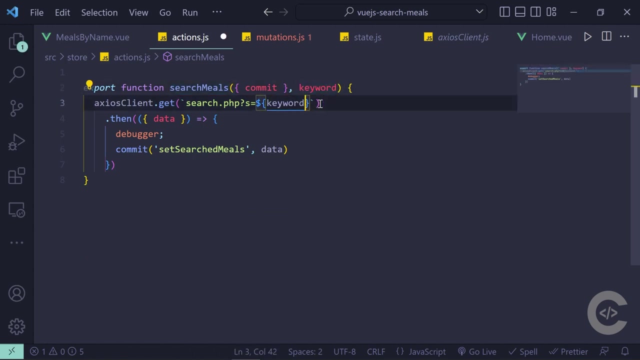 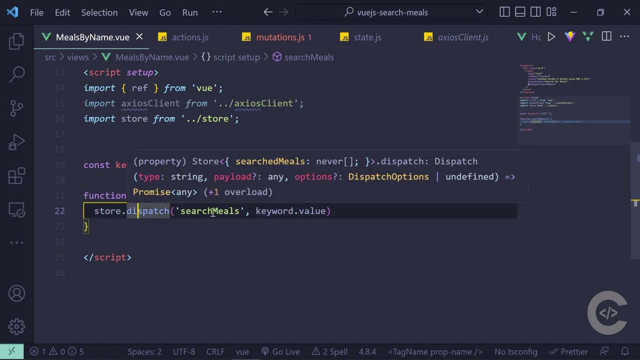 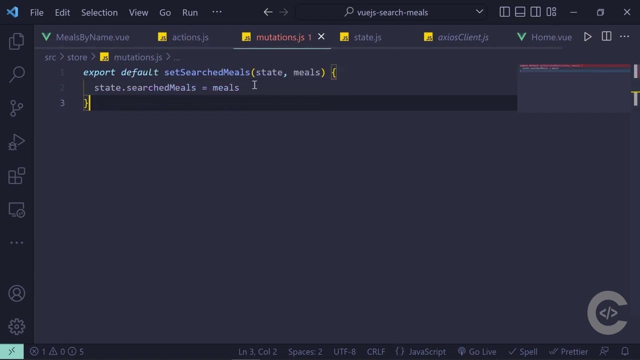 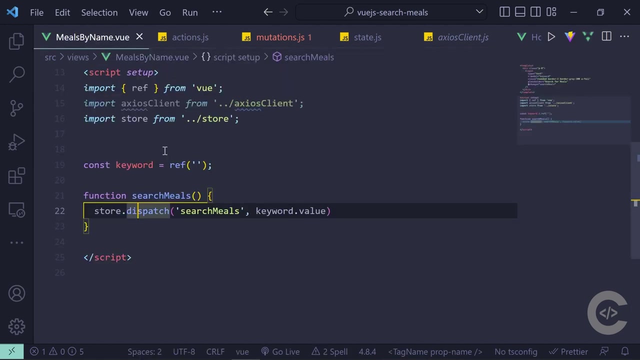 inside this store will be enough so i'm just going to change this into an array okay we have the search meals inside the store uh state now we go back in mutations and set state searched searched meals this is called searched meals searched meals equals given meals so now we have a mutation now we go back into actions and i'm going to call commit set set searched meals and i'm going to specify data right here and let's create debugger here as well to make sure that the data is what we want now we save this and now we go in the meals by name we have to call store and the store needs to be imported as well store.dispatch and dispatch will call our action so in this case the action is called search meals so we're dispatching search meals and we're going to pass the keyword the keyword will be keyword dot value all right and if we go in the actions i think we just need to accept a keyword without dot value and pass it like that like this okay we make requests we basically call action of the store then the store action makes requests to the server gets the data and calls the mutation mutation saves the data inside the store inside state and now we need to access the data using uh from the store state so i'm going to create right here const um const meals equals computed and we're going to return from here store state searched meals all right and if we 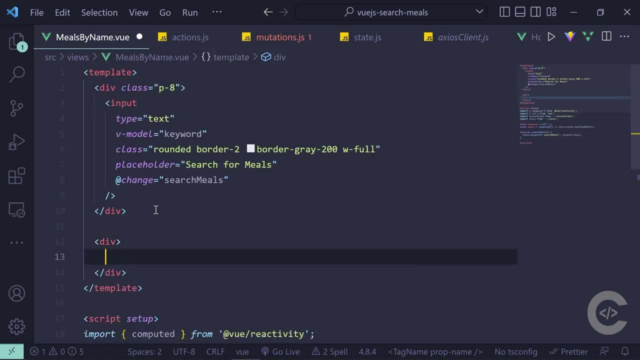 scroll up down and i'm going to create a div inside which i'm going to output searched meals 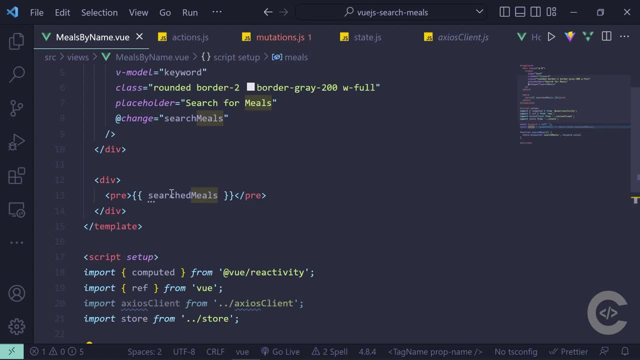 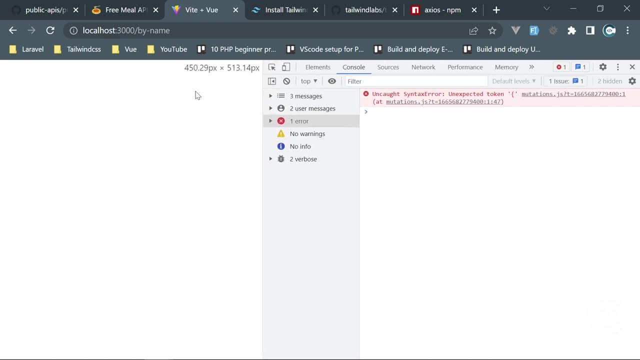 that's going to give me no we called it just meals and that's going to give me the searched meals let's have a look in the browser so we have by name and we have an error in the 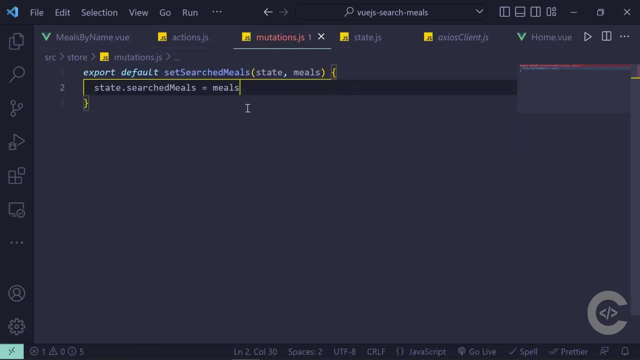 mutations let's go in the mutations export default i think function is missing right here export 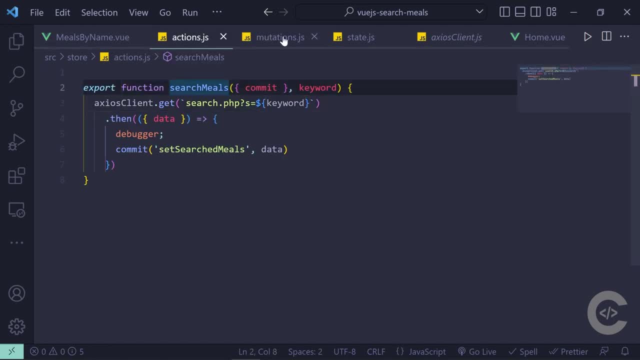 default function and that should not be default it should be just export function so we save this and 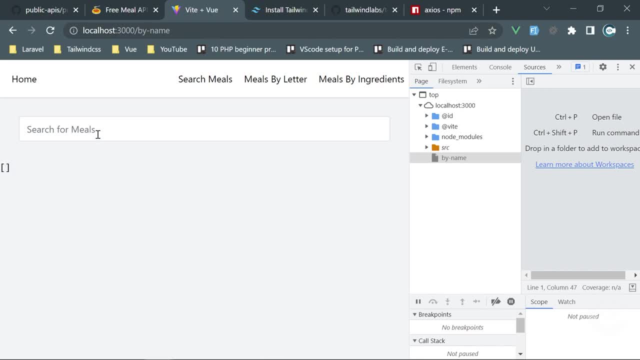 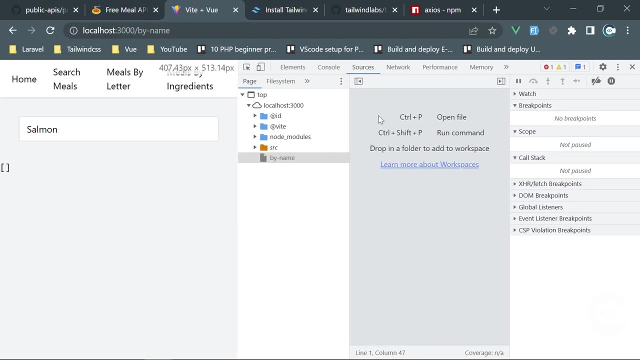 okay now we have meals to be an empty array okay let's search for salmon and whenever we click outside that's gonna make a request 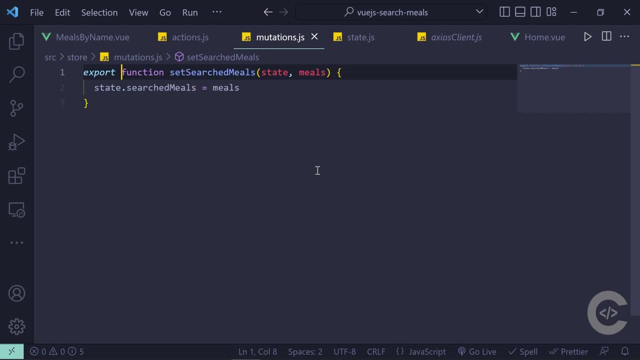 however we have an error access client is not defined well why it is not defined 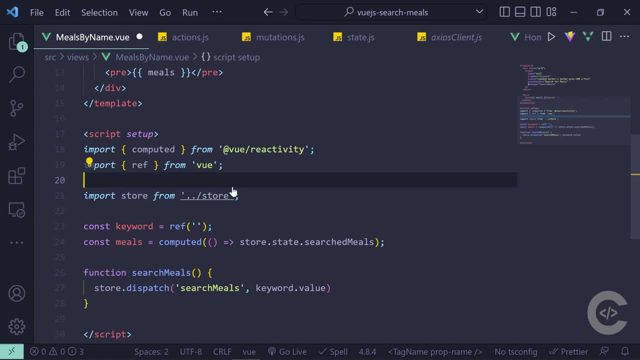 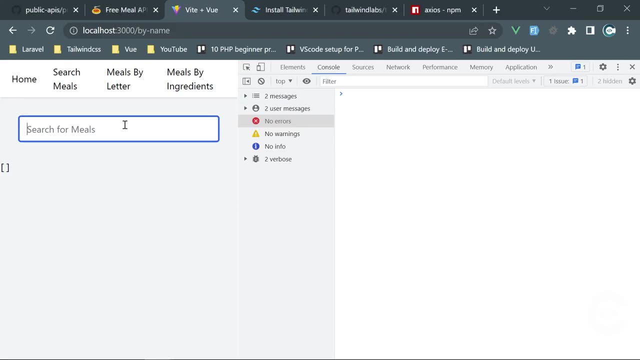 access client because we moved this access client into actions so if we go in the actions we have to import access client right here so i save this and now let's look for salmon 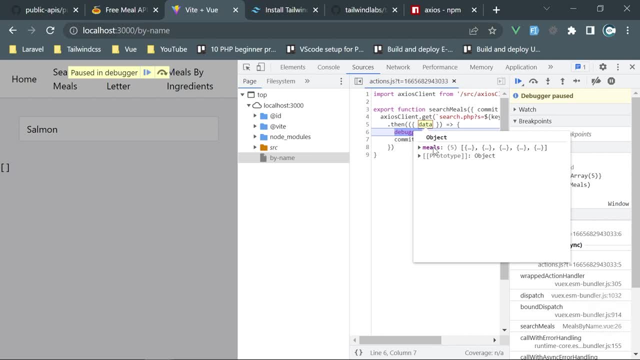 all right now the request was made and we have the data and we have five meals right there so the data actually contains 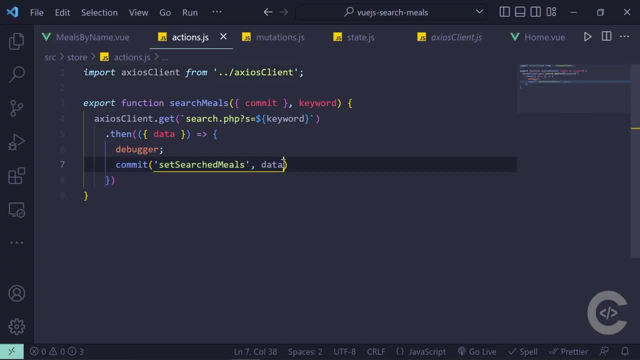 meals inside so we need to go in our project and access data.meals and pass it to the mutation 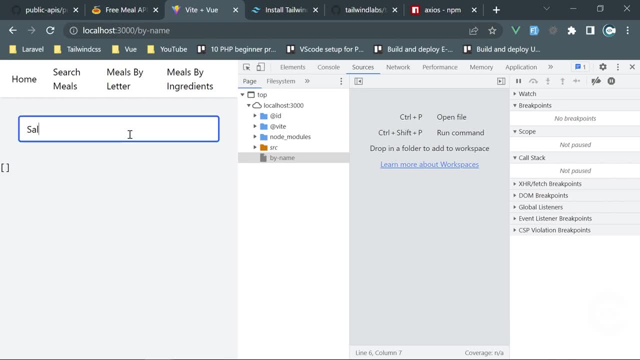 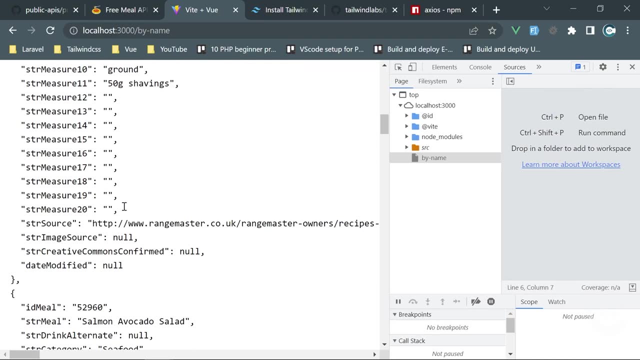 all right and now if i just reload the page and search for salman again and we see right here all the data about that specific meal we have five meals and we have 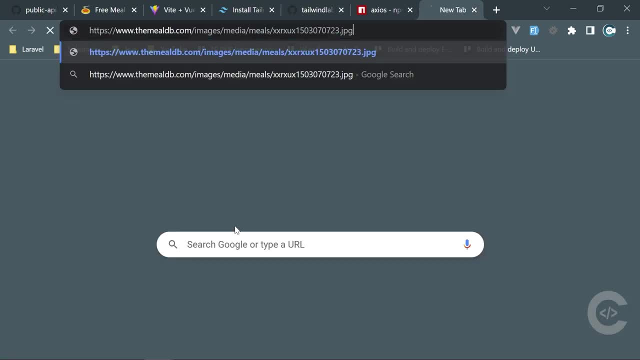 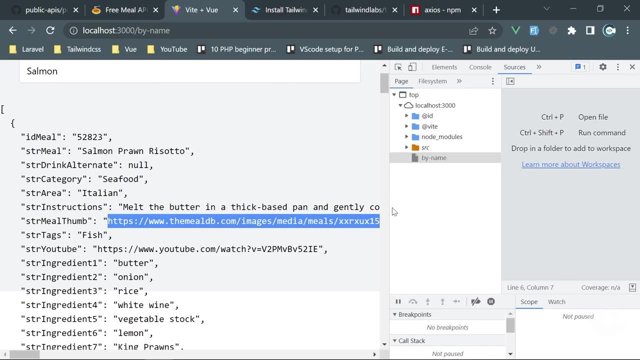 also i think thumbnail for that meal that's excellent oh great so now let's display this 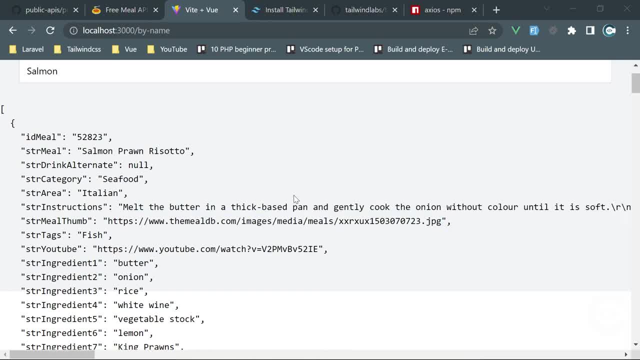 information in the component right so i'm going to collapse this and let's go in the meals by name 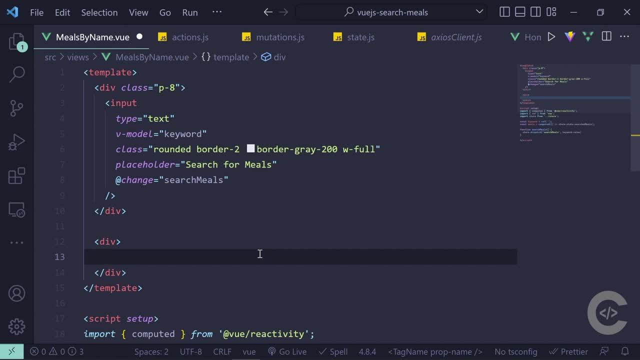 and let's remove this pre and we will need div we will need a v4 meal of meals 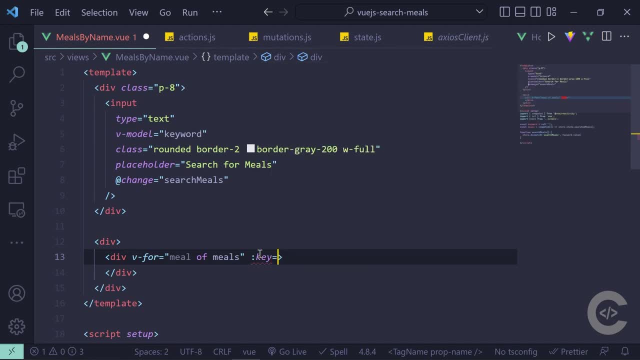 let's give this one also key equals meal.id i think no it has id meal let's give it id meal inside there we are going to display first image and let's give it source which will be meal dot source meal thumb source meal thumb okay we have that 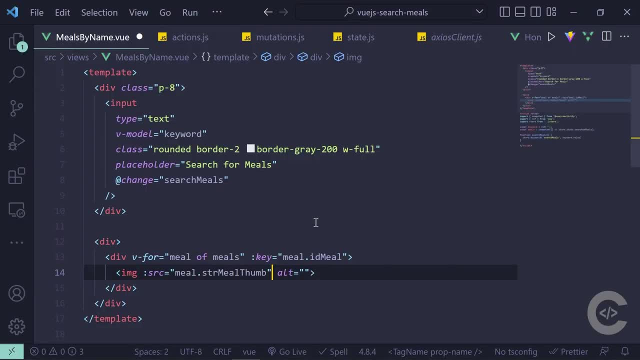 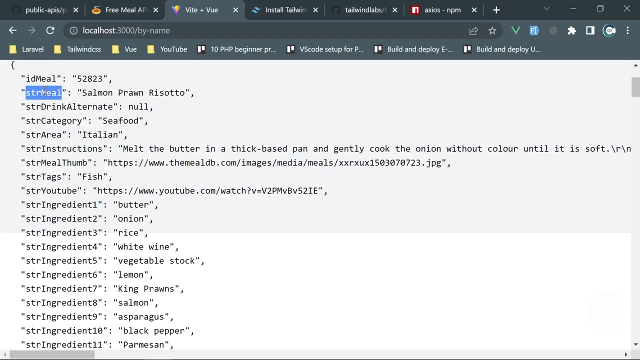 specify alt as well which will be str meal let's give it like this down below we're gonna have like a title inside probably h3 we're gonna have meal dot meal dot what str meal probably down below we probably i have a like a one sentence instruction if there's something like this no there's no one 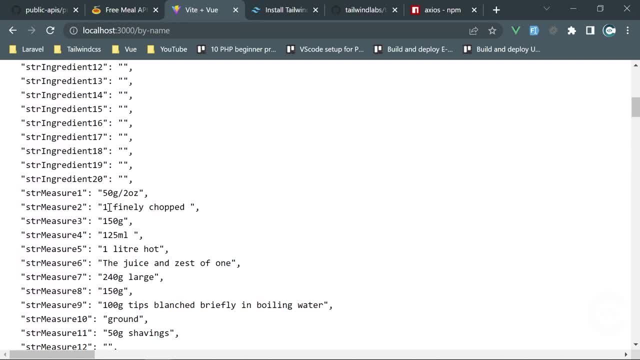 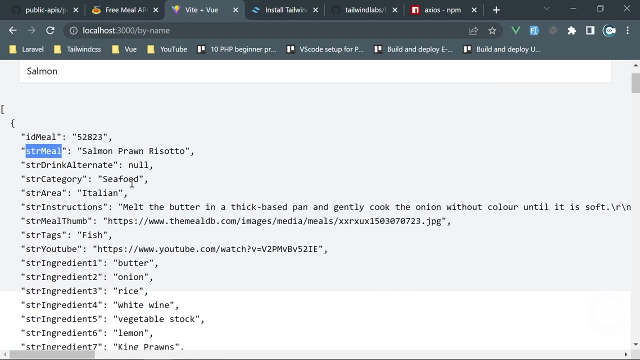 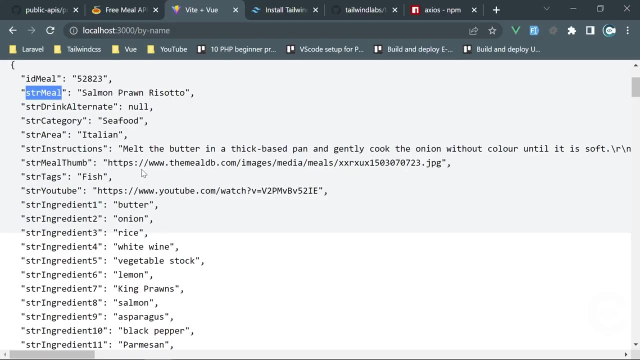 sentence instruction we have all the ingredients measures source okay what information can we have down below i think there is nothing we can put okay let's create div okay let's create div 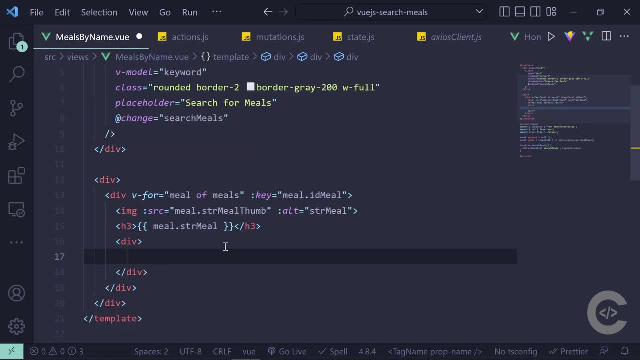 instead of paragraph and inside there we are going to put right there two buttons 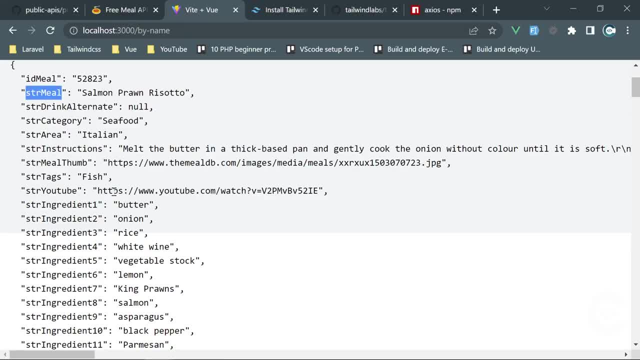 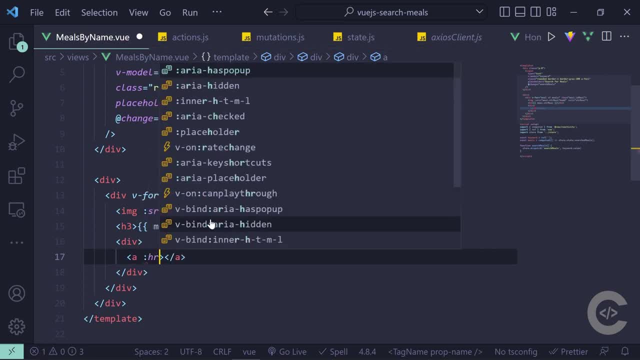 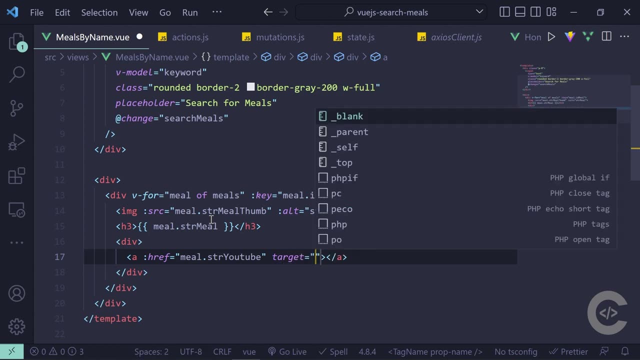 the first button will link to youtube so we have str youtube as well so that should probably be an a with href to meal dot str youtube and let's give it also target underscore blank and here we need 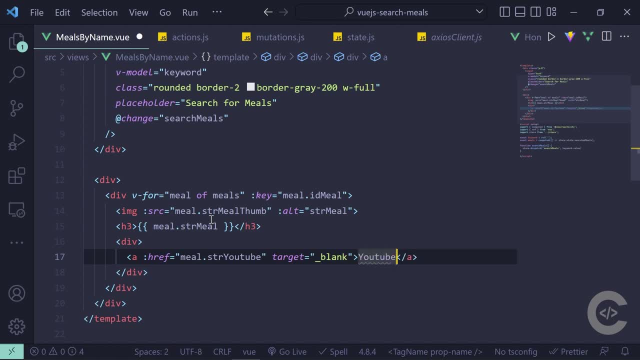 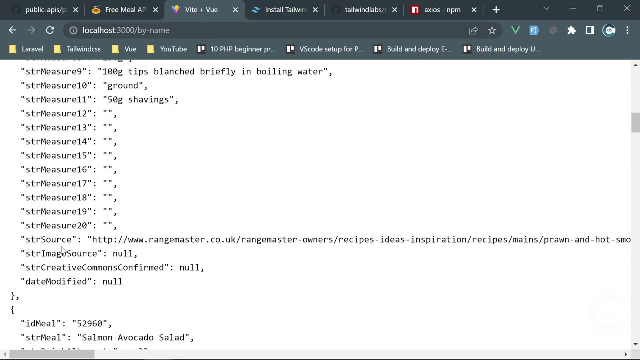 output probably just just youtube youtube and the second will be for the actual source maybe 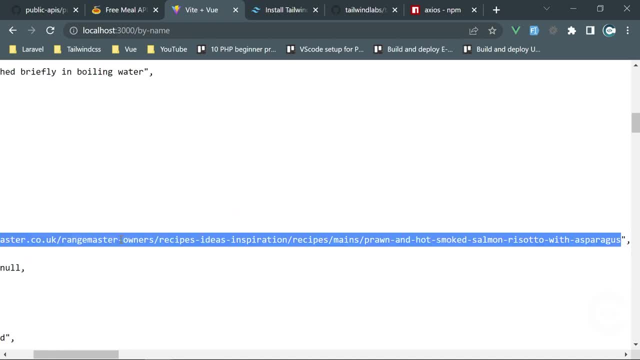 so that's that is probably some kind of original source all right if we just check that 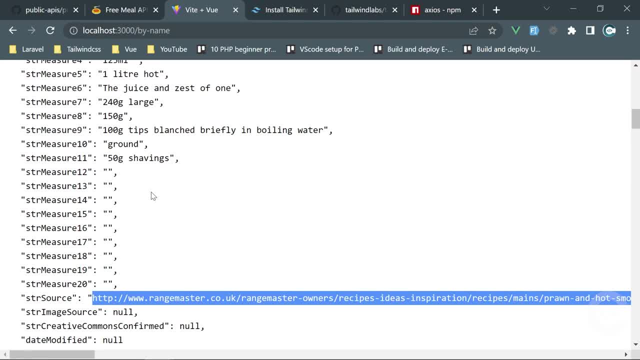 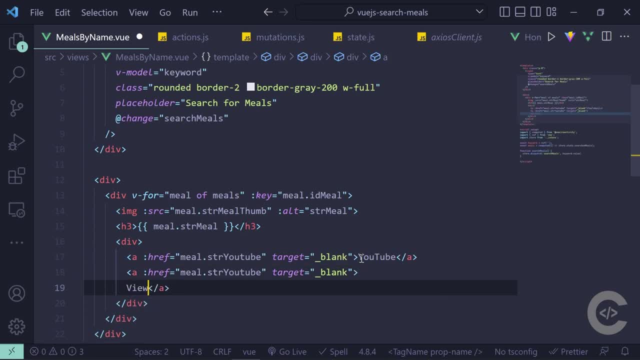 yep it doesn't seem to be working okay let's put it here oh no that's within this environment so we can closer look at the~~ 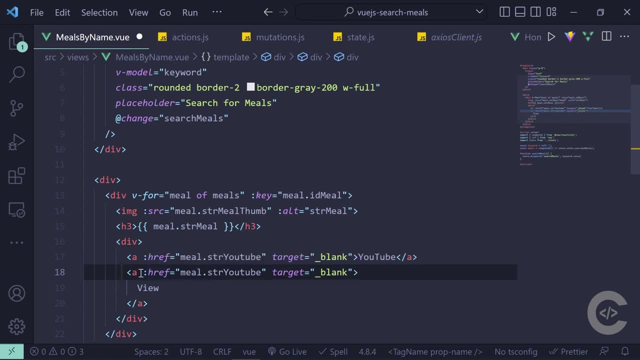 100 viewer well that won't work 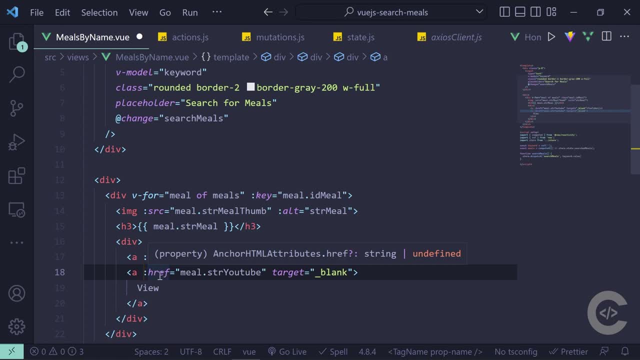 so let's say we're going for meallit iting link let's go detail page ready yet so we're going to create that later but for now let's just specify it 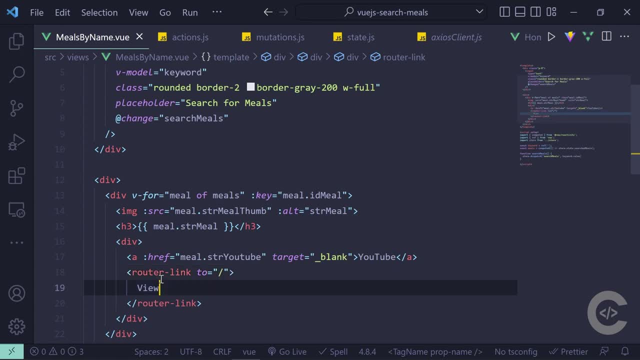 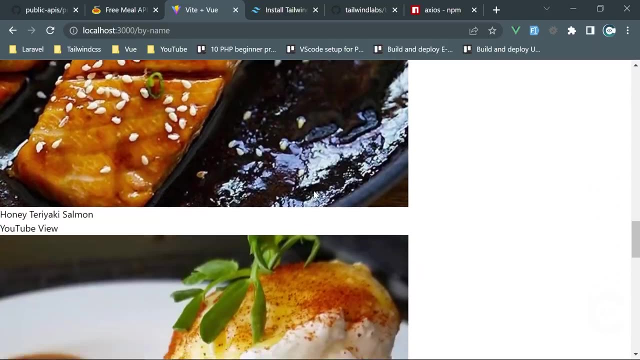 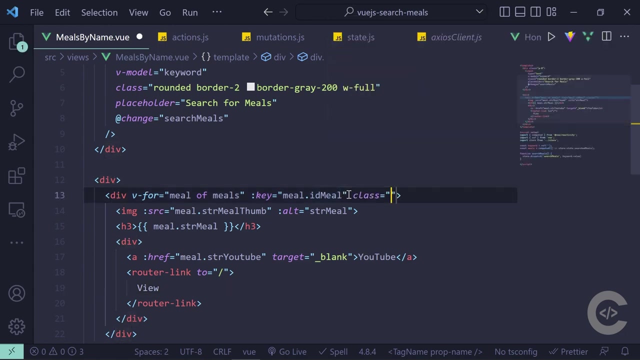 again to slash all right and we have view so I saved that and this is our page however we need to adjust it okay I'm going to give this one class grid and that's going to be grid um 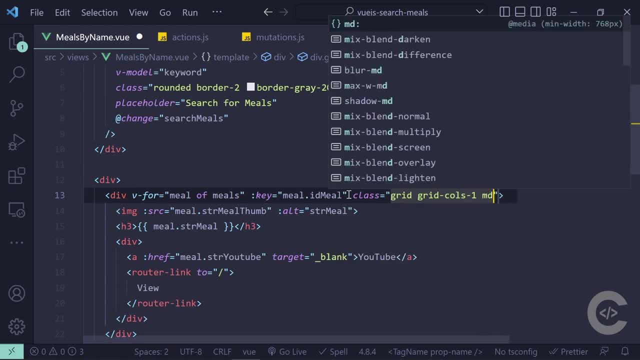 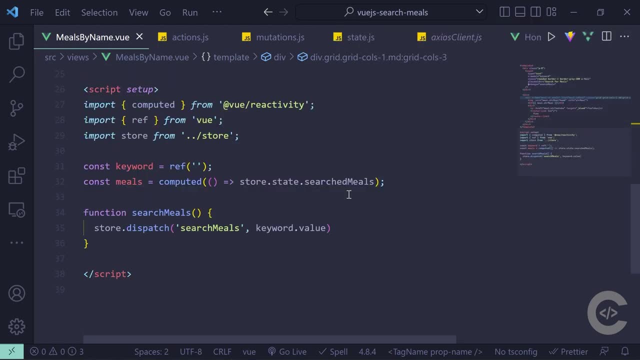 grid calls one but on medium we're gonna have grid calls three medium and above okay now let's see what do we have there 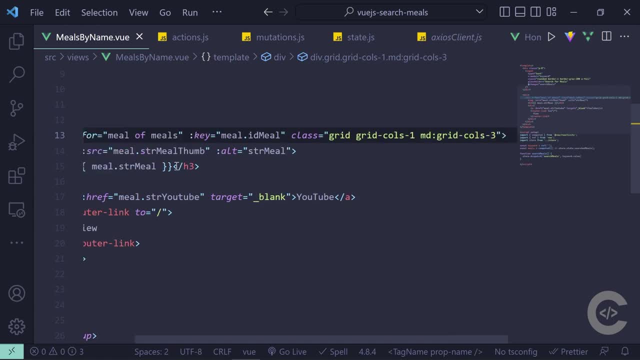 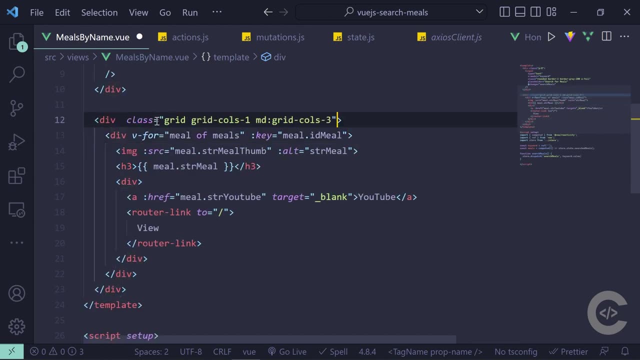 grid calls one grid calls three no I gave it to the wrong element this should be given to parent like this okay let's give this one also gap uh gap three 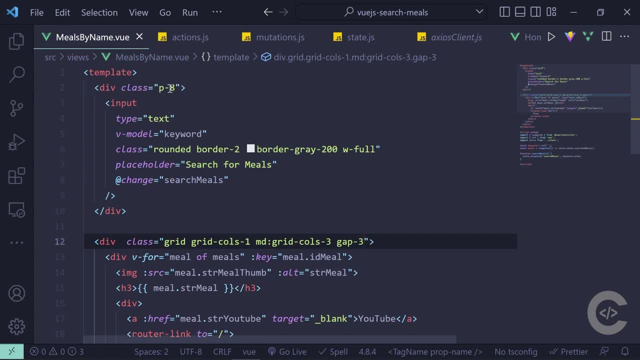 this is good uh we have that input with padding so probably we should give this one padding as well padding 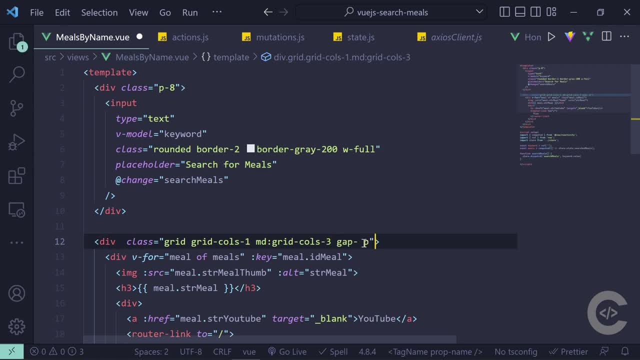 excuse me so gap three and padding eight okay I want to increase gap maybe up to five 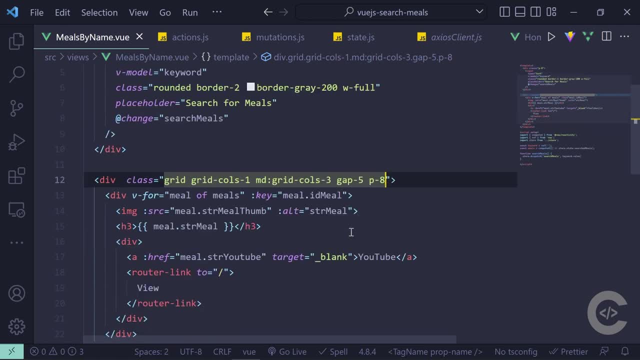 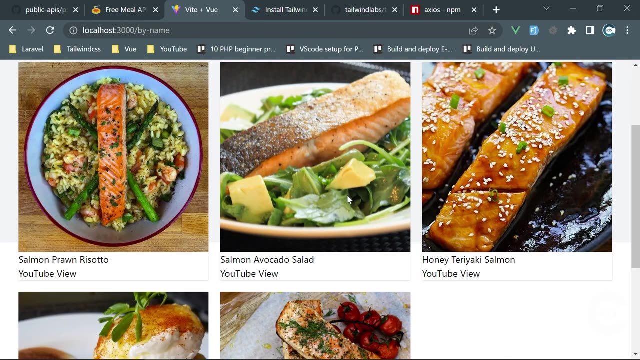 okay this is good now let's give each individual meal plus BG white and shadow okay 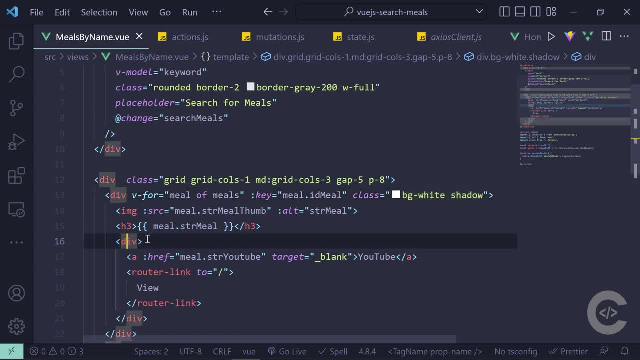 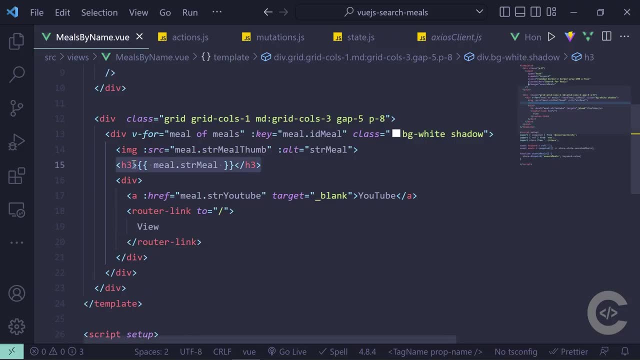 um okay this is the title we have image then title and then we have buttons okay let's give this title and the buttons uh padding x3 and padding y adding y2 see how that looks like 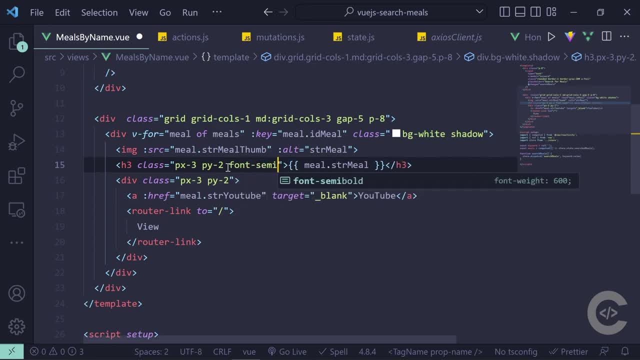 let's give this h3 as well font semi-bold this looks nice however padding should be increased let's give it padding 3 totally all right so we have that 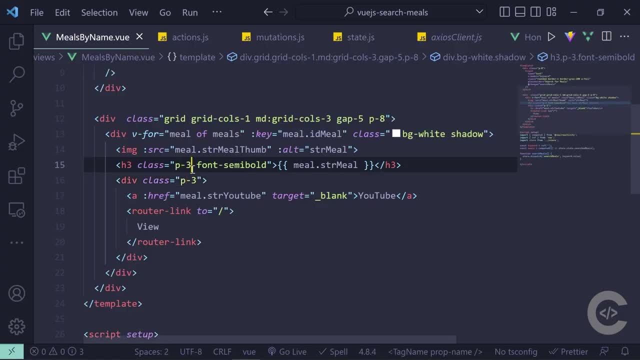 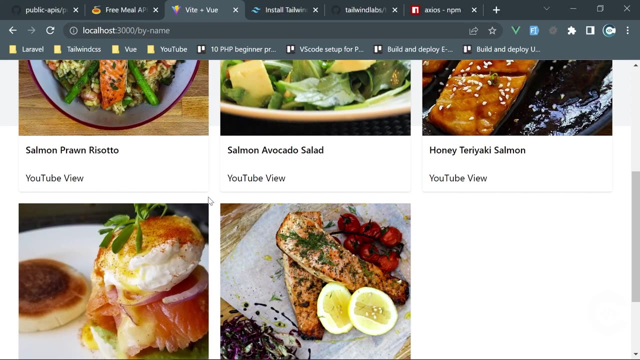 this looks nice but I want to make it even better so let's give this one rounded now we should have rounded corners 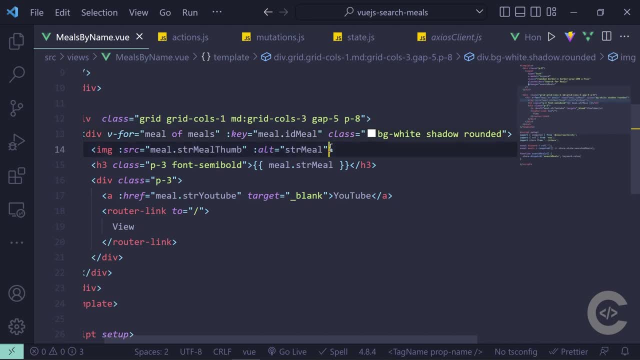 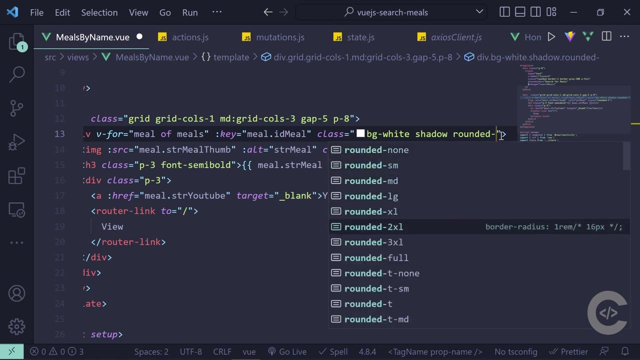 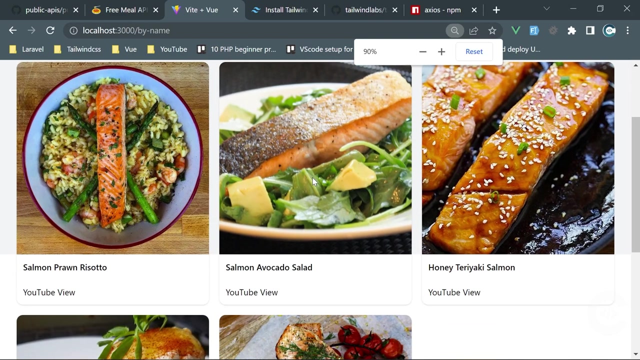 but the image is not rounded so on the image I'm going to give it rounded rounded top and let's increase this into rounded rounded LG maybe or rounded Excel and let's change this rounded T into rounded T X Excel as well okay here we have so the images basically are very nice very nice 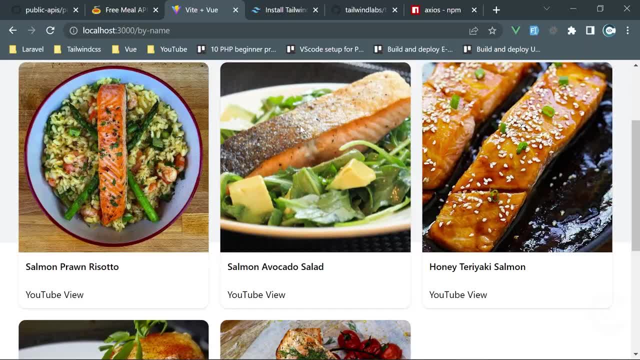 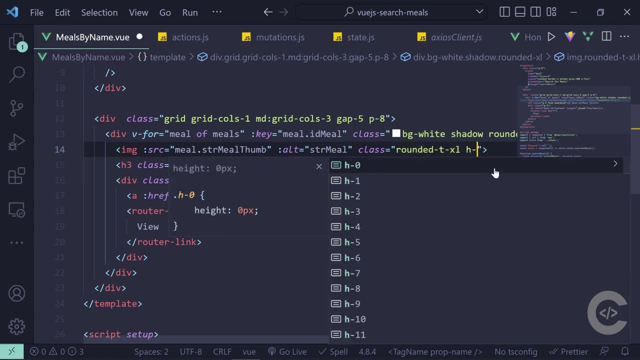 but they are I think very large in hate if we can reduce them in hate that's going to be good so if we just give them hate of 24 maybe let's see how that works 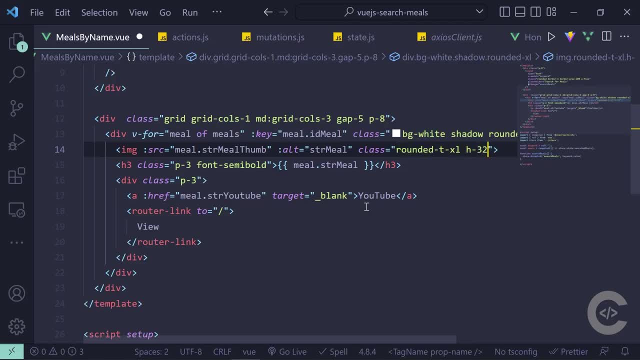 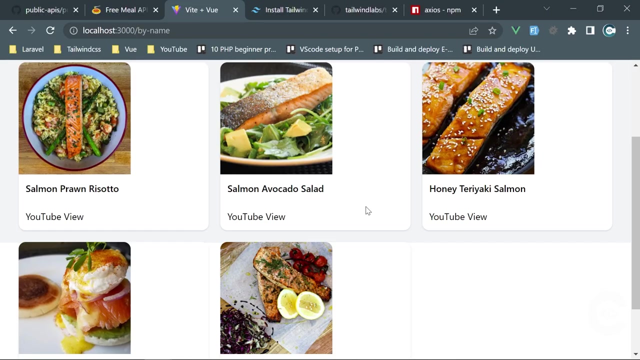 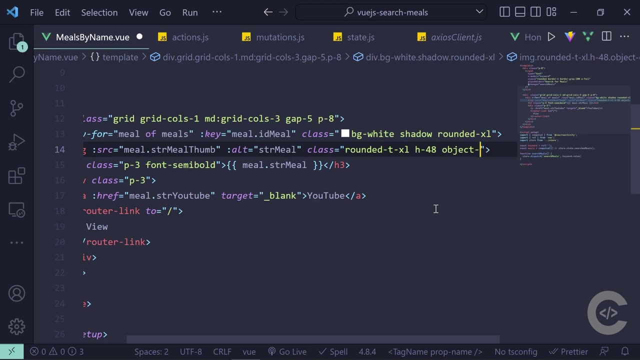 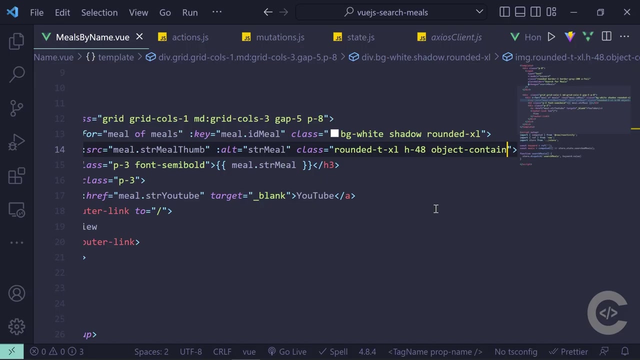 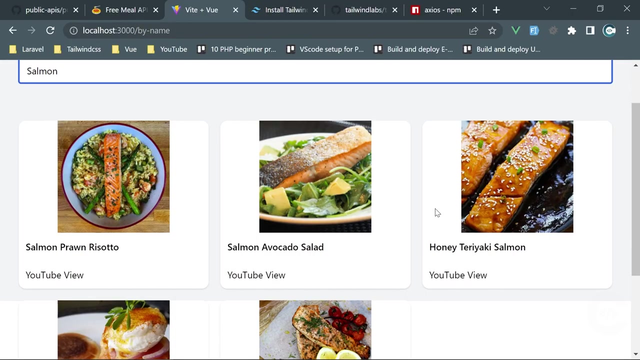 looks like this too small hate of 32 48 let's do like this but we need to give this image also object cover let's see Salman okay object cover doesn't do what we want object contain object fill we need to give it like full width W full probably and then object contain no object 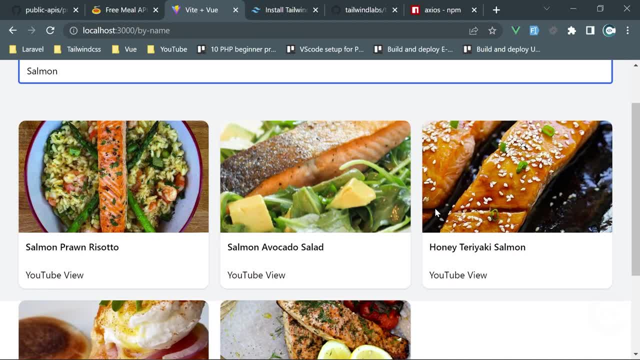 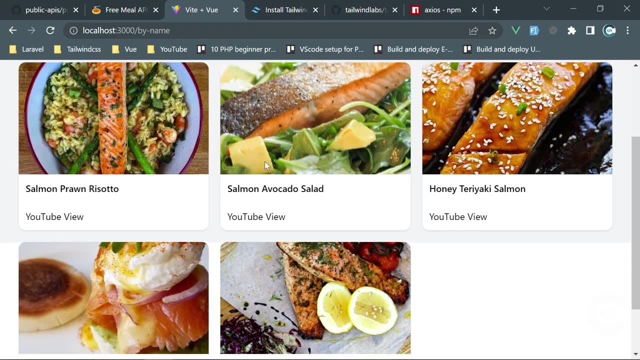 cover okay this is what I wanted okay so we have much smaller width now I think this is much better and if we just 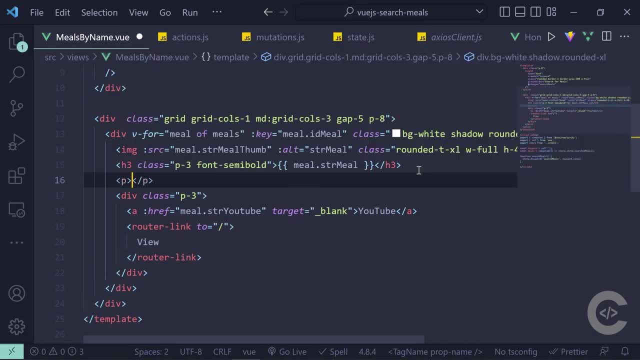 just put a dummy paragraph right there just to see how that looks like because I want to make it also really nice well you know what I'm going to put everything in a div because that's going 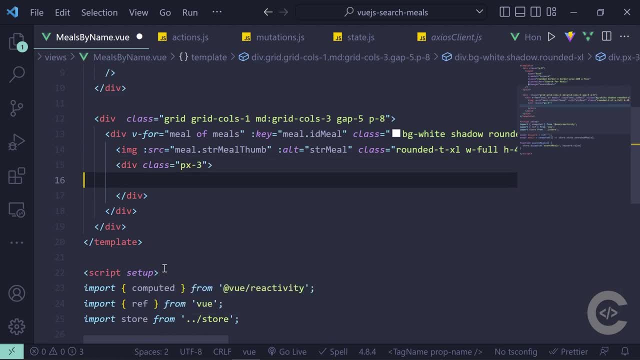 to be a description side so padding of three and paste everything let's reduce this size not that 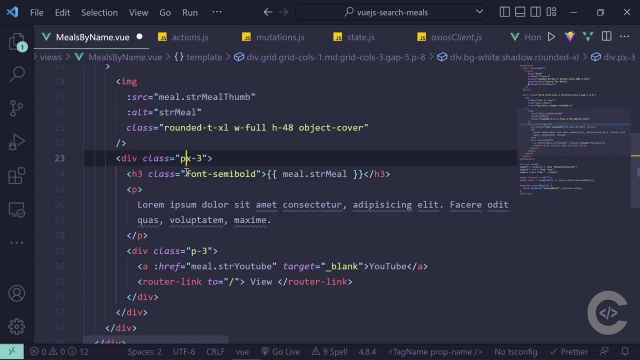 much and let's remove padding from here and from here here as well 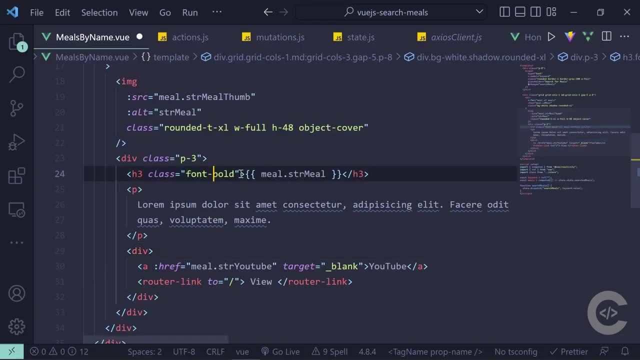 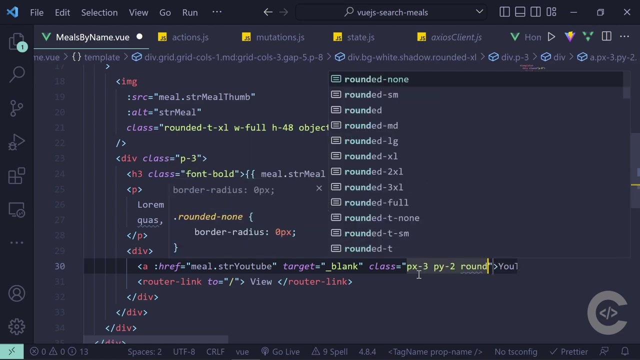 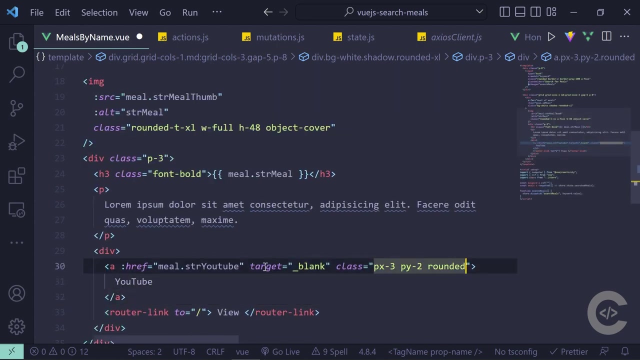 I think this is great let's make it a font bold and we have the description and now let's give some styles to this YouTube button so that's going to be button so let's give it padding x3 padding y2 let's give it a rounded and let's give it also 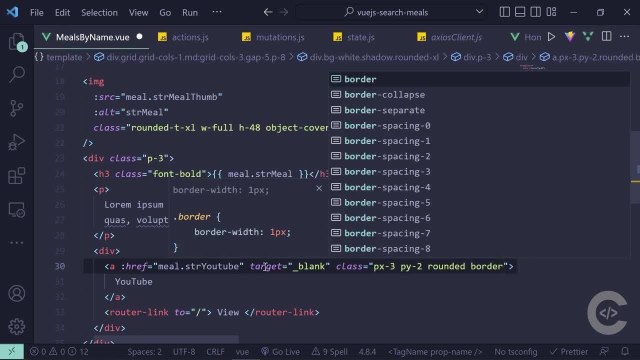 border I'm going to make it outline button so we need border and we need order red um border red 600 probably 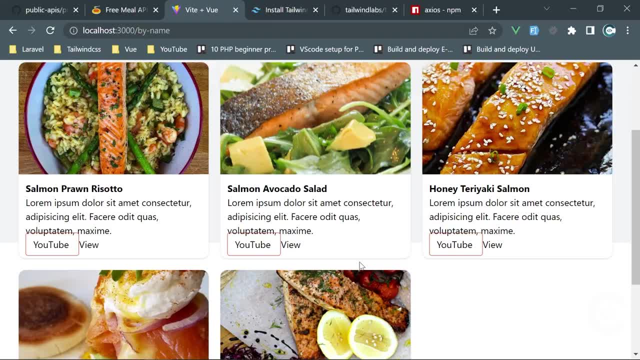 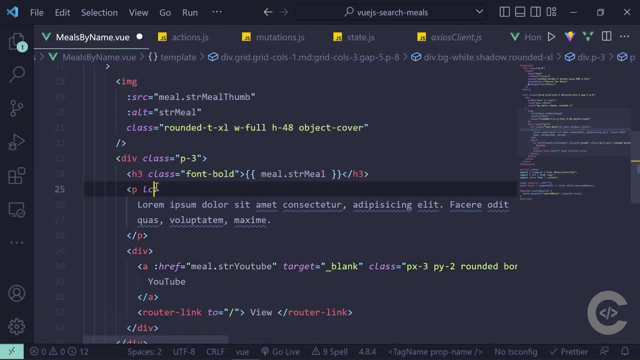 okay however the text is above button so let's give this margin button four okay we have this YouTube button let's give it border two and on mouse over 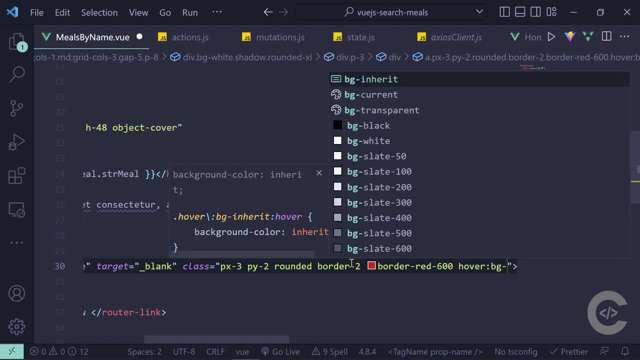 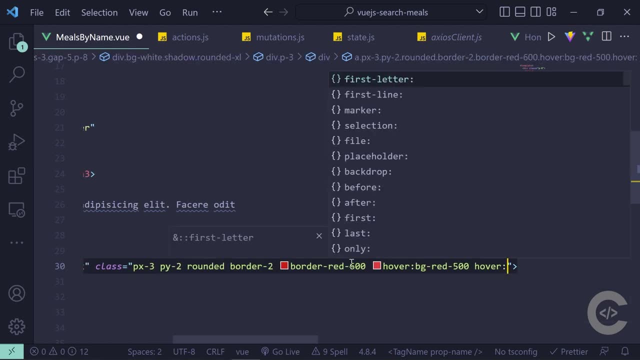 on hover we're going to give it PG uh PG gray uh sorry PG red 500 and on hover we're going to also give text white so we save that and we see this YouTube button and we can give it transition as way and we see this YouTube button and we can give it transition as well and that's the end of this video thank you so much for watching and if you enjoyed this video please like and subscribe to our channel and don't forget to activate the bell icon so you don't miss the next video it's the vendetta it's the next video I'm going to end this video so until the next video see you in the next video bye-bye bye-bye transition on colors 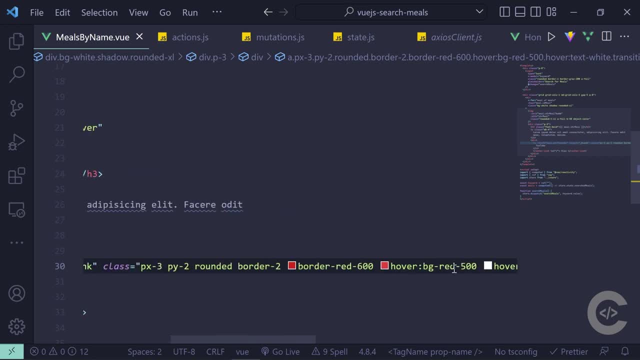 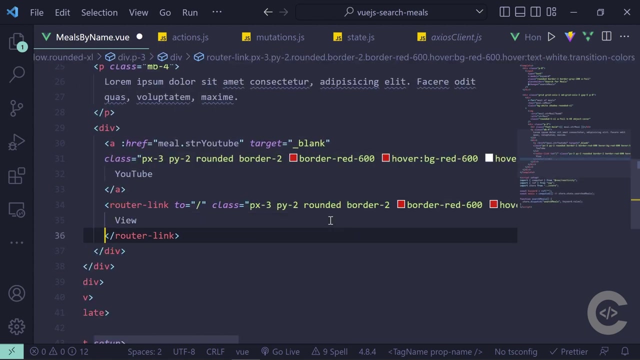 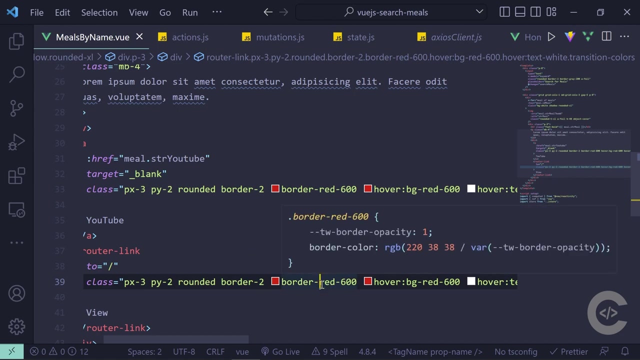 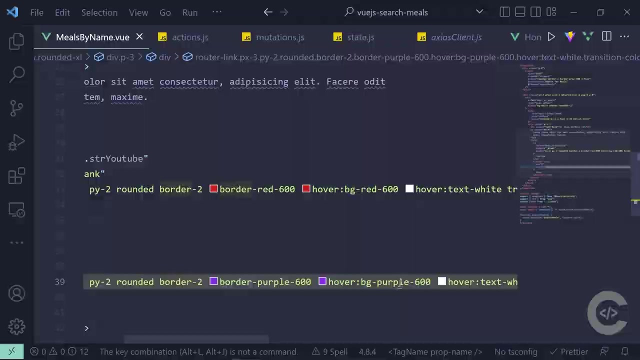 this looks good we have let's change this into 600 as well okay and let's create this let's give something similar but different colors to this view button and let's paste them right there and let's move them on the next line and we will need let's format the code and we will need instead of red let's give it let's give it um maybe purple purple 600 well i'm going to give it you know what i don't want this outline style so i'm going to remove this we are going to have border 2 we are going to have pg red 500 on hover we are going to have bg red 600 and let's see 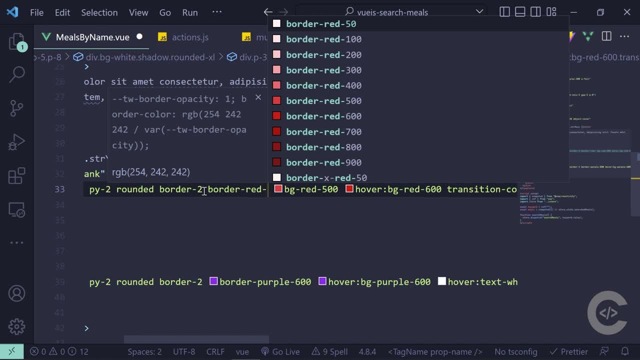 and we're going to have also border red uh 600 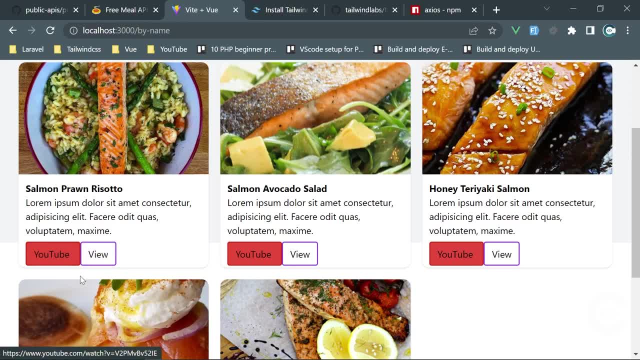 and of course we need text white 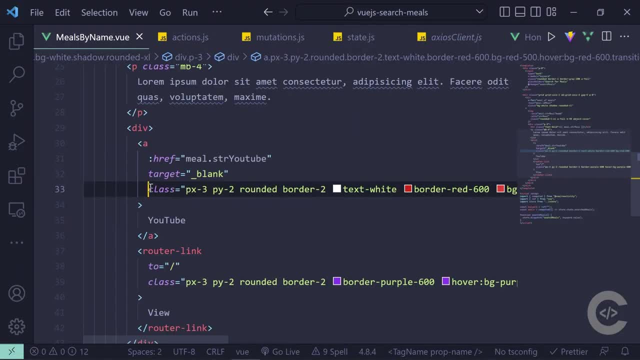 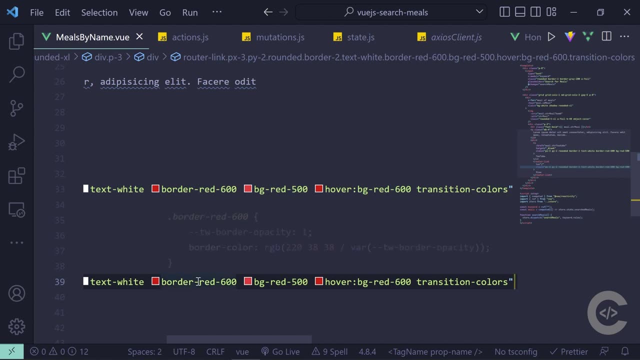 okay and let's do something similar for the below button so i'm going to replace this part but let's look for all red and change that into purple and let's 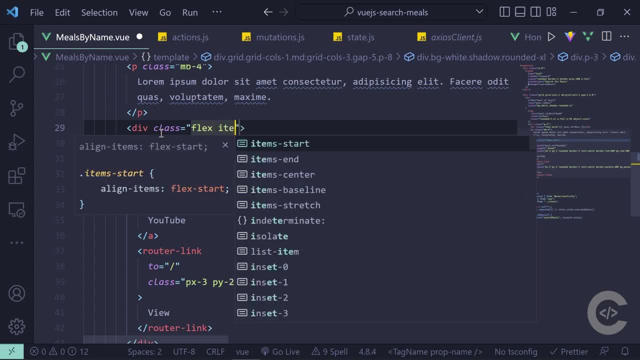 let's give this parent lex items center justify between 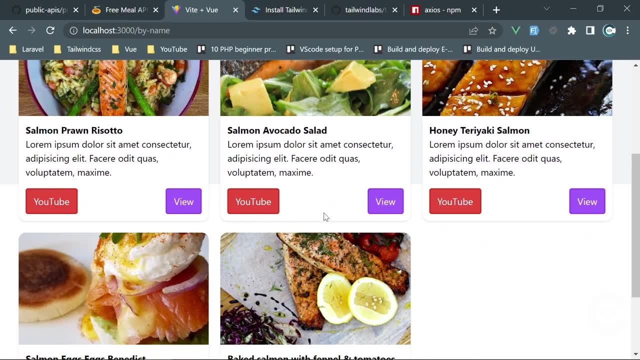 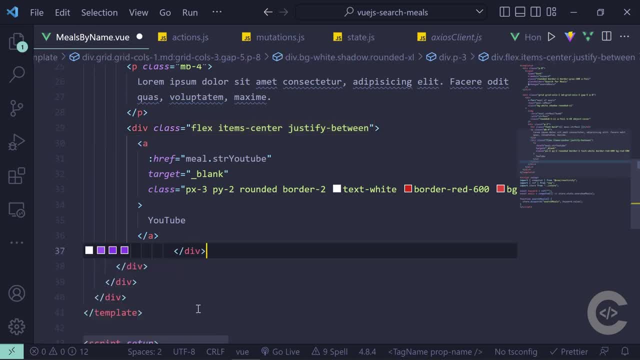 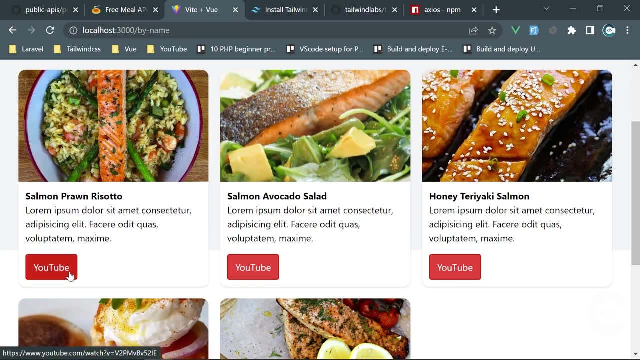 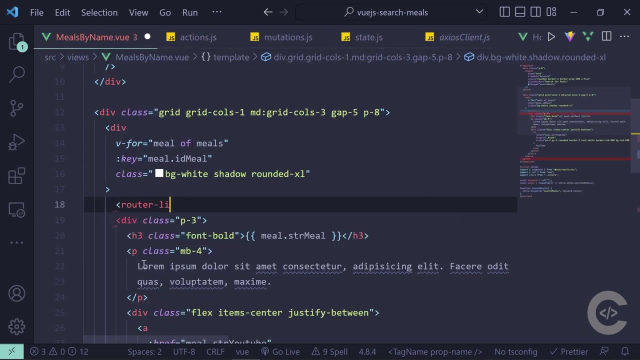 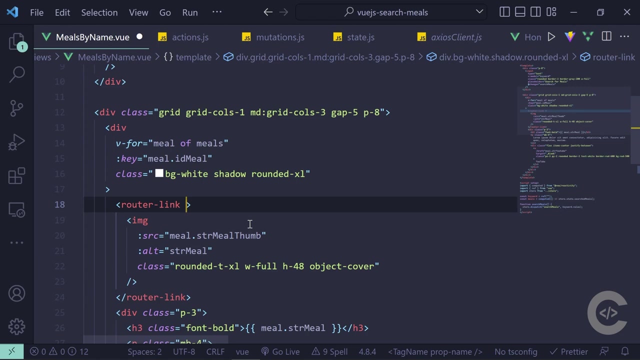 okay so we have those buttons however maybe not super nice especially this purple one i don't like i decided to completely remove that and whenever i click on this image it's going to open the details page and we just have the youtube link we just have the youtube link which is fantastic but i'm not going to use it too much um let's change it a little and funny that matters i also noticed that the images are certifying theisaite is turning red i know like, which I think is fine. The best one will be to have a YouTube icon as well, but I'm not going to spend more time on this. So let's take this image, and we're going to wrap this inside router link, and we need to create the page for the meal. We're going to do that, but for now, let's just give it slash again and observe this page. 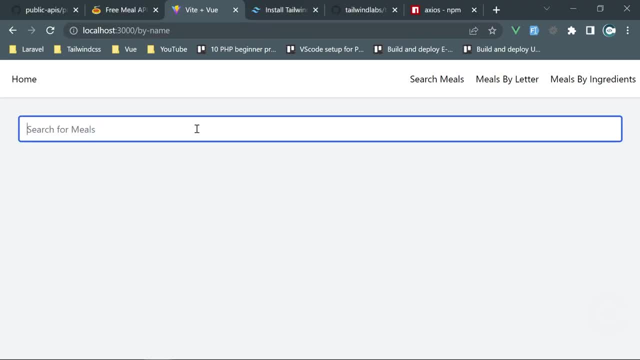 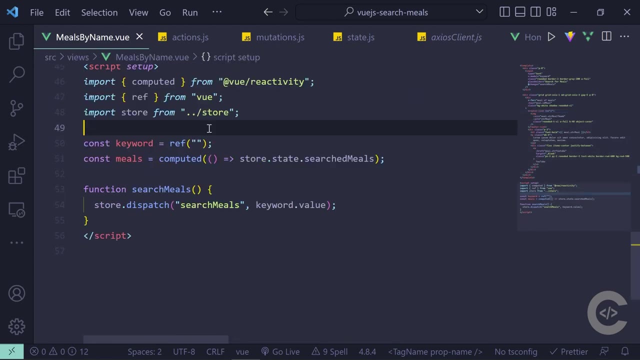 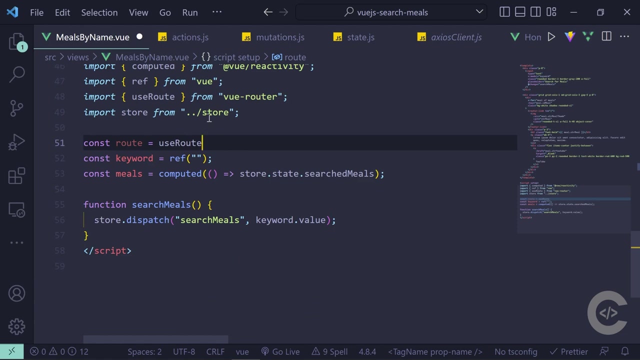 By the way, whenever we search something, I want to save this in the URL, because when I refresh the page, I want to take that and just reapply it. Okay, so let's do this. I'm going to scroll down below, and I want to take the current route. So const route equals use route. Okay, and that use route was imported from your router. So we use the route, 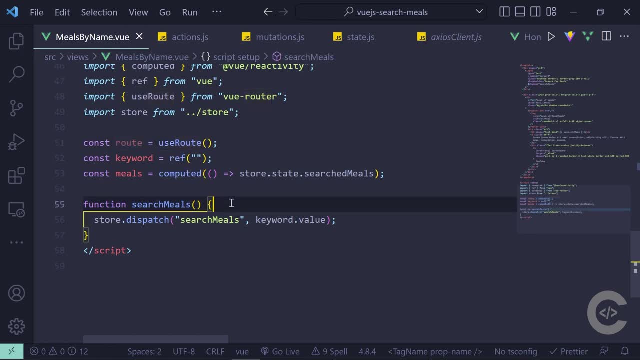 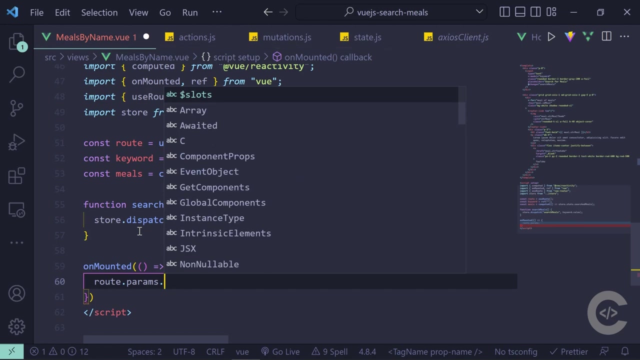 and that route basically will contain, it might contain in the URL, the keyword. So what do we do here is that on mounted, let's create on mounted. Whenever component is mounted, we take route.params, and it might have, what is the name of the param? Let's open router, 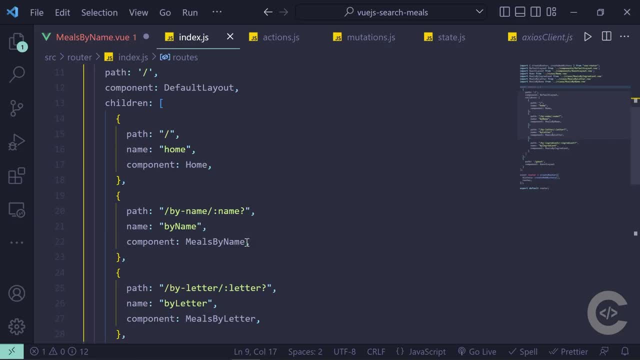 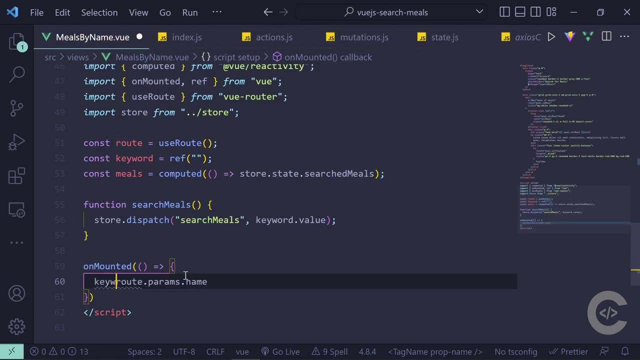 and we have right there, by name, and the param name is called just name. So we take route.param name, and we're going to assign this into keyword dot value. Okay, in this case, we're going to have 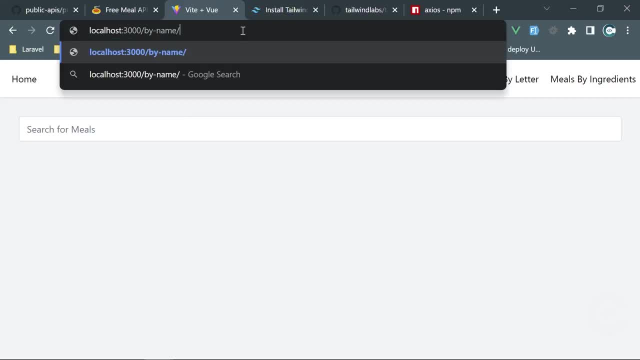 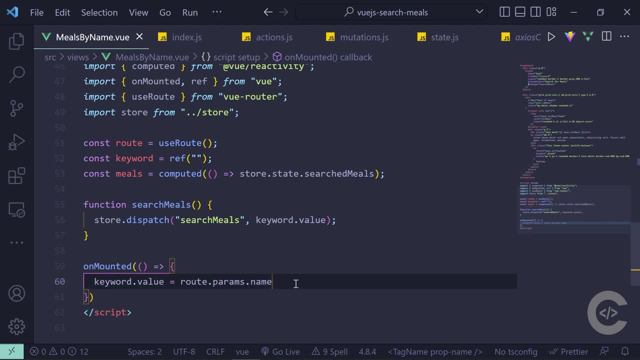 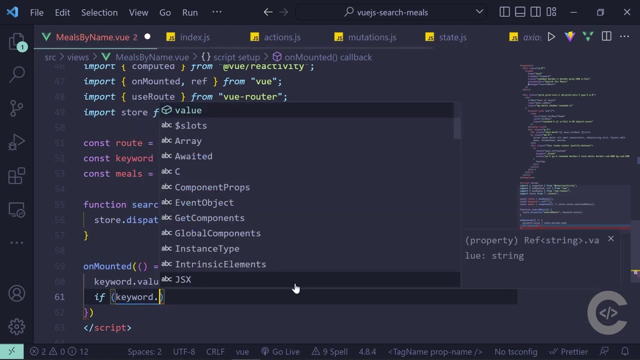 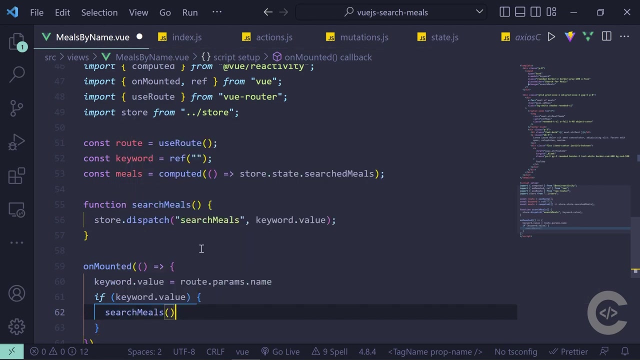 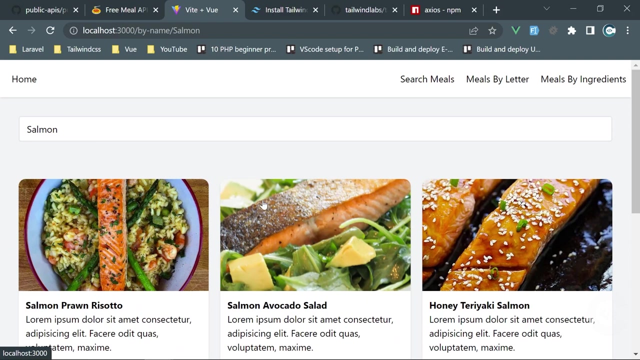 two-way data binding. And if I just type salmon right here and hit the enter, we see salmon right here as well, and we're going to also make query to get salmons. So how do we do that? If keyword value exists after it was mounted, then we're going to call search meals. Okay, so if you just reload the page, we see those salmon meals. And clicking on this opens YouTube 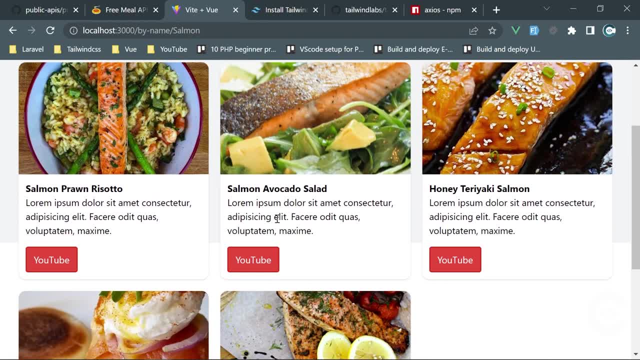 channel, and clicking on this should open the inner page. All right, this is looking really good. 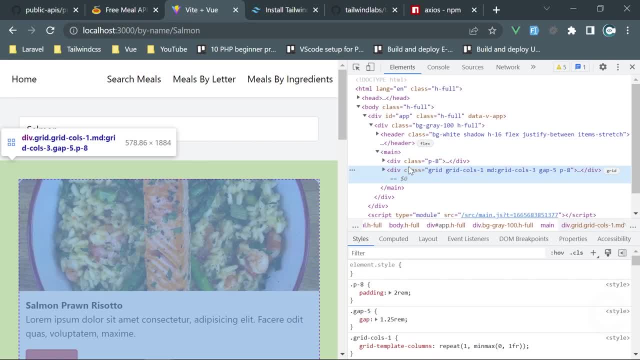 Let's inspect it for some final tweaks. This one doesn't need padding button. So let's scroll up, 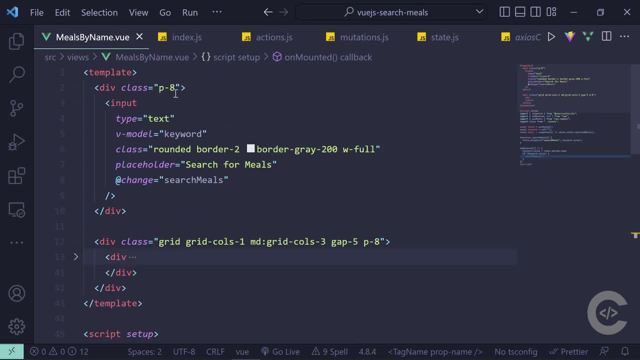 and let's disable. So this one should not have padding button. So padding button zero. 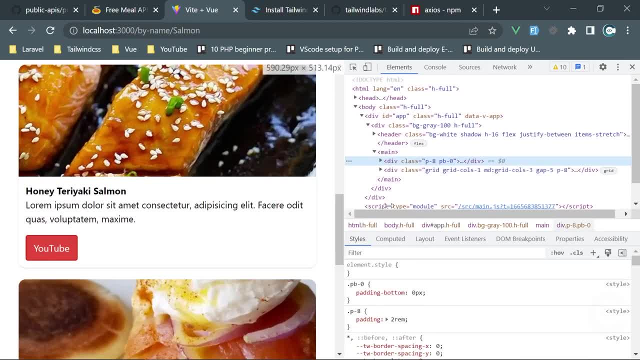 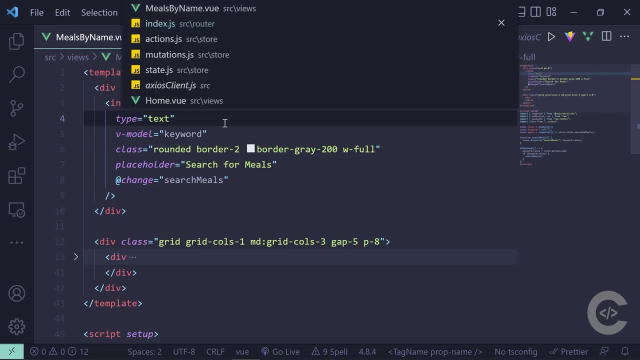 That's more like it. And we have also it responsive. Okay, and because we, we did it, we thought about that. Now let's implement the meal inner page, we go in the router. And down 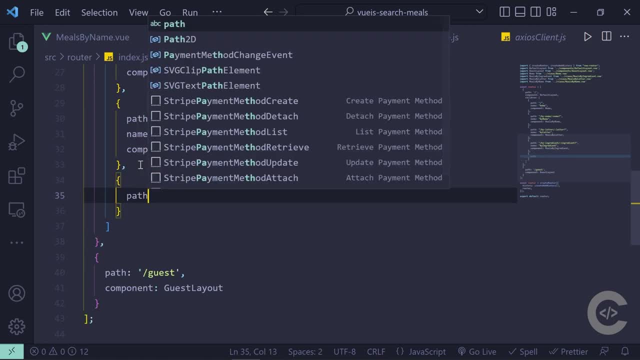 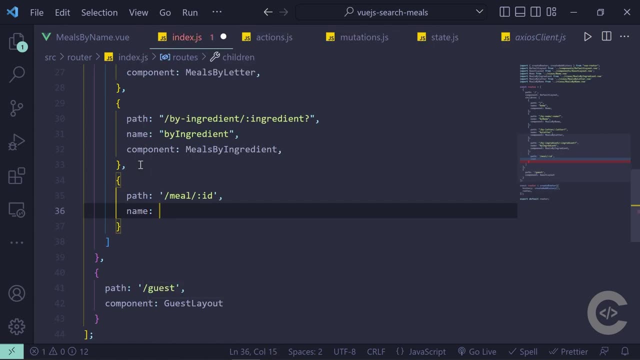 below, let's create another path. That's going to be meal slash and ID. And we're going to have name right here, it's going to be meal details. And we're going to have component right here. That's going to be 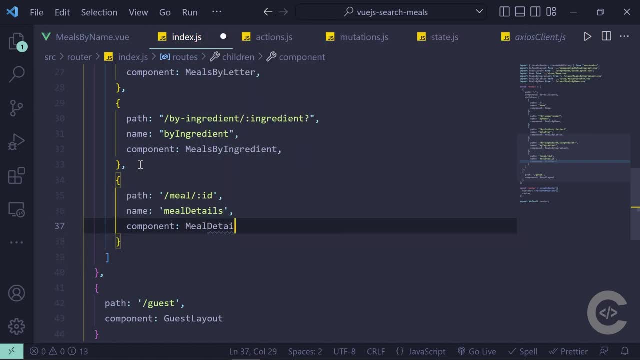 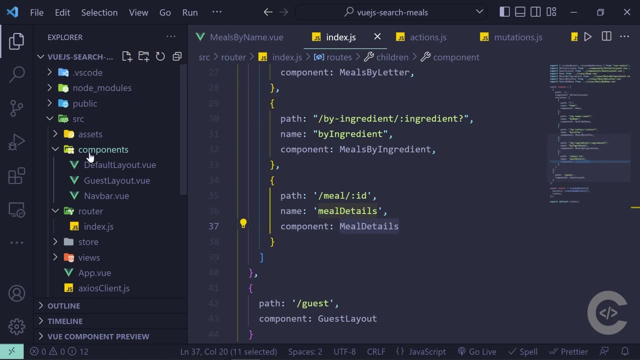 how should i call it meal details probably meal details all right so we go in the components and no i'm going to go in the views and create new component dot view 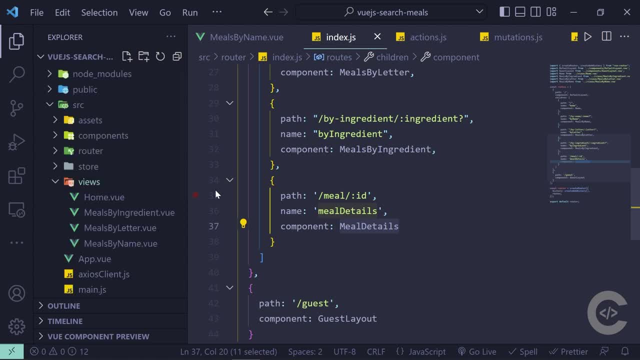 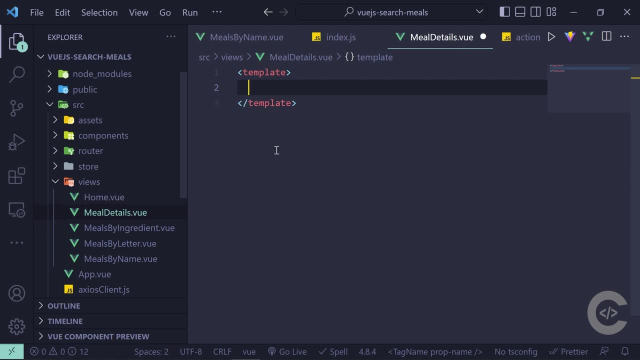 it's 2 a.m midnight right here and maybe i'm a little bit tired so template it we go in the meal details so now let's create script right here as well we need that 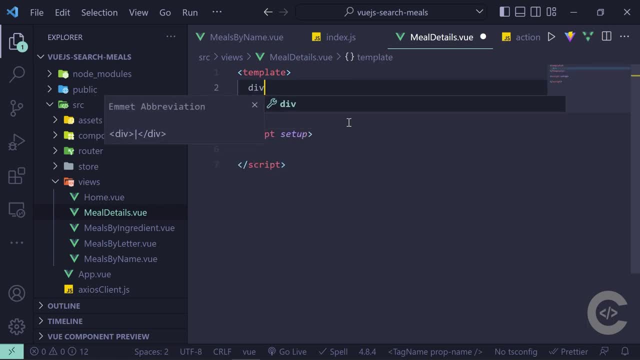 with setup and for meal details let's define div we are going to create a main cover image for the meal and then details and description and everything okay so let's create an image but we don't have information about the meal yet 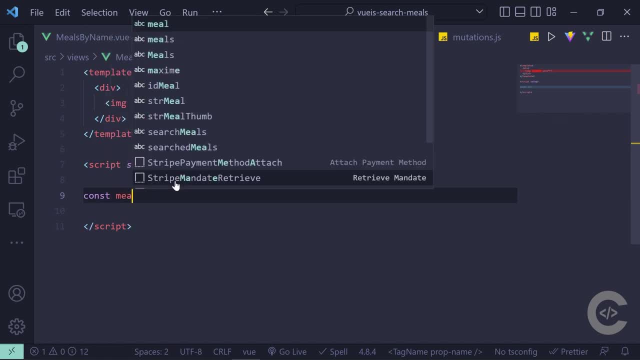 okay so let's define right here const meal that's going to be a reference to by default it's going 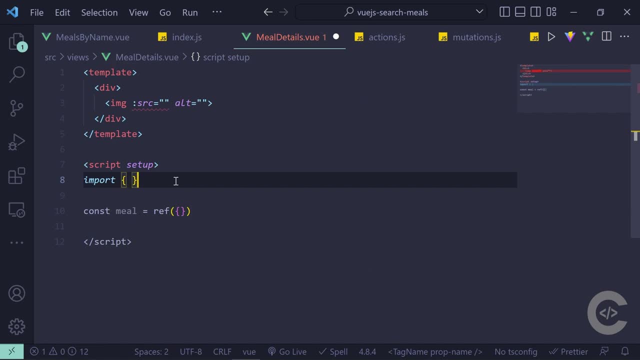 to be an empty object and we have to import from view we have to import ref from view now we have meal and we're going to access meal dot source okay i forgot what was the actual name so let's just print entire meal 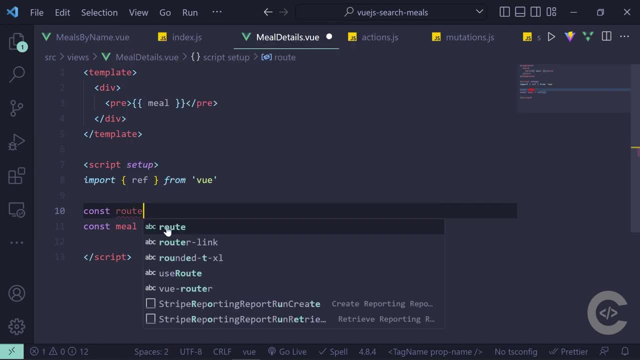 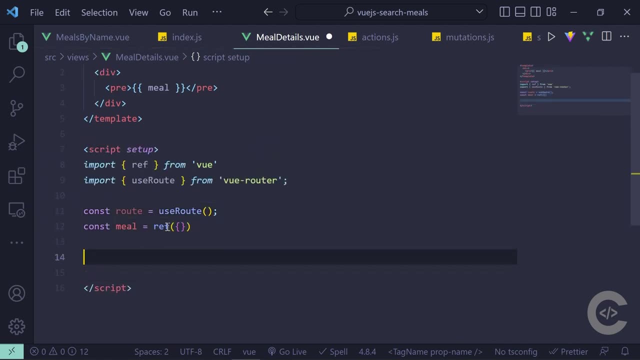 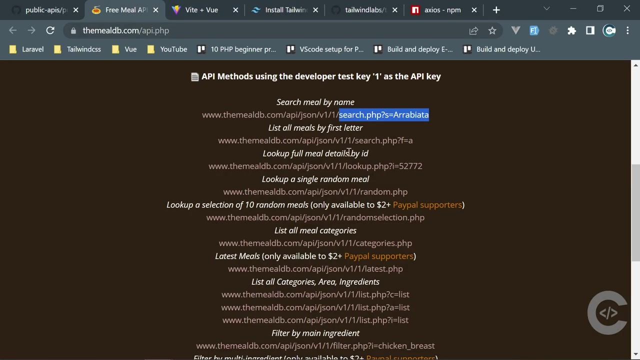 but we are going to take current route as well wrote equals use wrote all right and then unmounted we are going to take wrote params dot id and we're gonna fetch the meal details and the end point is called to list all meals by first letter 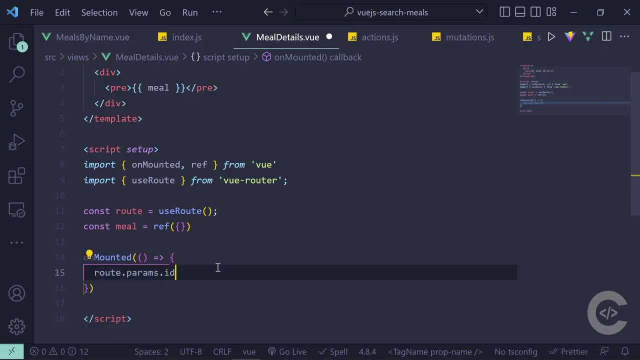 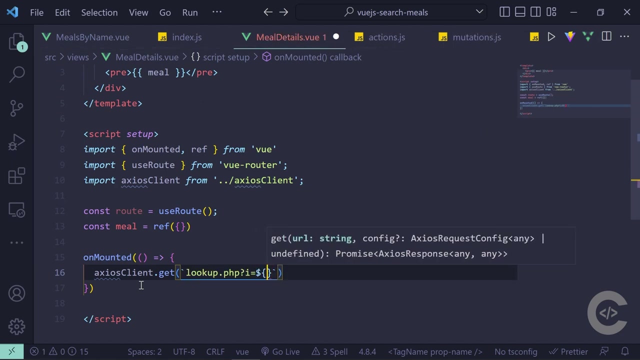 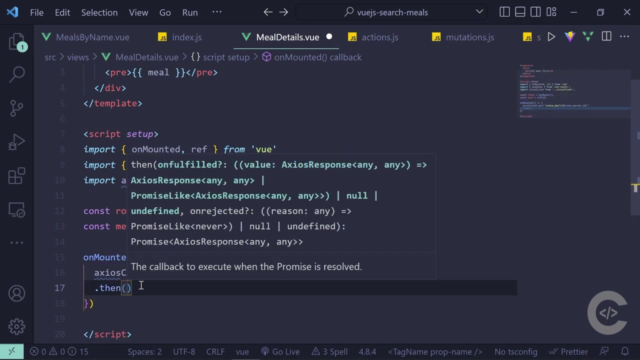 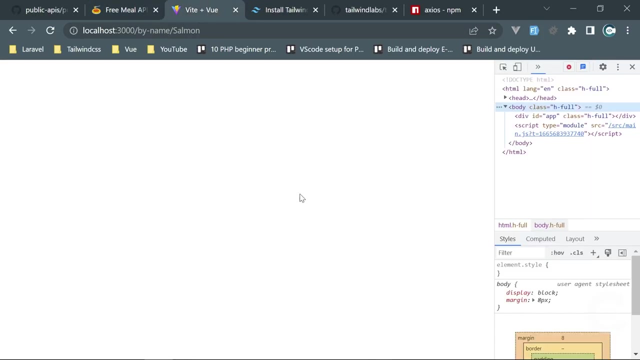 this is the end point okay so i am going to now okay let me think do we need to get the meal details and save that in the view x uh not sure so in this case um i'm not going to call an action of the store instead i'm going to directly call axios client get specify that url and write the measurement in one element and specify the voluntarily ah here we need uh wrote params id okay we get meal inside then we take the data and to structure that uh from the response we take the data and then meal dot value equals data and let's right here hit debugger as well to see what is the actual data coming so if we just if we just we have an error let's see meal 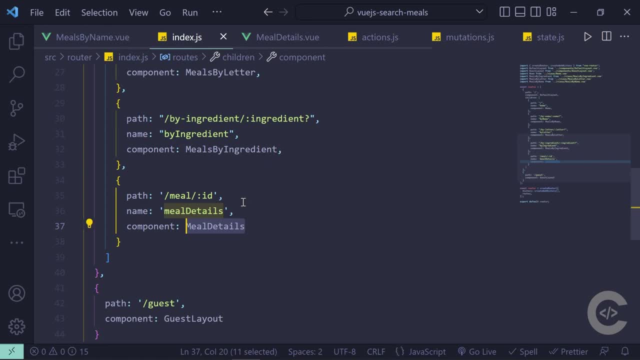 details is not defined that's correct let's go in the router and we have to import meal details right here 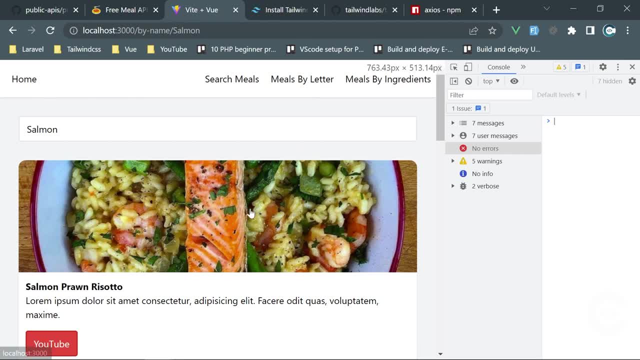 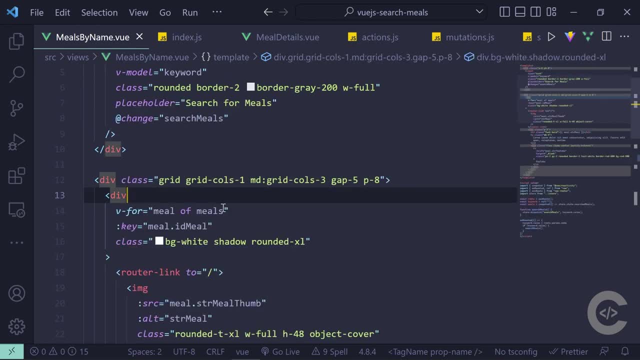 here okay and let's actually link to the meal details from meals by name so right here we need to change this into 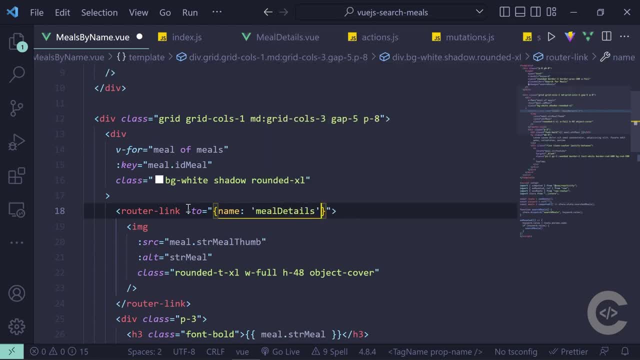 name meal details and we're going to specify params right here and id corresponds to meal 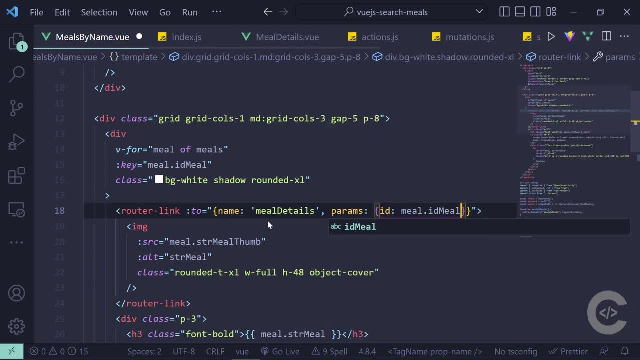 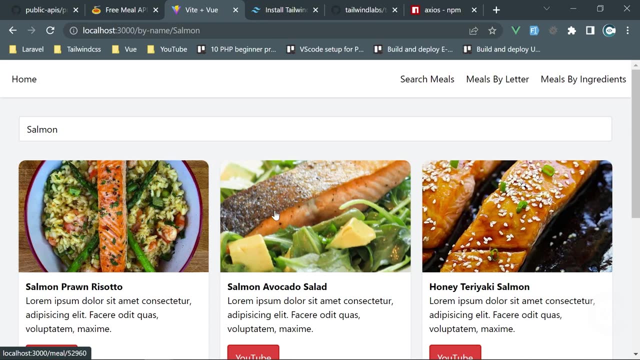 and what is id meal id meal okay we save this and now let me remove the right side and now on mouse over 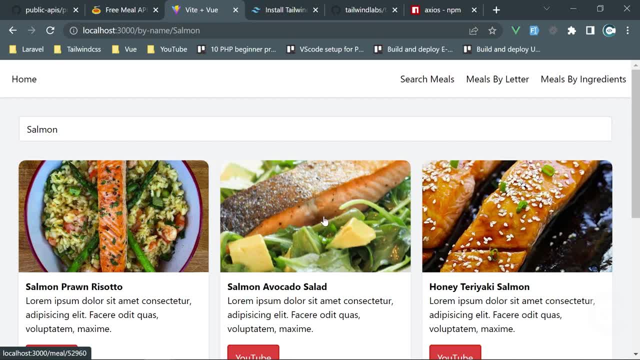 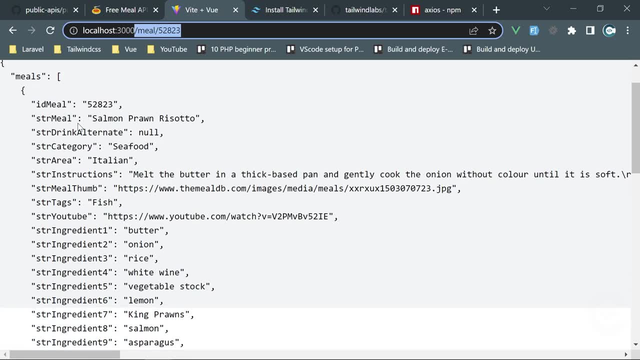 we see at the bottom left the urls are changing so i click on the first one and this is the meal url and we have all meal details so we have meals right here and however 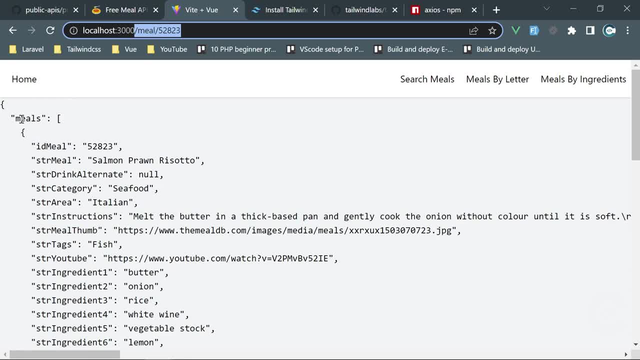 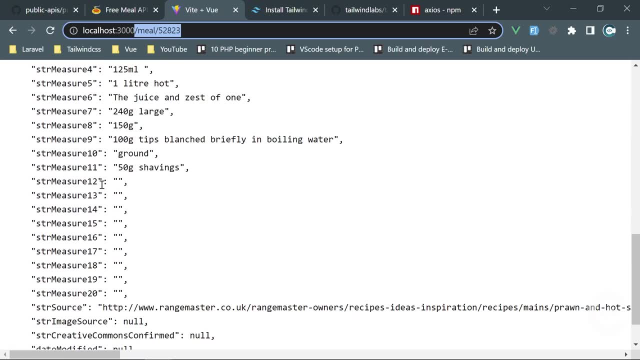 it's going to return only one meal right there because we're gonna take that by id 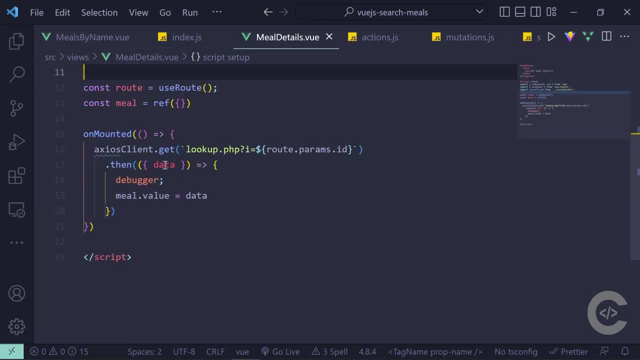 so if we go in the meal details this data will have dot meals inside and we're going to take 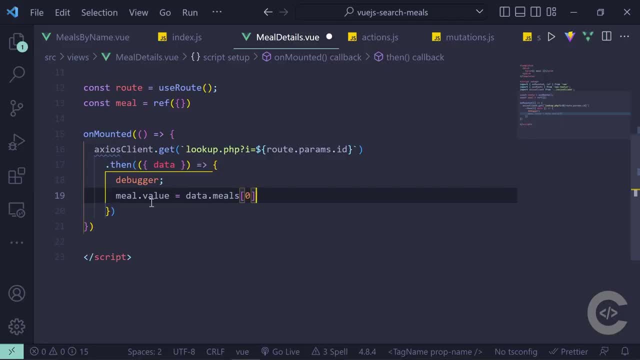 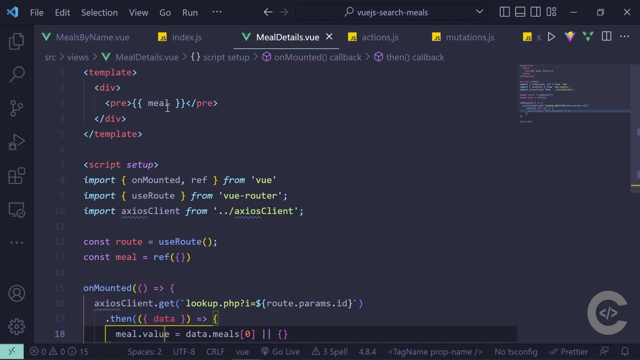 the first from this meals at 0th however this might not even exist so if this doesn't exist let's take empty object okay so that we don't have any error in the template 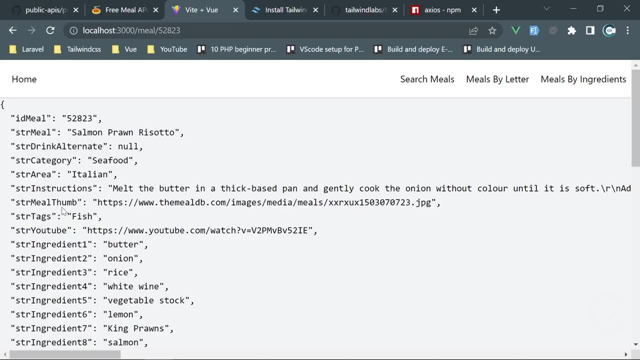 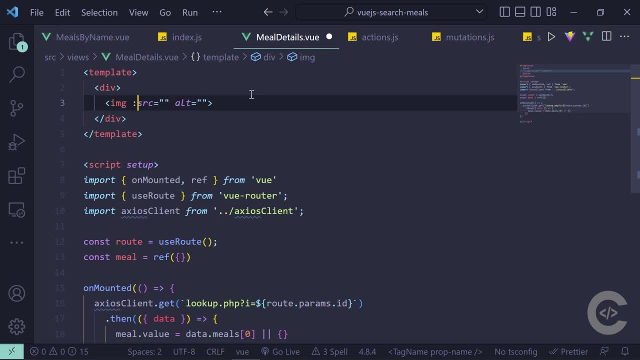 and now we print entire meal which looks like this now let's take this image and display that we will need that right here meal dot source and then right here we'll need meal dot str meal 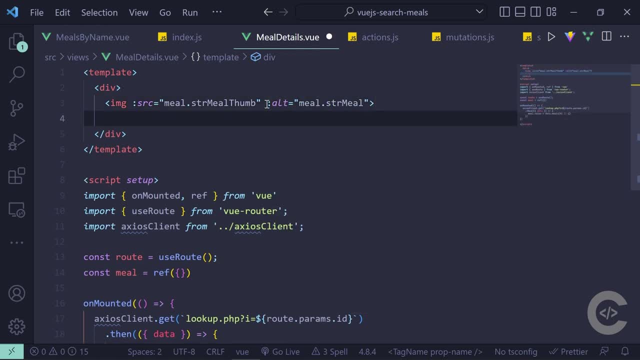 using colon then we need yeah let's first display page one with meal dot 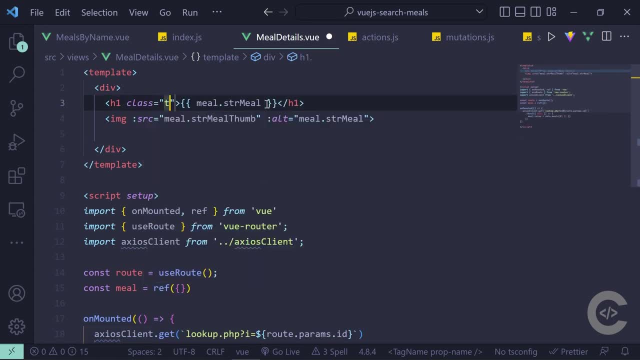 str meal which is going to be the title let's give it some time on cs classes text like 5 xl 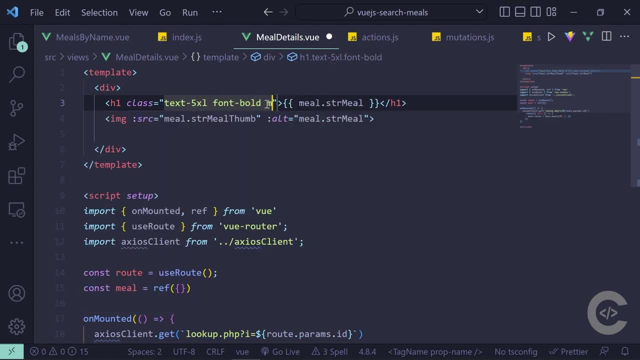 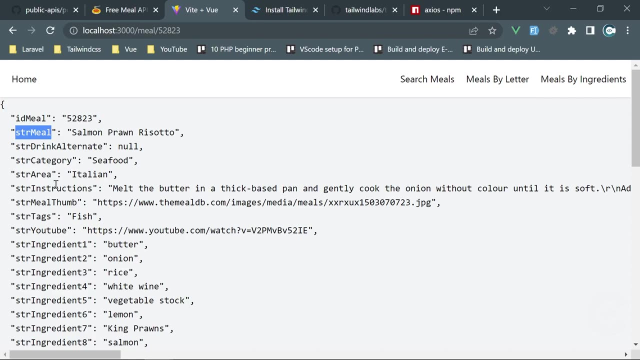 font bold and margin bottom 5. then we have this image and then we're going to display str instructions let me actually output 3 as well because i don't want to lose everything about about those um 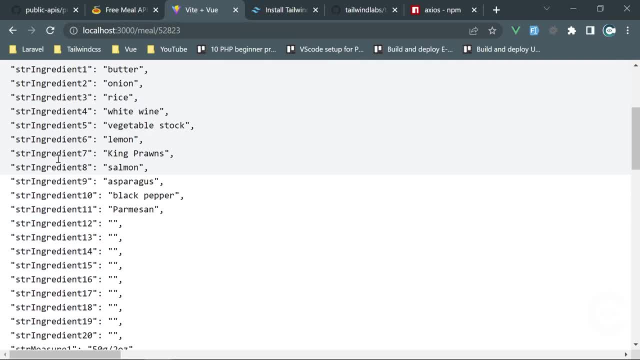 about this meal object basically okay we have those ingredients which we can list them we can show this as well 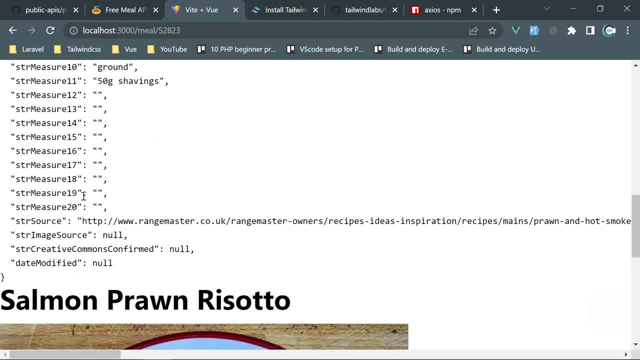 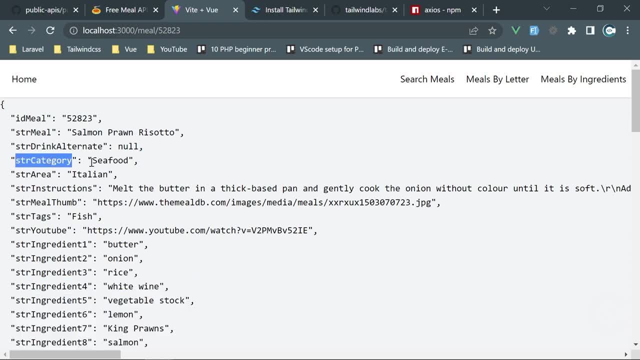 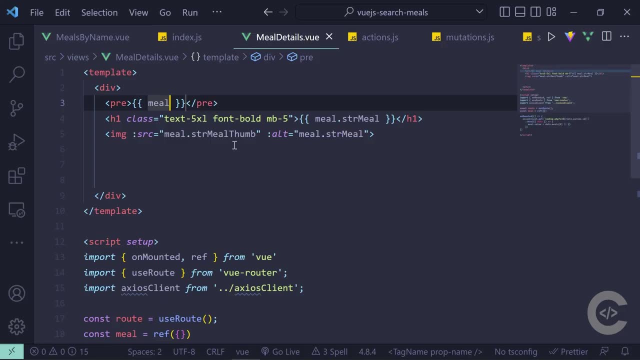 YouTube link and measures as well and the source link as well basically probably we should show everything which we can show category as well and area okay let's let's save this and have a look so we have the title and then we 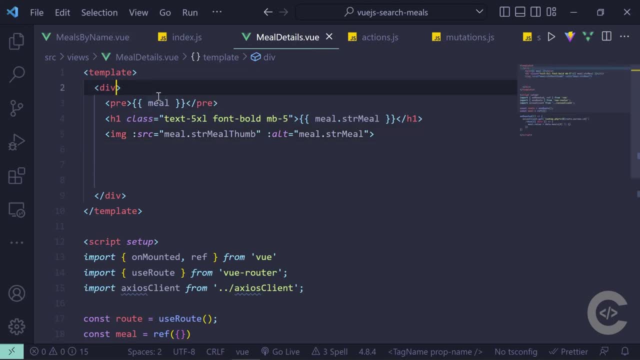 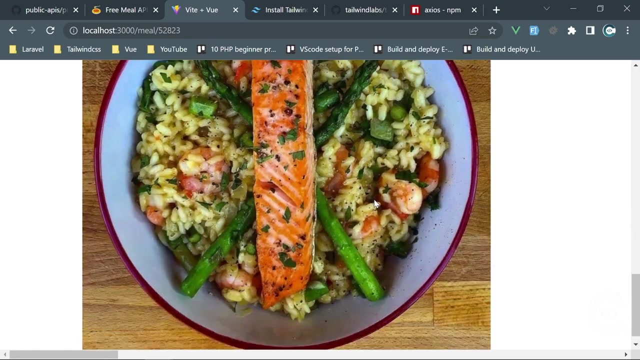 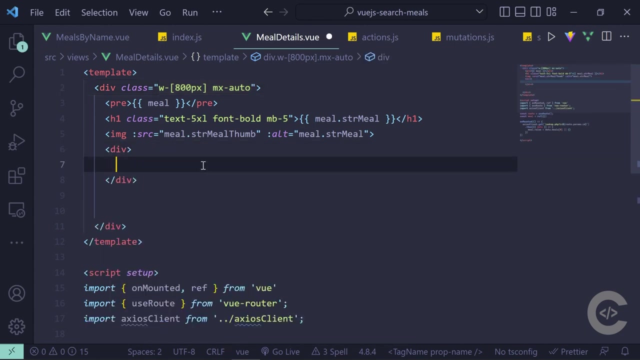 let's put this in the center so let's give this one width of probably like 800 pixel and margin X auto now this is in the center let's at the bottom let's put a div with a few few fields, let's display here 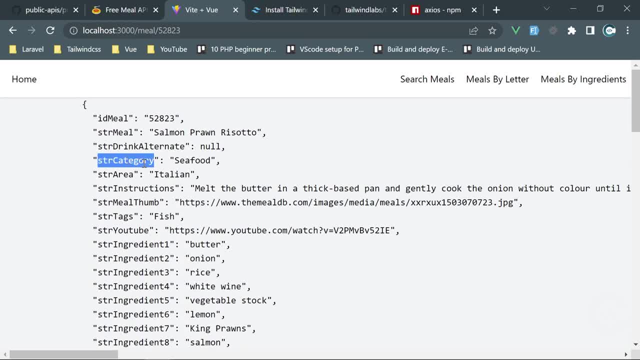 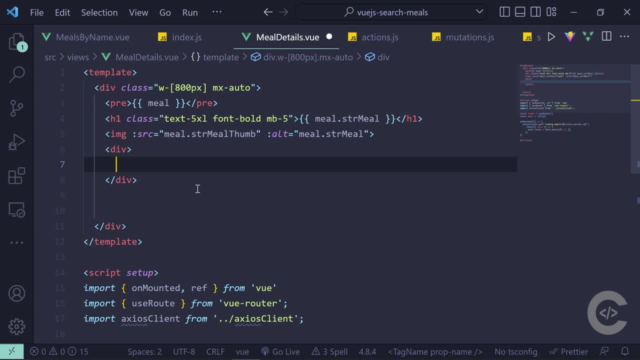 a few fields, let's display here here category area and tax okay let's display them category that's going to be meal str category we are going let's put this in its own div and that prnd will have grid grid calls 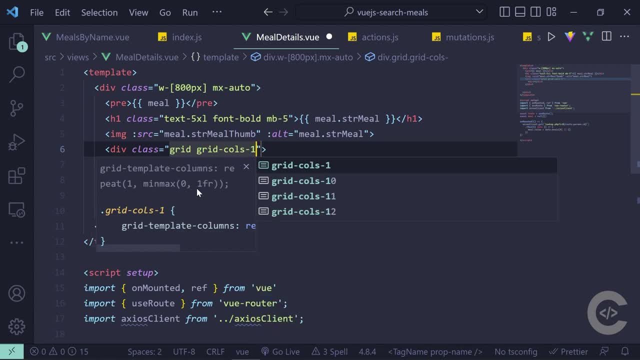 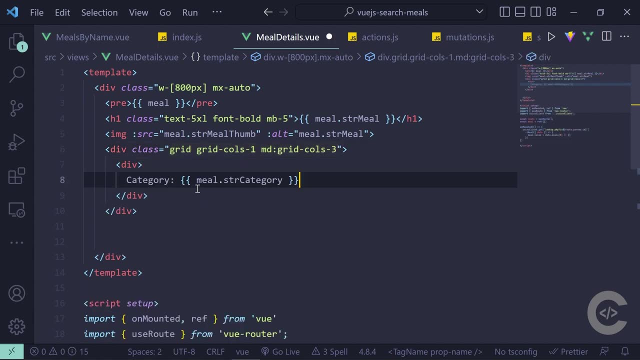 grid calls one and on md grid calls three all right so we have it right here and let's duplicate this two more times and we will need area and it's going to be str area and str tags so right here we need tags tags here 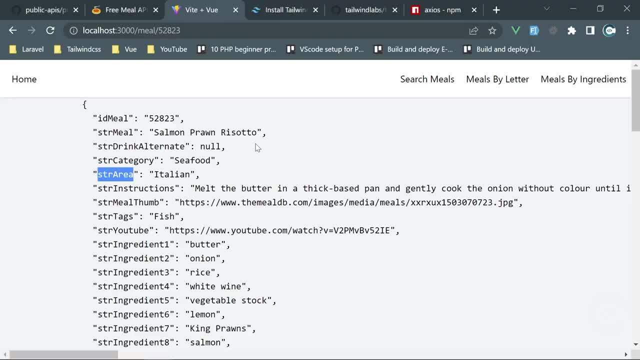 so we save them and let's check how this looks like 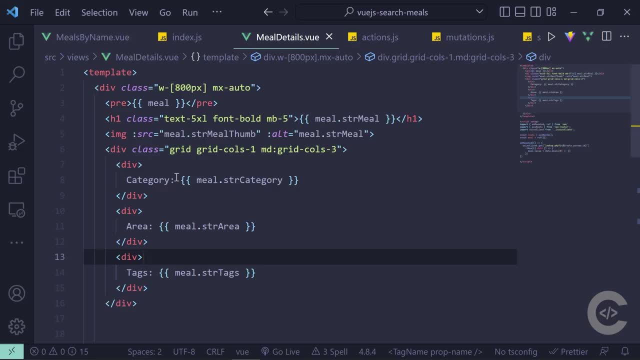 okay this looks nice let's make the left part strong and give it font bold perfect let's give this one also text lg and padding y2 so we save them and let's check how this looks like 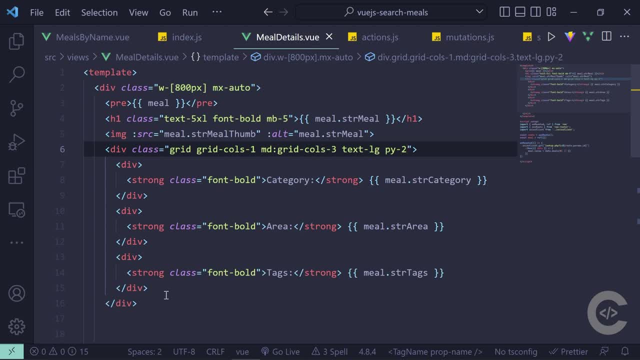 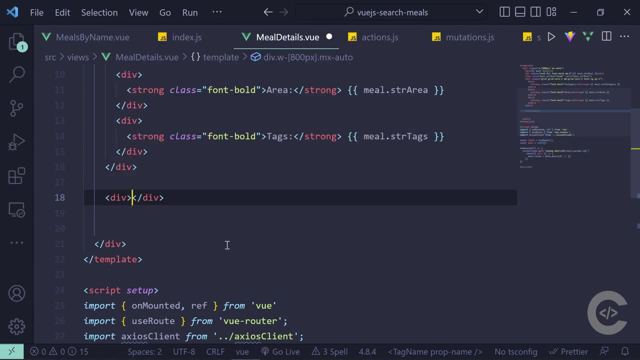 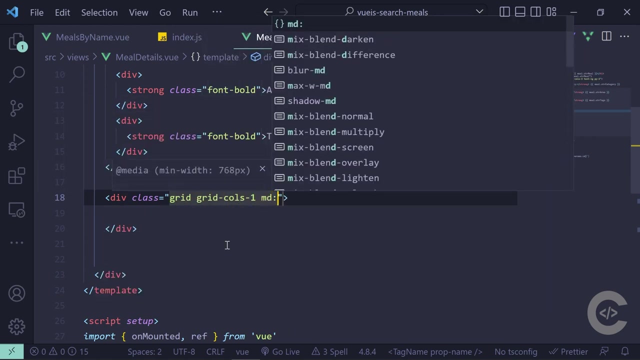 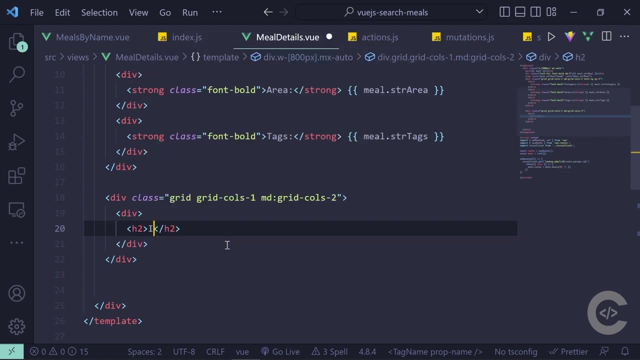 some small padding okay then down below we need to have two sections ingredients and measures so let's create div with class grid grid calls one on md grid calls two we need the left side to be h2 ingredients and we need to output all the ingredients right here 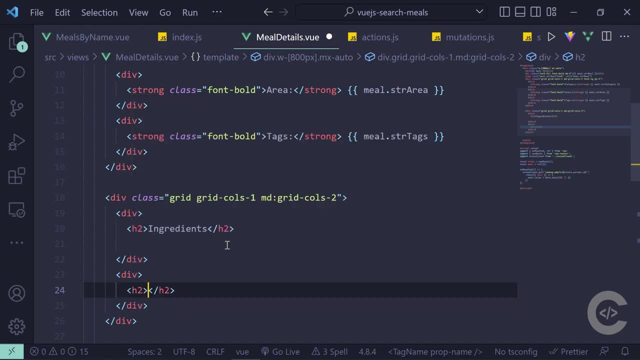 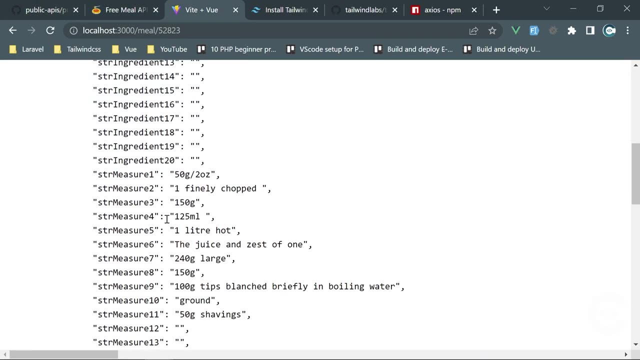 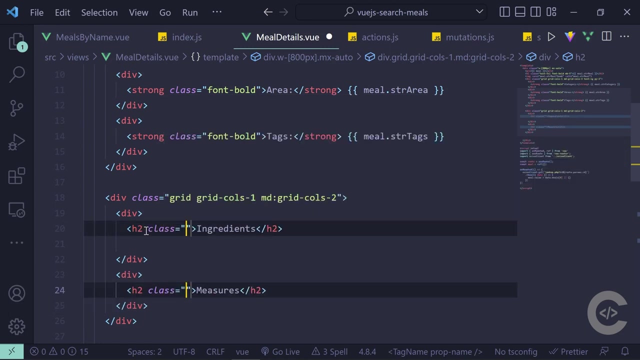 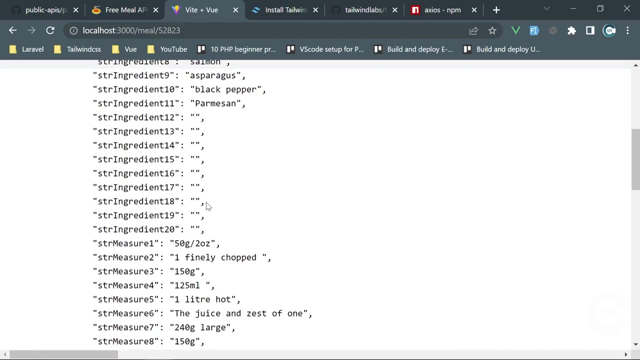 and then we need h2 what is the second part where's that ingredients and i think measures yes measures so we have them now let's give them some styling text to excel font semi-bold margin bottom three okay and now let's output all the ingredients which are not empty so we have 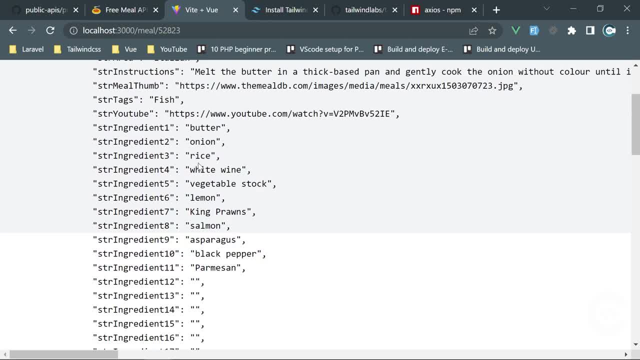 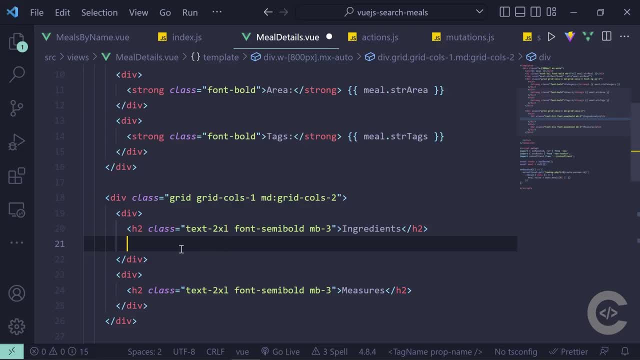 like 20 ingredients okay so now i'm gonna make a loop from 1 to 20 and output those ingredients 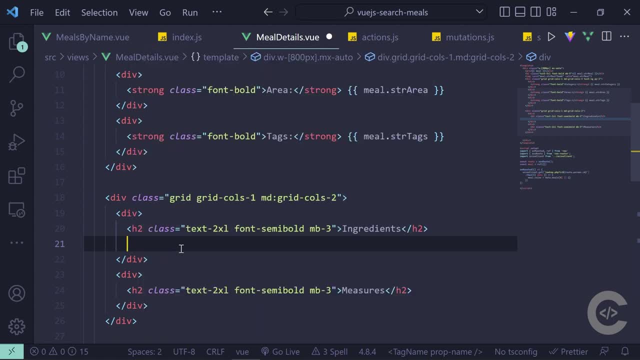 so for let's create let's create what let's create ul 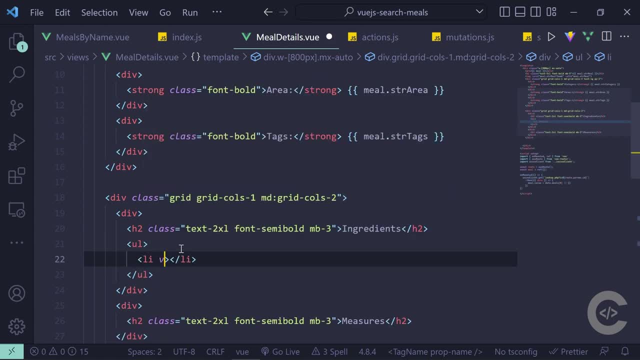 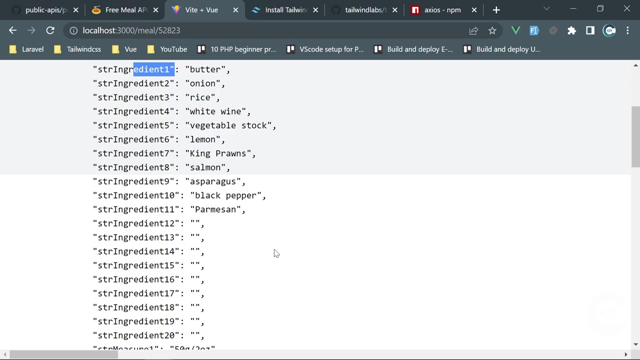 and le and v4 v4 i so i'm going to just call it i and i want to create basically i want to iterate from 0 to 20. well i think if i just i want um 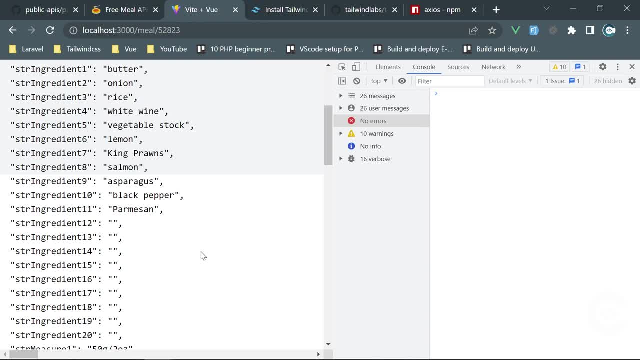 just i equal zero while i is less than 20 i need to iterate so if i just i want um just i equal zero while i is less than 20 i need to iterate so if 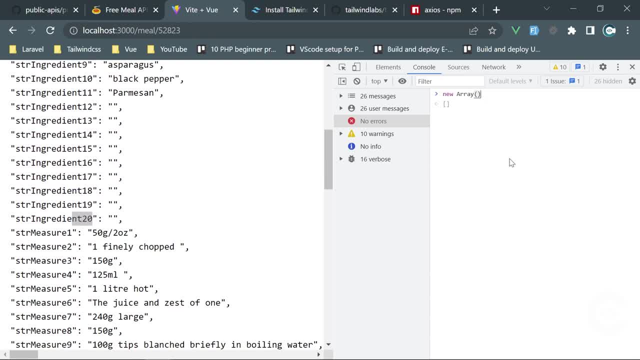 just create new array like this and in the argument give it 20 that's gonna give me an 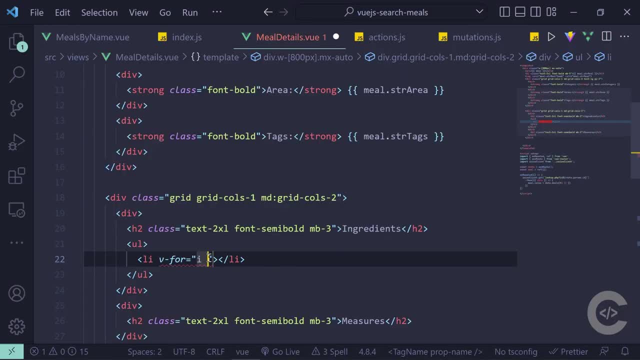 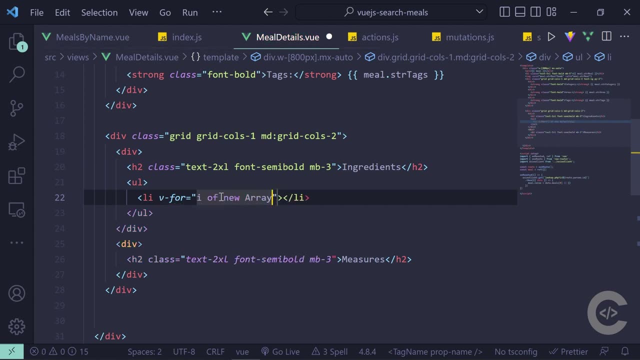 array with length 20. so i think i can iterate over this so i of new array not sure if this will work in the template passing here 20 not sure we will test and i'm going to output 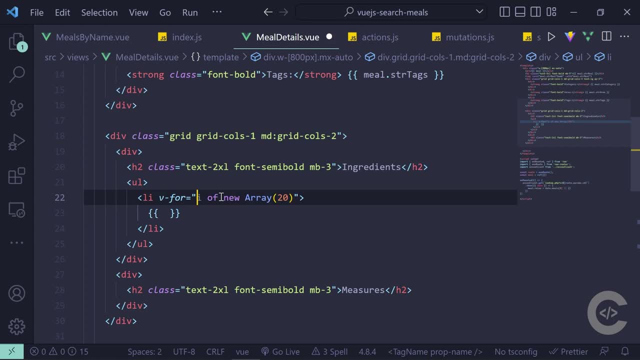 we have i and i'm going to output i need index i is not an index i is the element 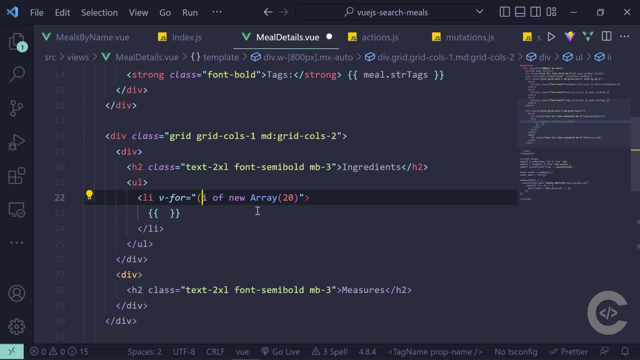 i think i can take the index like this this is the element and index let's just output index we save this and have a look yes 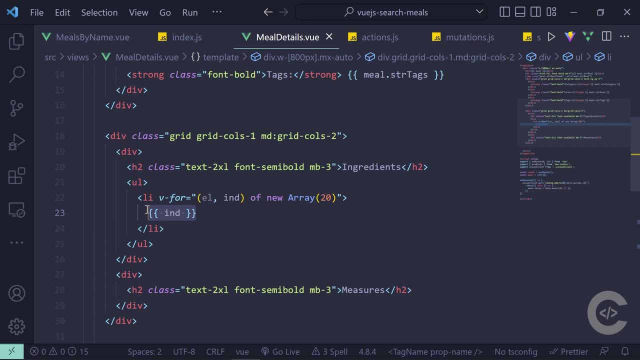 here we have zero from zero so we basically do like this we write the if right here or this even can be template and then inside we're going to have le with the if and we're going to check if meal 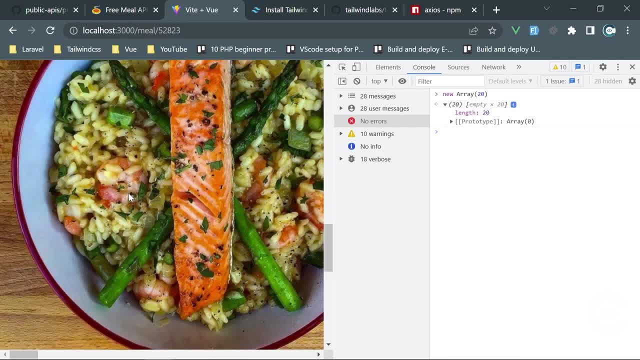 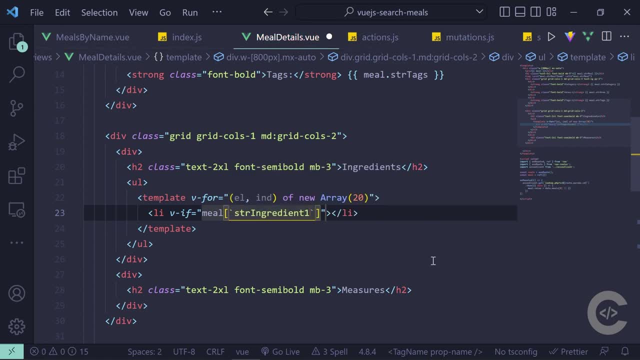 with square brackets and we have those str ingredient right so like this str ingredients then right here we need index plus one if that exists okay so ingredient one if that exists we are going to output this right here okay so let's 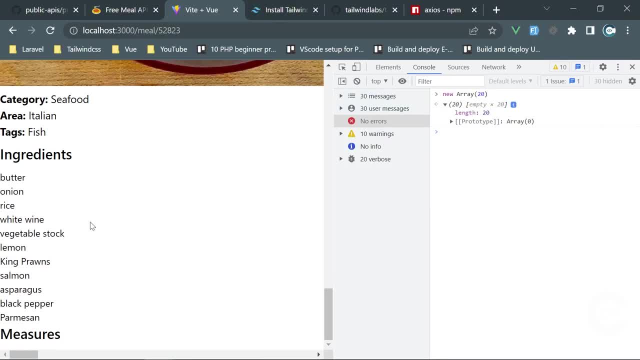 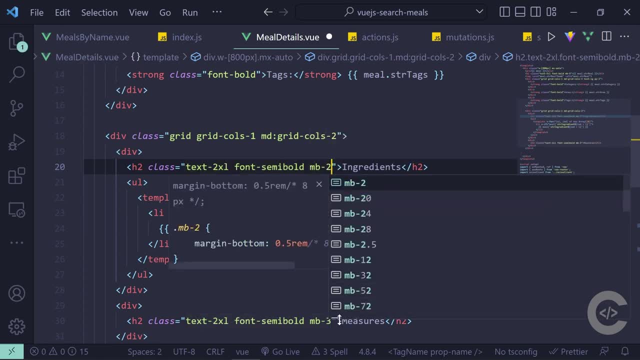 have a look so here we have all the ingredients this this is fantastic and let's reduce the margin bottom 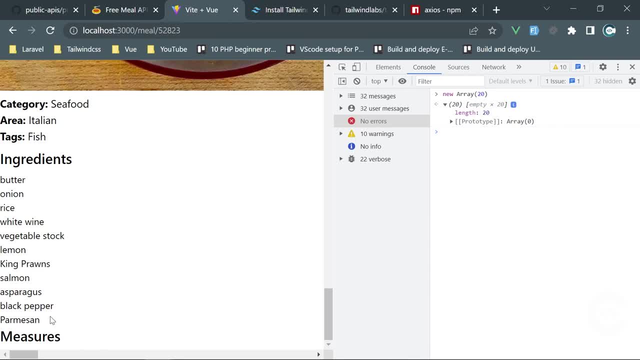 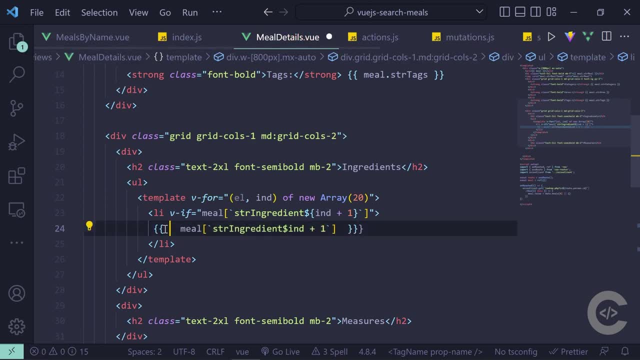 okay and we have only like 10 ingredients okay we can even output index in front of it uh oops something happened 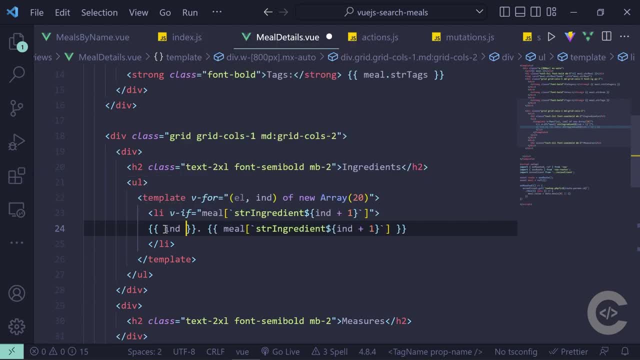 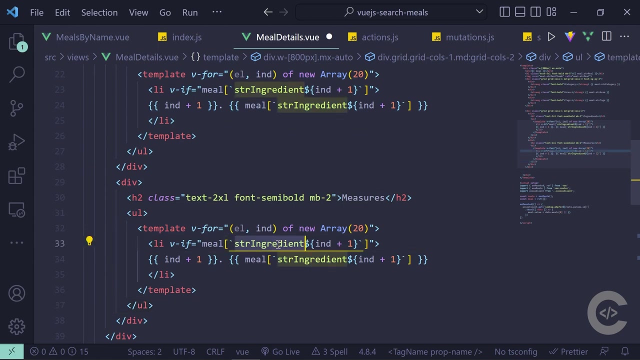 okay ind uh we should have ind plus one and dot here we go and in the same way in the exact same way we can output measures so st um let's search for str measures 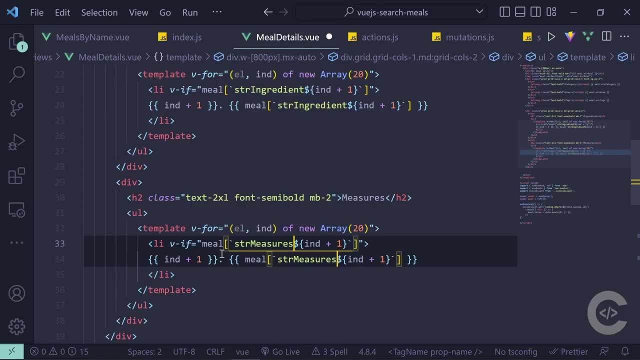 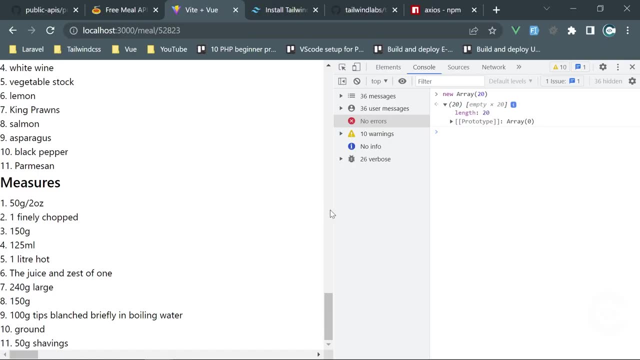 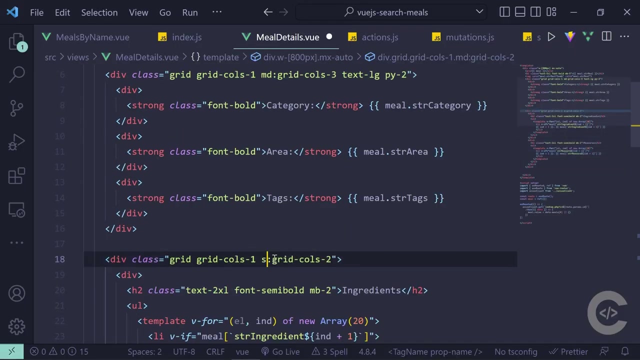 or str measure i think it's in singular form str measure and here we see that it's in singular form str measurement all right if i reduce this part now well i think i should change this grid into sm 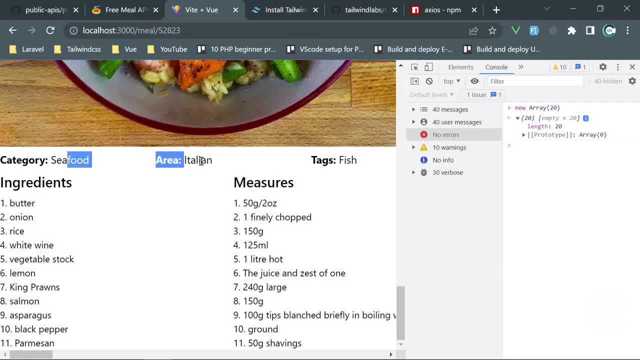 and right here as well i'm going to change this into sm 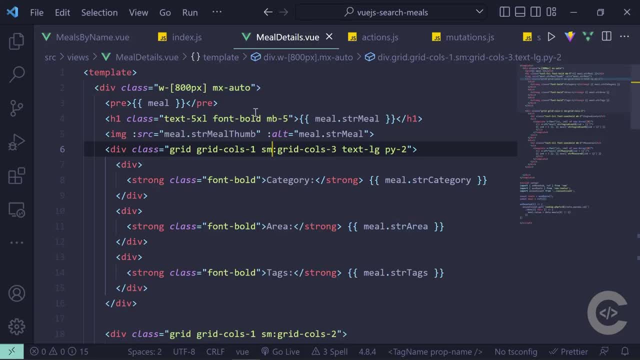 okay and this is my page however i'm gonna give this one all so padding 8 maybe 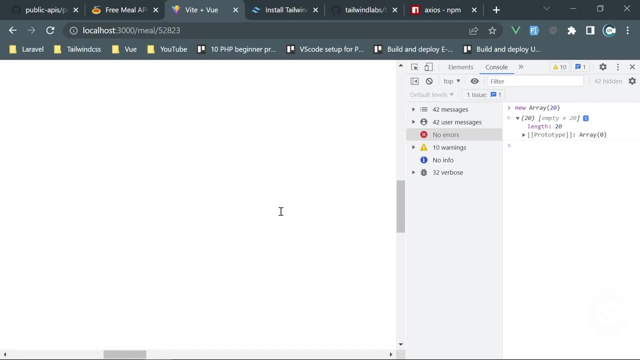 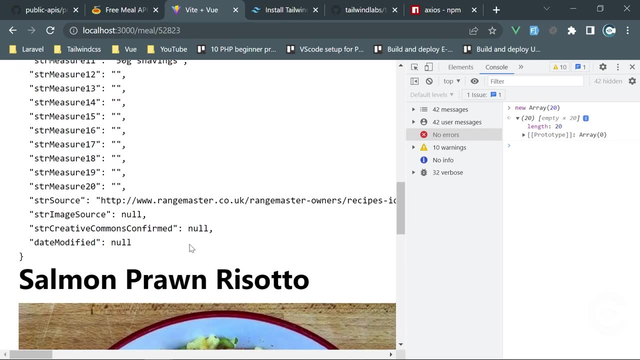 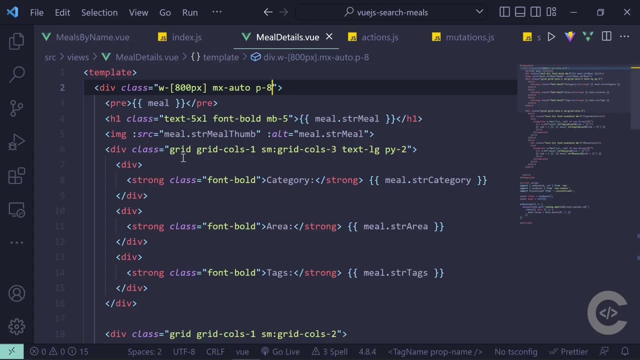 now we have horizontal link which is basically for this link okay that's not a problem and at the bottom let's put these two buttons one for source and second for the youtube video so let's go in the meal by name and here we have this youtube video button and i'm going to create 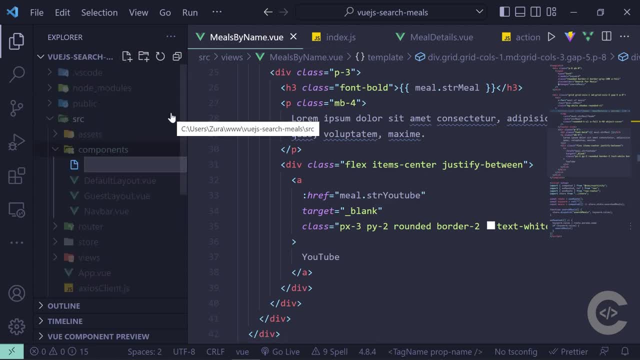 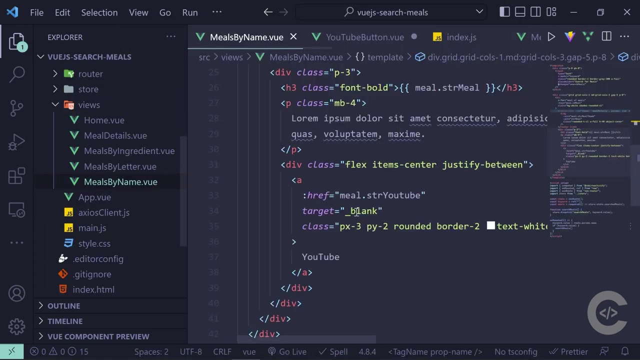 now reusable component for this go in the components and we are going to have we can have like a general button component or we can have youtube button component okay let's make it youtube youtube button dot view let's generate template right here and i'm gonna copy this and at this moment i'm gonna use you 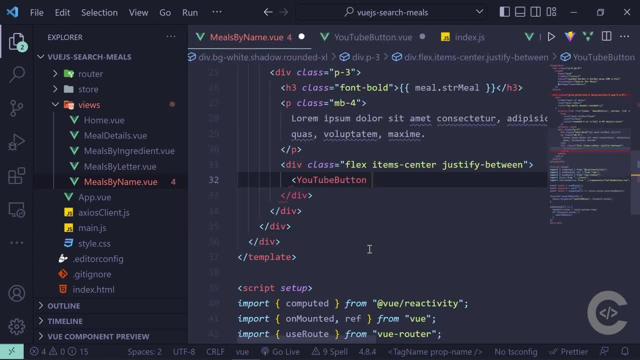 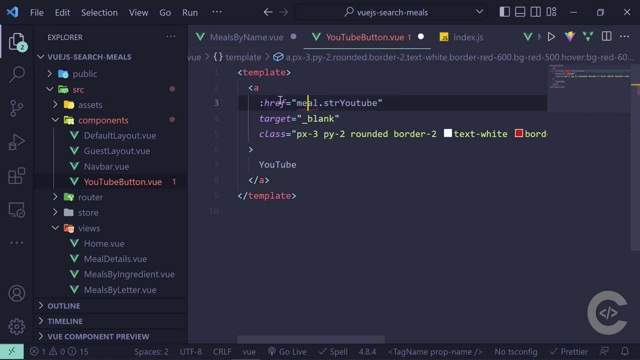 youtube button and we need yeah we need also uh slots right so i can leave it like this youtube button and then paste this right here but first i'm going to define the href which is going to be a prop but then this text 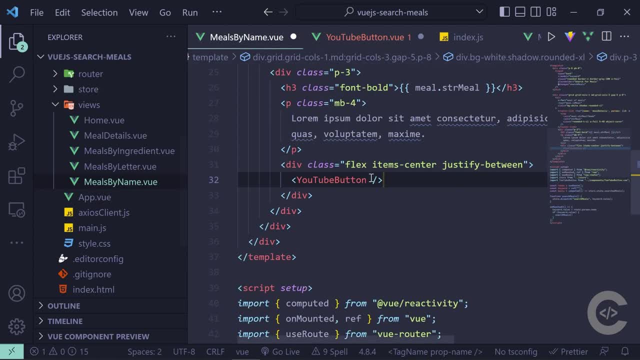 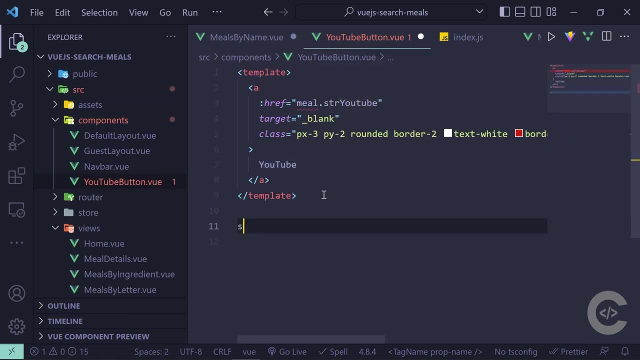 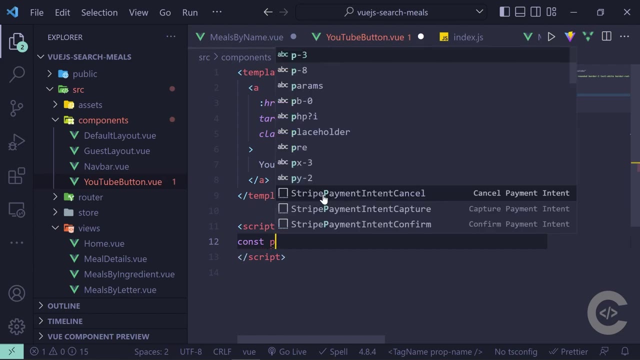 will always be youtube what if i want to give it a name go to youtube for example i won't be able to do it like this 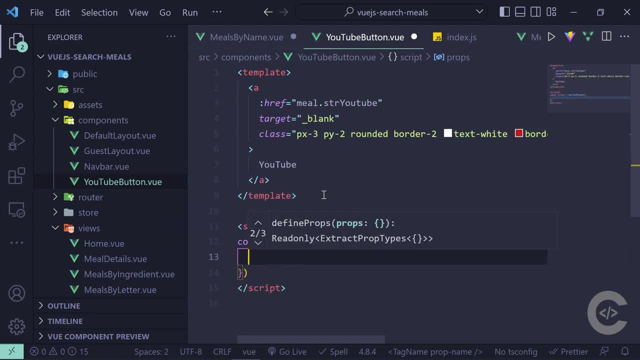 define boys and we're gonna define href to be string all right so we take this out href here 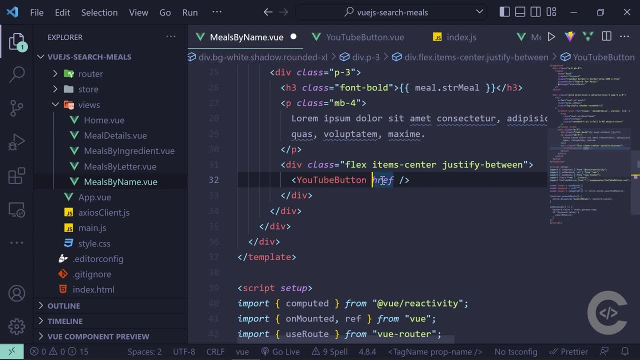 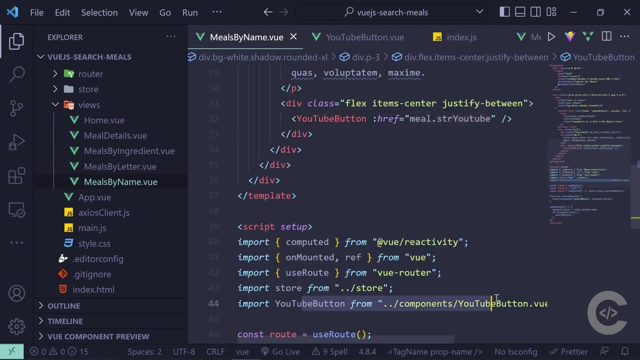 and then href i'm going to specify href to be meal str youtube so if i save this now this youtube button was automatically imported in the script if i save this 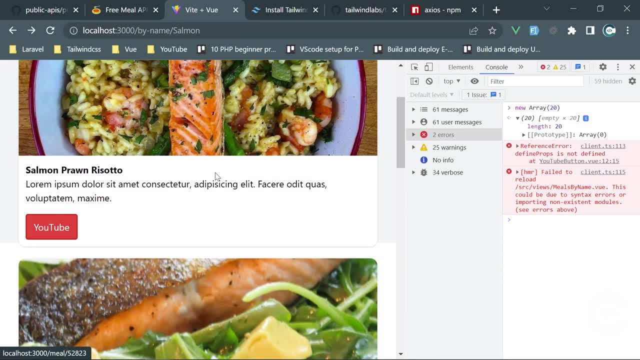 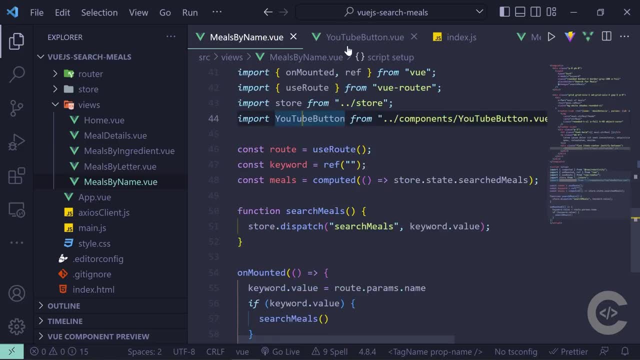 and go back basically we still see this youtube button uh define props is not defined okay we don't see that define props 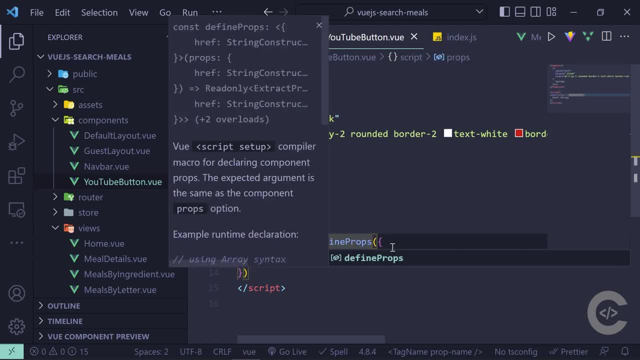 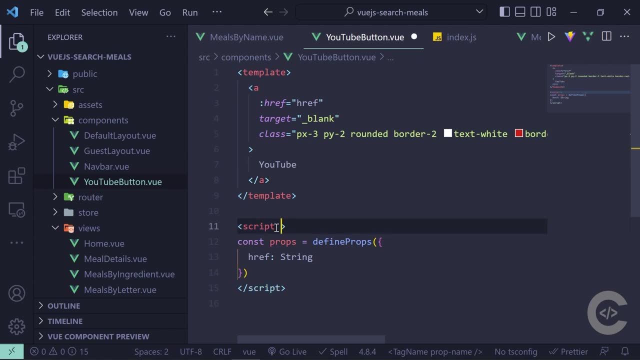 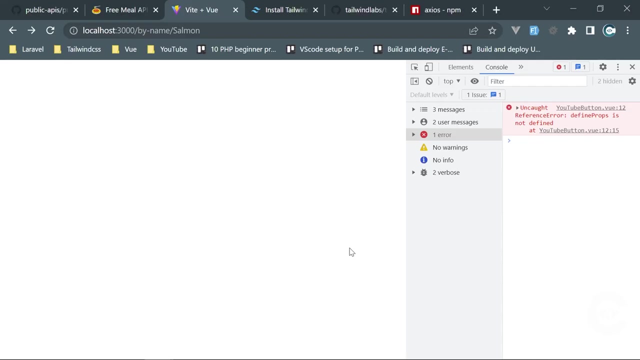 what is the reason why is not that defined that is not defined because i don't have set up script right here okay and just because of it we have this error let's check in the 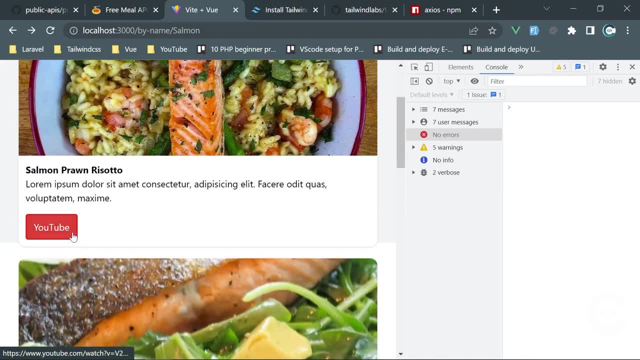 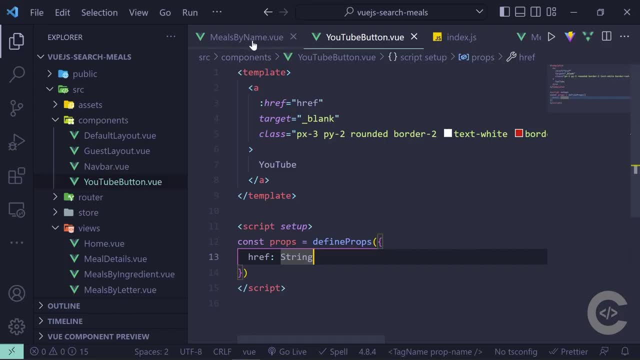 browser now here we go and we see this youtube button and clicking on that opens actually youtube video so now if we go in the inner page and we open 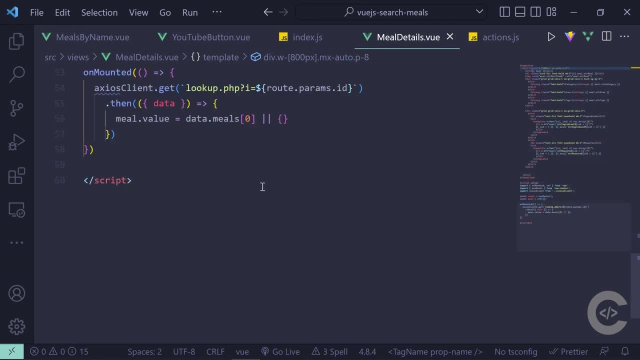 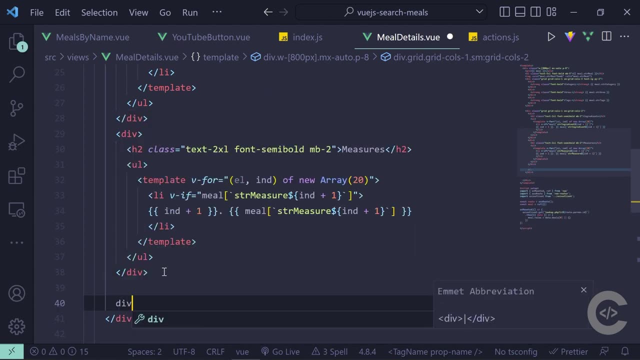 pen meal details at the very bottom we can probably right here i'm going to create a div and inside there we are going to i'm going to put youtube button all right but we are going 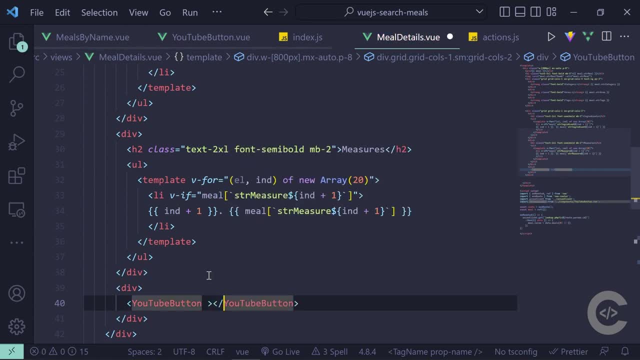 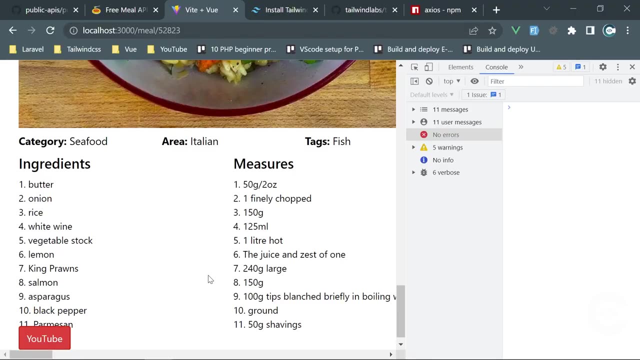 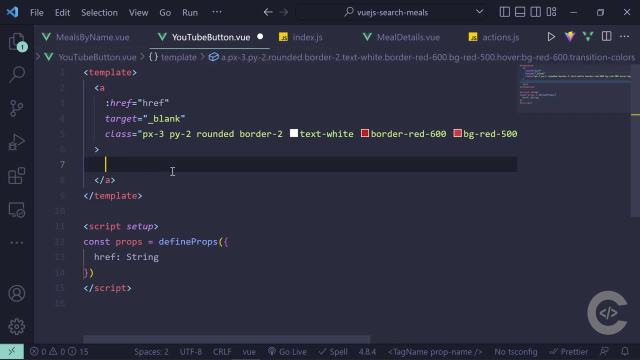 to accept text as well so if i give it like um like go to youtube okay i don't have that possibility at the moment right here so if we go in the youtube button i am going to output right 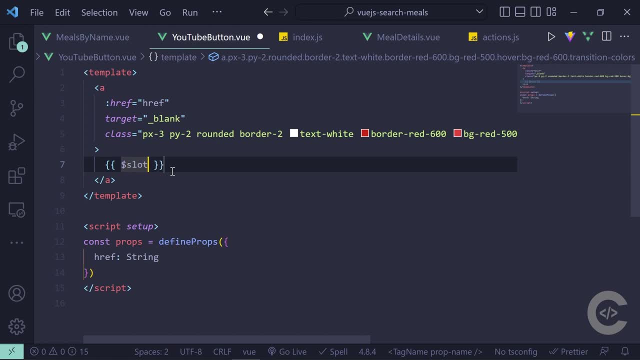 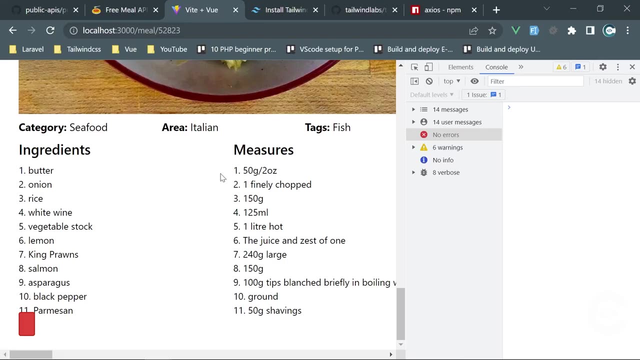 here default slot i think this is how it should be not sure not sure but let's have a look okay okay it 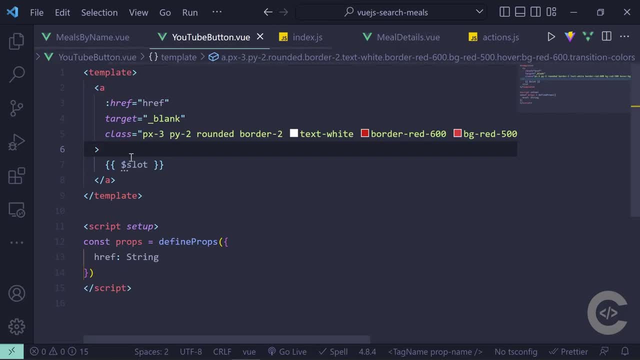 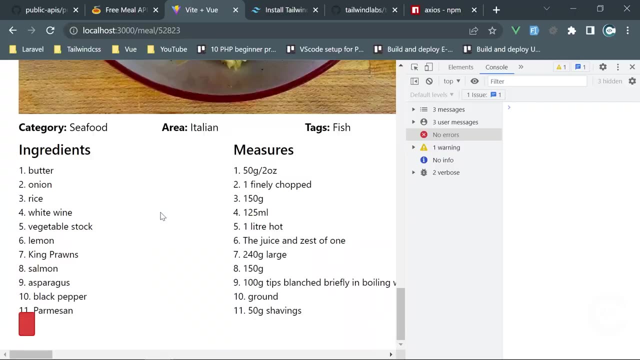 doesn't output anything probably the store sign is not what we want no that is not that is not it let's go meal details 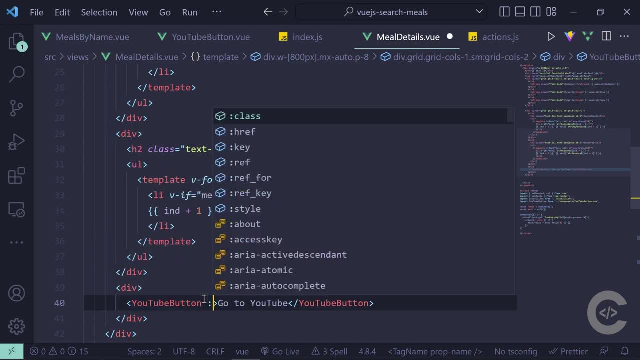 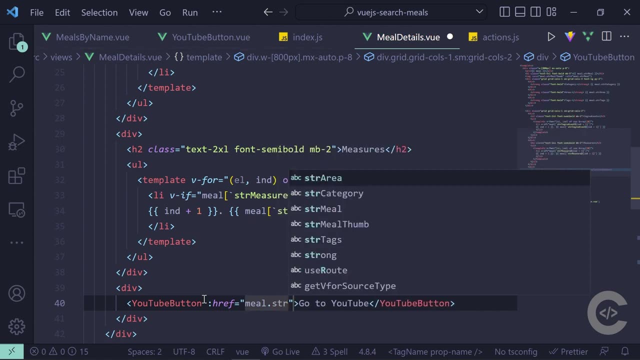 let's specify first href to be meal str str how it's called 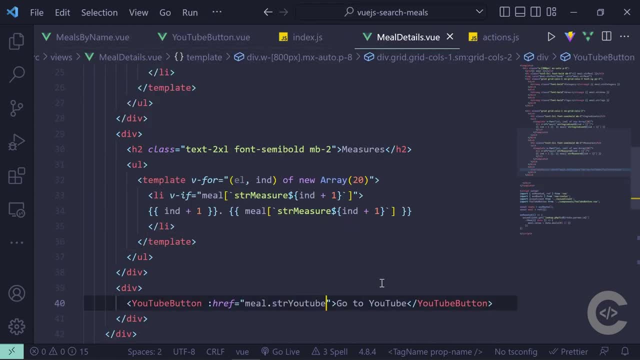 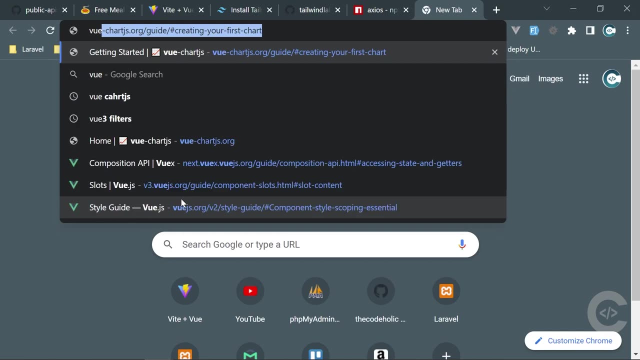 str youtube okay so we have this um but something doesn't work so view three props not props but uh slots 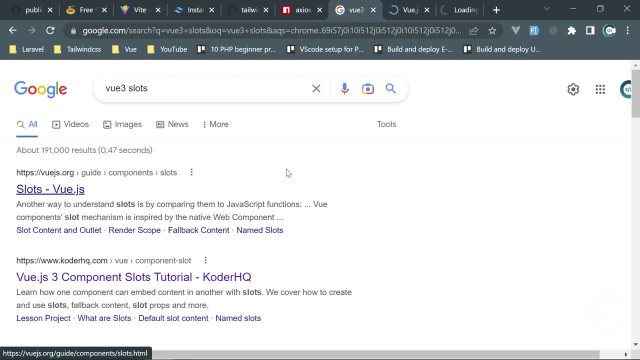 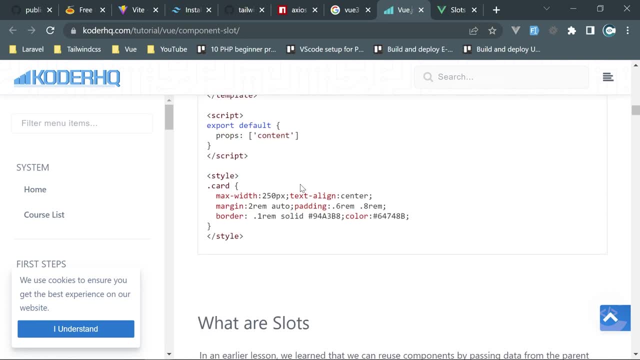 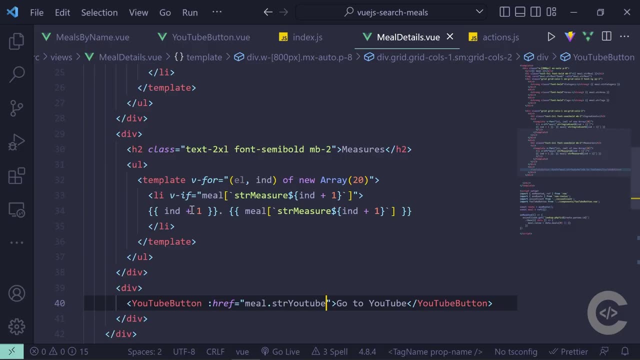 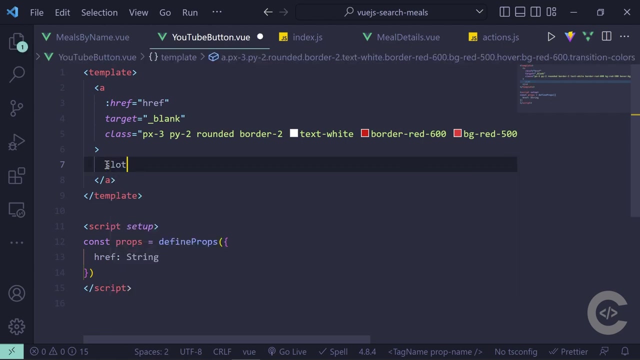 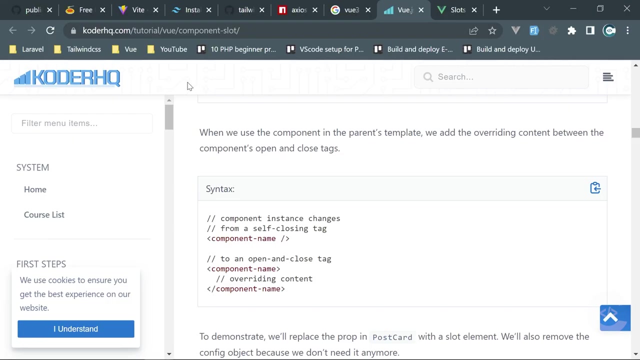 okay let's let's find this out we have card okay what are slots i know what are slots in the template we need to find a card okay let's go with card okay let's go with card okay let's go with need a slot. So if I go here, I think I need to define slot here. And just save that and 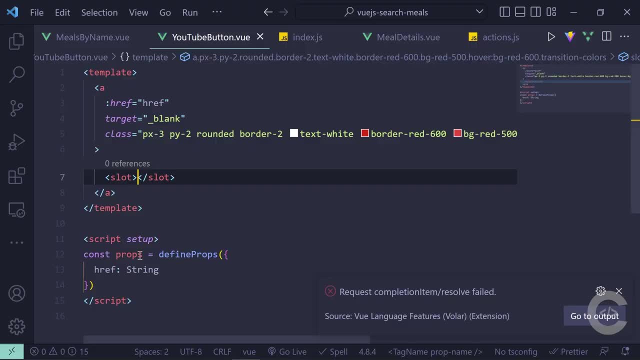 have a look. And right here we see go to YouTube. Okay, I think I mixed this into Laravel when 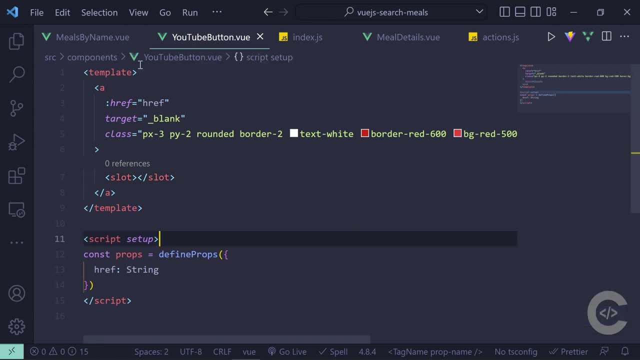 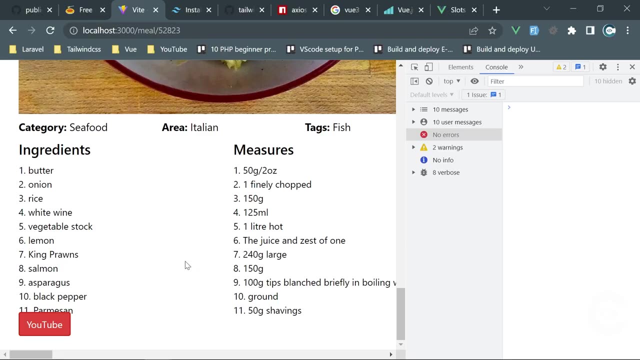 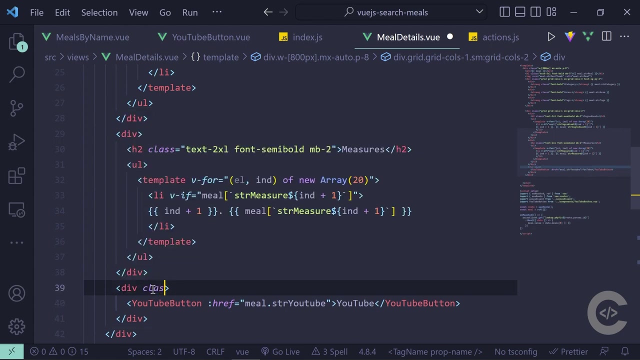 I used these curl braces. So now if I go in the middle details, I actually want to change this into YouTube again. And let's give this one margin plus margin top four. And let's create a second button, which will be four. 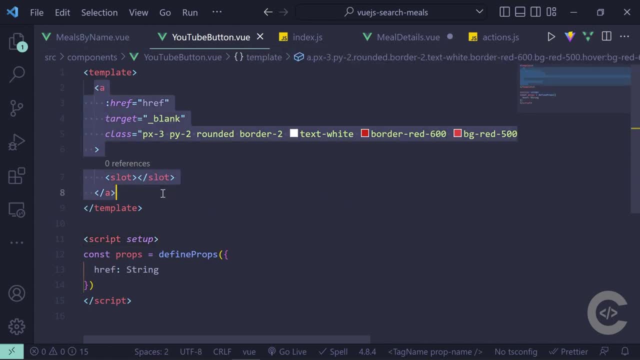 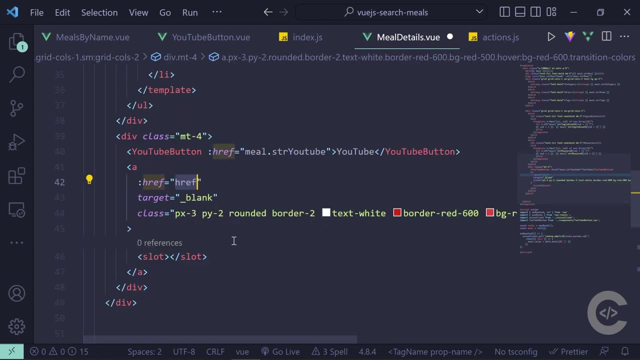 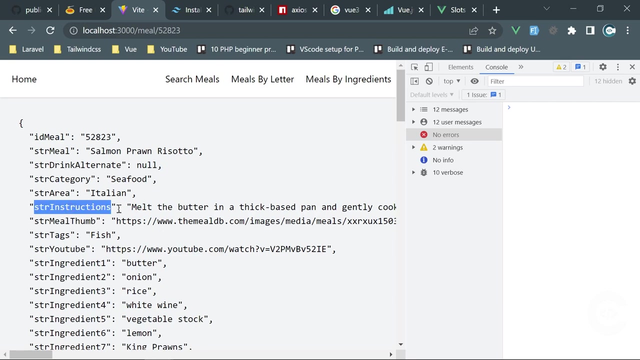 That's going to be for source. Let's put this right here. It's going to have href as well, not the href, but mil and... We need str instructions, by the way, which we don't output. 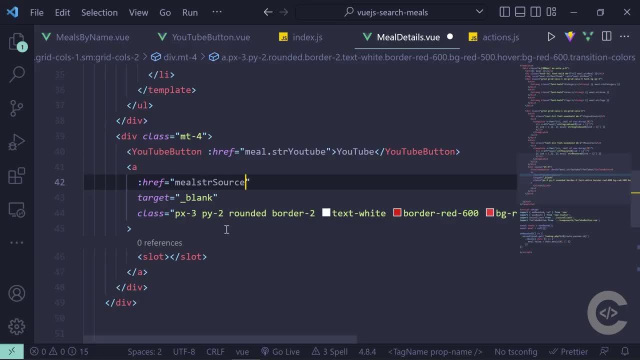 But down below we have this str source. So we need that, mil.str source. However, again, 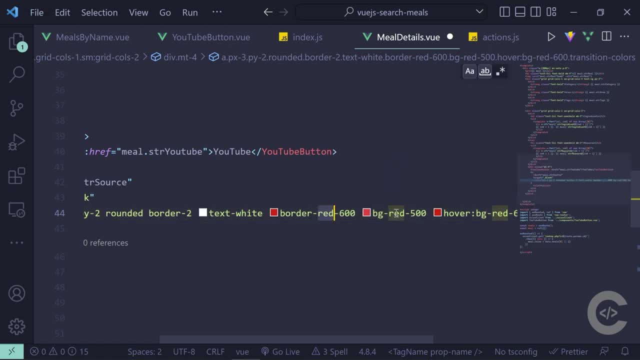 let's change this into indigo or purple. Like previously I had purple. Now I have indigo. 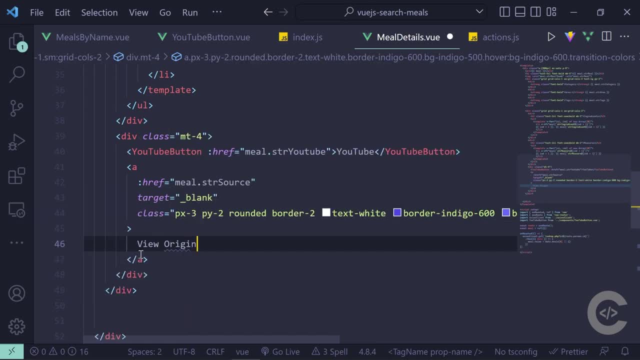 It's fine. View original source. Don't like the color. Don't like the color. Text white. let's change this into text gray 700 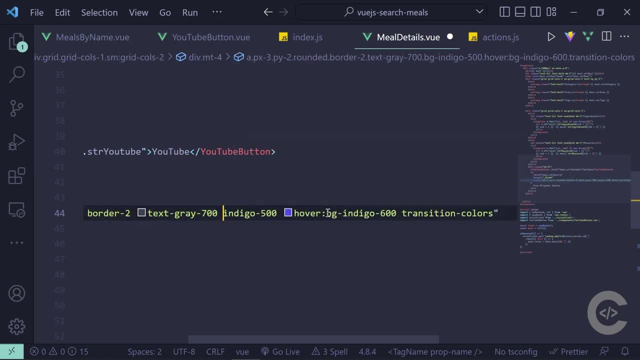 border let's remove background remove on hover let's give it pg indigo like 200 maybe let's remove border completely 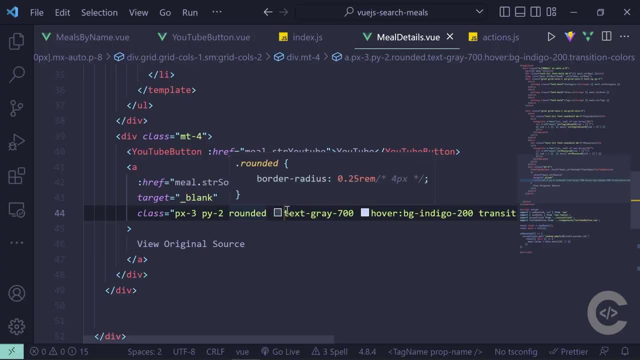 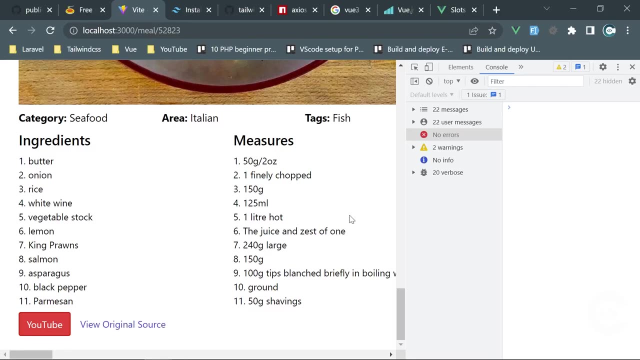 and let's give it text indigo 600 this is something better in my opinion in my personal opinion we have text gray and 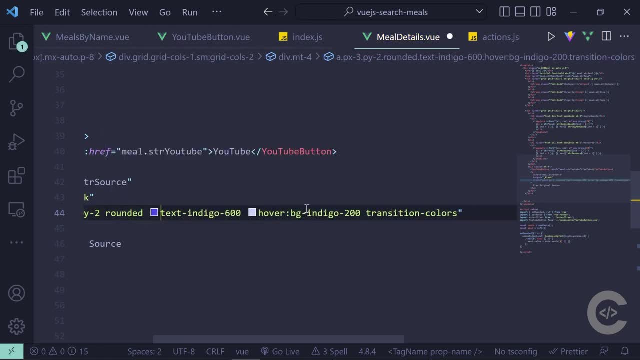 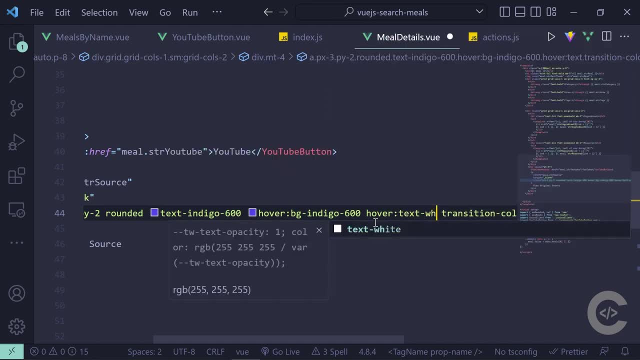 and let's give it pg indigo 600 and on hover we can give it text white let's see this is not also bad 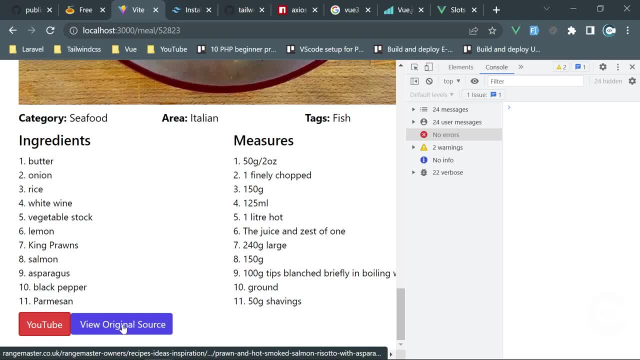 however this one has a larger height this one has a smaller height i think this is because of the border 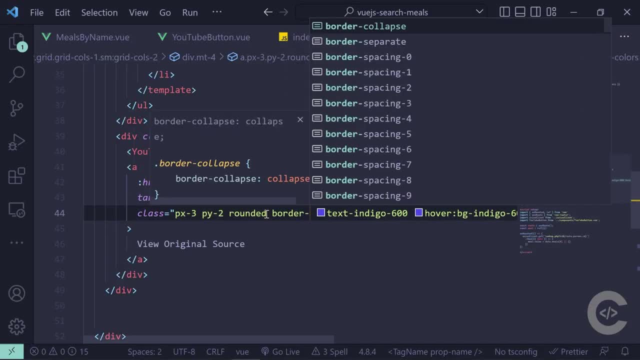 okay if we give this border uh border like two and border transparent 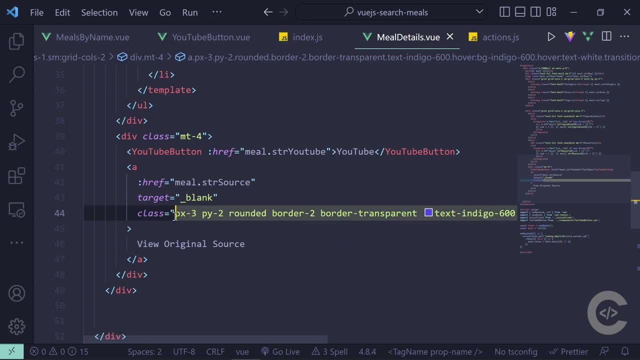 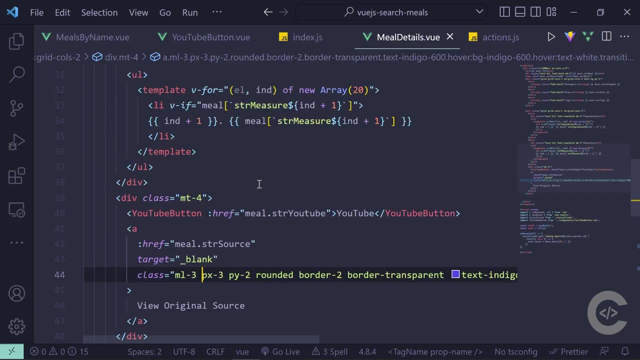 this is more like it okay let's now give this one also margin left three and here we see that and now let's output all the instructions 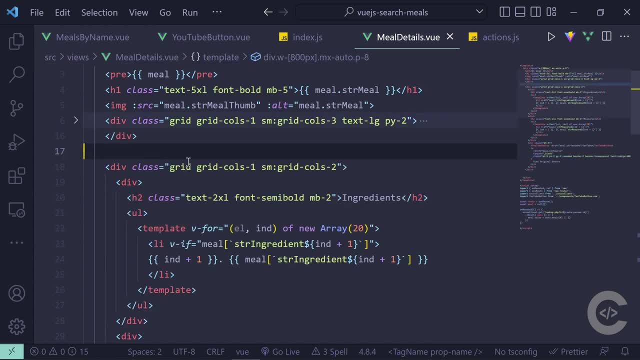 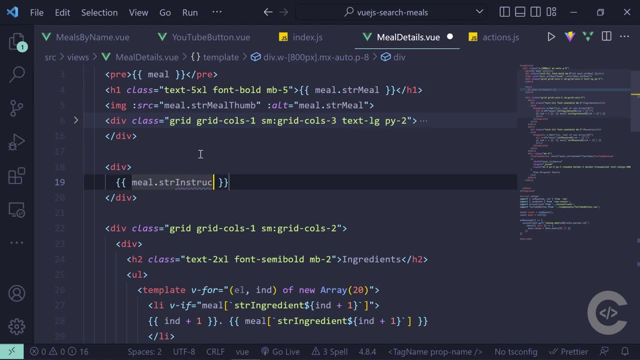 so we have this section we have then ingredients and measures and at this point we can output meal str instructions 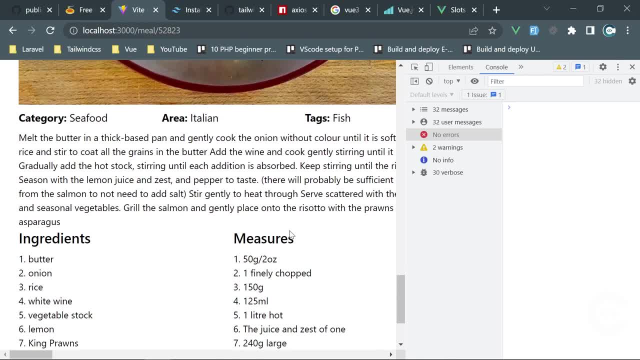 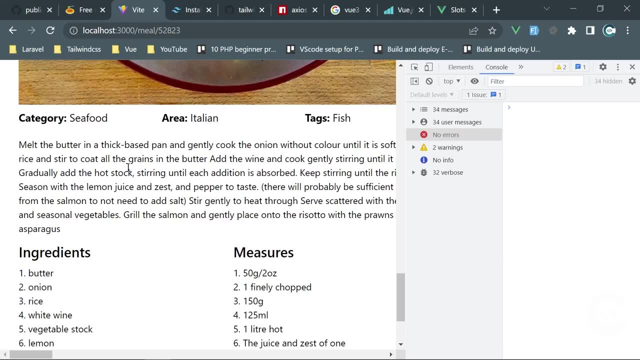 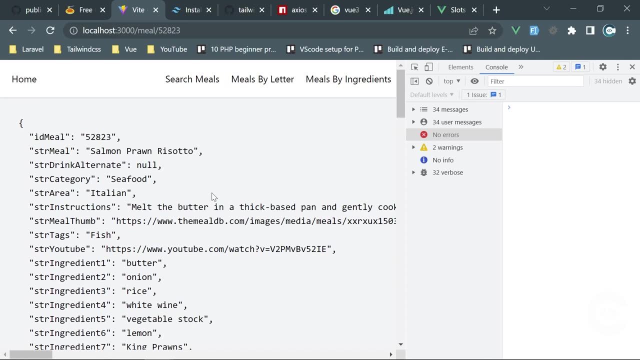 and we see this here let's give this one margin of vertical three okay i think there is nothing remained right here we have the title we have the instructions we output area category we have the youtube link ingredients measures and just like this we have 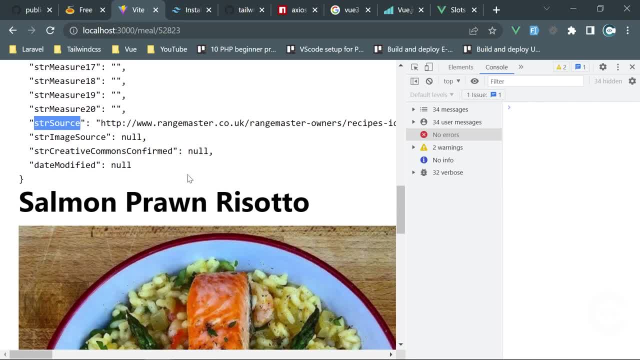 the inner page let's remove this presence data for this page i wanted to do something different 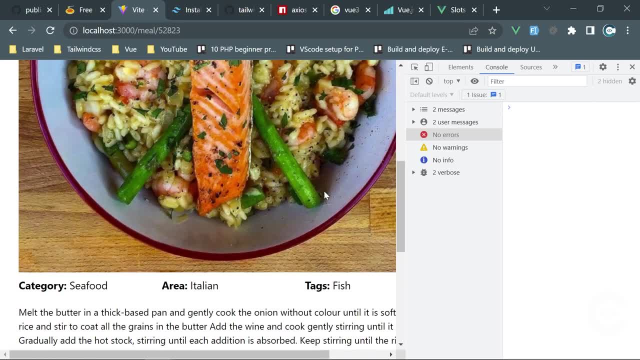 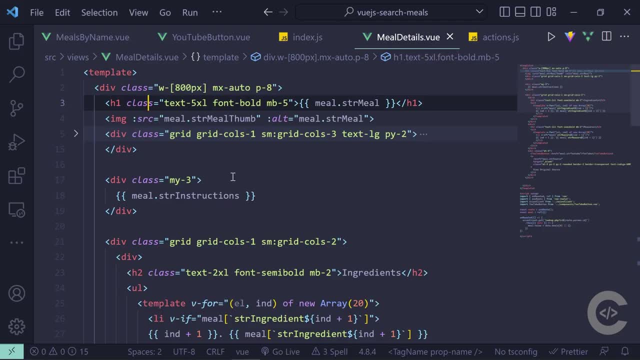 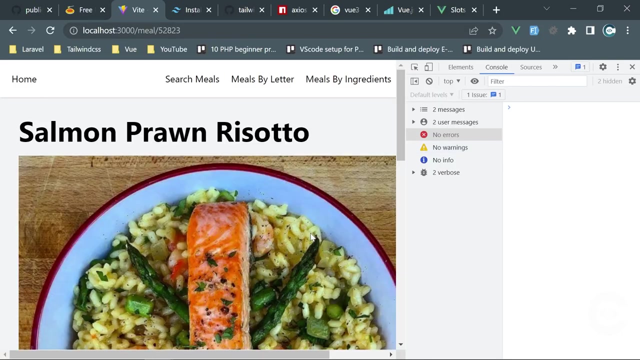 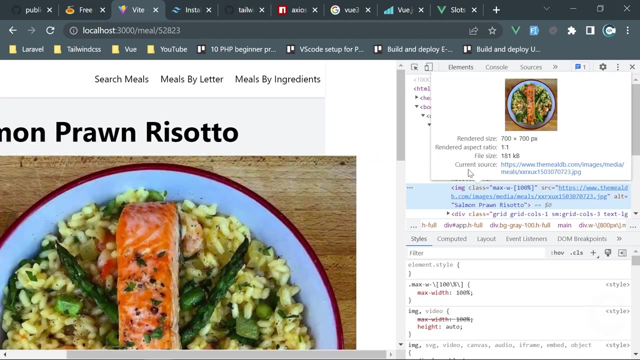 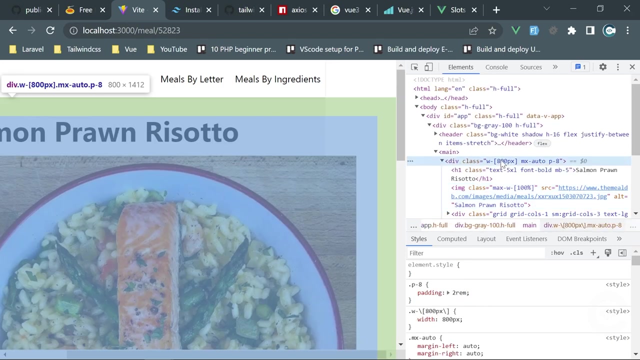 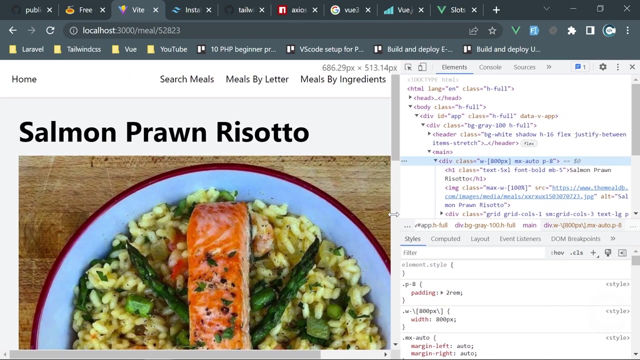 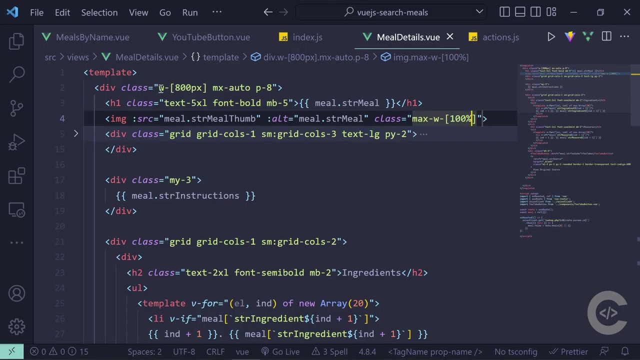 pre and reload the page and now let's see we should not okay the image is very large and we need to give this image max w max w full max w 100 maybe i don't remember this by heart so i think i can give it just 100 percent like this no it still doesn't work okay it has max with 100 percent but it does not uh-huh this is because of because of this width 800 okay well this should have maximum width of a 800 max w 800 and we should be good 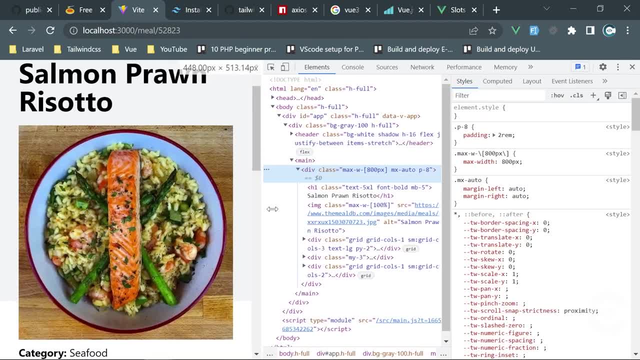 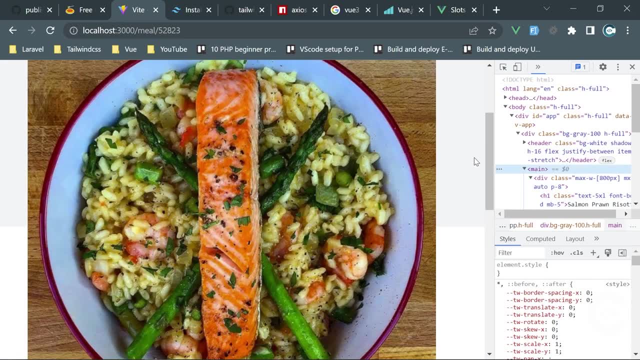 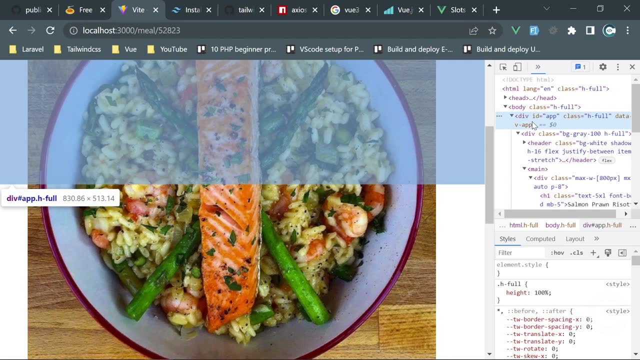 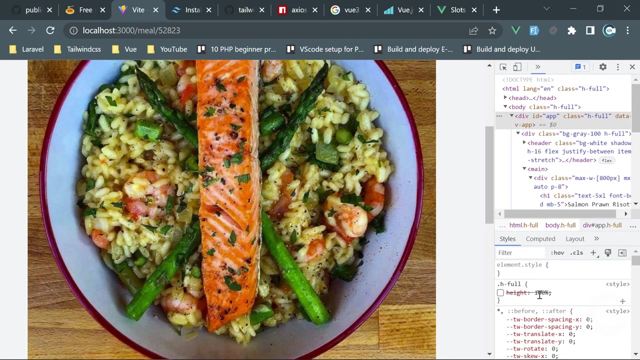 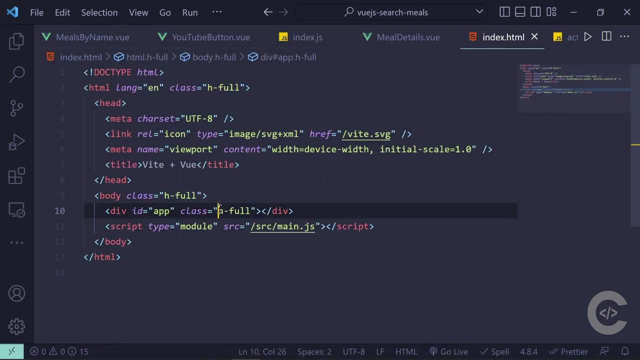 okay i think this looks nice what is why this color is different here's the main and we have up and the up has each 100 percent which is something we should remove probably or it should be mean h 100 so let's open index html and give it mean h 100 and we're going to add this to body and html as well 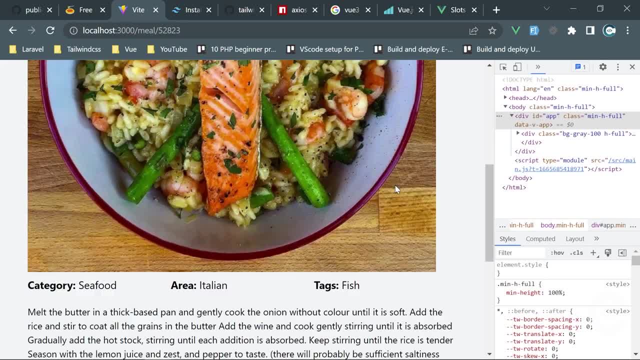 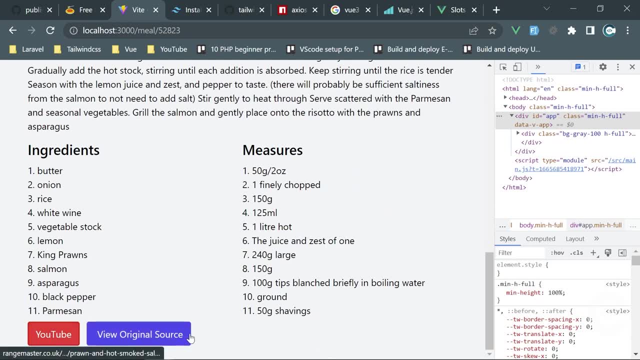 okay so here we have the meal detail page this is something still i don't like 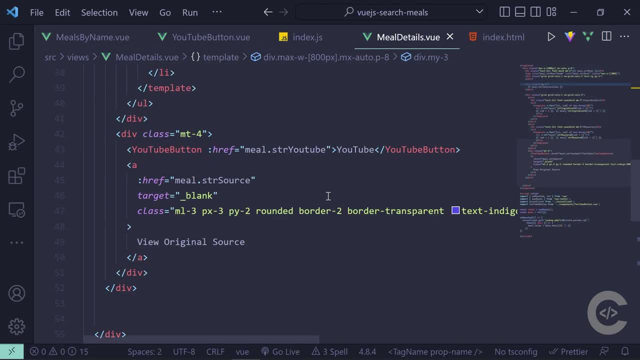 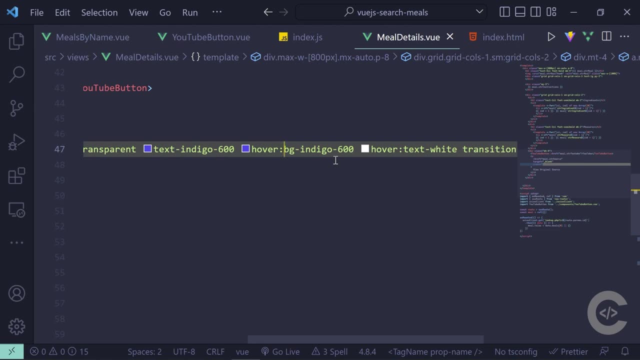 i'm going to quickly change it let's just give it text and not hover 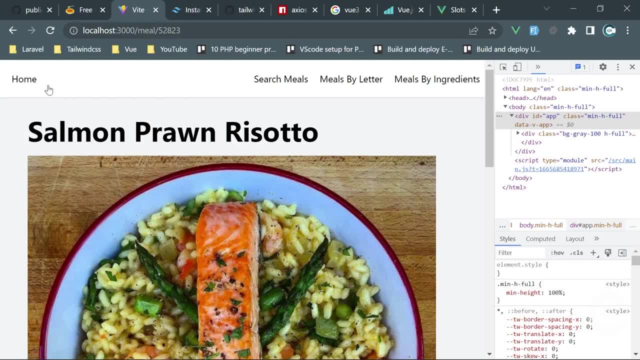 okay now i go back and we see these meals however the youtube 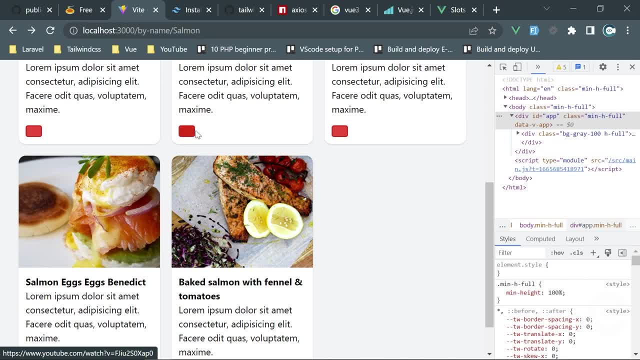 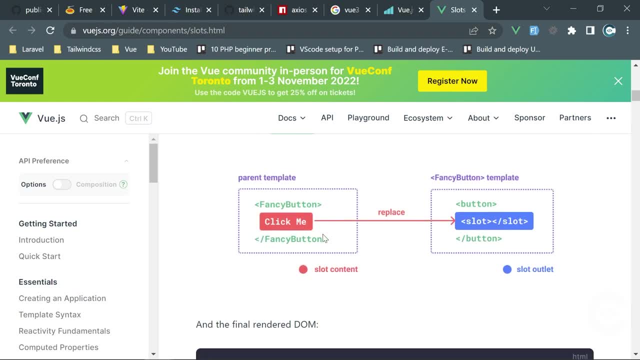 uh yeah this is something um we don't have default slot so we implemented uh slot but we need default one as well 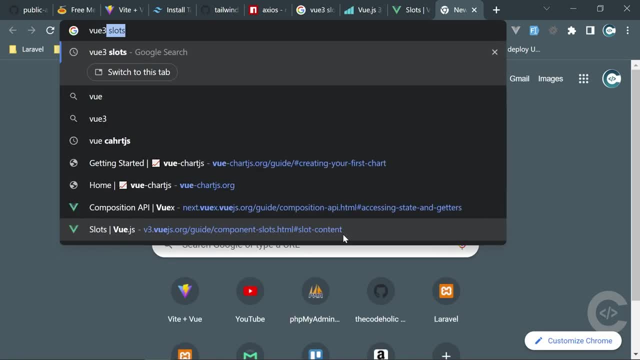 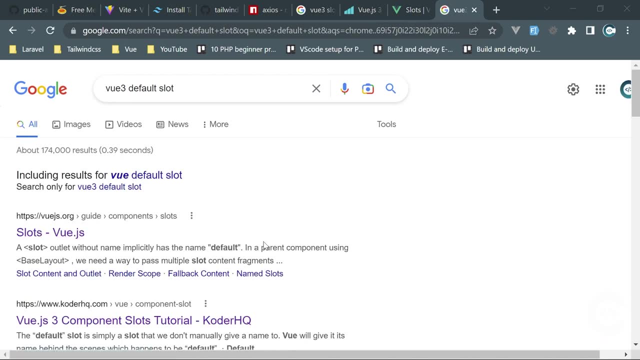 let me look for uh view three default slot i don't remember this specific thing yes i think 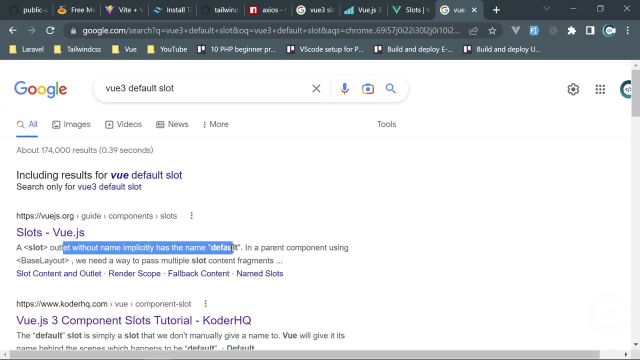 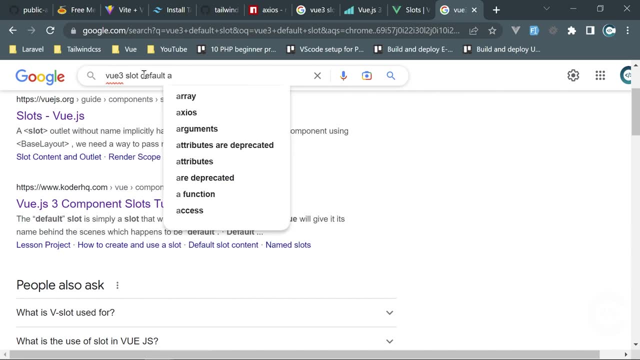 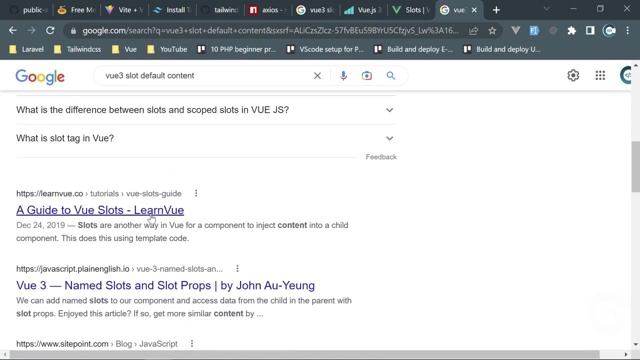 the slot outlets without name implicitly has the name default view slot default value or default content this is i want this is something this is something we have set here 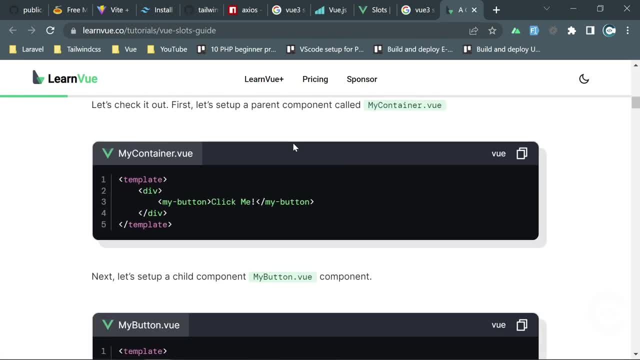 so for that this should be the default content you see this is a default value is set to default content we have the slot we have name slot header and content 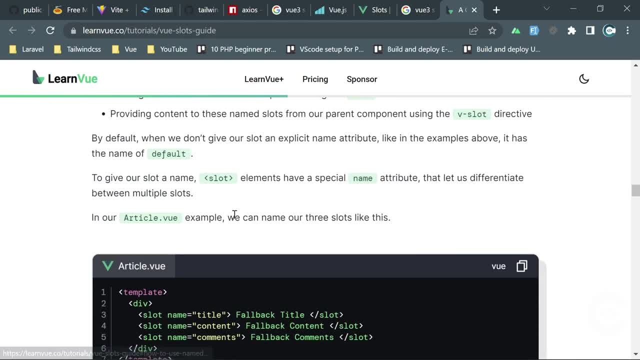 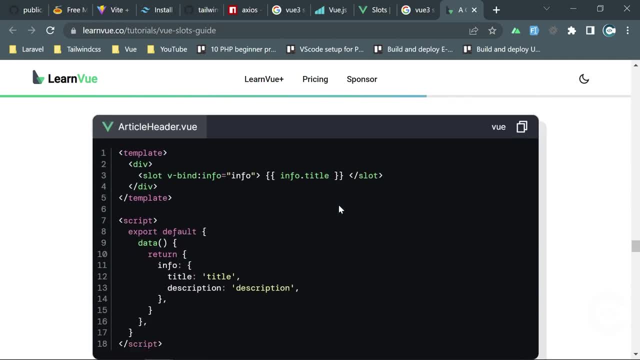 and what about the default okay this is something this is something which i am not interested 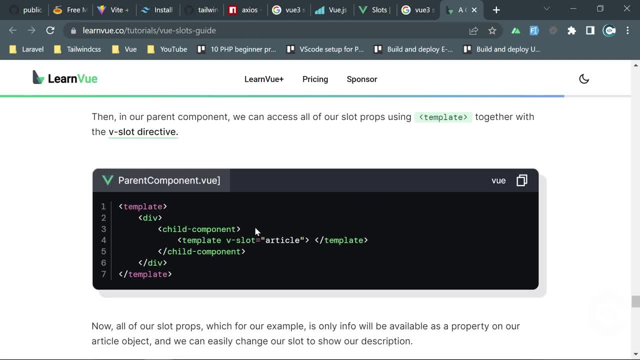 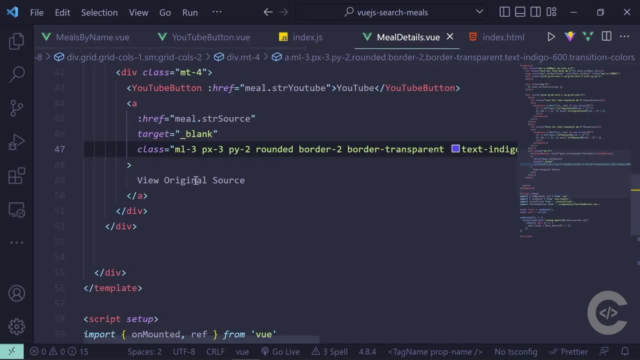 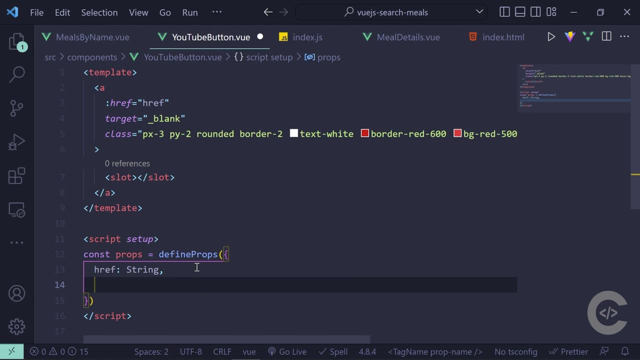 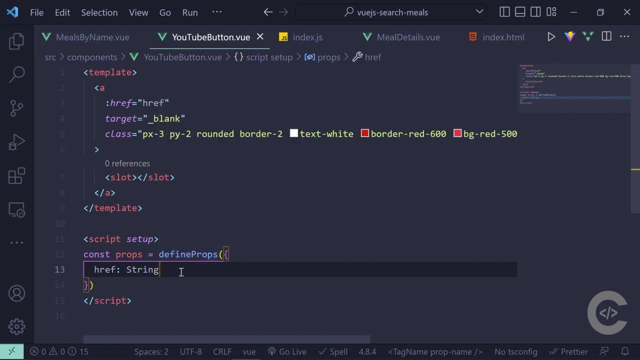 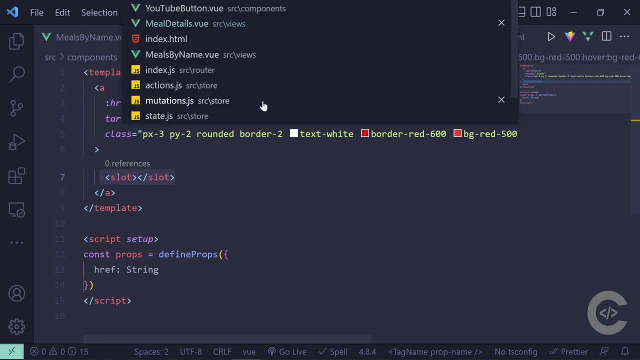 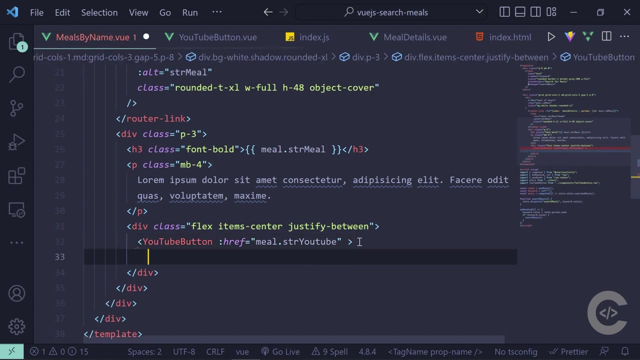 well this is something which is which will not give us what we want if we want icon to be provided inside this meal by name from from here so in this case we can provide a youtube right here 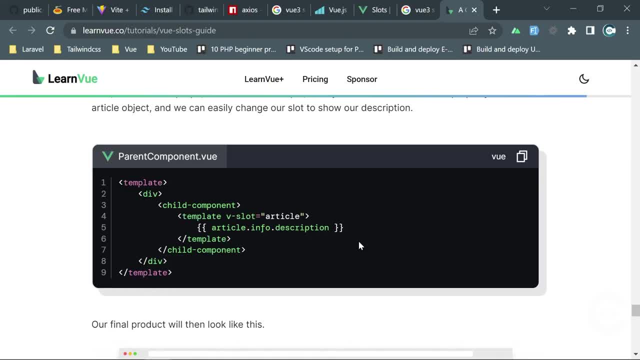 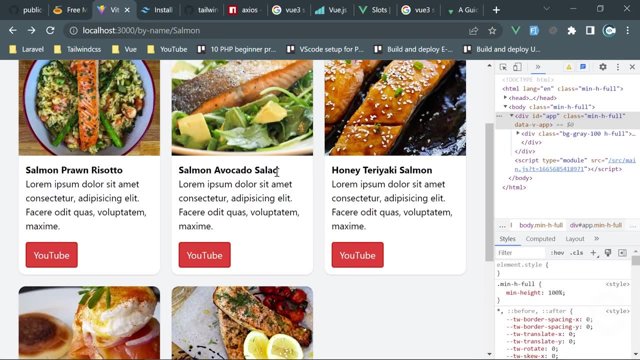 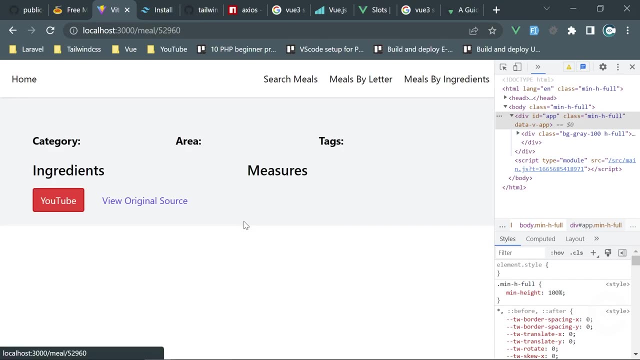 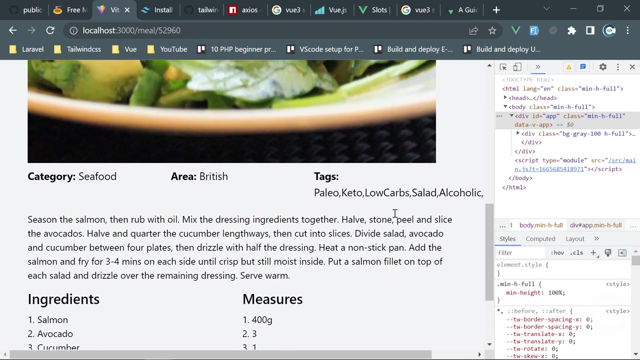 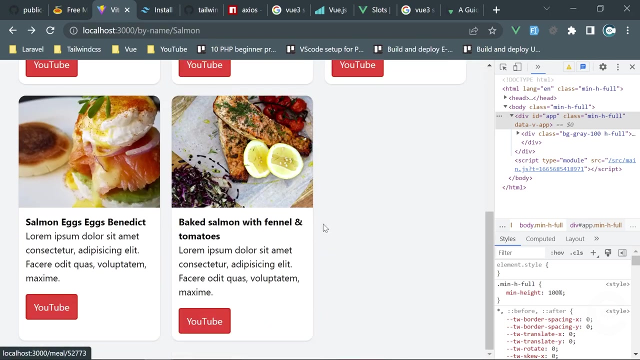 I'm going to find out it later how to have this default value all right now let's let's have a look so we have this youtube button however I think the button is very large not sure why but I'm going to leave it do not touch it okay click click the second one nice we have a lot of tags right here let's open the other one okay this is not bad all right we have like two more pages 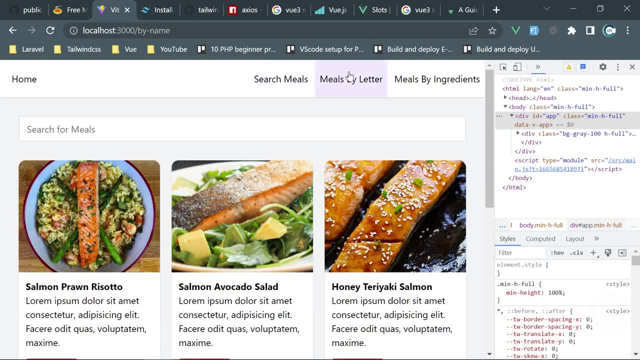 but I think because we have the listing and we have the details page that's going to be very straightforward and very easy all right so if I now this is something I wanted to mention if I 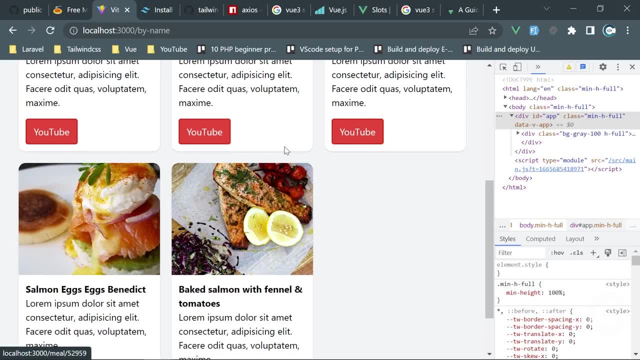 now click these search meals I see those five you 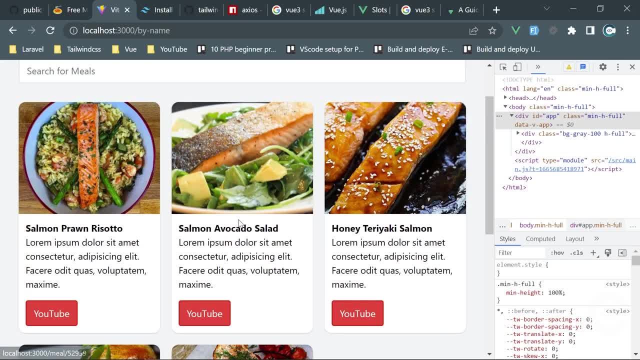 now meals because they are saved in the view x okay and those are basically loaded 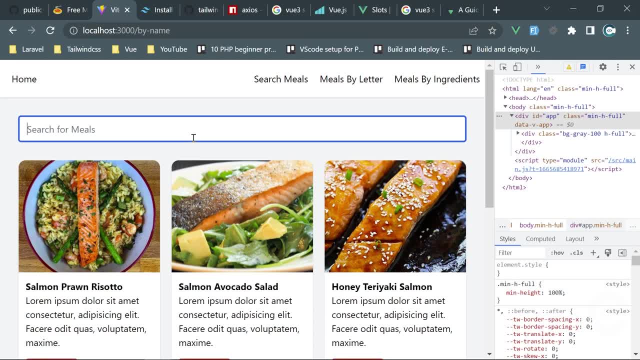 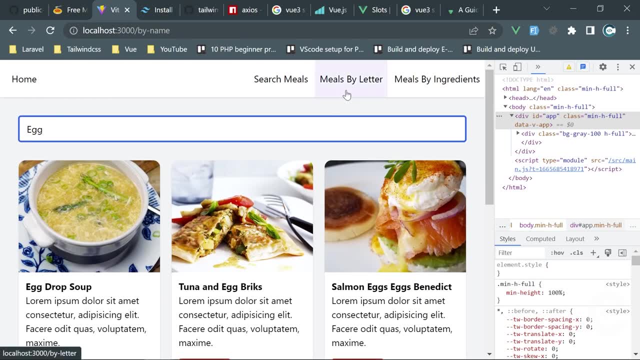 and we can if we just type something else like egg for example we will see egg recipes of course now let's go in the meals by letter and implement that but before I do this 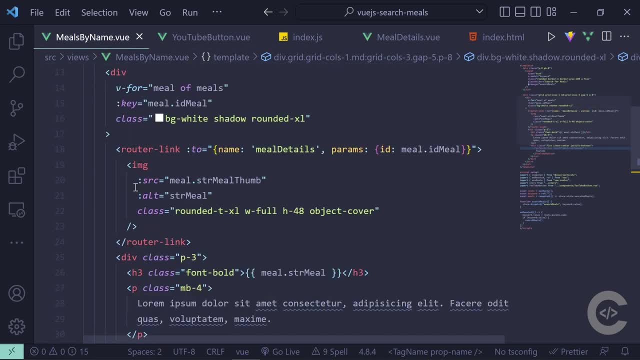 I want to do a few more things meals by name here we have this each meals by name 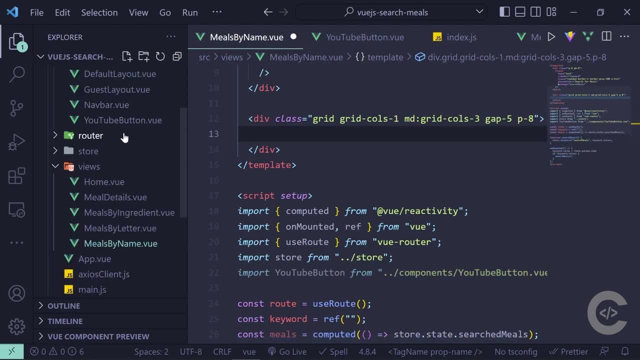 and I want to extract this and put in its own component so in the components I'm going to 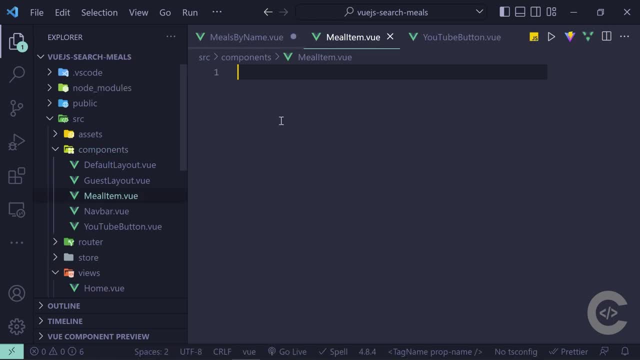 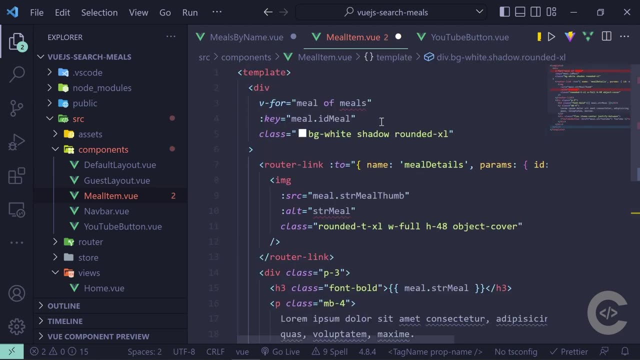 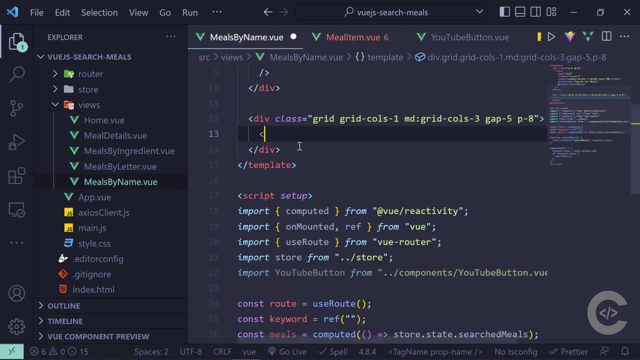 create meal item dot view and create template right here paste everything and we have a couple of props this v4 can be taken out from here and put this meal item right here 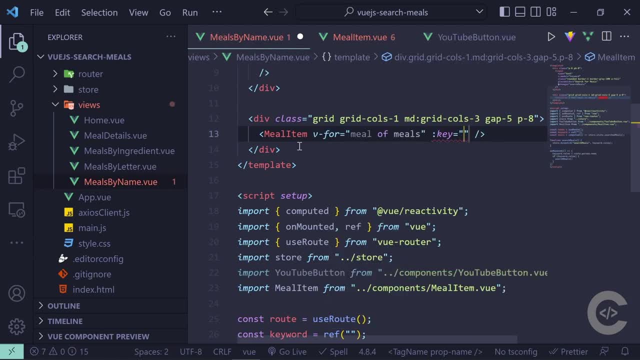 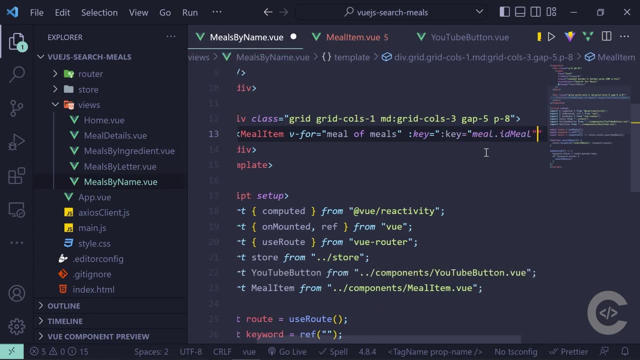 v4 and key can be added id meal here as well let's take this key oops 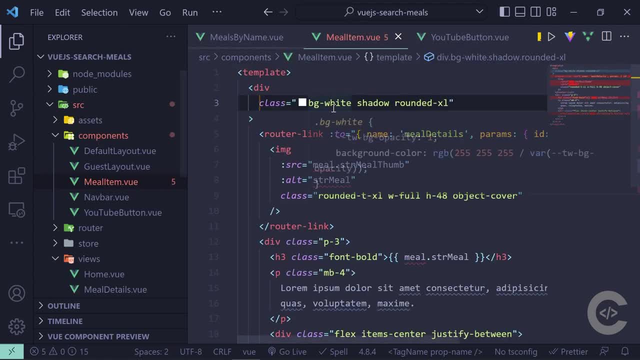 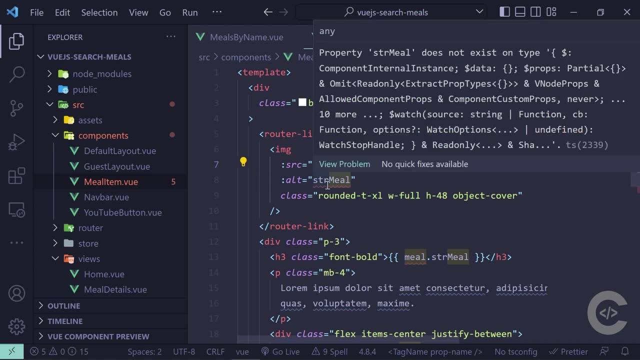 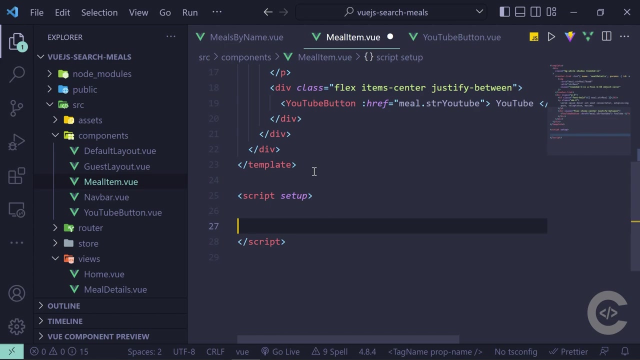 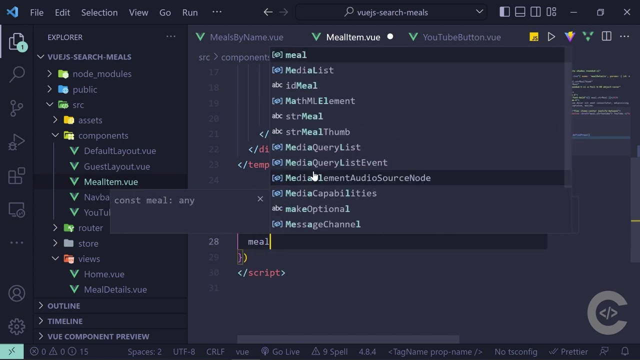 however we will need these colors we will need probably a single prop which will be which will be meal so let's create script right here with setup attribute and and const props let me destructure the props and take meal and that equals define props and we accept meal which needs to be object 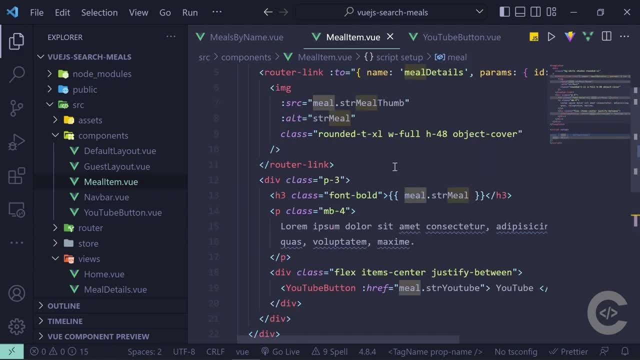 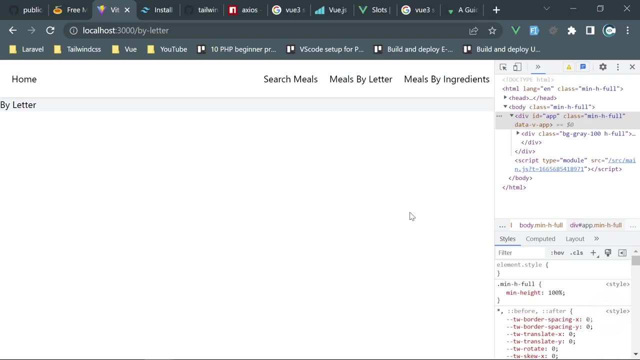 all right so now we have this meal and i am going to just fix this bug meal dot str meal and everything should work in fact if i go on the home page search meals and i think 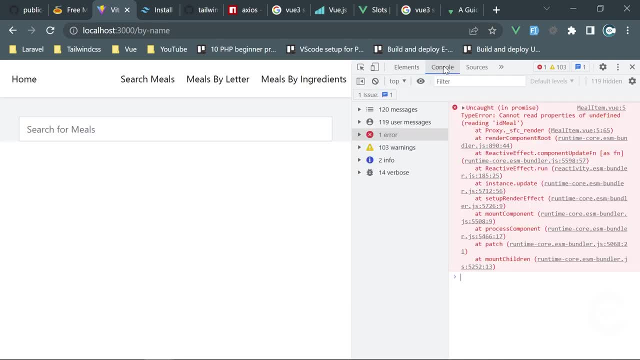 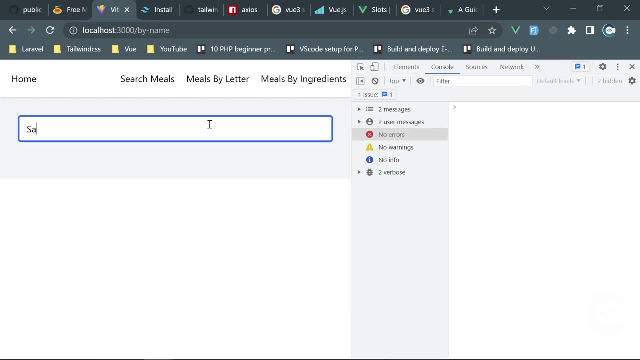 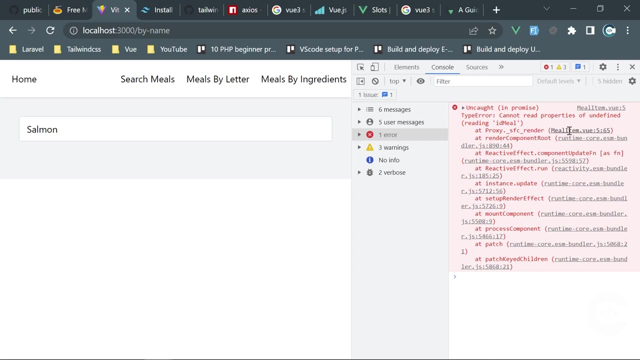 we have an error id meal let's reload the page okay let's type salmon okay country properties find to find id meal meal details meal id meal okay let's go to the home page search meals and i think we have an error ID meal let's 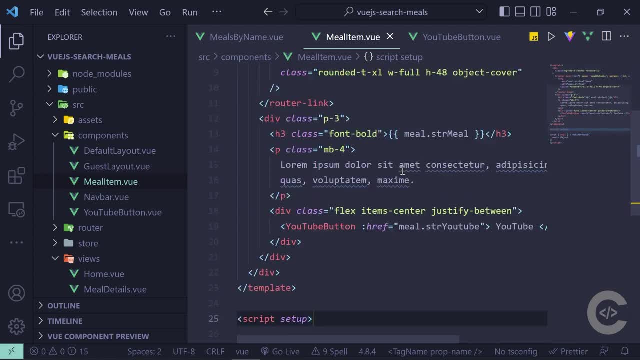 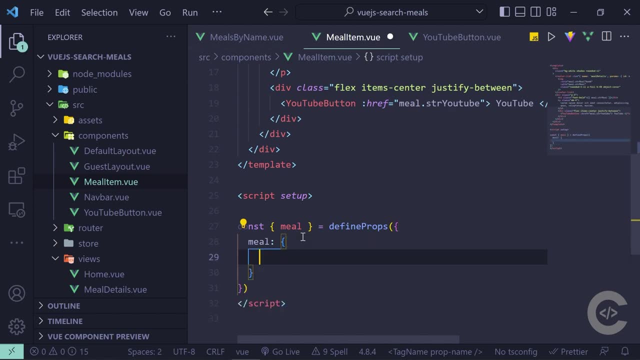 right here meal id meal okay what is this meal i think we don't pass meal let's make this meal required required true and then type equals object in this case we should see a different error 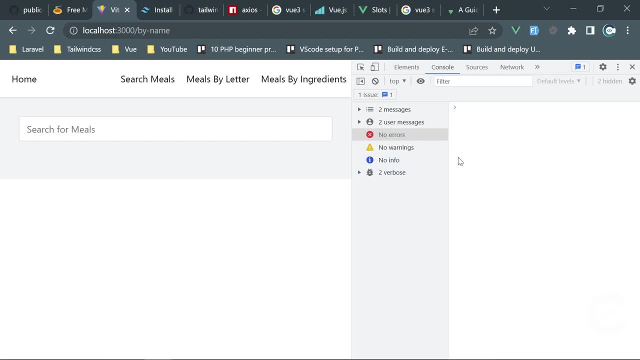 you can't read properties to find a fine reading item let's reload the page let's rename it and then start putting it on saying we please we will not tell you 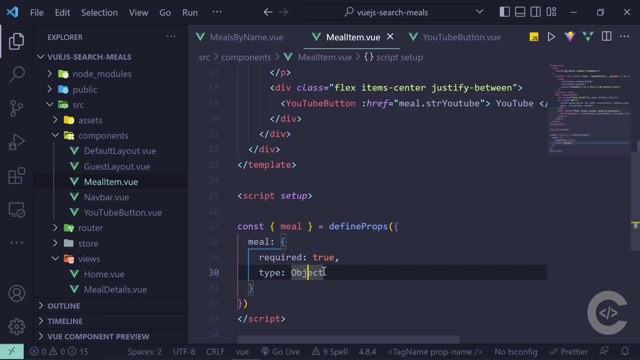 we lived here ok so i don't know why 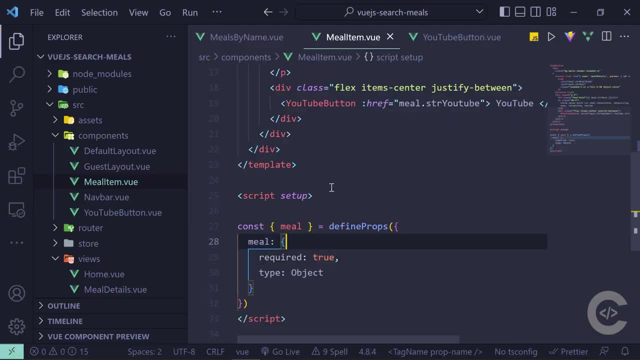 but uh it doesn't tell me that the meal is required but i know the reason right here 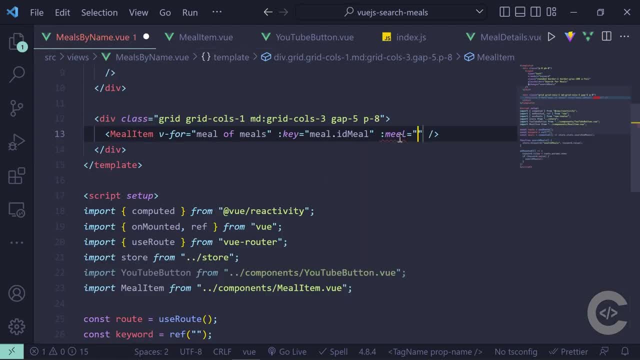 let's collapse everything right here we need to pass meal equals meal just like this 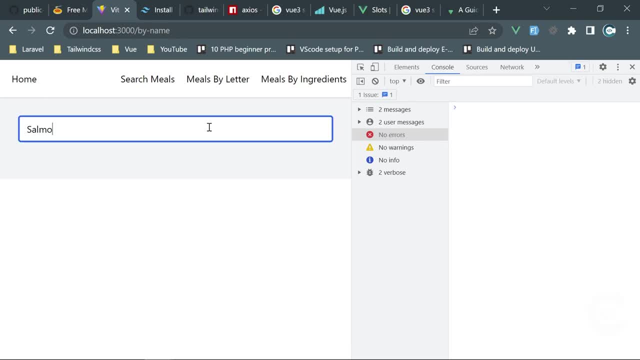 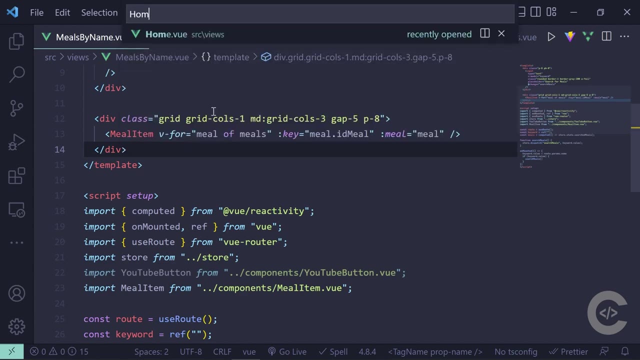 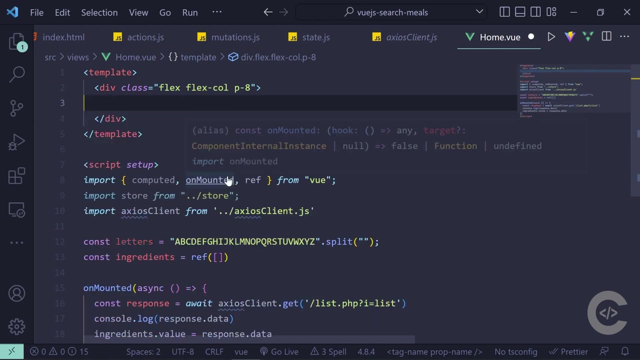 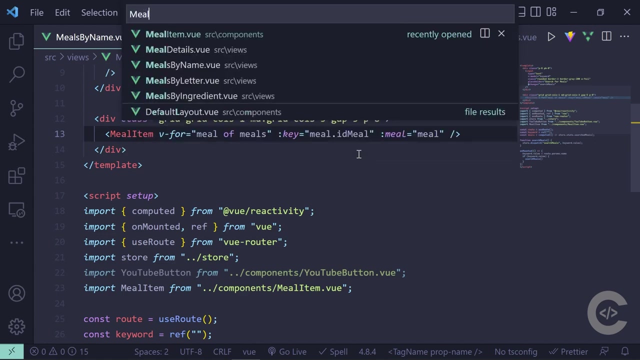 and if i hit the enter let's see salmon hit the enter here we see all the salmon receipts let's go now meals by letter and this is a place we're going to render this following letters so if we open now home page and if i just take that grab that and we need to open meal by letter and i'm going to paste this here like this 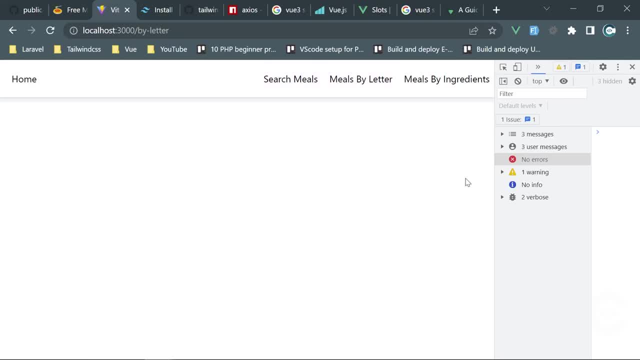 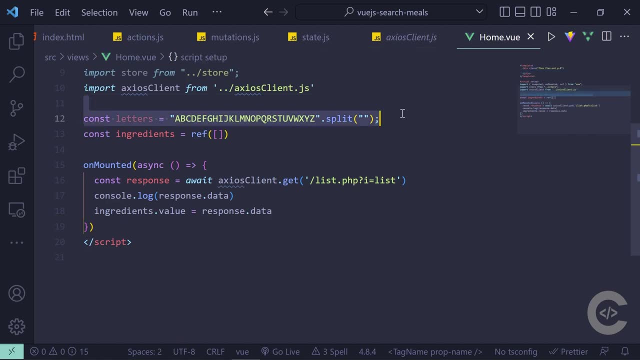 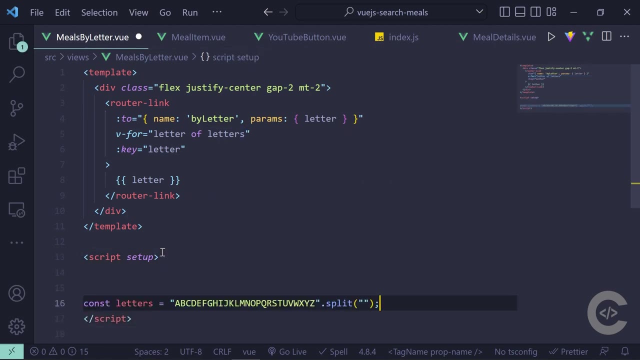 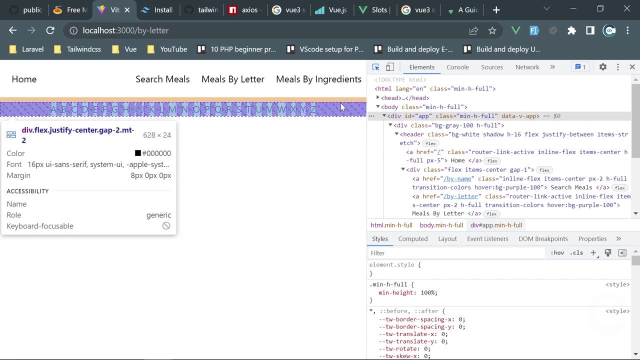 meals by letter below the page we don't have letters so let's go in home page and take these letters and put them right here okay we see those letters however again the background is some kind of a blank space and we need to close that and go on the homepage and take those letters and put them right here okay we see those letters however again the background is?! is mean age 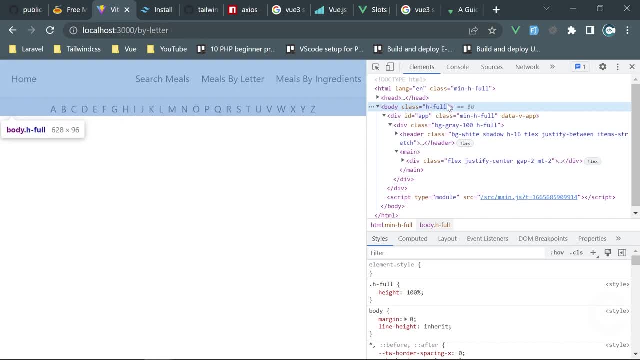 it should be age 100. 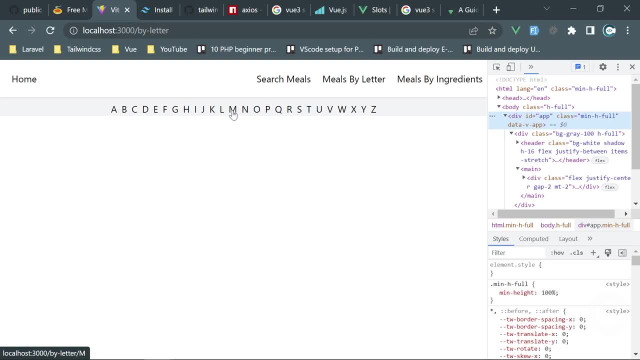 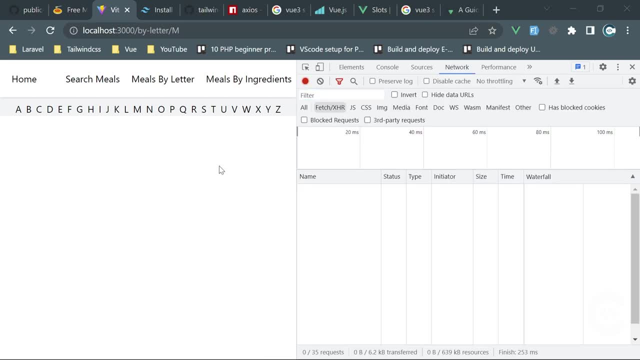 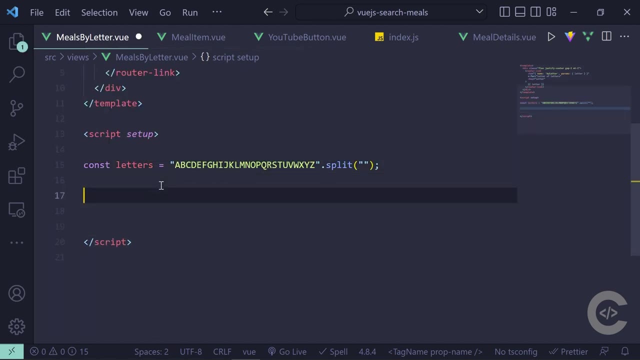 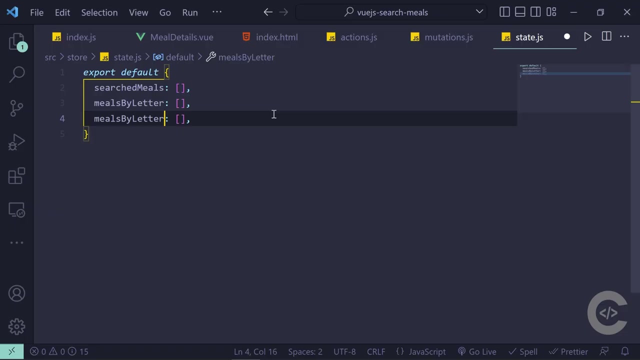 okay let's skip that let's skip it so now i'm going to click m and the request should be made to fetch all meals starting with m so meals by letter scroll down below and we're going to save this in the vuex so let's start now open state and we have searched meals i'm going to duplicate this and call meals by letter let's duplicate this third time and meals by ingredient meals by incredients ingredient okay we have now you have now 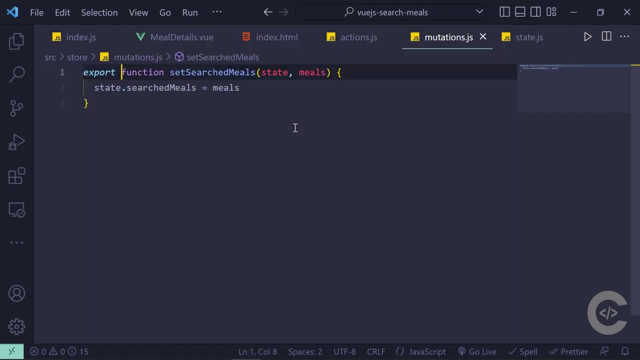 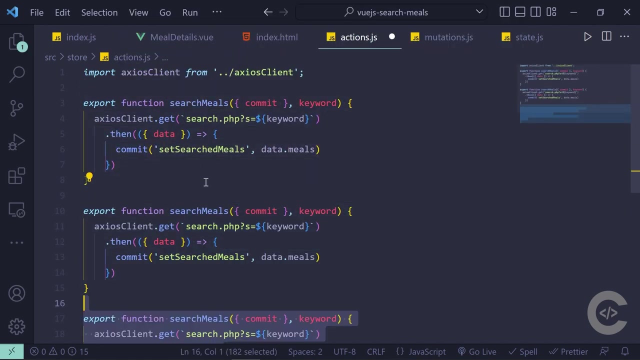 state now let's open mutations and let's duplicate this and this will be set meals by letter we accept meals and meals by letter equals given meals and that's going to be set meals by ingredients and that's going to be meals by meals by ingredients now if you open actions we need to duplicate this method two times 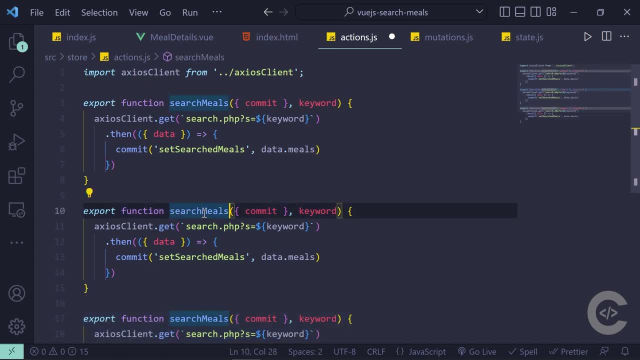 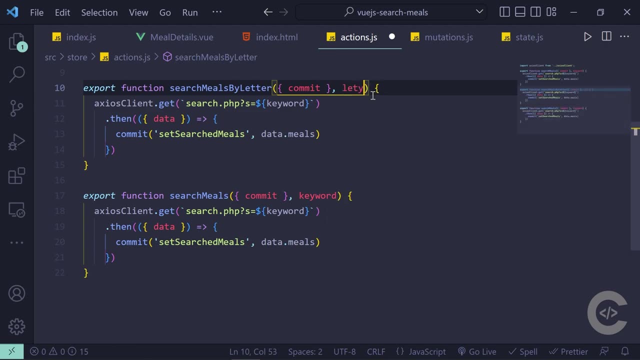 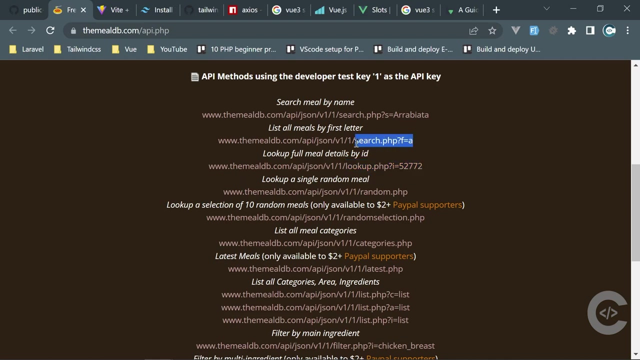 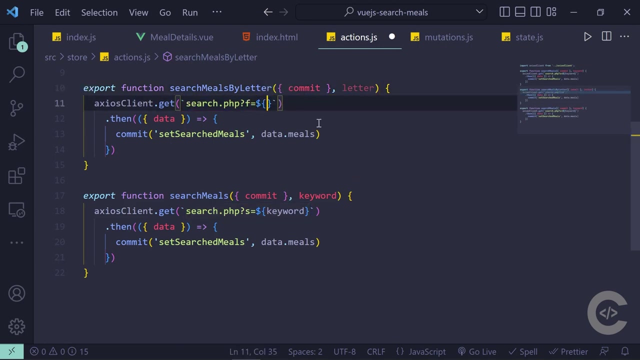 that's going to be search meals by letter and we're going to accept right here letter letter and what is the endpoint and what is the endpoint the endpoint is this so i am going to replace it and for the letter we are going to have 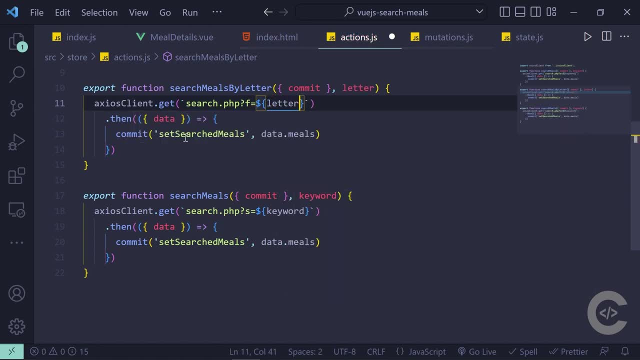 a letter we get this data and then in the mutations we have set meals by letter so we specify it right here data meals and implement the last one search search meals 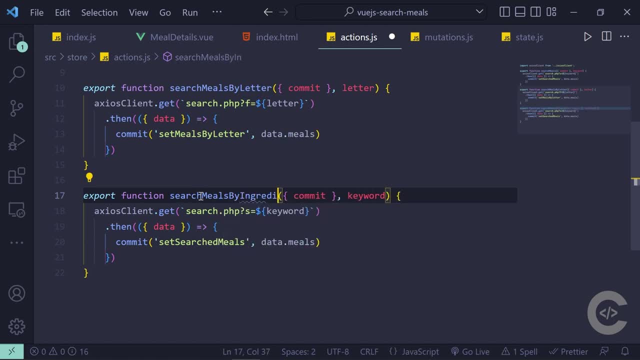 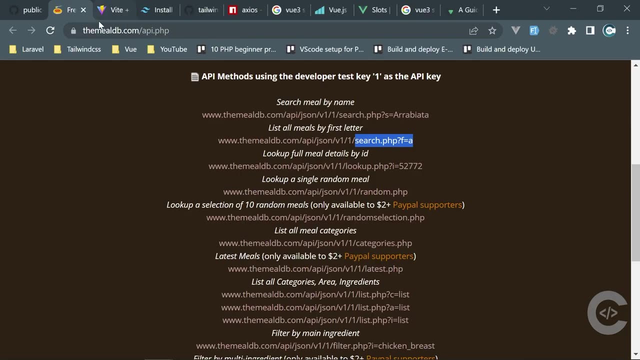 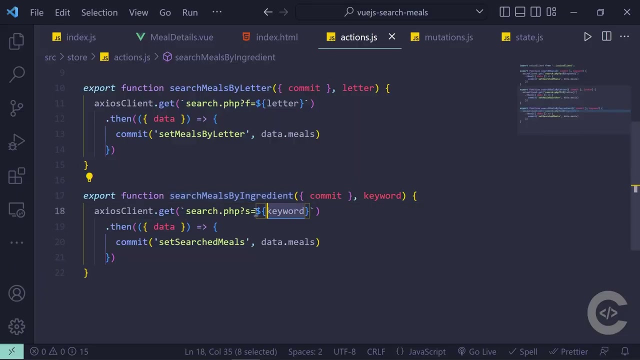 meals by ingredient ingredient okay what is the url for that the url for that is this so we put this right here 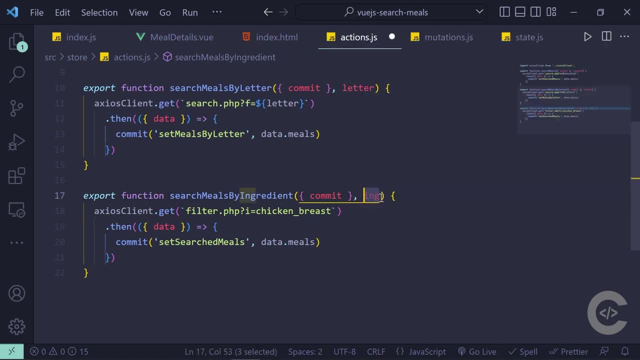 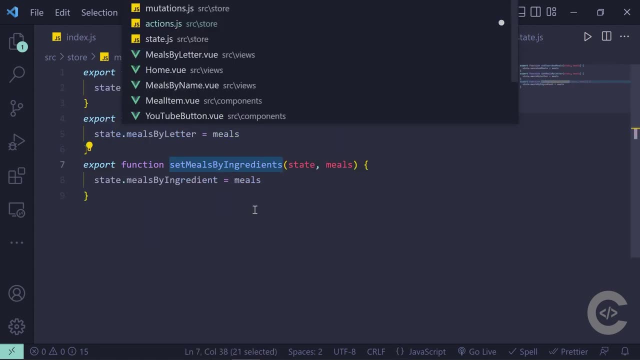 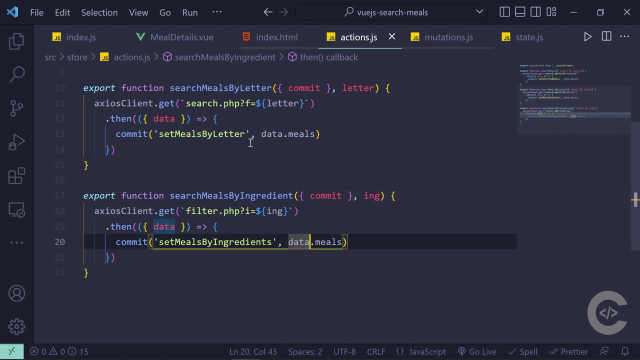 this is going to be ingredient and i'm going to put this like this and this then we're not going to have to do anything else so we're going to have to do this we're going to set the uh call the mutation set meals by ingredients and we pass data meals and 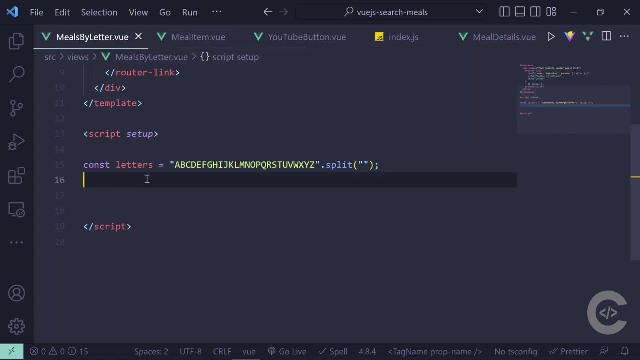 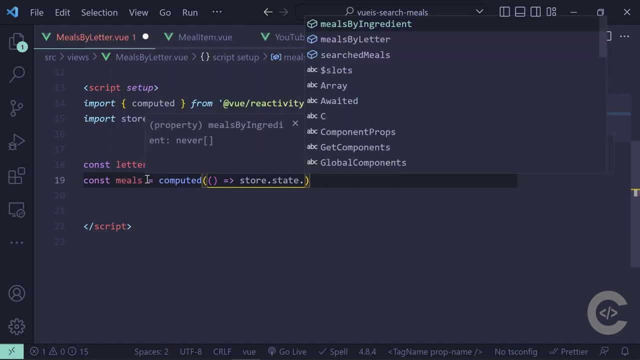 using this in meals by letter we can already access to meals const meals equal computed store dot state dot meals by letter all right so we take these meals 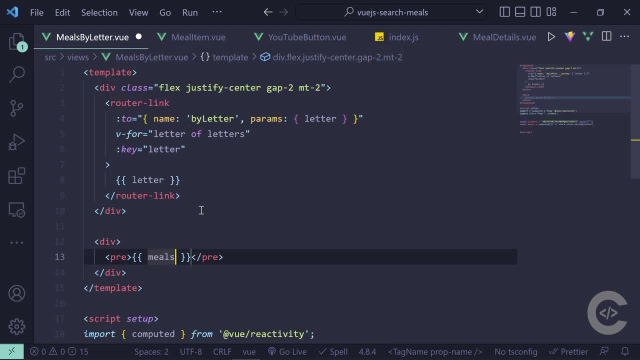 and let's output them right here 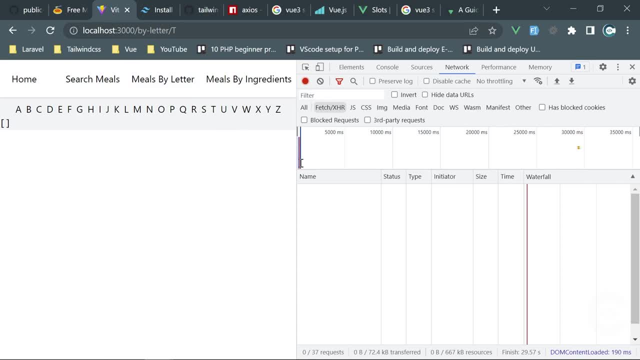 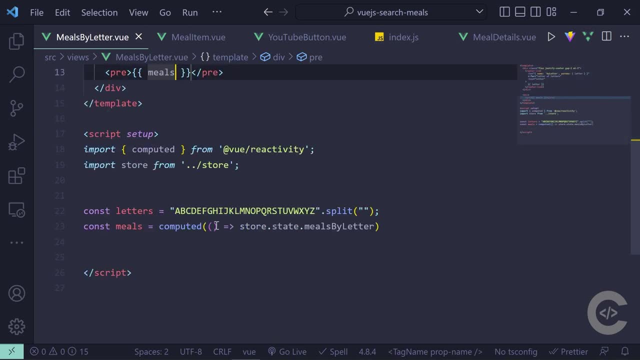 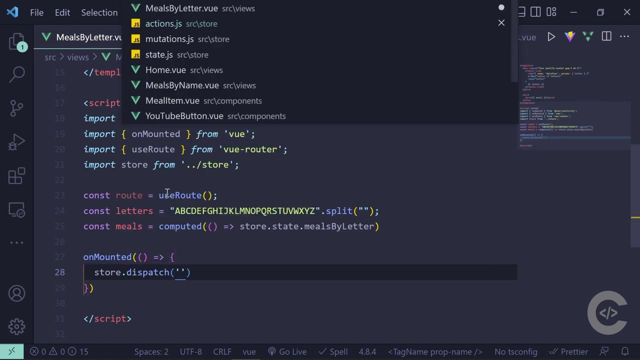 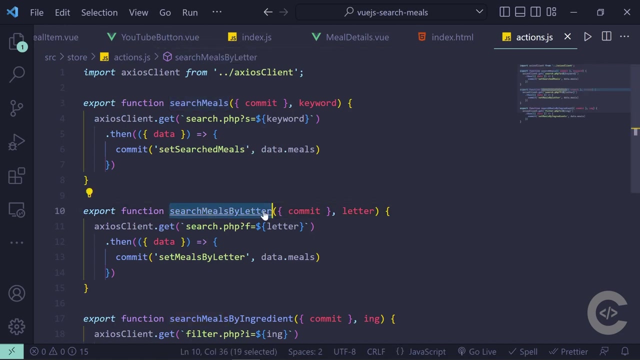 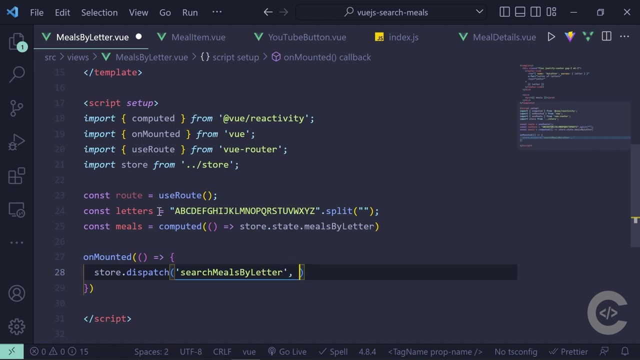 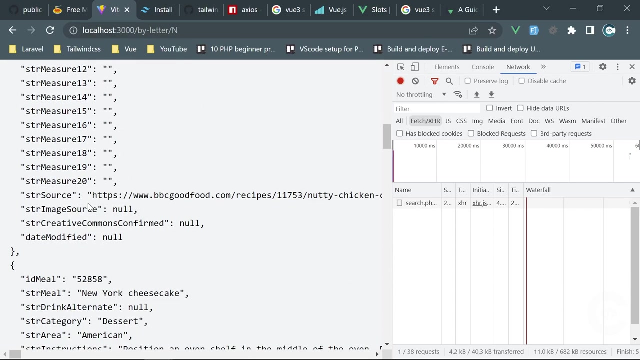 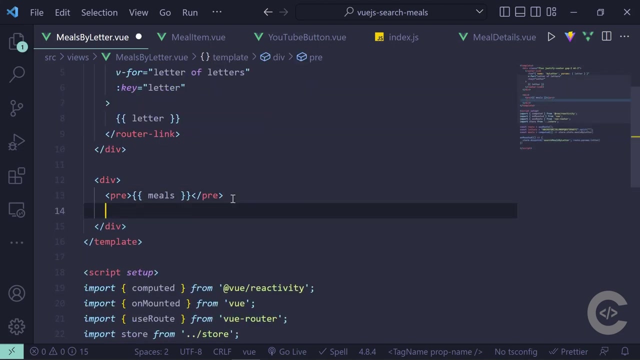 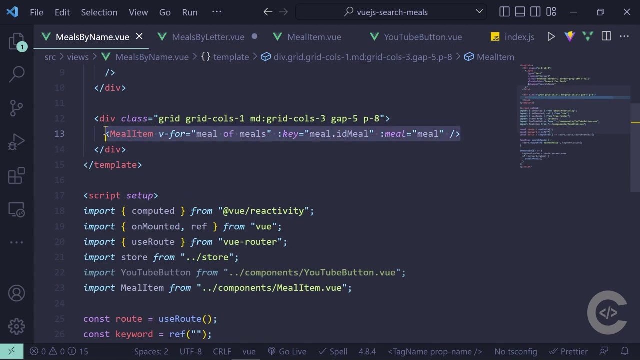 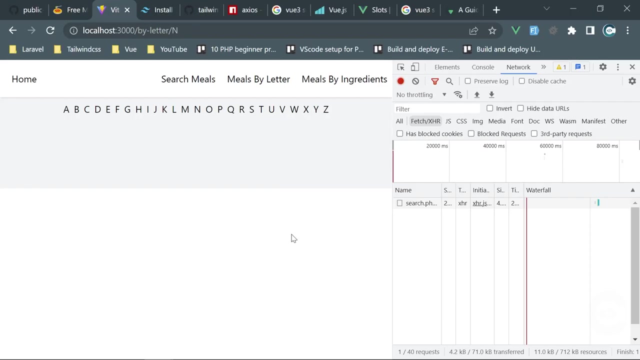 so click on t for example i think the request is not made okay the request is not made because on mounted basically we need to take the current root letter so we need const root equals use root and then down below uh const let excuse me we are gonna use store dot and dispatch what is the action the action is search meals no search meals by letter okay we're going to dispatch that and we're to pass the chosen letter that's going to be wrote dot params dot letter so i save this and here we have all meals all right how many meals do we have like two or three now we can iterate uh for like we have we have these meals by name and i need to take this basically copy this part and put this right here saved it and reload the page the request is made response is received data is not rendered 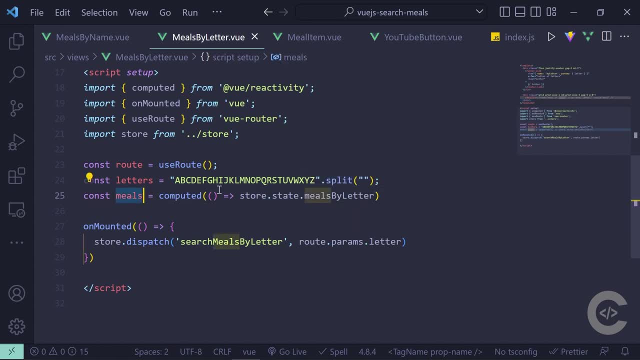 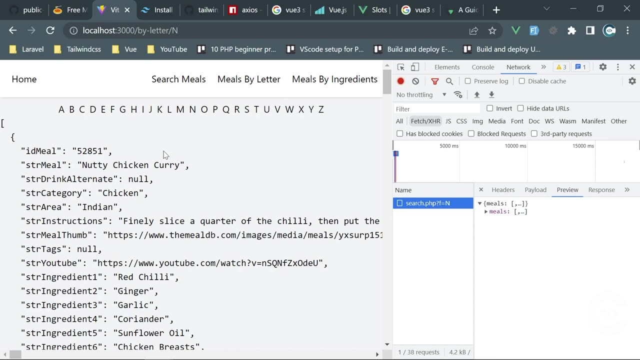 why let's see what is meals meals is an array 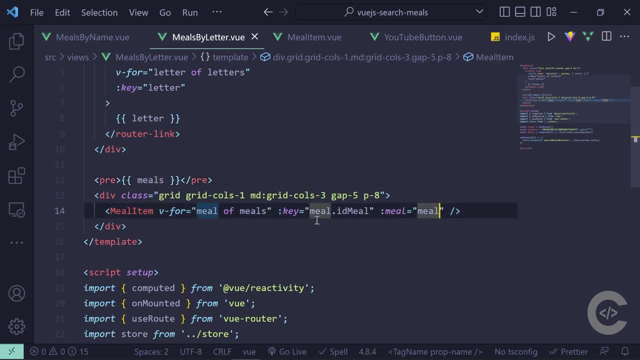 okay we iterate over meals we pass meal we have meal id why it didn't render the data 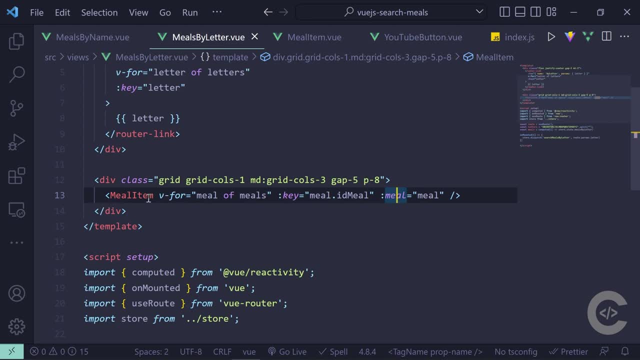 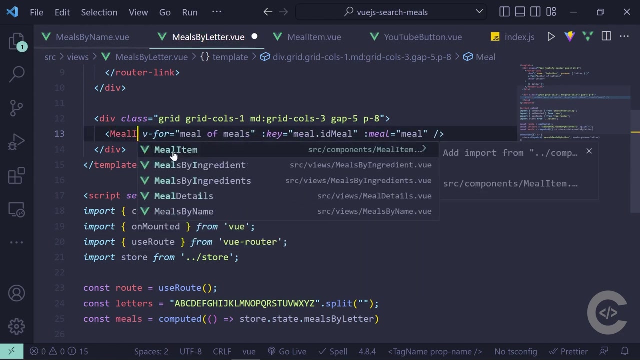 okay what is this colon meal we take the meal and give it right here let's open yes this meal item is not imported okay this is the problem meal item hit the enter that was imported save that and here 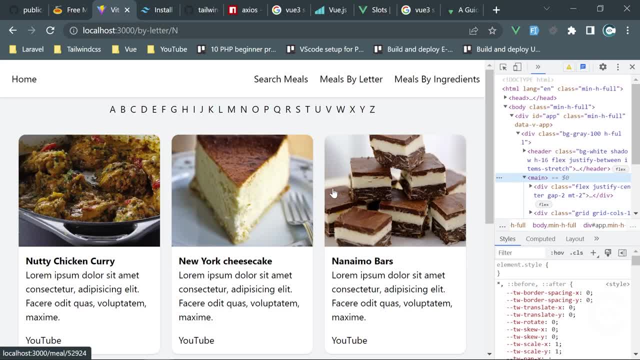 we see so those are meals meals by key meals by key 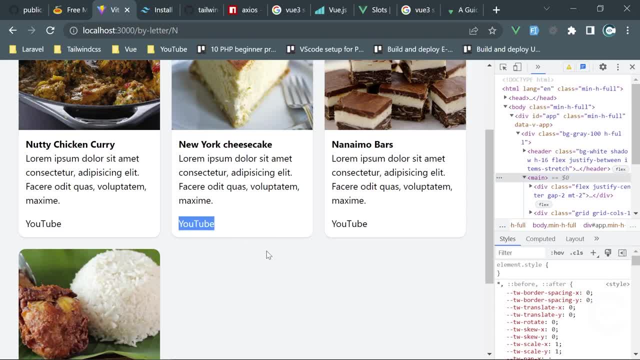 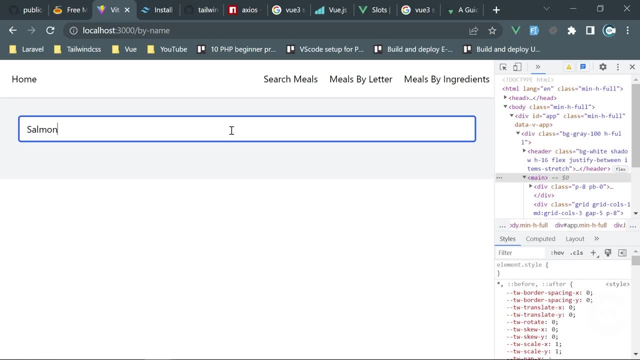 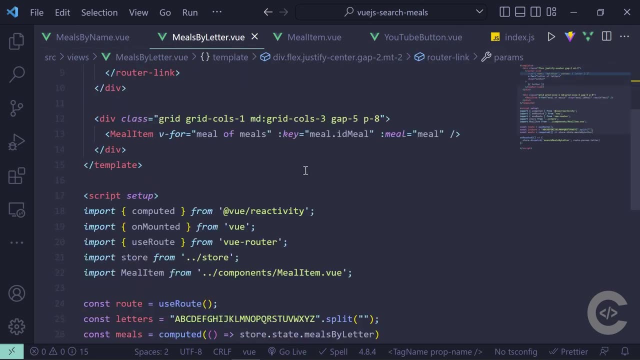 the YouTube the YouTube element is not displayed properly is it displayed for search by meal like salmon hit enter no we have a broken that we go in the we 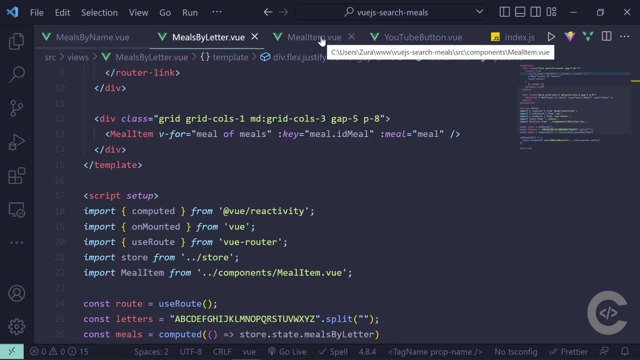 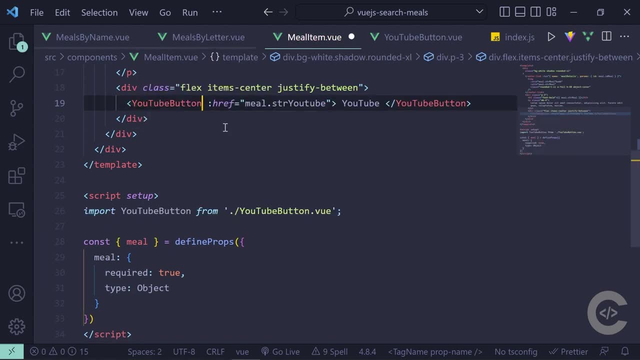 are doing to go in the meal item I think we need to just import this so if I just delete this and start typing this code will automatically import that for me so 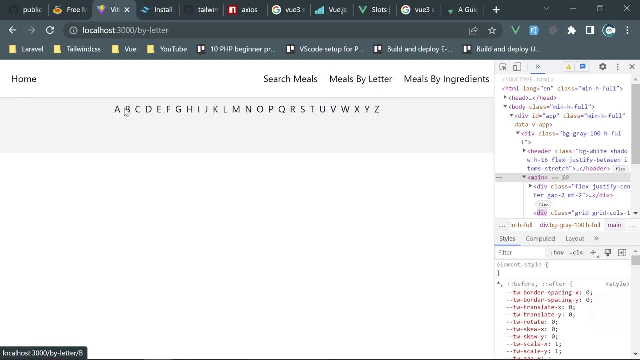 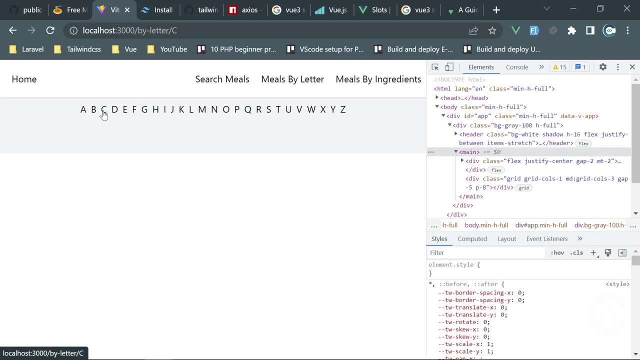 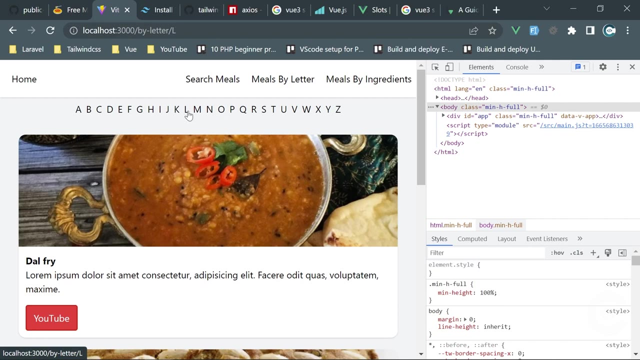 I save this and it's now visible meals by letter let's click a okay doesn't load anything B C D let's reload the page however okay whenever you click so 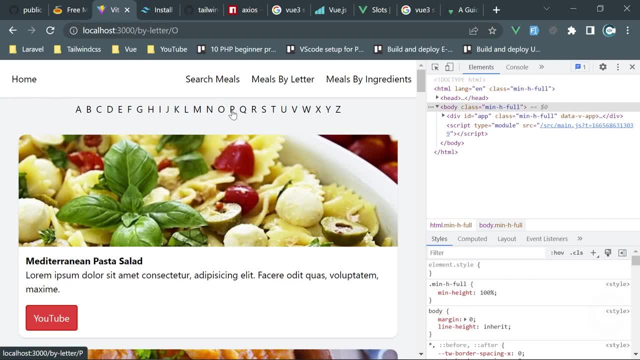 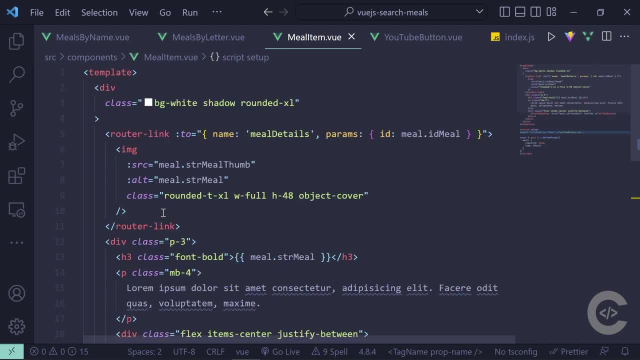 when you reload the page it works but whenever you keep clicking it doesn't do anything well because we don't listen to click and we don't listen to the route change 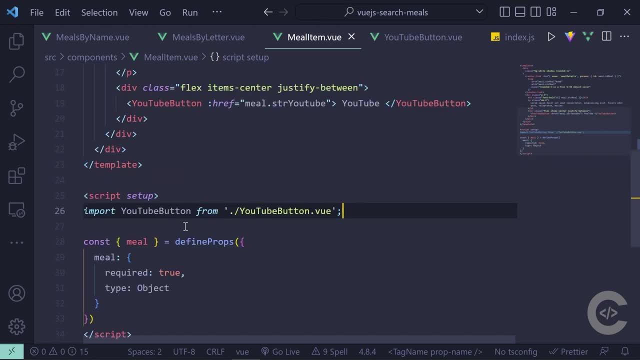 as well okay so I think the best will be to listen to the route change if we go 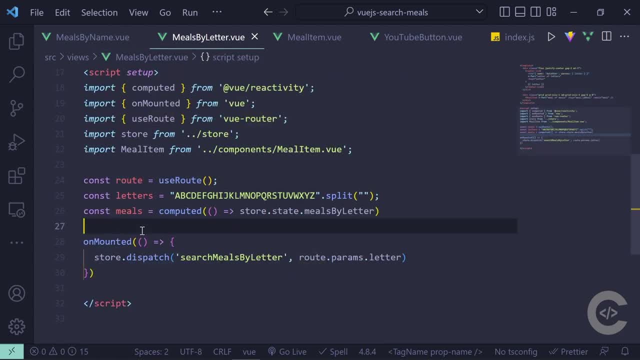 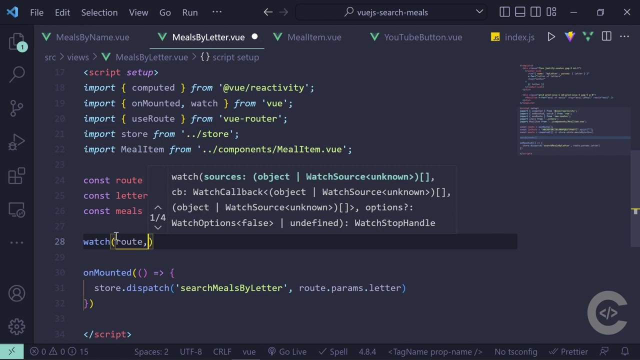 in the meals by letter we have this route and we can implement easily add a click click right here but I think we need to listen to the route chain so I'm gonna use watch right here and we're gonna watch to route current role 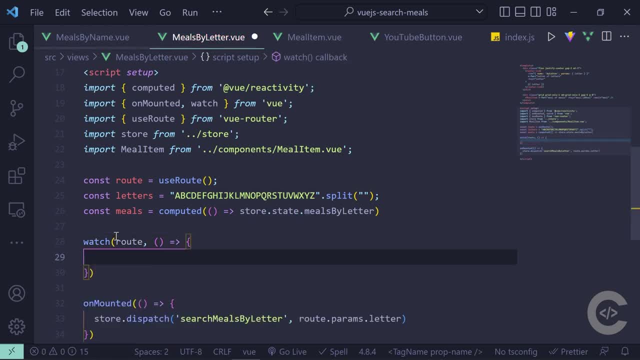 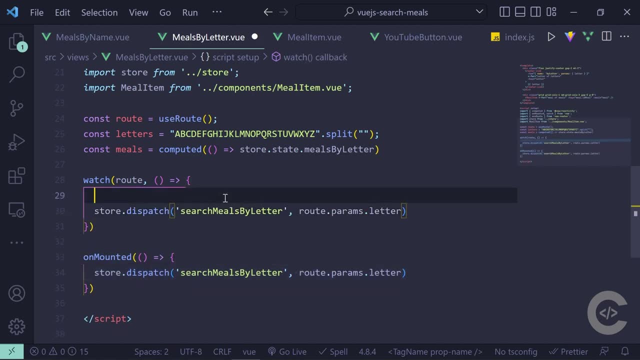 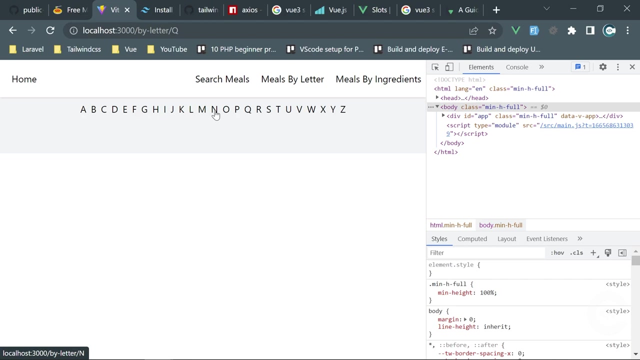 and whenever this will be changed i need to basically dispatch search meals by letter okay which needs to be imported i save this and click on n and the request is made imported oh 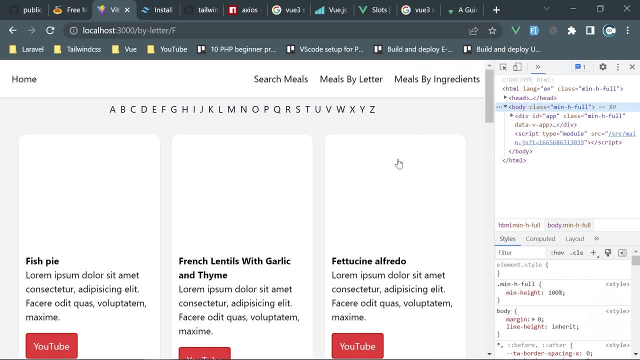 updated okay as you see now the data is coming whenever i click on those 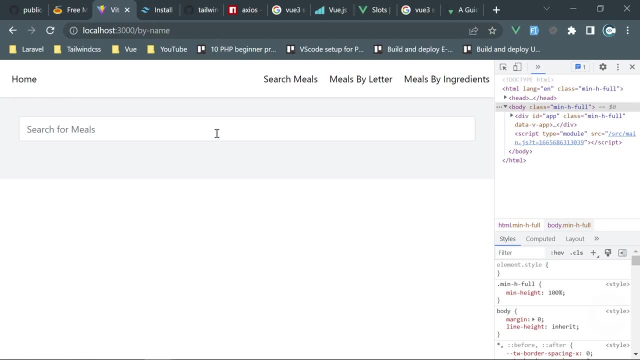 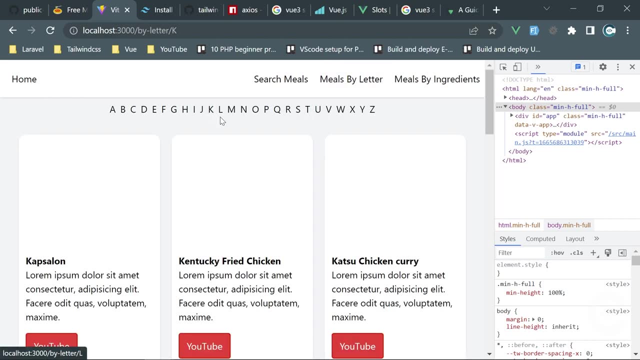 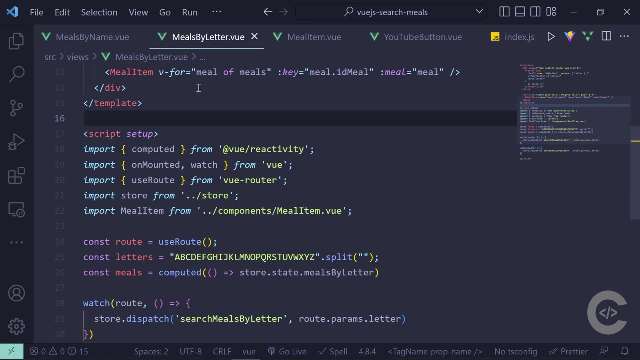 all right so we have search meals by keyword we have meals by letter as well and now let's implement meals by ingredients so right here we need to display all the ingredients meals by ingredients 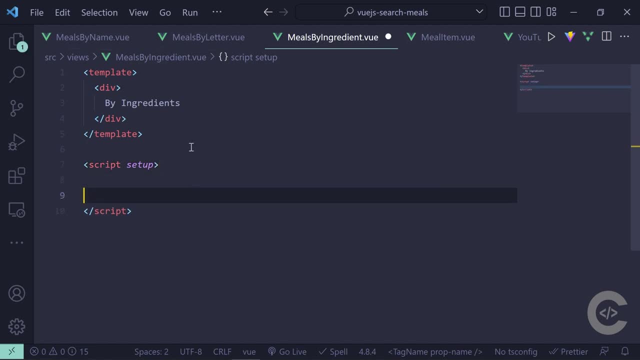 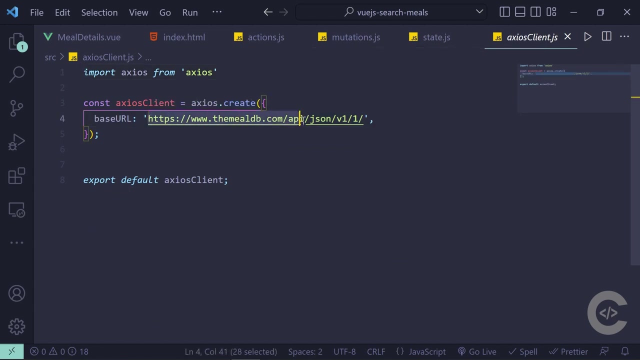 ingredients let's go right there and i'm going to make requests on mounted axios client however before i continue inside axios client i have this hard-coded url if you decide for example um to commit and push this if i decide to commit and push this it's not good practice to have on a 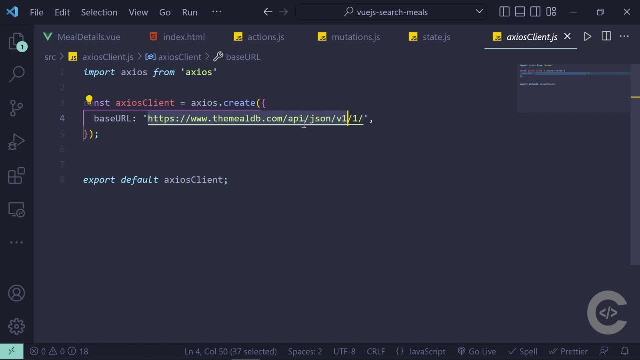 like production ready applications come this one to come it in pushed or to say it in different words ah this might be okay if all your coworkers will work on the same url however if you are using your own api something you are building on you should have this url in an environment variables in the .env file, in fact a vite 힘 this future developmentisión word.env and in produce enterprise 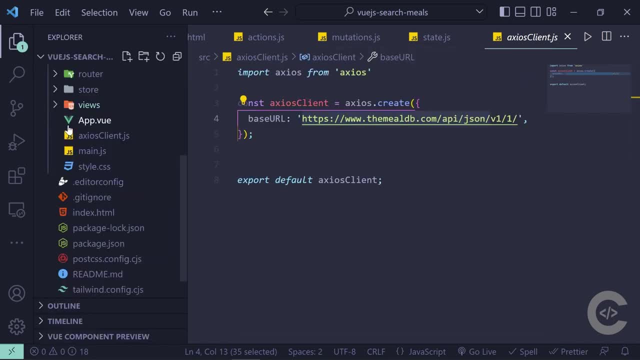 locals file in fact a wide and this future development underline so you can use this and video 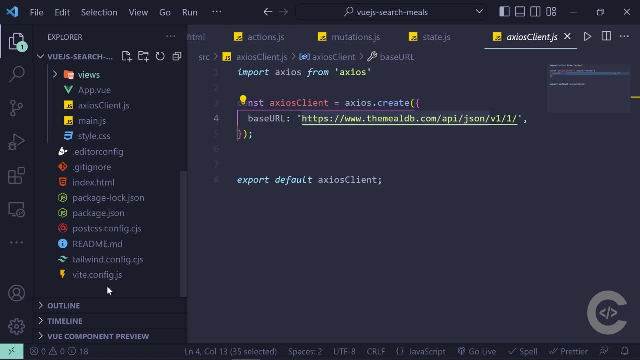 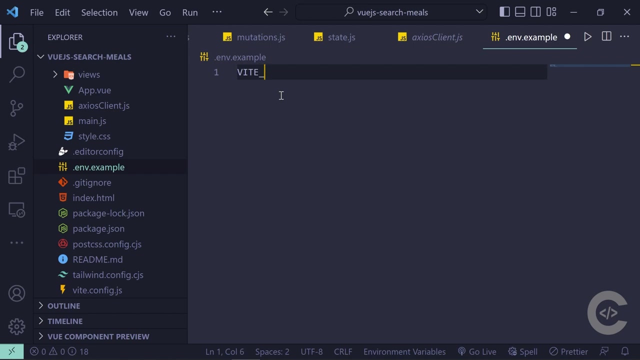 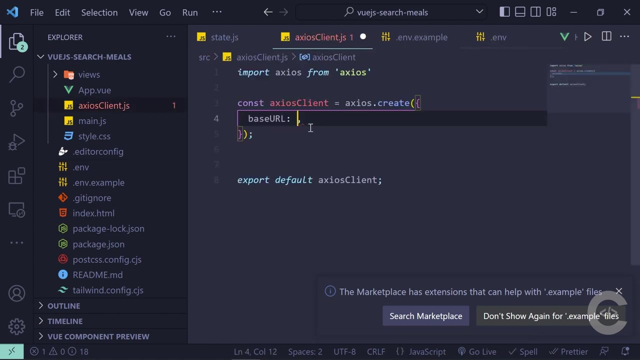 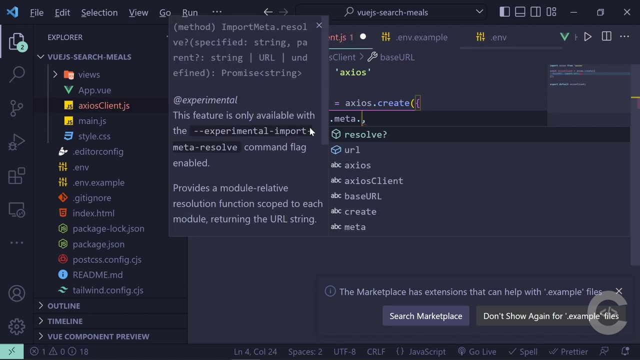 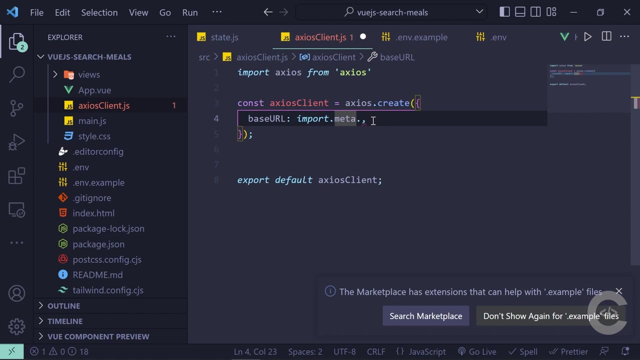 installation already supports .env so if we just create right here i want to do that .env and first i'm going to create .env example and here i'm going to type vite api base base url and that's going to be my url this url okay so i'm going to put this right here and then i'm going to create a copy of this env example but i'm going to call this simply .env okay so i save this and now if we go in the axios client we have to use it in this way import .meta.env how it's called import.meta we need env right here .env and then we need the key what we set right here okay let's define it and let's save it and i think whenever we change something in the 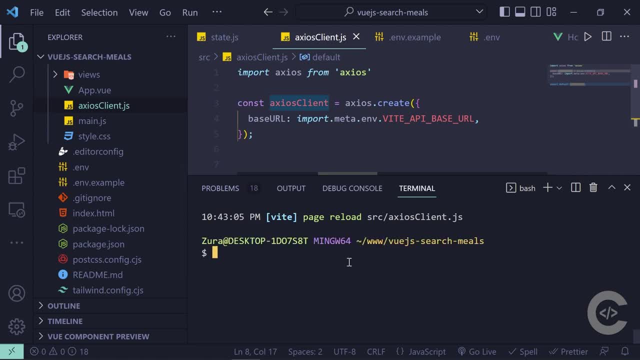 .env example we need to change something in the .env example and i think whenever we change something in the .env or we just create .env we have to reload our server so npm run and dev 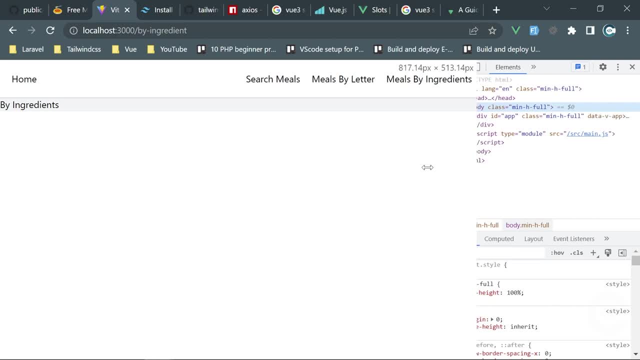 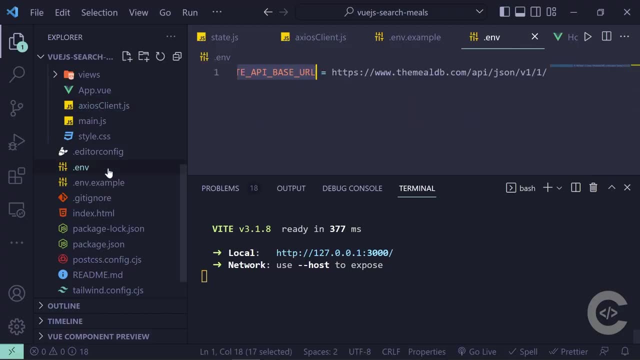 we need to run this and now if we just reload the page let's see search meals salmon hit the enter it works if i open my env and change a single letter right here and which will now point to 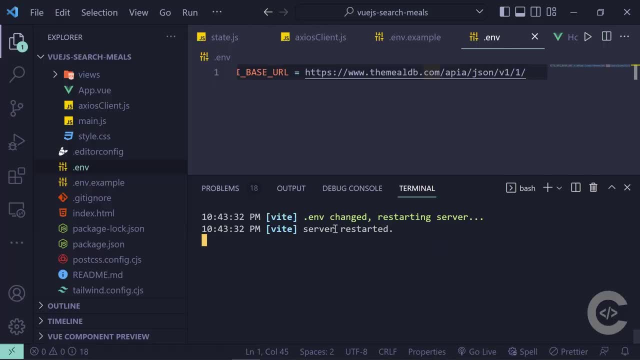 a wrong url and server actually restarted and if i just reload and make request to that url 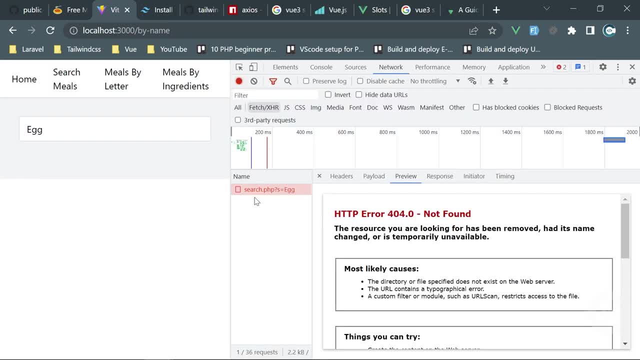 we're going to see error in the network okay not found all right so let's revert this into 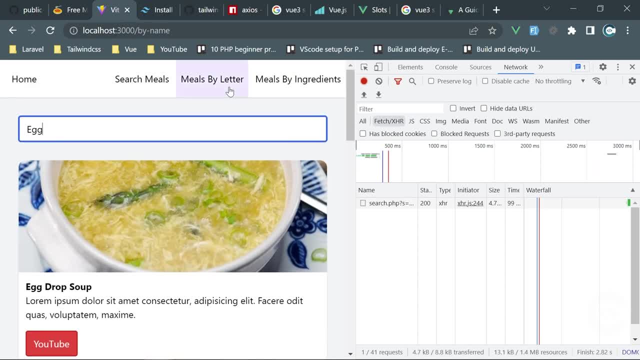 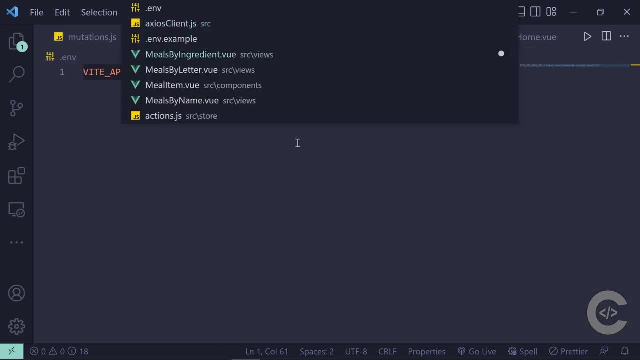 correct one and type egg right there and it's going to return so we have that implemented and now let's go back into our meals by ingredients so 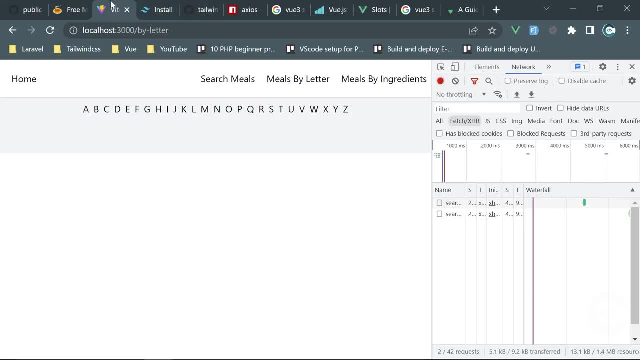 using axios client we're going to get all the ingredients and the endpoint will be this 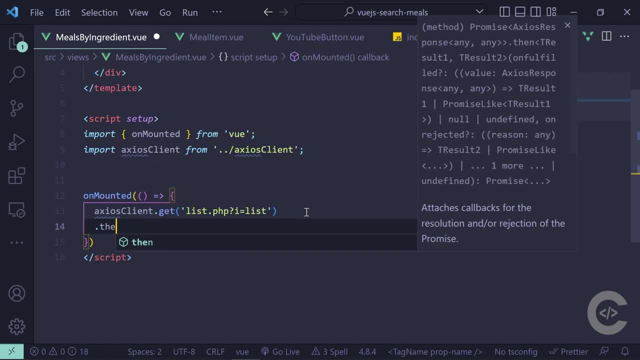 let's put this right here we get response we take out data from there and let's create right here 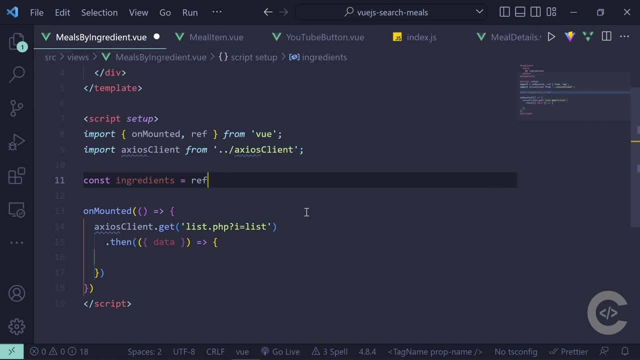 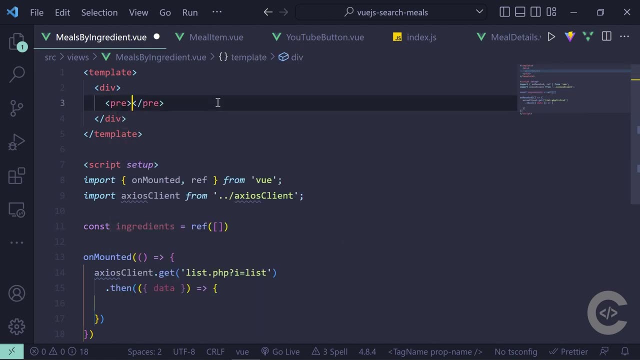 ingredients that's going to be ref by default empty array and let's output right here ingredients 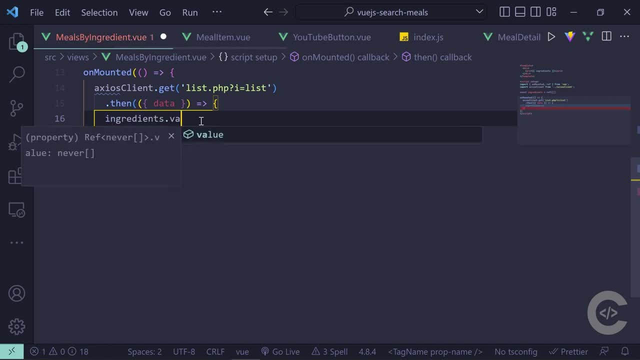 then when we receive a response ingredients dot value equals data and let's put again 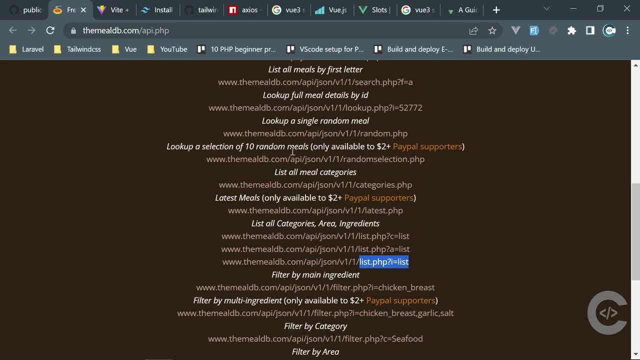 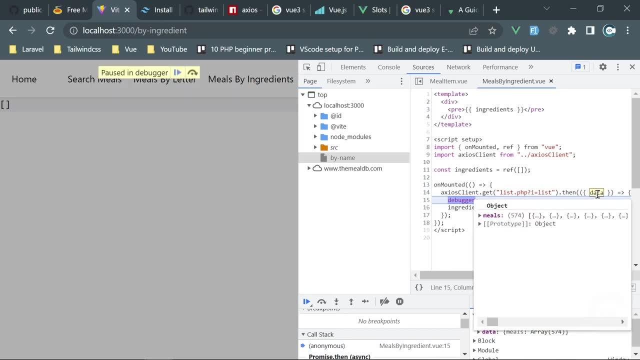 debugger right here just to see what is the actual data coming if we go in meals by ingredient here it comes the data contains meals right there 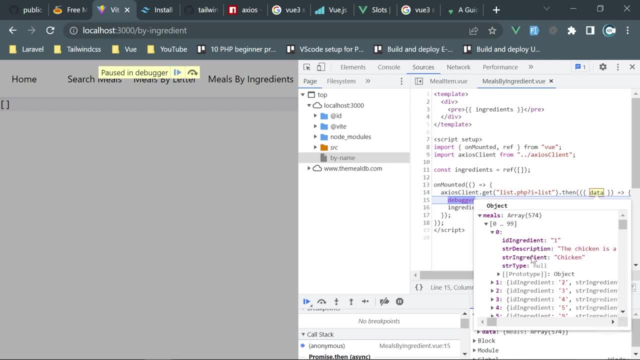 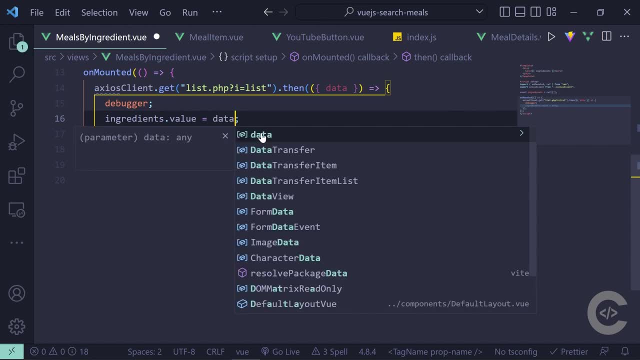 and we have id ingredient as your description is your ingredient all right i think we just uh need to take uh data dot meals from here and we have ingredients 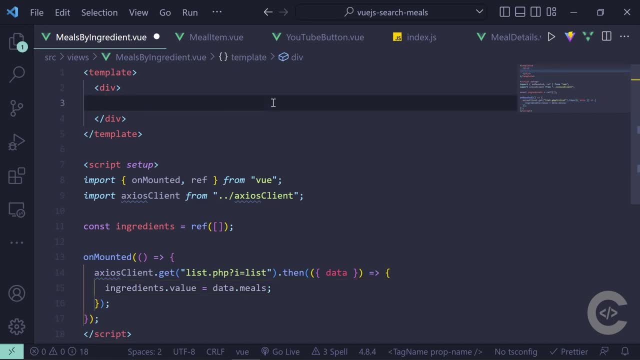 and let's start iterating over our ingredients so let's create um div with v4 oops v4 ingredient of ingredients 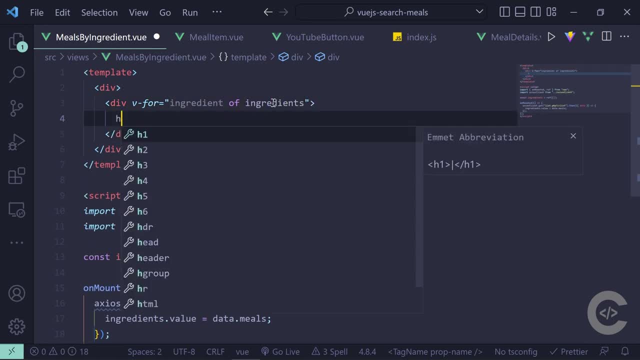 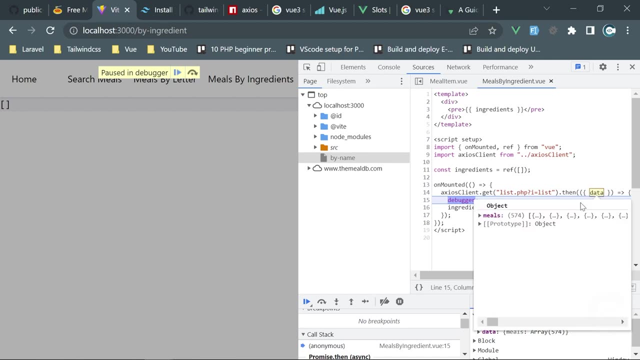 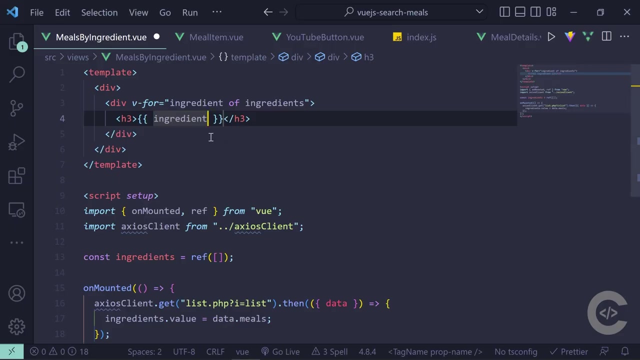 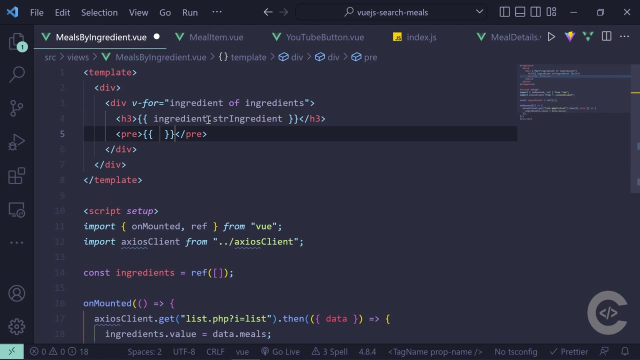 and we are going to display ingredient what is the data look like it has str description str ingredient so we are going to output str ingredient and then we're going to output 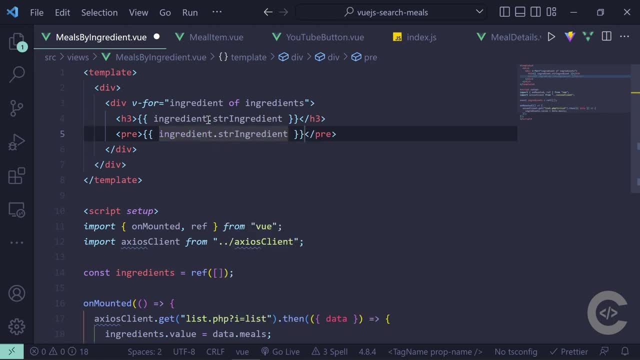 ingredient str description all right let's give it some styles class text to excel font bold let's give this one key equals ingredient.ide let's give this one also classes bg white 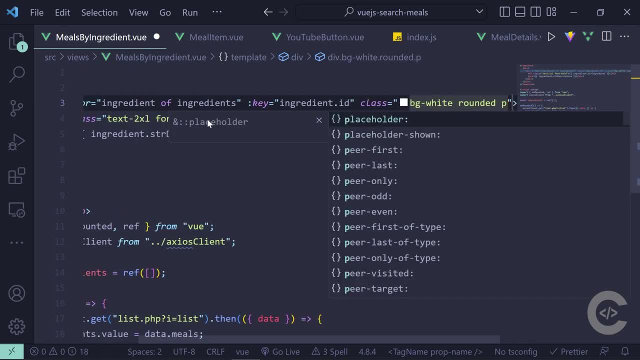 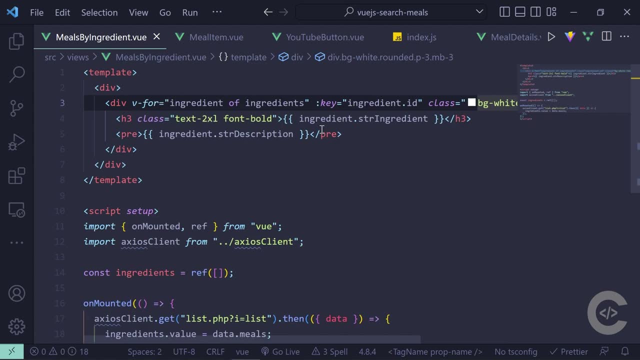 rounded a padding of three and margin bottom of three so i save this let's change this prayer into just paragraph 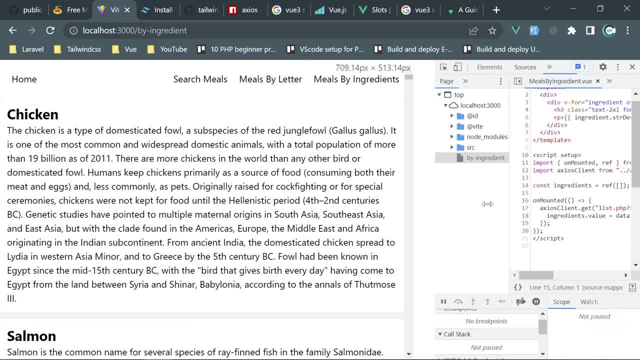 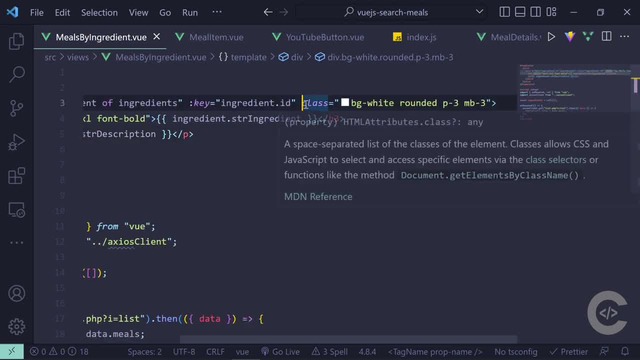 and let's proceed now let's just reload the page okay so here we see that let's give this one shadow as well shadow 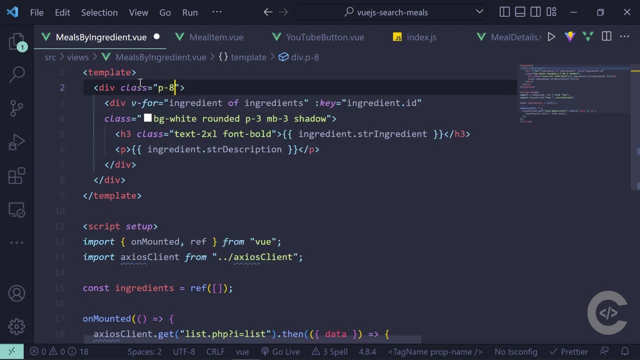 and let's give this one padding of eight 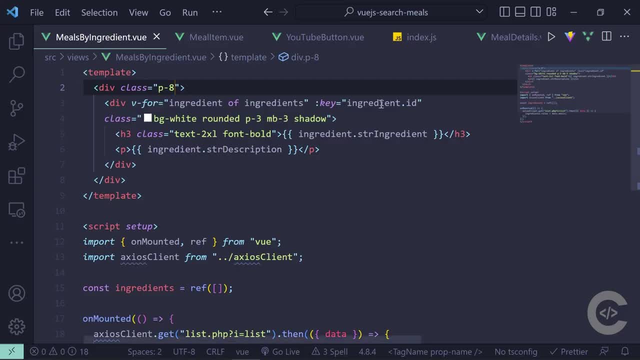 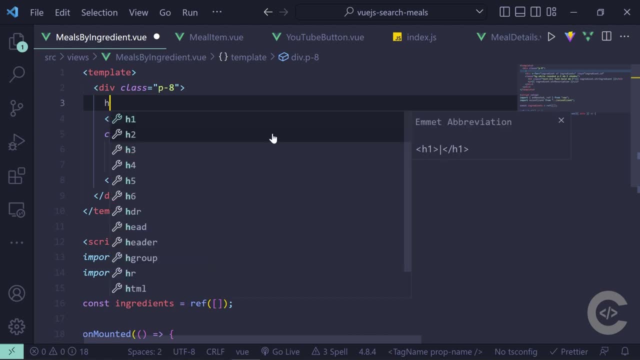 here we have these ingredients let's give this h3 also margin bottom two and let's create page title as well meals or ingredients 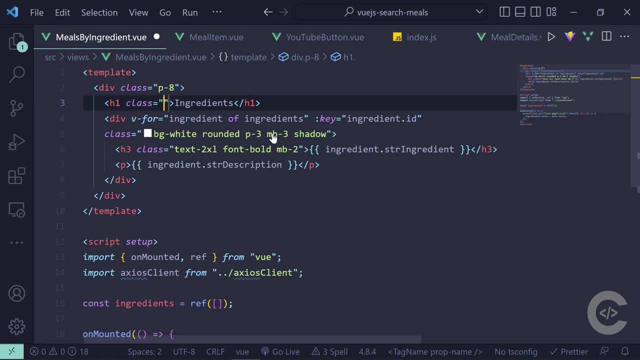 it should be something like text for excel probably font and the margin but supposedusing the the hex and the margin bottom four 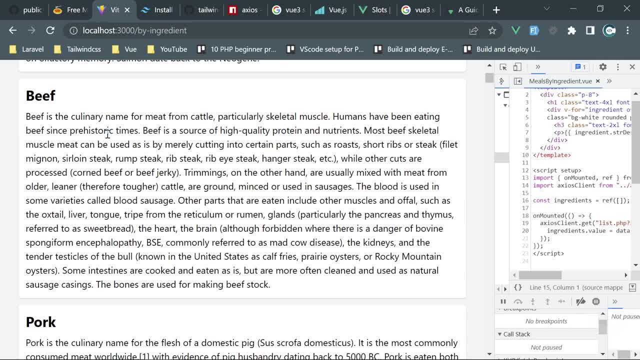 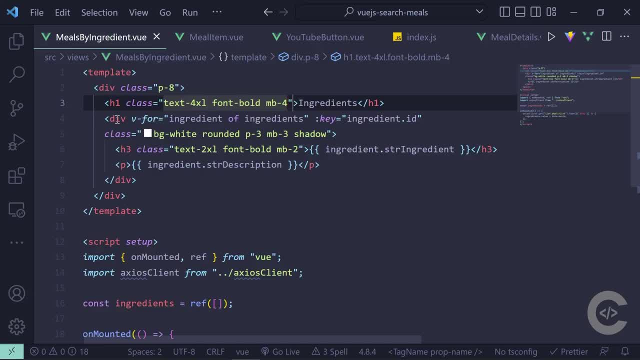 okay we have all those ingredients and whenever we click on them we want to take meals for example i want to take meals for avocado so let's just make this div 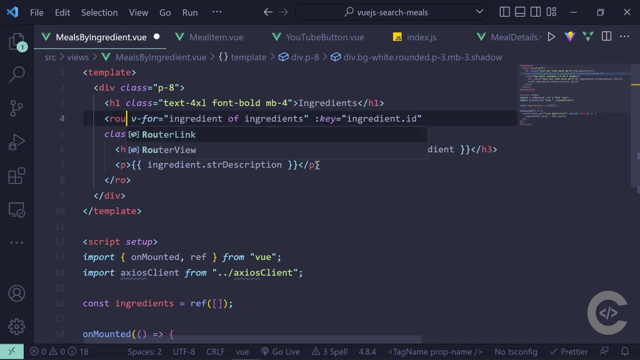 let's just make it router link router link so we enfrey almost all jacket is called noodles for tomorrow look i have the settings here for today so i mean they are yea you know you can go any time worth it and the model what i see here 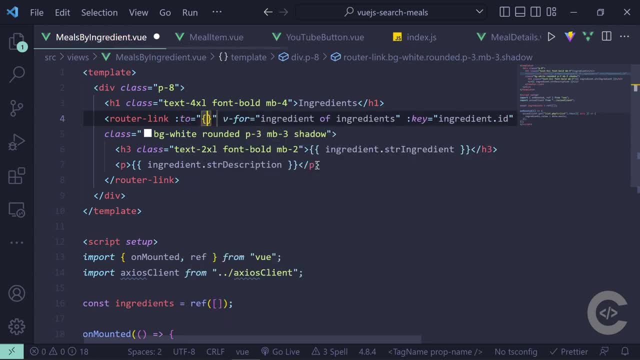 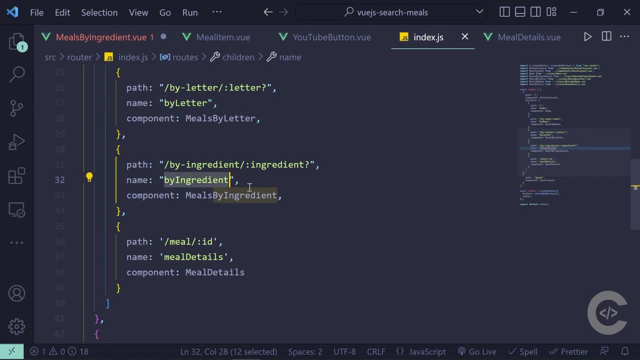 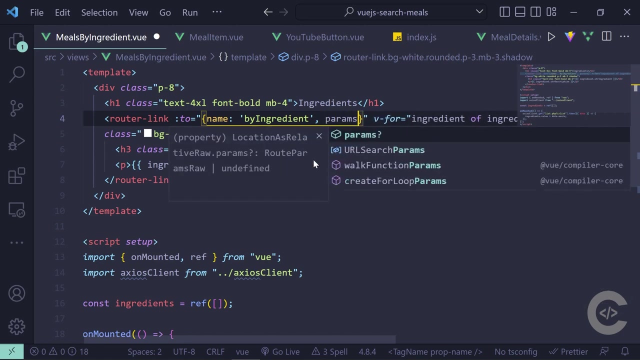 then we link this to page called name as open rotor and it is called by ingredient by ingredient we specify param right here and the param will be ingredient so ingredient corresponds 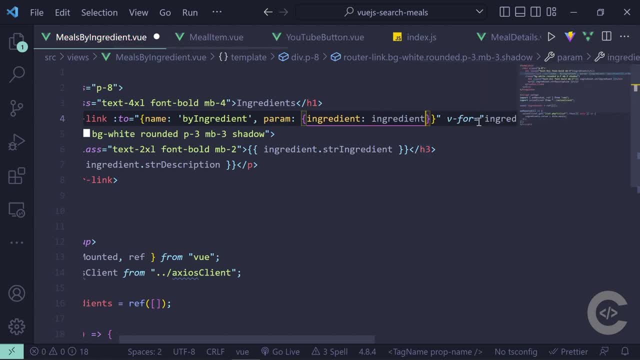 to ingredient dot id something i think it's called id ingredient ingredient let's save and test this 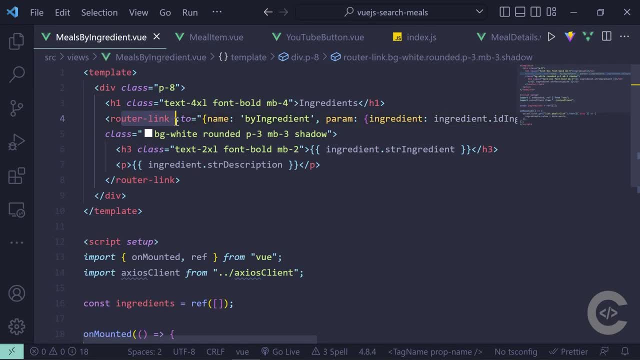 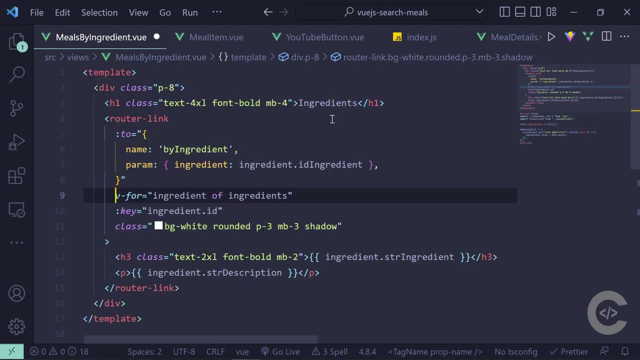 okay now a lot of things was broken because this rotor link basically is not a block level element so if we just format the code if we just give this one block 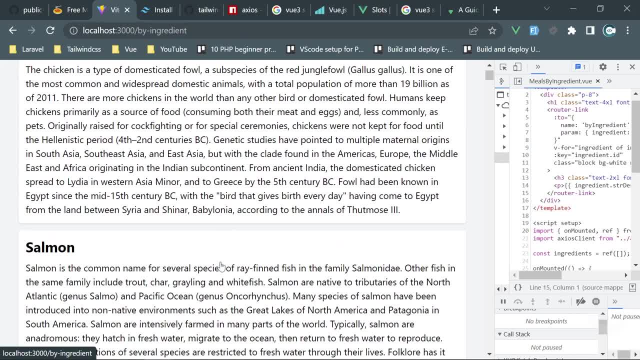 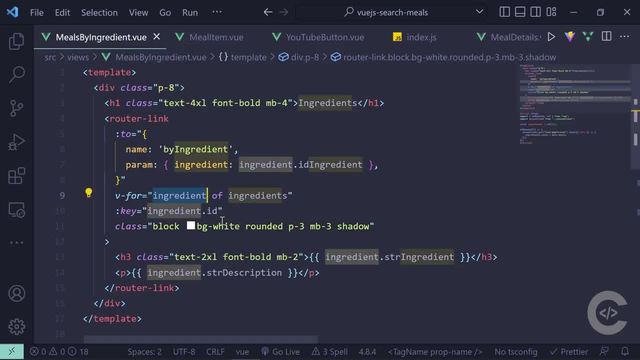 everything should be fixed all right and on mouse over we don't see the url changing in the bottom left so probably we didn't take this id correctly is it just id let's just output ingredient 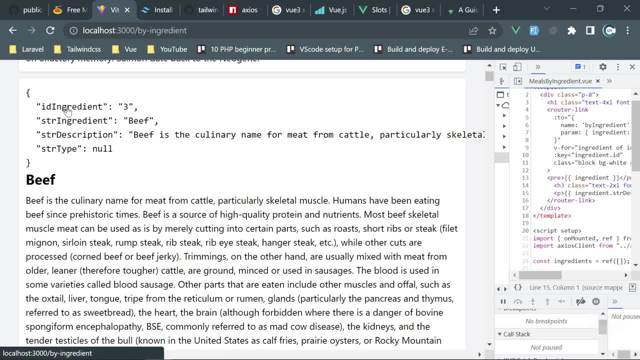 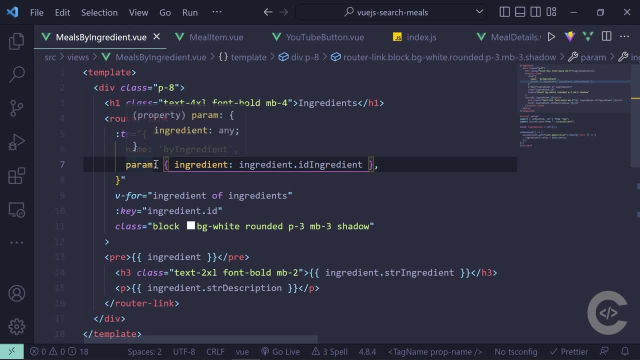 id ingredient this is how it should be are you following from primedia funding id ingredient 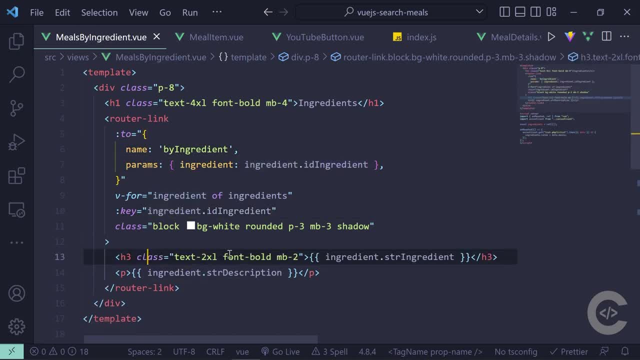 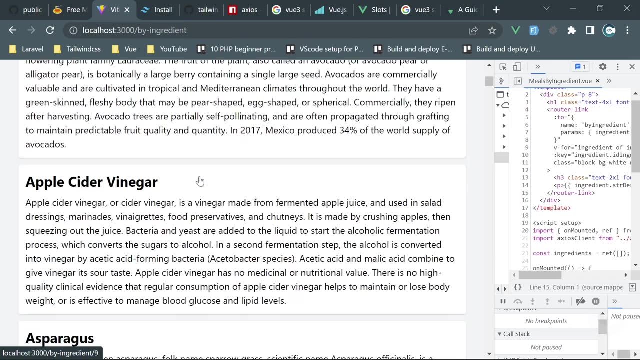 in gradient this doesn't work rams params it should be params okay we have all the ingredients and i'm going to click on avocado where it is so i'm going to 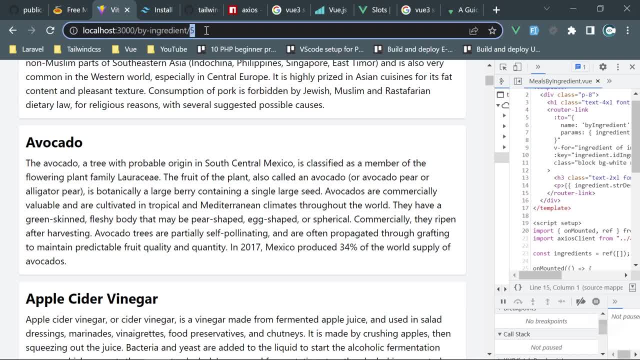 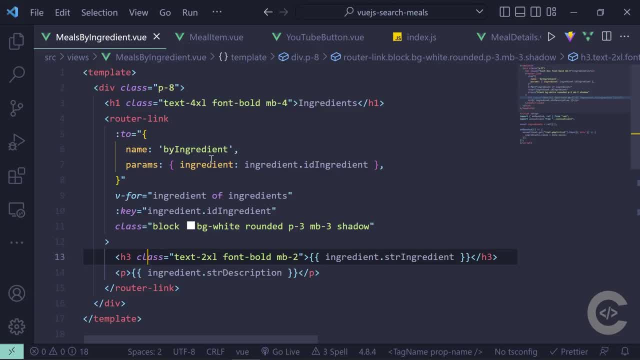 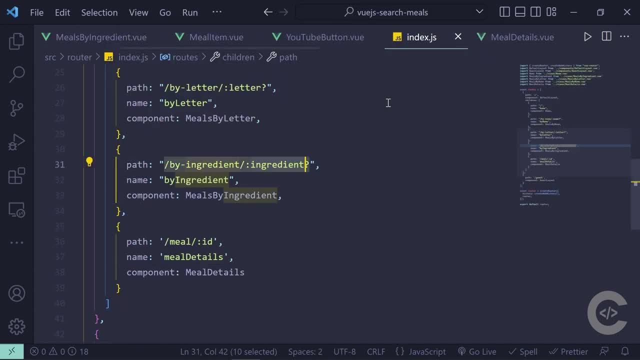 click on this and it changes the url okay that is something else we we need to handle which we didn't thought about it before so this is the ingredient page if we actually open this and if i click on this and wrote her we see that this is um the component actually is wrong 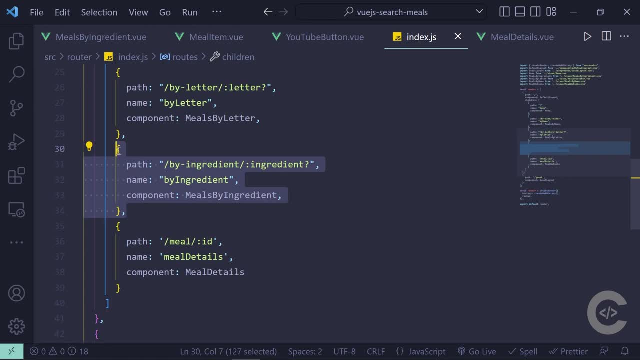 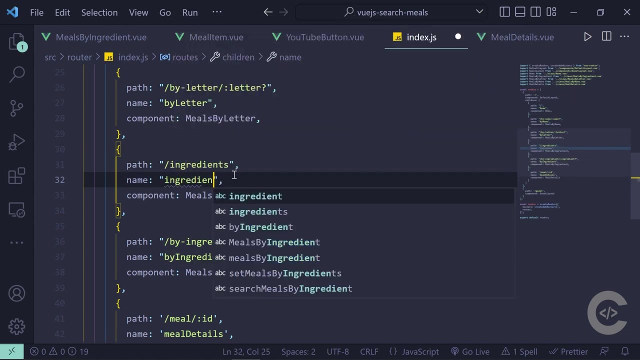 meals by ingredient those are basically ingredients page so if i just duplicate this and that should be that should be ingredients simply ingredients all right and i'm going to remove everything and that should be ingredients 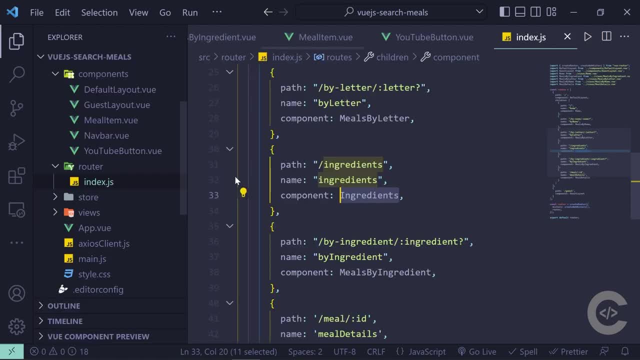 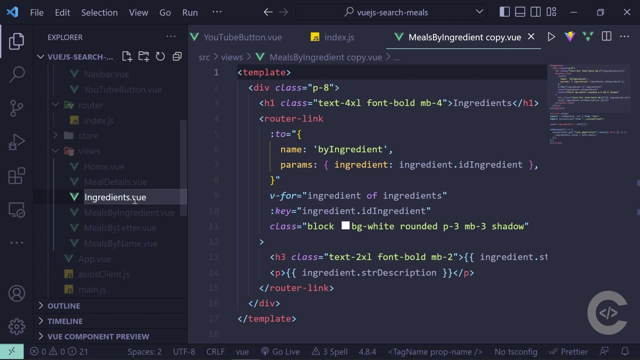 ingredients and we have to create this ingredients view let me actually duplicate meals by ingredient and I'm going to call these ingredients and hit 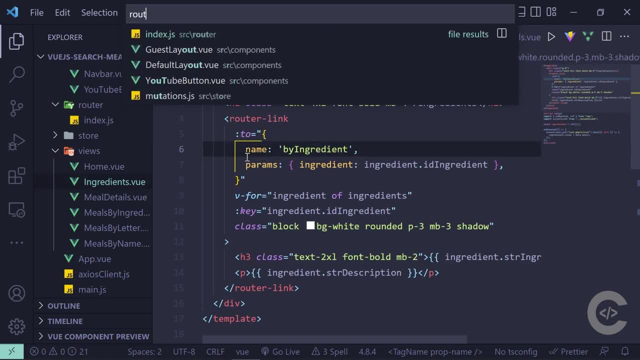 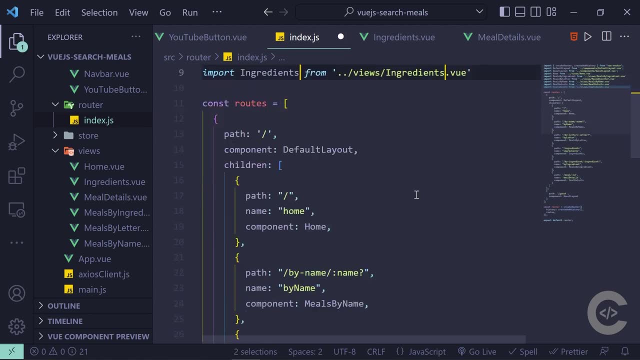 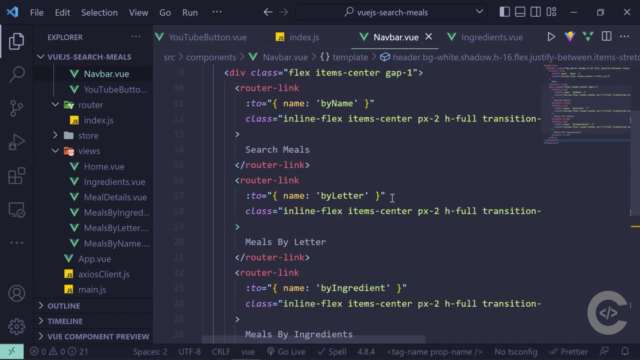 the enter and if we go in the router and we have to import ingredients here alright and if we now open navbar we have to link these into ingredients 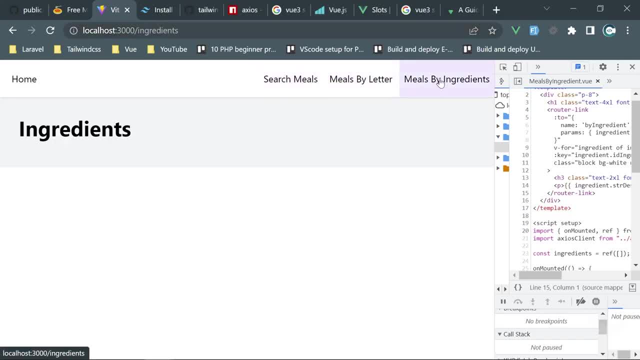 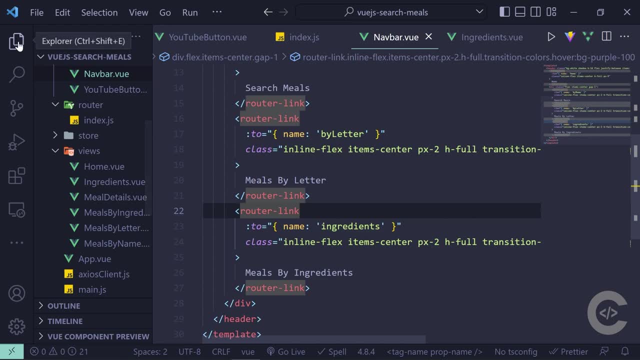 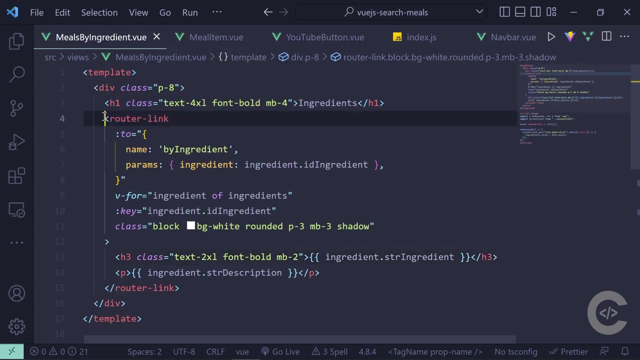 alright so let's check this out we have ingredients that works fine however now when we click on this it should activate meals by ingredients and in this case we can remove this 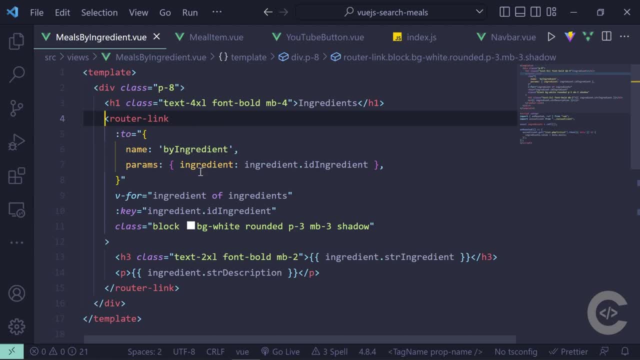 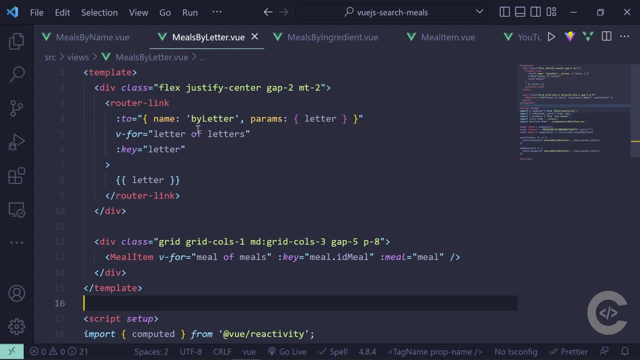 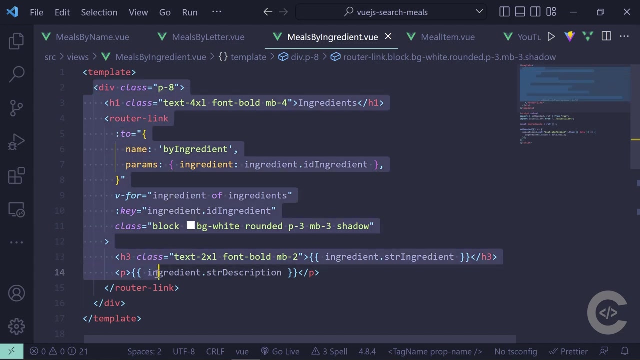 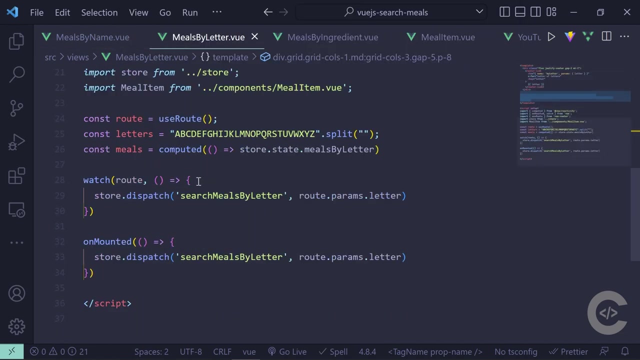 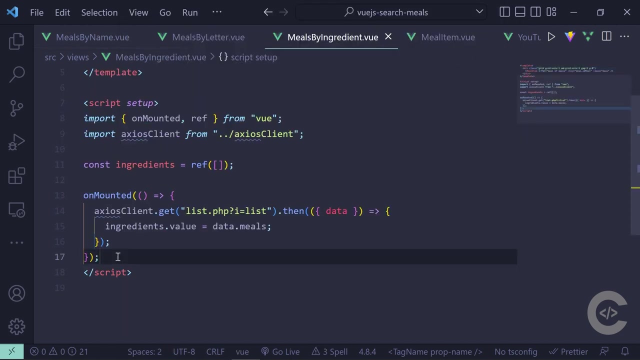 rendering ingredients instead we need to render meals and the template basically will be very similar to meals by letter okay because this we need this part so basically I'm going to replace this part and let's have a look what we have down below we have watch and unmounted so we need unmounted so let's just quickly do that meals by ingredients so let's remove 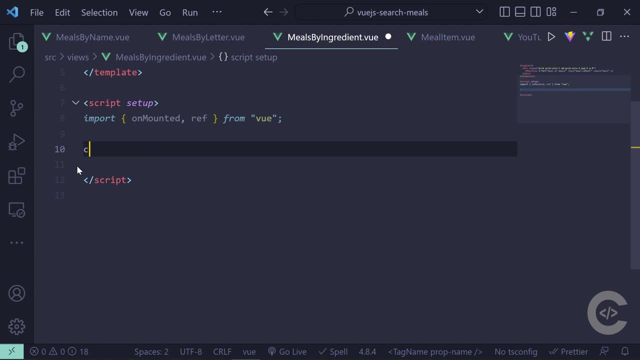 everything and we need const meals to be computed oops computed coming from store 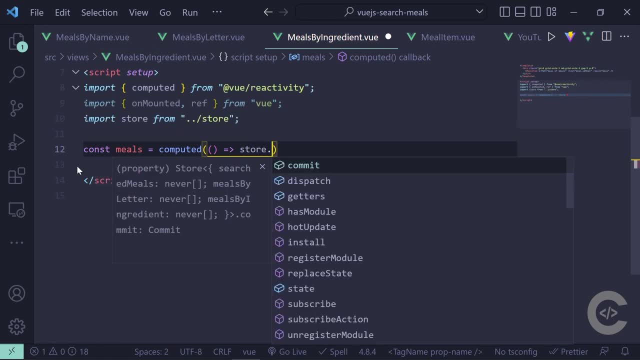 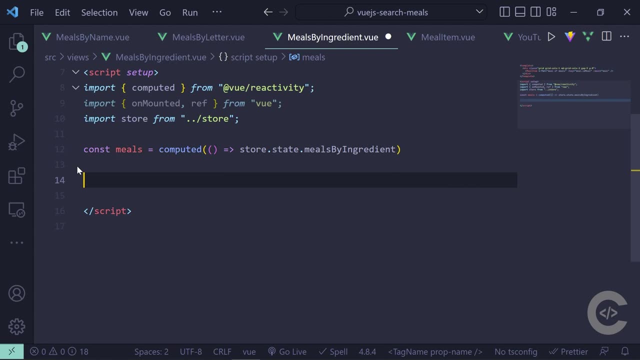 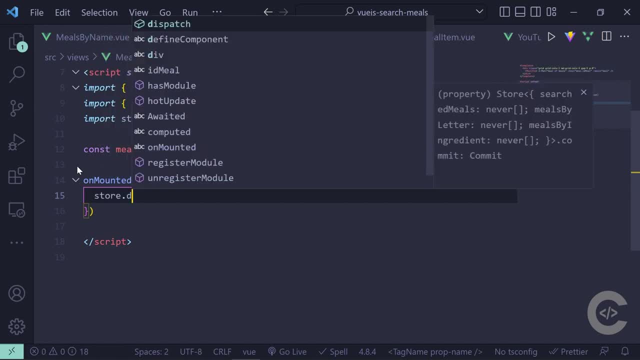 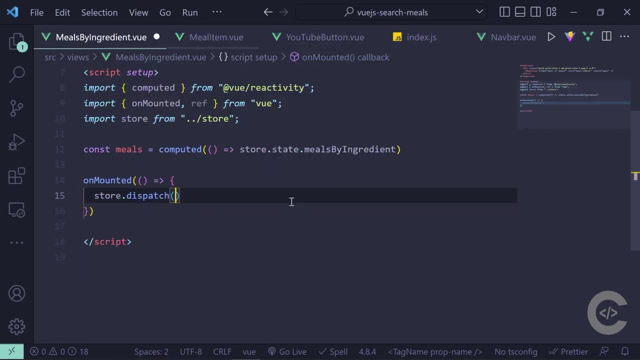 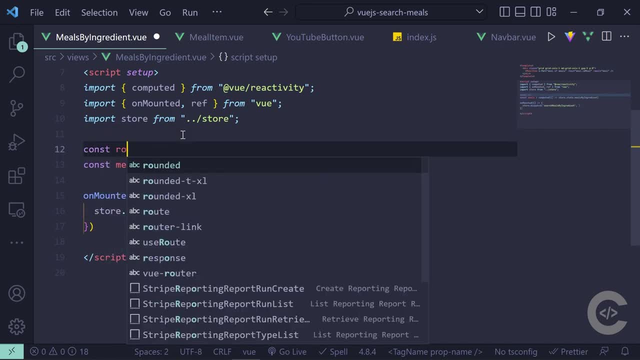 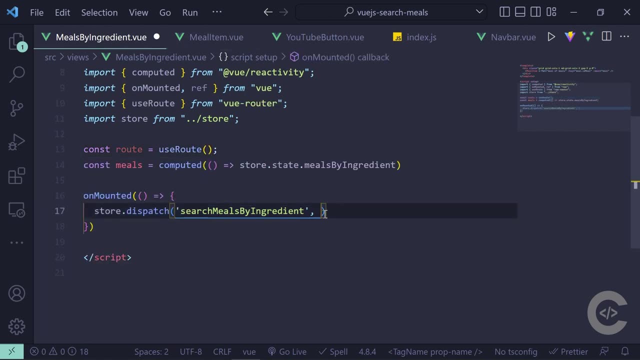 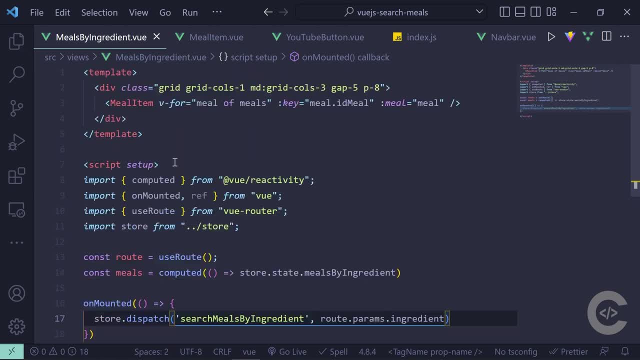 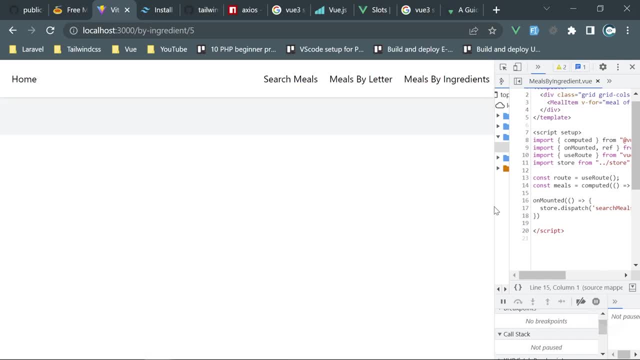 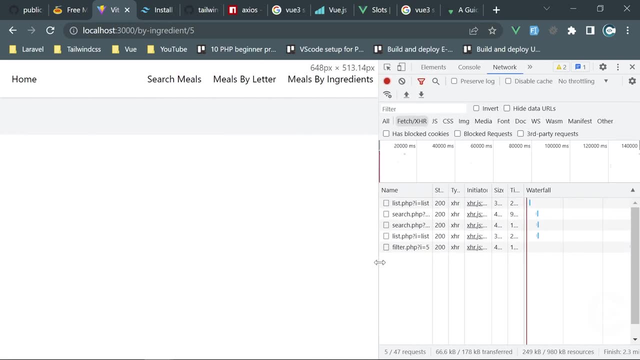 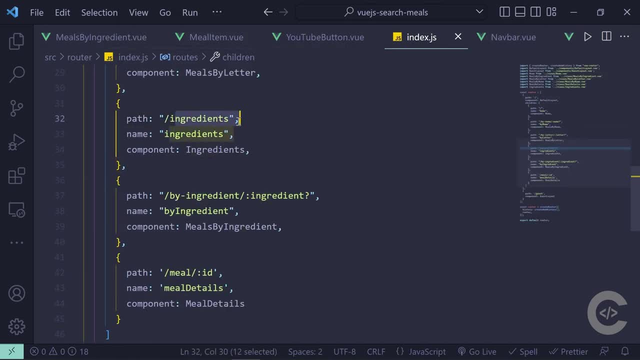 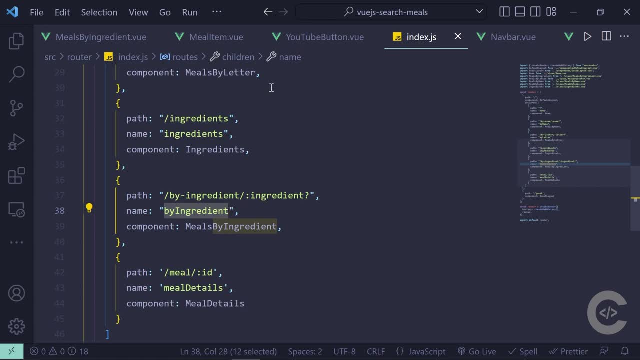 store.com okay what is the root name for the ingredients component by ingredient 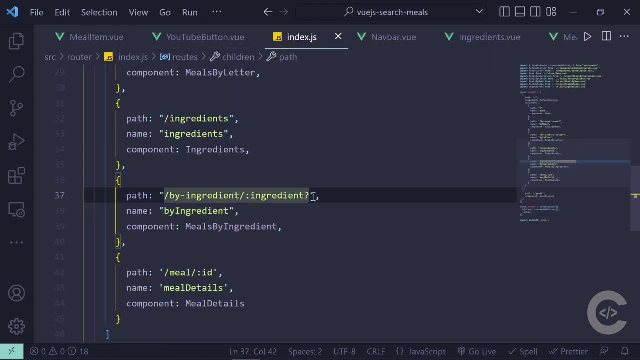 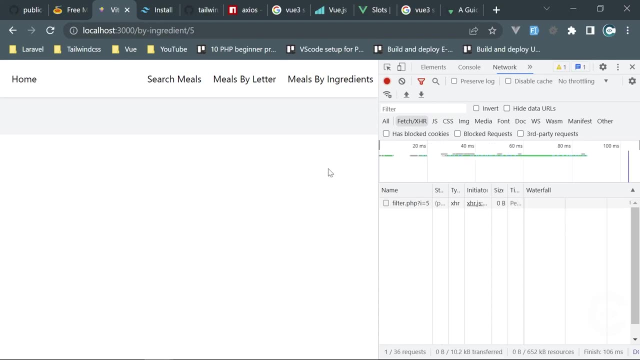 and we provide ingredient and that ingredient should be mandatory okay in this case this is how it should be so we save this again and reload the page and what happens let's go in the 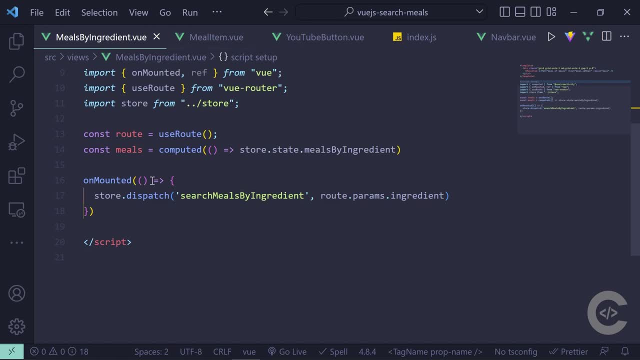 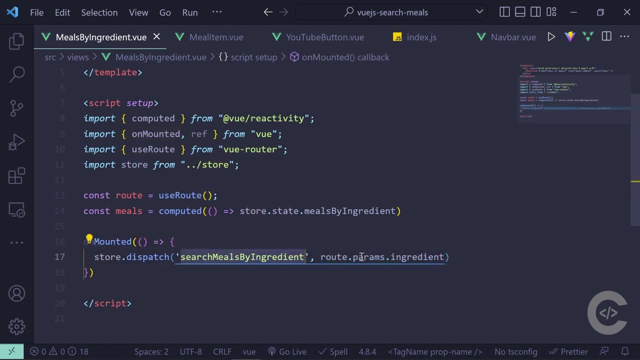 meals by ingredient and understand unmounted unmounted is imported then we have store store is imported the request is the request made here let's put debugger here let's 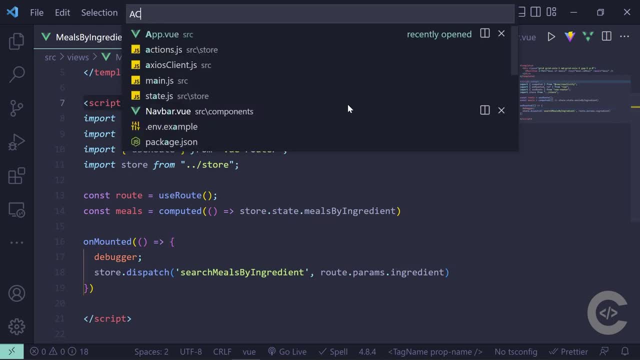 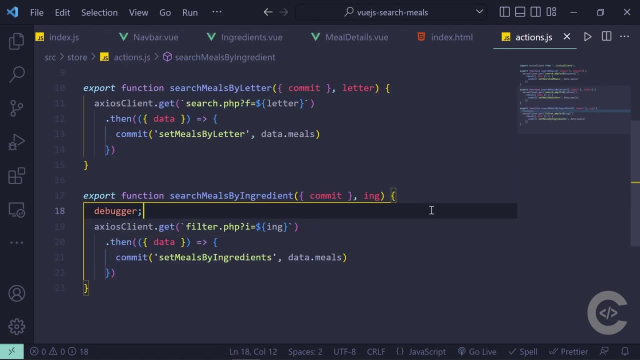 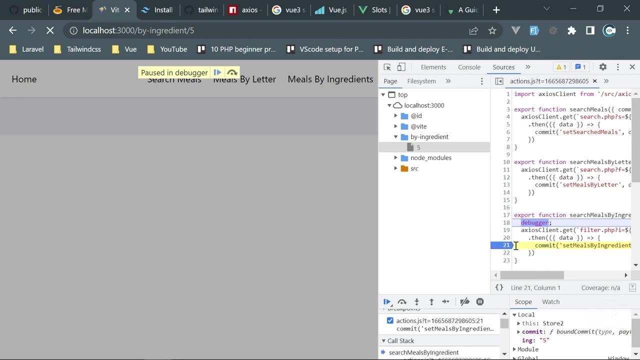 here it comes let's put another debugger inside actions and see so we just follow that it comes into actions let's put a breakpoint right here we get 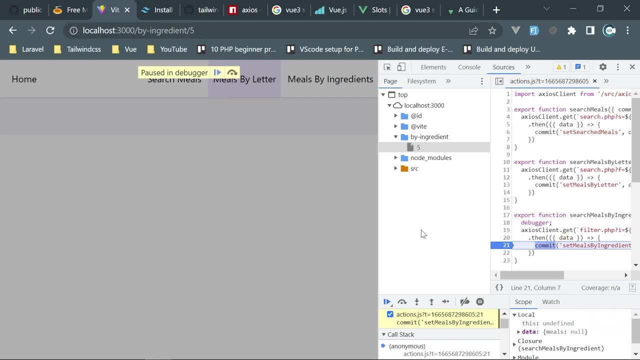 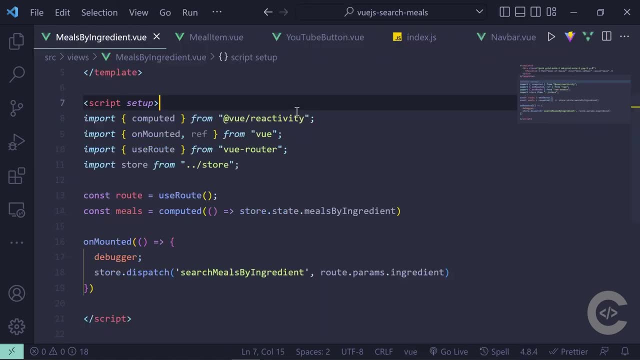 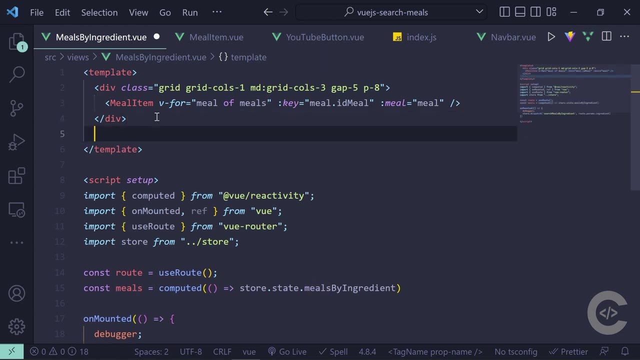 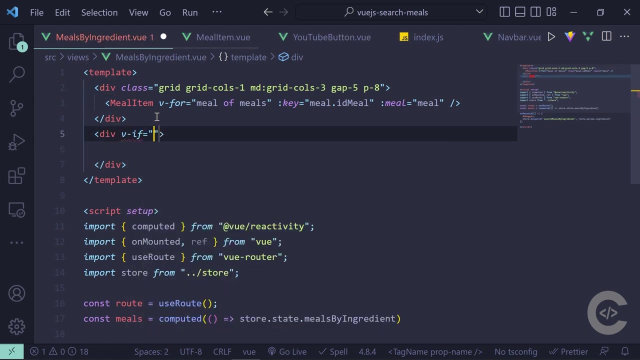 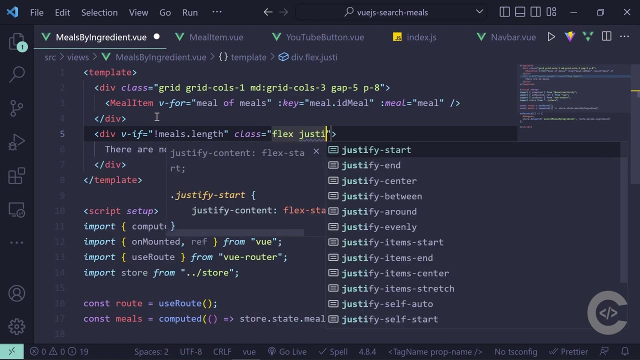 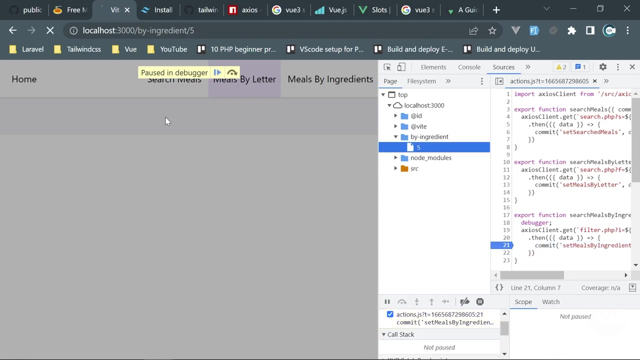 the data however meals is now i think there is no meals for avocado and that is the reason so if we go now in meals by ingredient and one thing which we need to handle is displaying there are no data so let's create div right here um if meals dot length does not exist then we display there are no meals and let's give this flex justify center text gray uh 600 all right and let's proceed and i think we need to 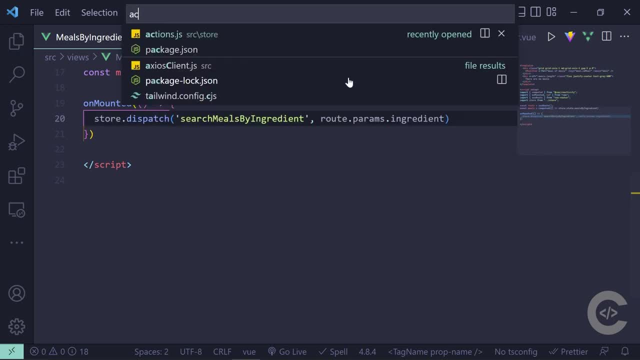 remove debugger from here and from actions as well 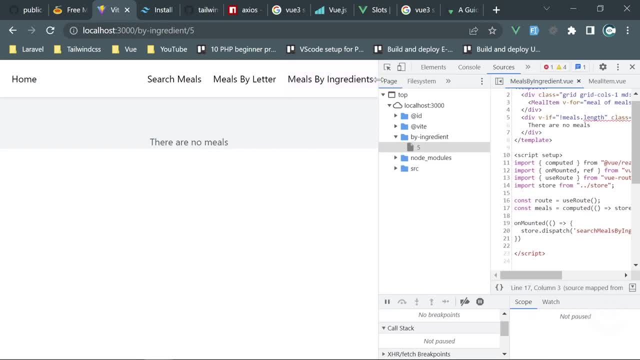 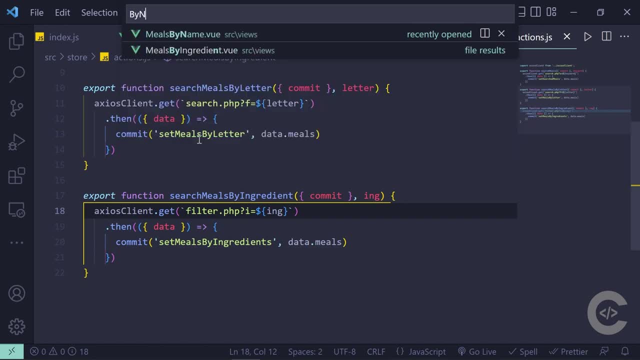 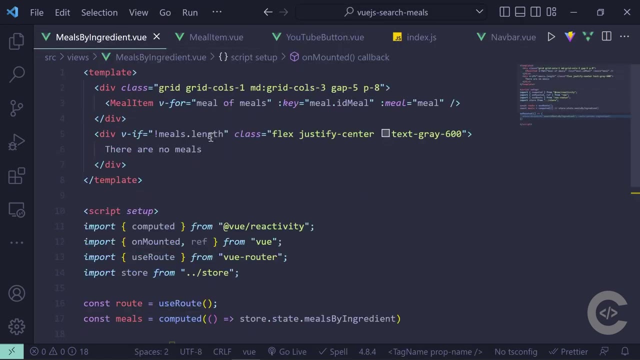 so now we just reload we see there are no meals okay right here we need to display the same message by name if there are no meals so basically basically we can put this in its own component 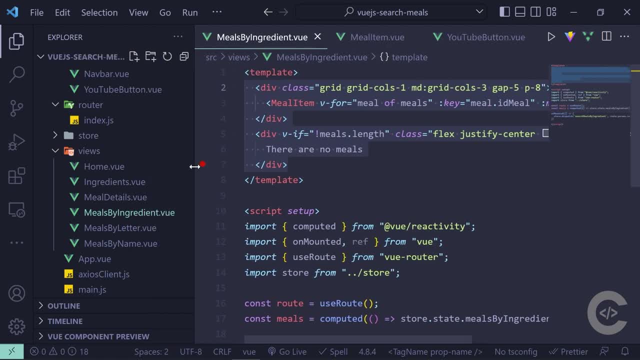 one and we can put in another component and we provide meals meals there okay if we go in the component 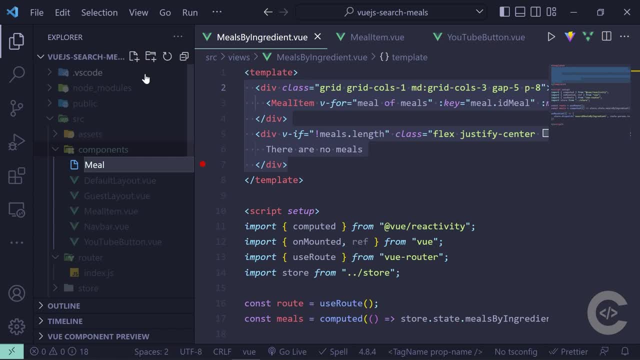 section i'm gonna create meals um meals.view and we have template there let's copy everything and we're gonna use meals 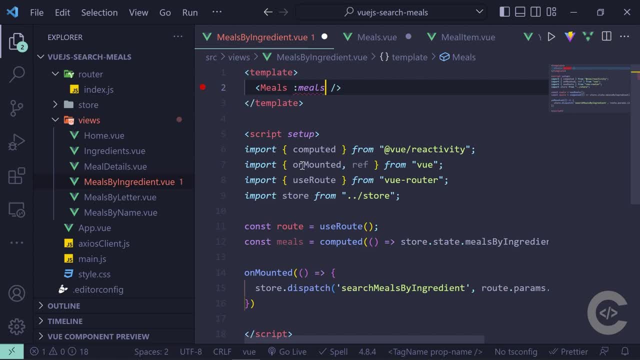 this is the meals component we're gonna use and we're gonna provide meals 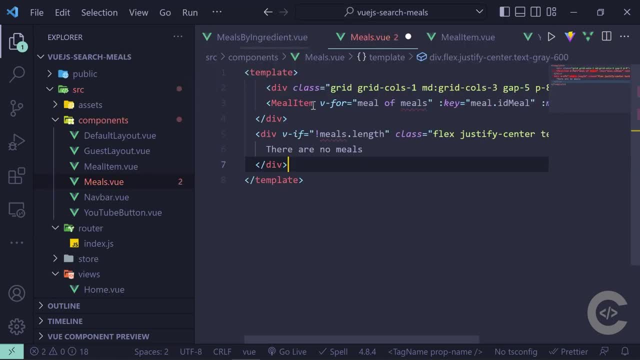 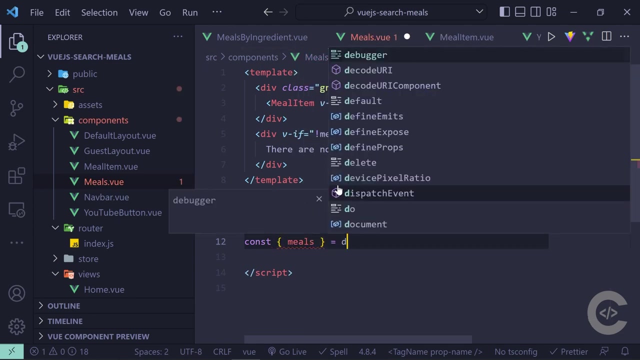 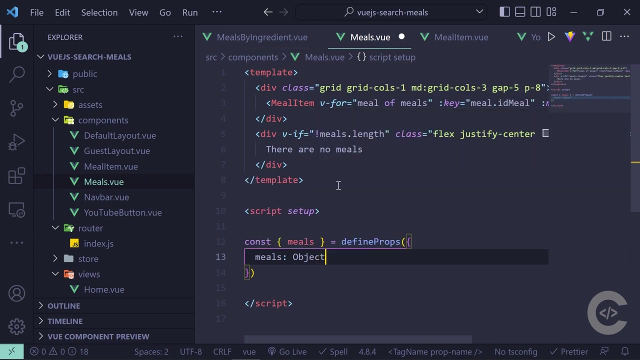 equals meals and then put the template right here and let's define prop using script and setup uh const let's destructure props and take meals equals define props and meals needs to be object meals needs to be object and we can specify that it must be required as well required true and type is object 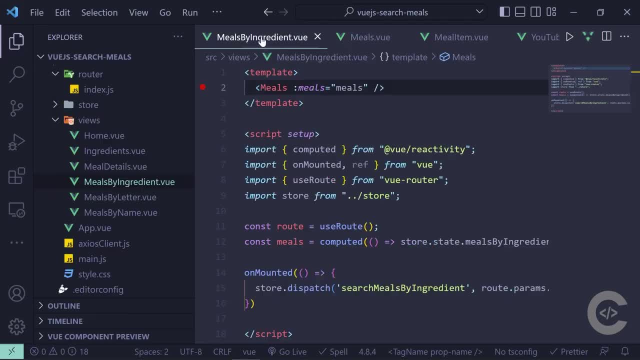 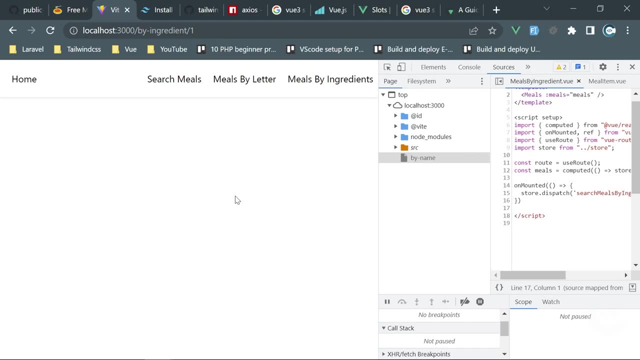 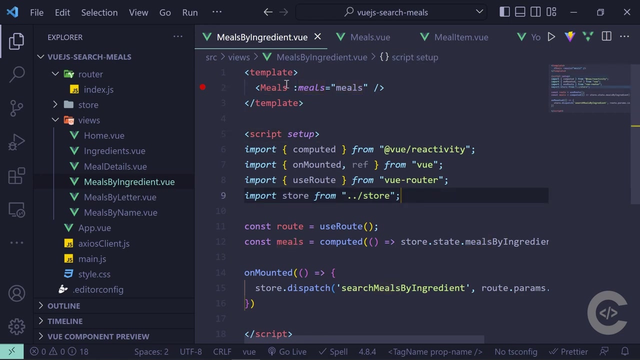 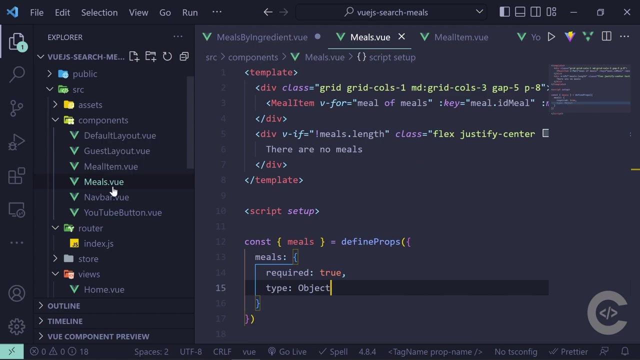 all right now we have these meals but we are using this by ingredients so if we go in the by ingredients click on this uh we don't see anything because meals is not important so let's import by the way why it doesn't import okay it does not import for some reason where is that meals created it is in the components okay it should be automatically imported but it is not so we have to do this manually 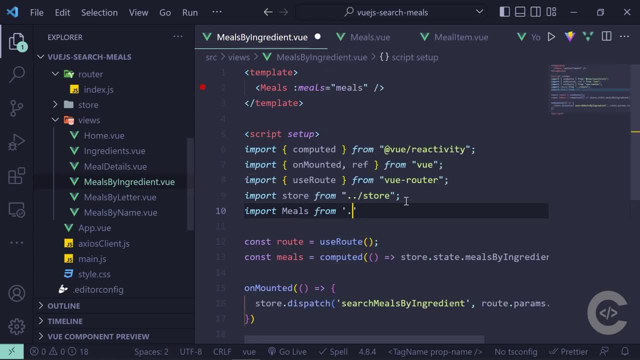 import meals from go one directory back in components slash meals dot view all 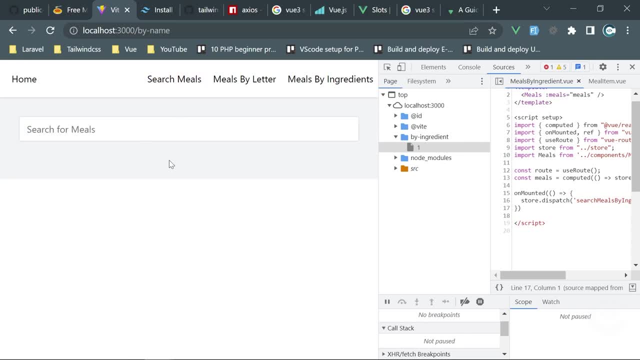 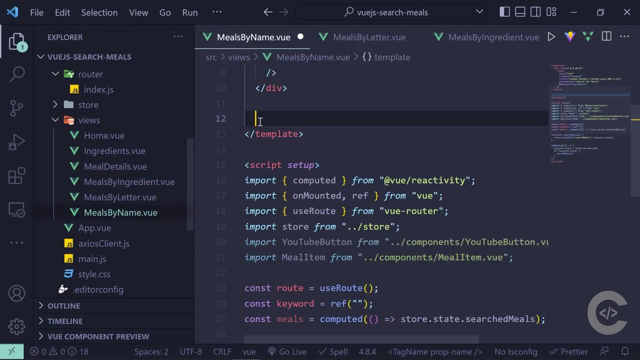 right we just reload the page and there are no meals and we need to display it right here as well so by name let's remove this and we have to use meals provide meals as well 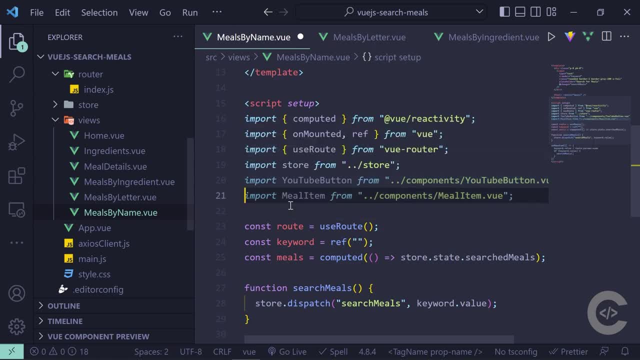 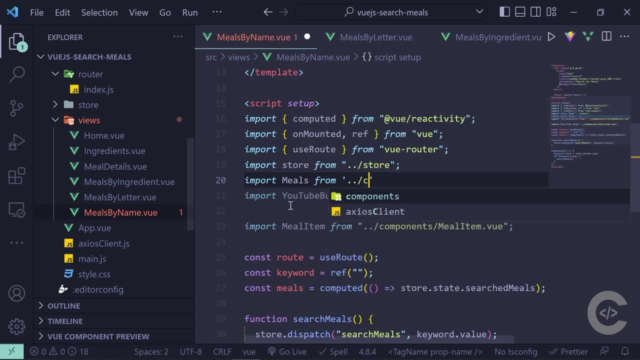 and finally we have to import import meals from components slash me not meal item but meals dot view and YouTube button and meal item can be removed because they are now inside 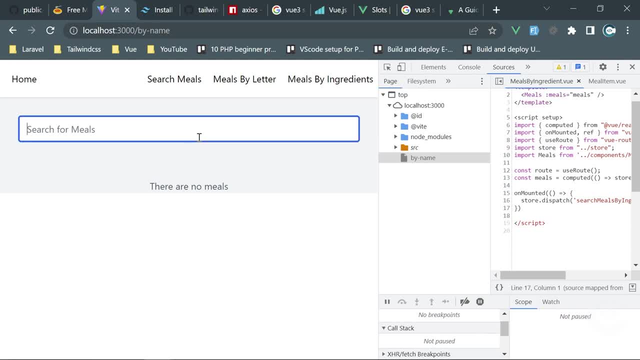 other component there are no meals search for egg now okay something is broken so we have to do this manually and finally we have to do this manually 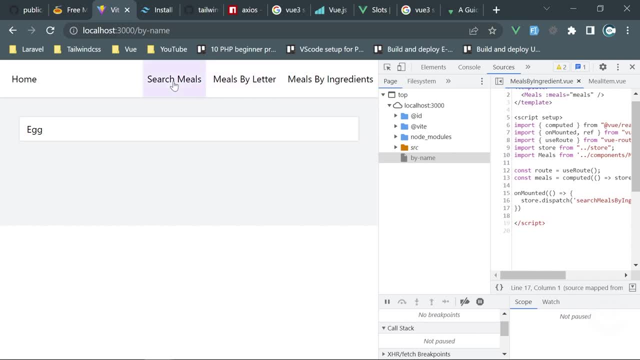 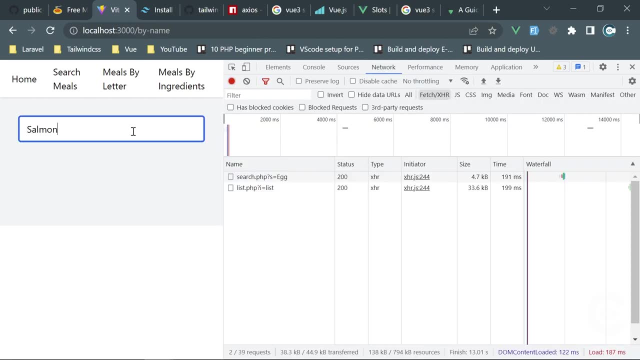 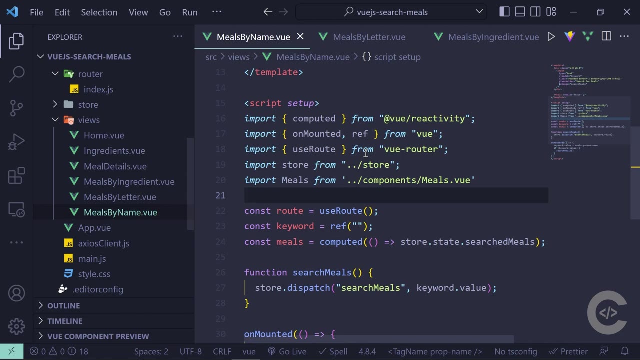 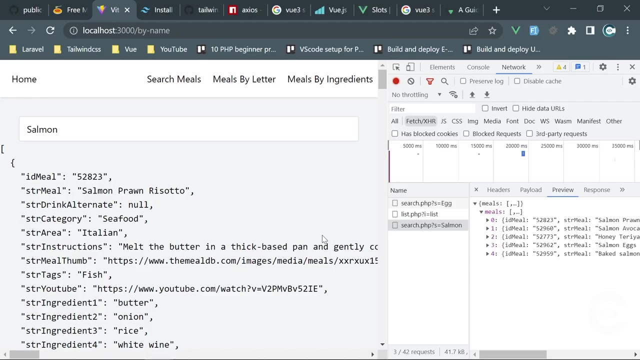 broken egg hit the enter okay we have broken something if we go in the network and search for salmon hit the enter the request is made we have meals data however displaying doesn't work this is meals by name and let's output if we have meals here we definitely have meals so the problem is probably inside this component 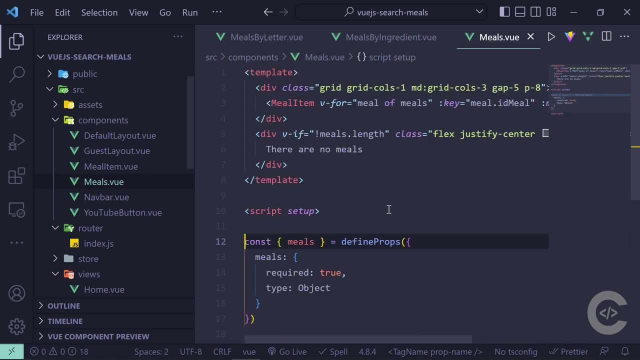 what do we have we have template and meals 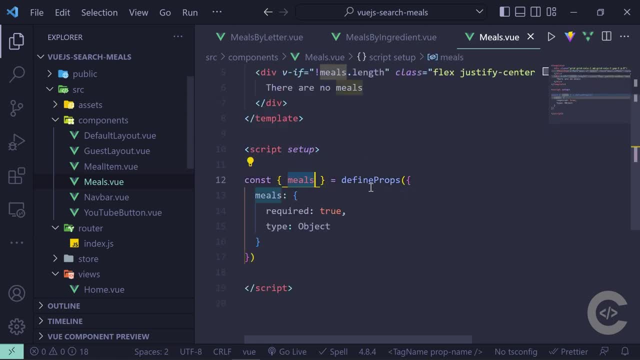 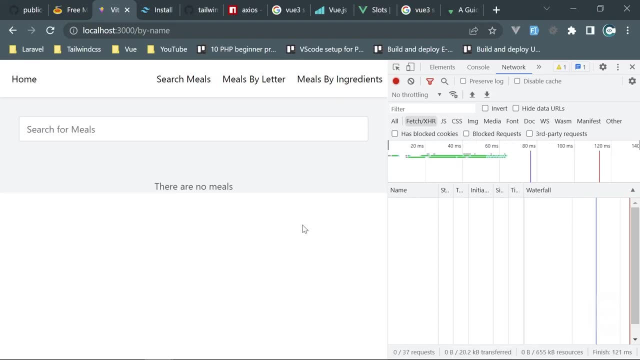 which is which must be type of object no it must be type of array this is probably 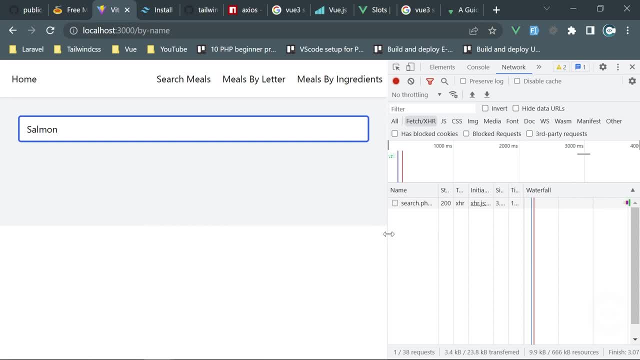 a problem salmon hit the enter no surprisingly that's not the problem so we have the meal 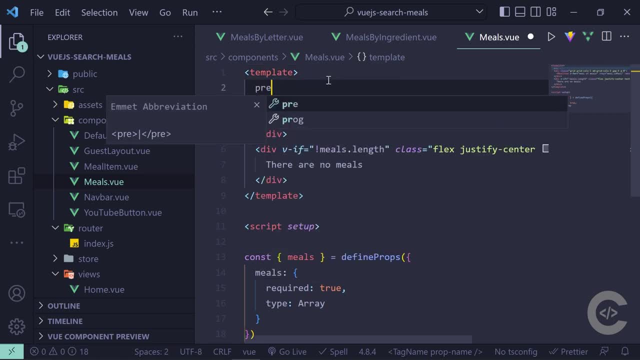 which is which must be type of object no it's not the problem so we have the meal which is which must be type of object no it's not the problem so we have the meal this component what mistake do we have if we just this component what mistake do we have if we just this component what mistake do we have if we just print meals 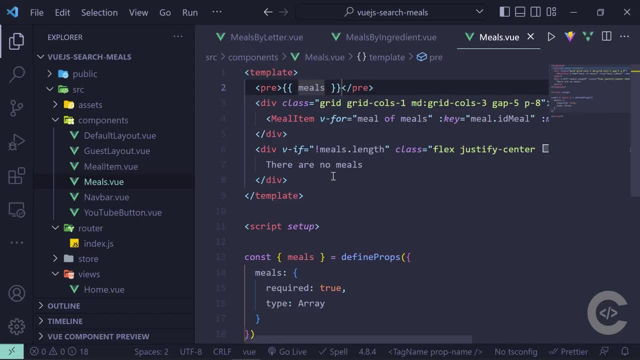 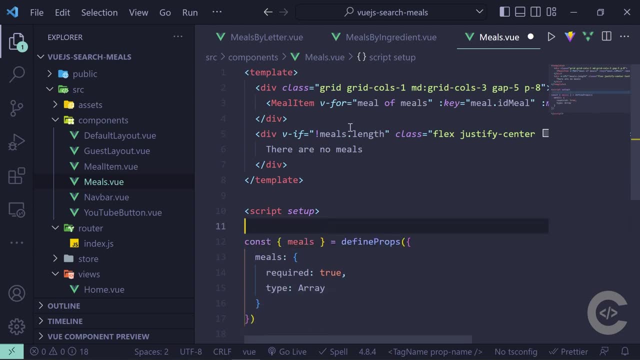 it is nicely rendered right it is nicely rendered right it is nicely rendered right i know the reason we are using meal item i know the reason we are using meal item i know the reason we are using meal item right here which right here which right here which needs to be imported so let me needs to be imported so let me needs to be imported so let me delete and retype 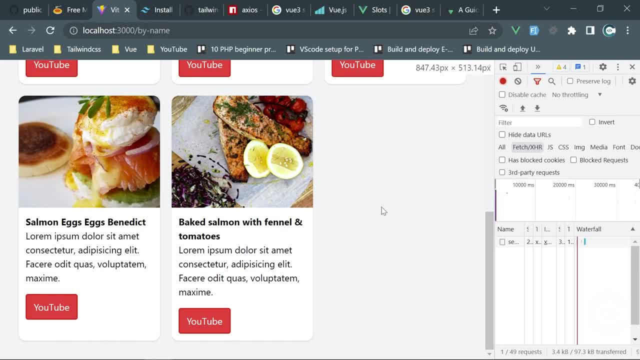 delete and retype delete and retype and it's going to automatically import that and it's going to automatically import that and it's going to automatically import that and now here we have it 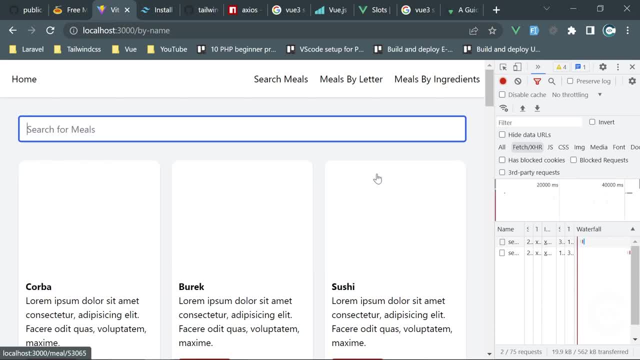 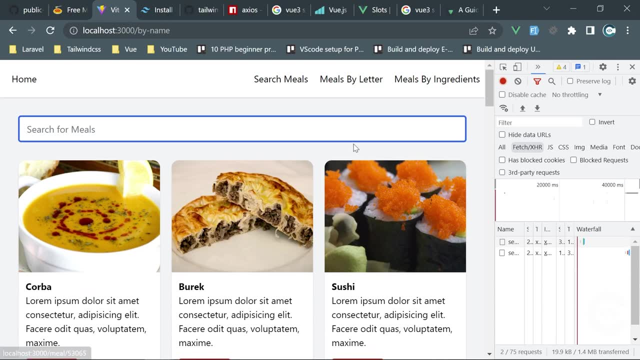 okay so if i delete everything and hit the enter nothing nothing is really um like the request should not be made and we should see that 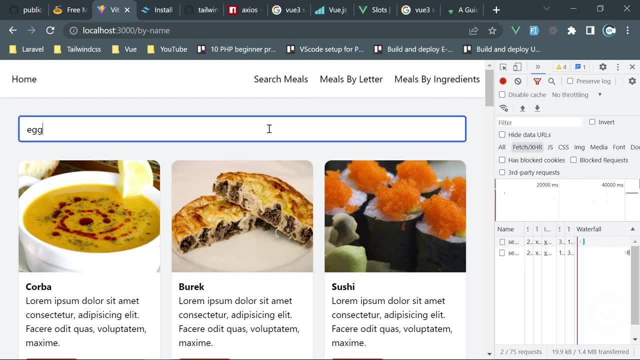 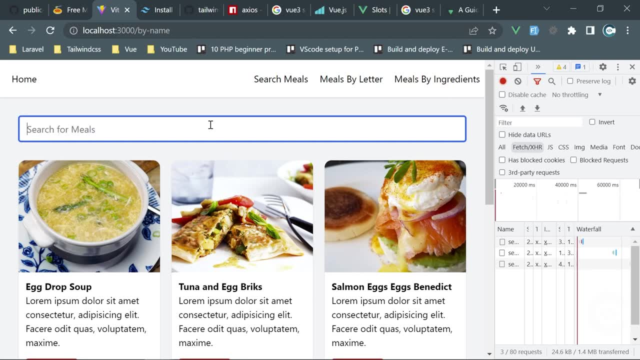 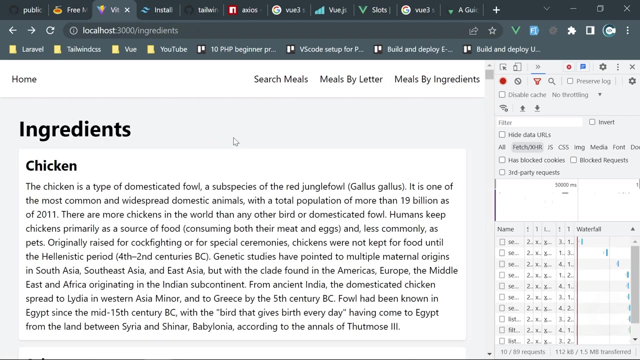 okay this is minor thing so let's type egg hit the enter we search for eggs um um what else can we search for like i'm stuck okay anyway um meals by letter that also works and meals by ingredient that does not work why because probably there are no meals for chicken 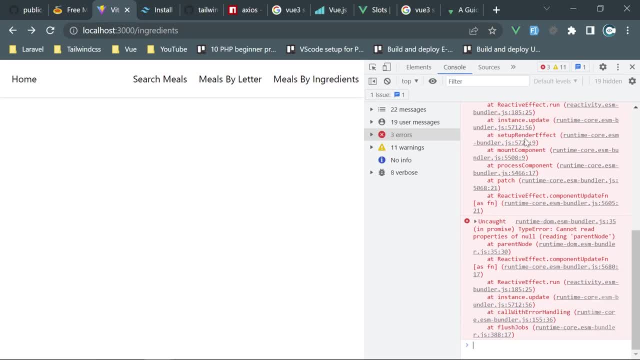 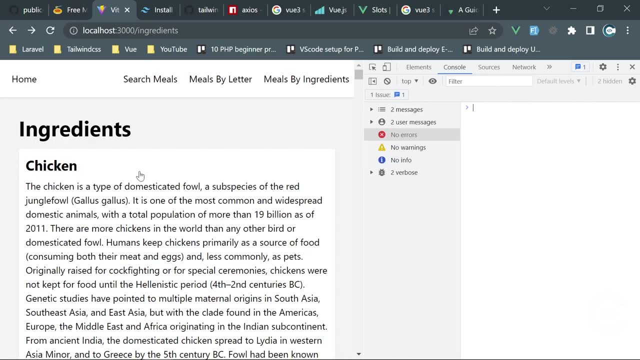 is that possible yeah why not we have some kind of errors as well let's reload the page she can click here and here's the error 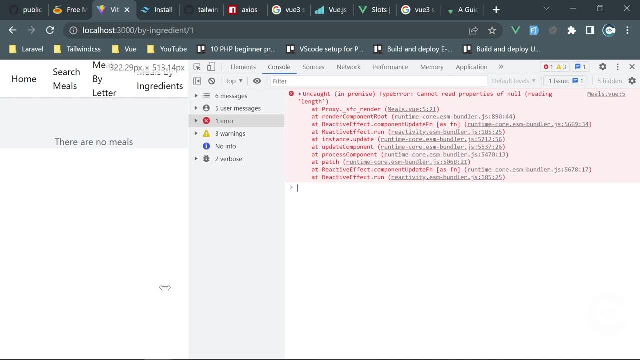 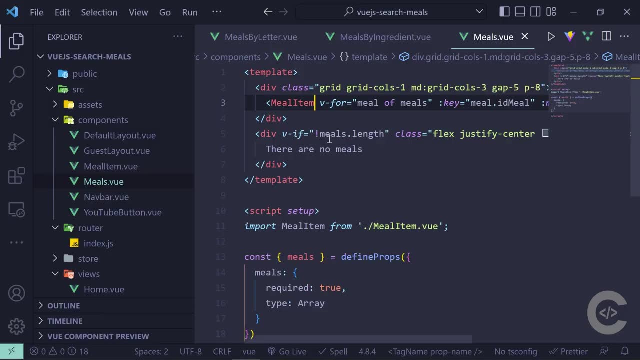 where does this coming from can't read properties of null reading length uh meals is meals null yeah i can specify default to be 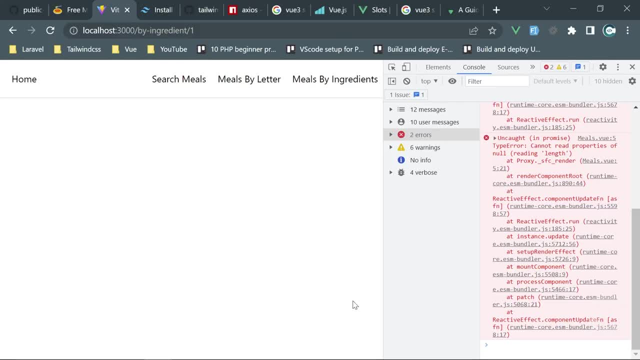 an array so that it will never be null 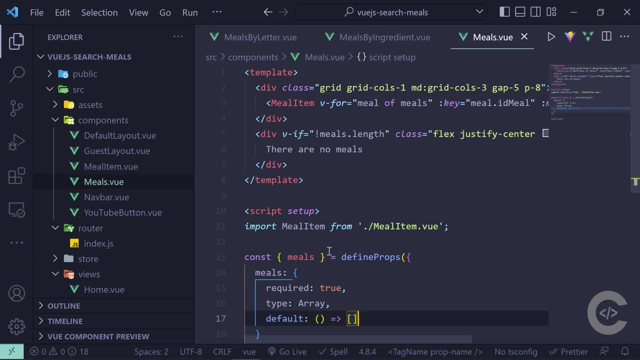 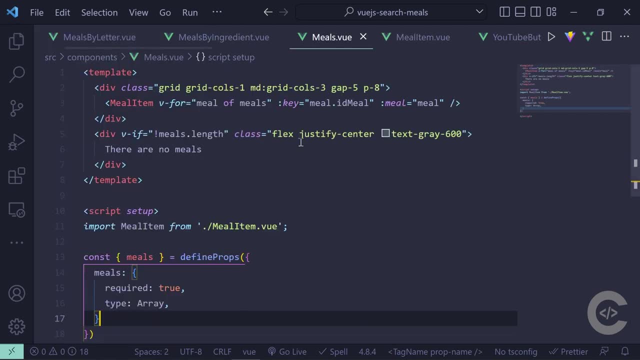 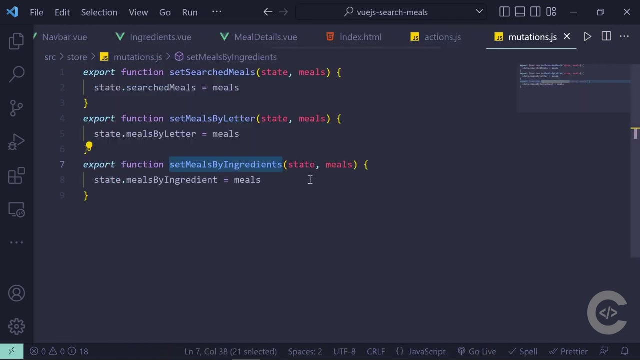 but that does not do what i want meals is actually now well okay how to fix that well in the mutations whenever we set meals if that is null and maybe we should do this for everyone like each method when this is now we 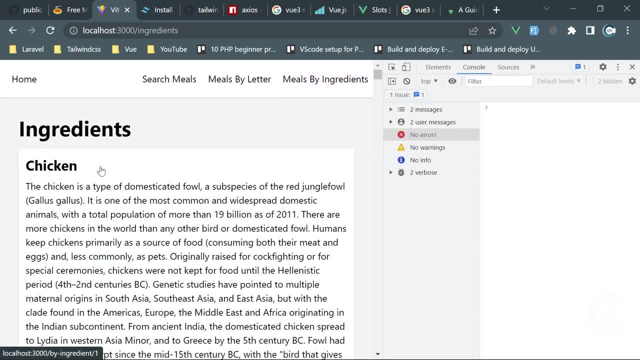 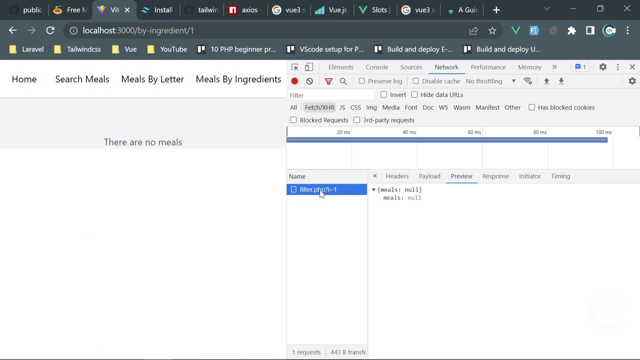 assign it to an array now if we click on chicken this shows there are no meals all right which is logical but why there are no meals for chicken not sure if i click right here and we see i1 how should we make request 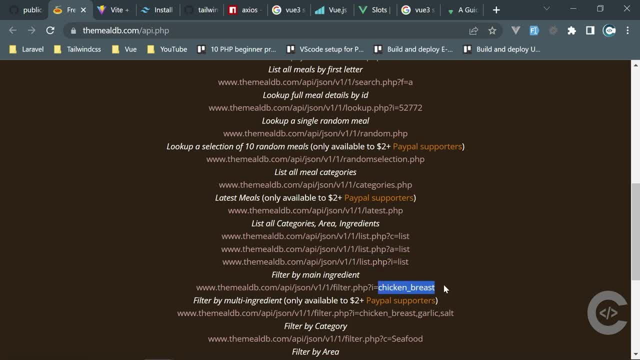 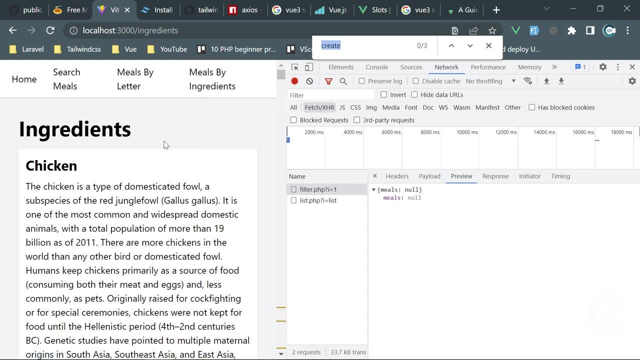 uh-huh we should we should pass not the id but the actual text probably chicken 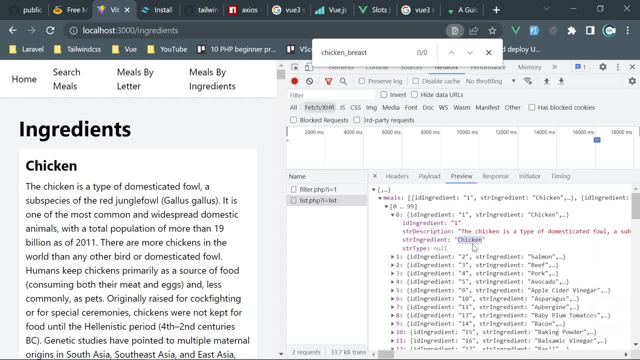 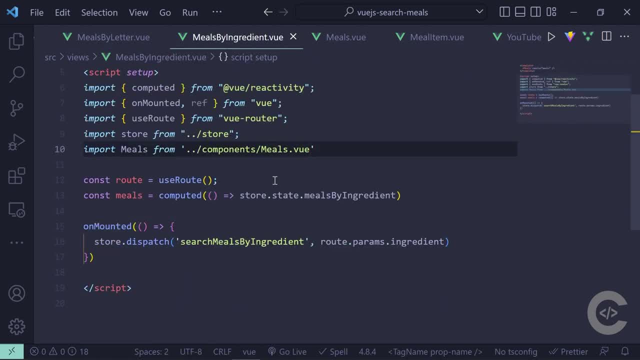 here we have all the ingredients and we should probably pass chicken so if we go in the uh not the ingredients but ingredient meals by ingredient and inside the ingredient we're going to have text so now we need to go in ingredients and when 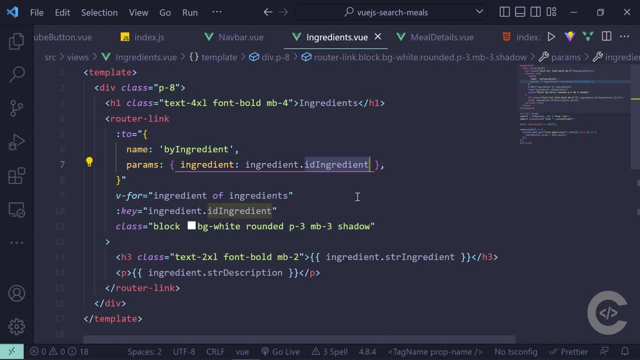 we set up this instead of id ingredient we should pass we should pass str ingredient okay let's test this now and here we saw it 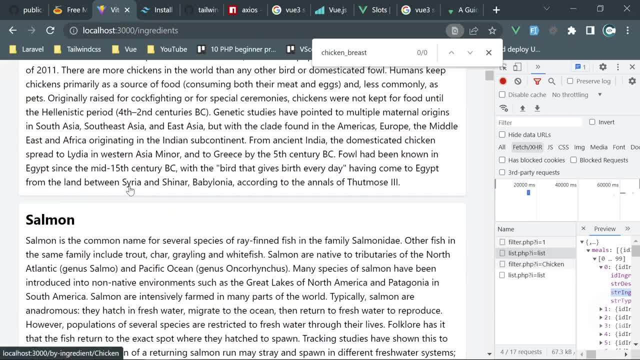 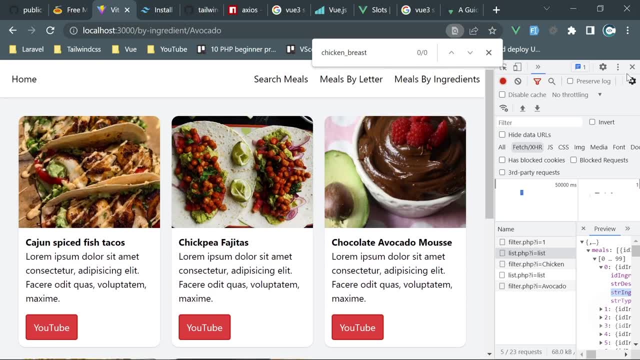 here we see chicken receipts and now if i click avocado i see i think something related to avocado if i go inside we see the details for that 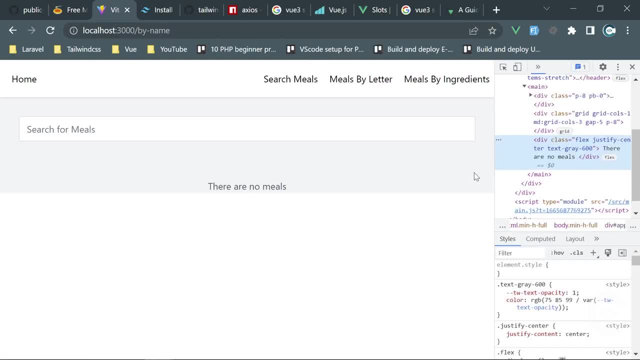 all right one small thing to fix uh it's almost no not almost but it's more than 3 a.m and i will not sleep if i won't fix that or it's over i don't know which one i'm going to play some other football match БакING jäей もう еще маленький на én bathing Regards 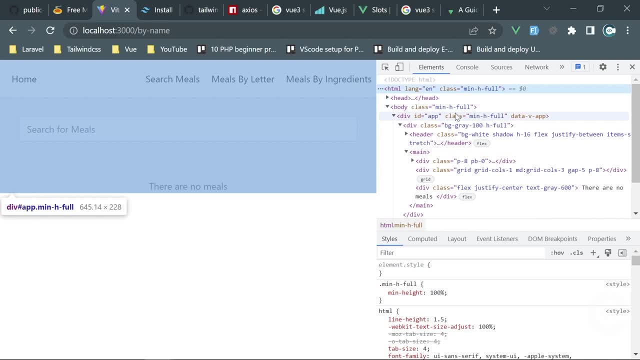 yağ is this hate problem so mean hate full why is that we just give it age full on 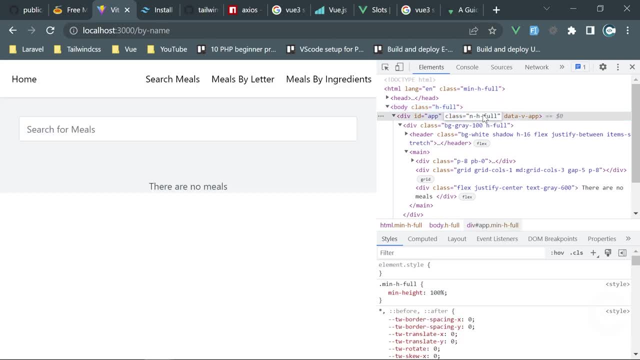 body and then age full right here we need to give we need to give a background gray to maybe body 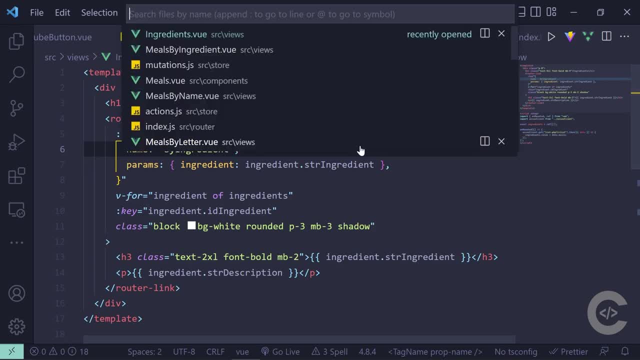 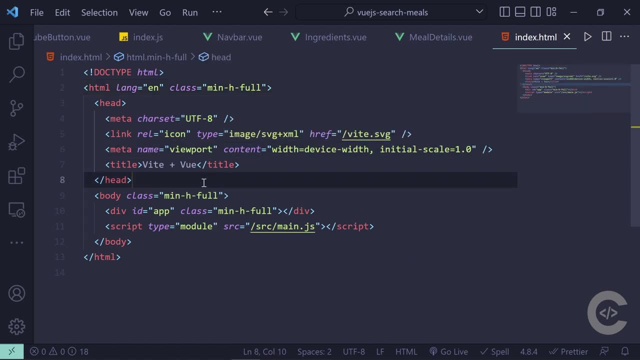 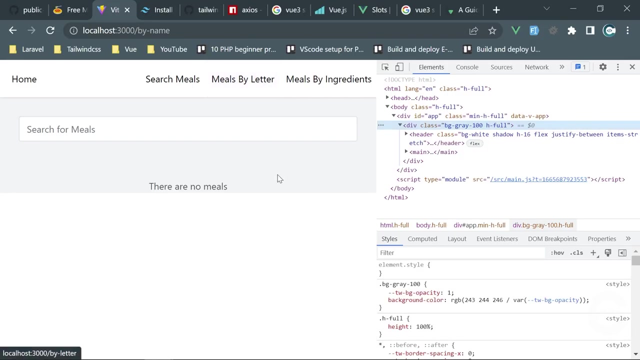 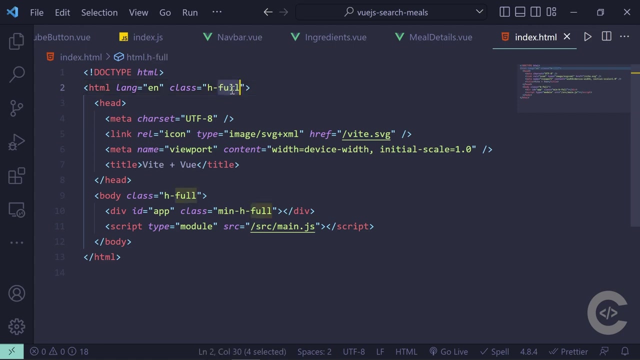 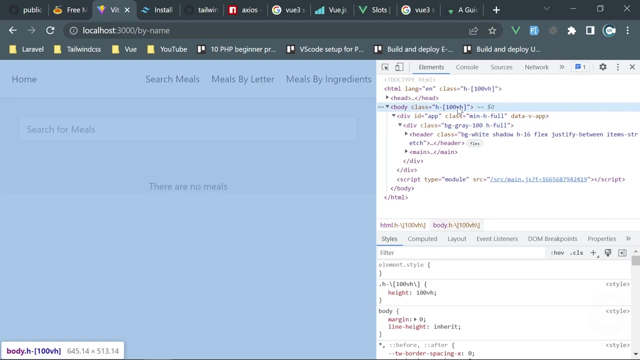 not this one okay if we now open index dot html and and we have to change some things here let's change this into age full or we give it 100 vh this is the h let's give it 100 vh here as well 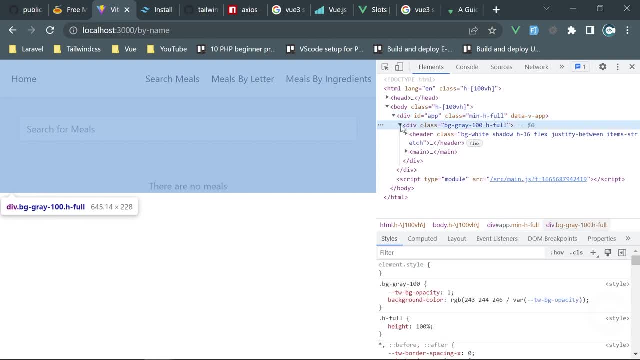 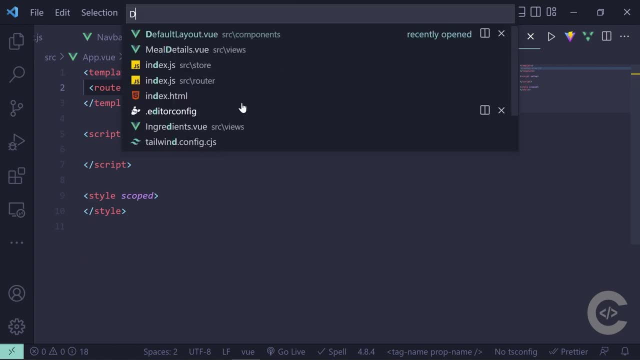 and there is another div which i don't know why it is necessary if we open now up view uh no it is probably in default layout i think we don't need that 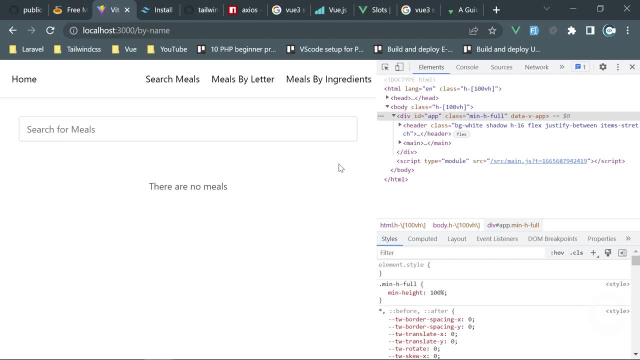 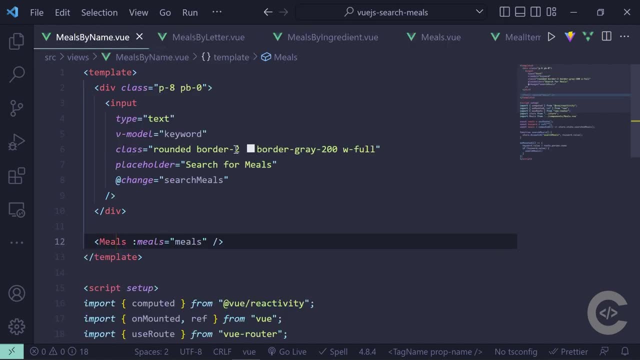 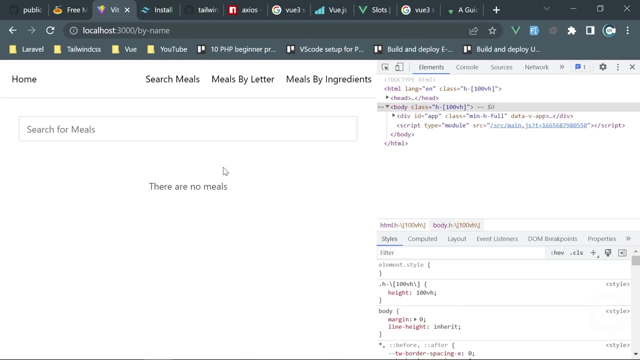 okay now this is fine however if we open a component by name here we have input and the input needs pg white it doesn't have background white or it does not sure 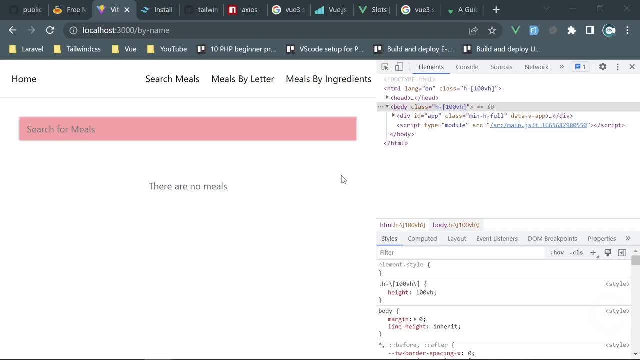 okay probably i just can't see it normally anymore 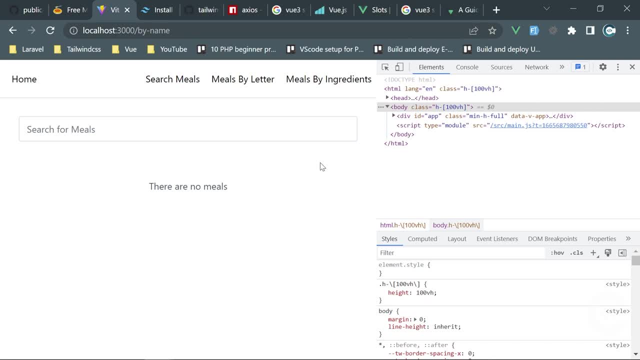 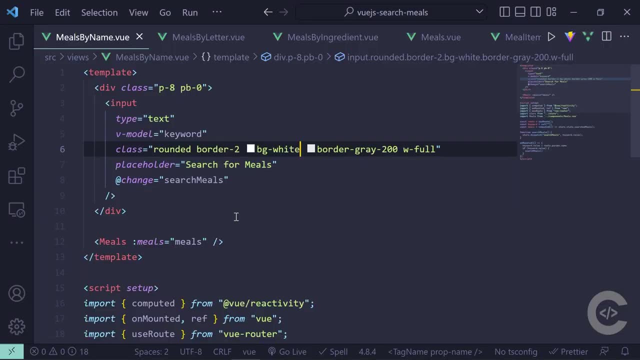 so it probably has this pg white but what is the actual background color i think it is also white in this case so if we 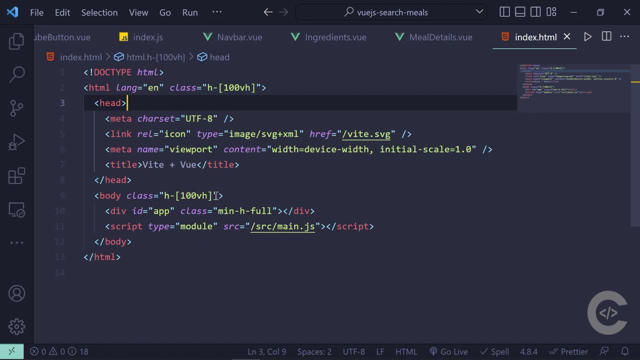 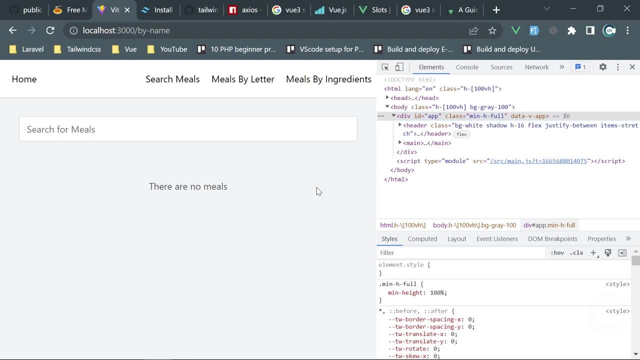 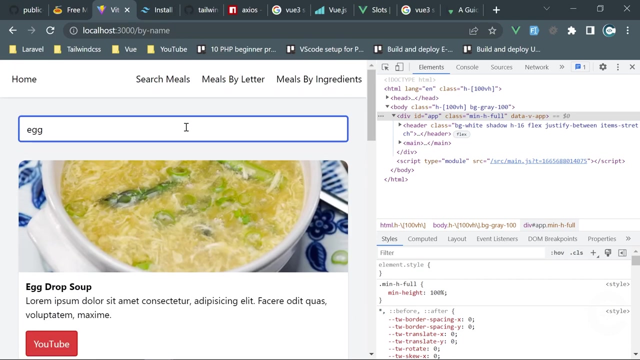 open now index html and go in the body and i'm going to give this pg gray 100 okay this is what i wanted so there are no meals i search something hit the enter it finds now if i just delete 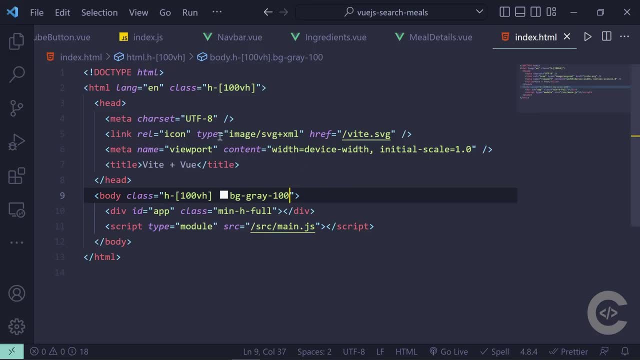 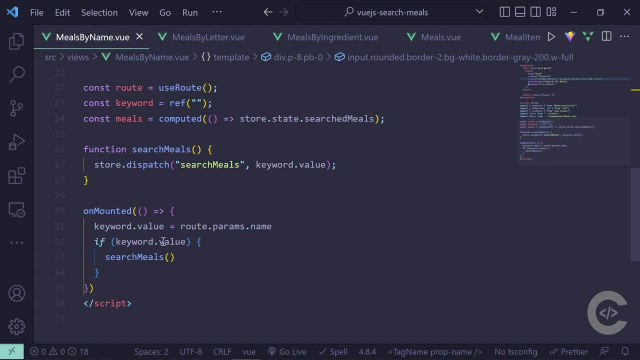 it then it should write there are no meals so if we open again by name here on change search meals is called on change and we have keyword here so basically we should not dispatch 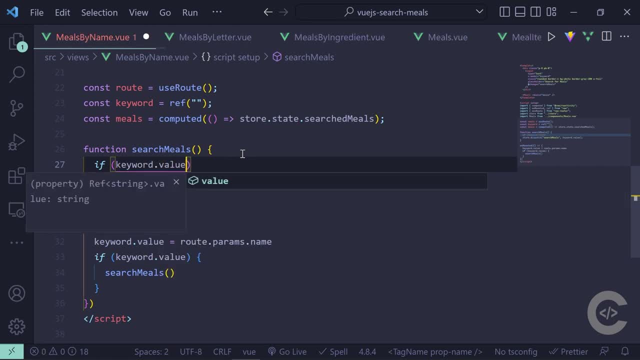 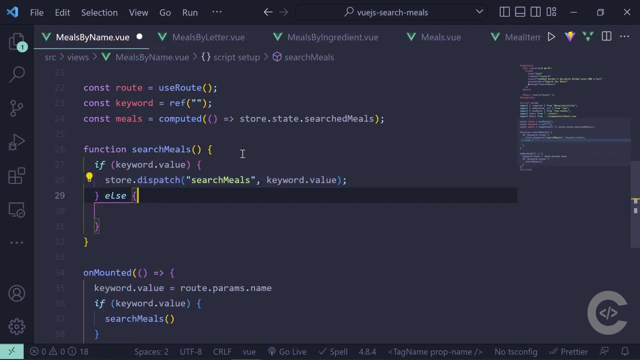 if if keyword value exists we dispatch it otherwise we simply remove all the meals okay in this case we can directly call mutation using commit and 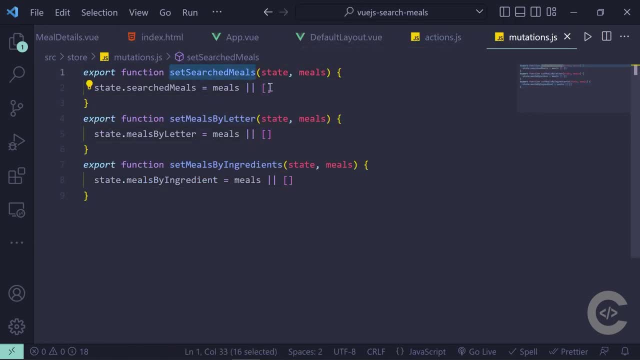 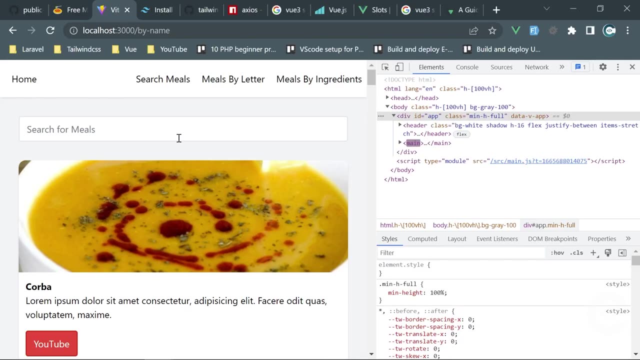 if you open mutations we see set searched meals so we set searched meals to be empty array if the keyword is empty so if we search for egg hit the enter we see that if we delete and hit 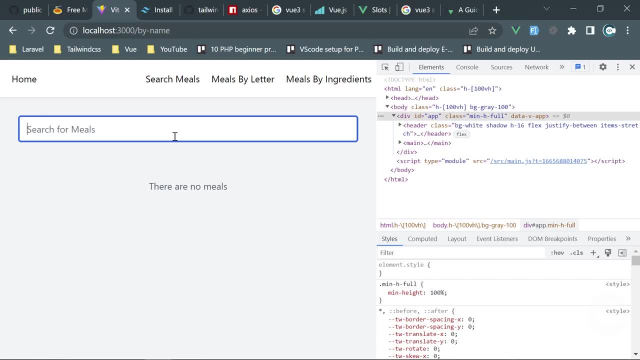 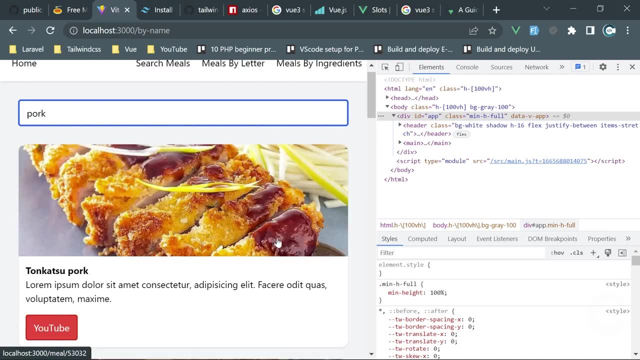 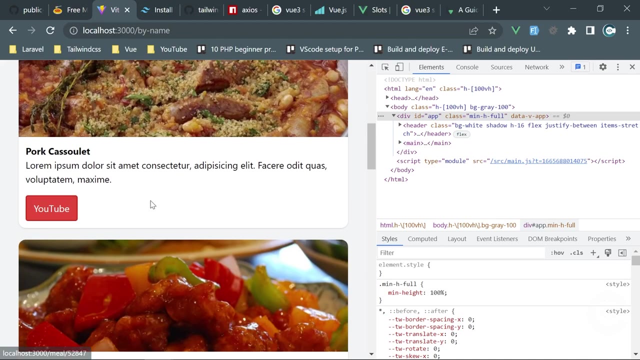 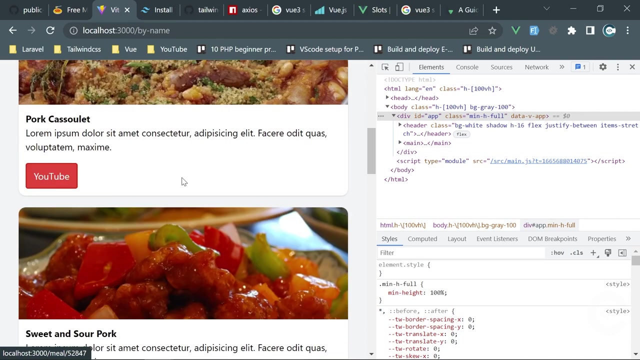 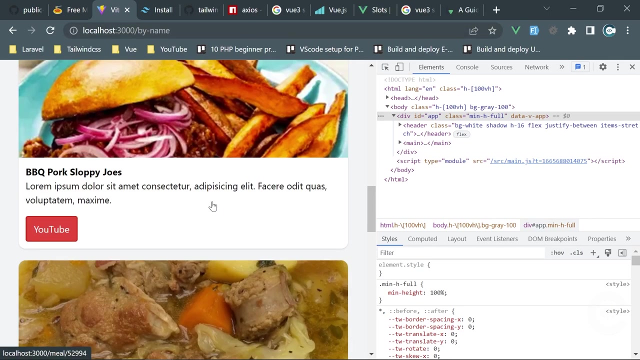 the enter we just reset everything okay however the idea of using view x was that whenever we're whenever we search for something and we find that then we go on another page and then come back we should see those receipts uh however not sure if yeah i think this is this is the filtered one however this is not affected in the url but yeah that is probably a topic 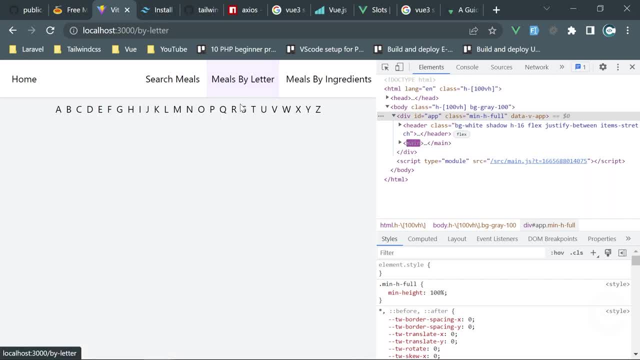 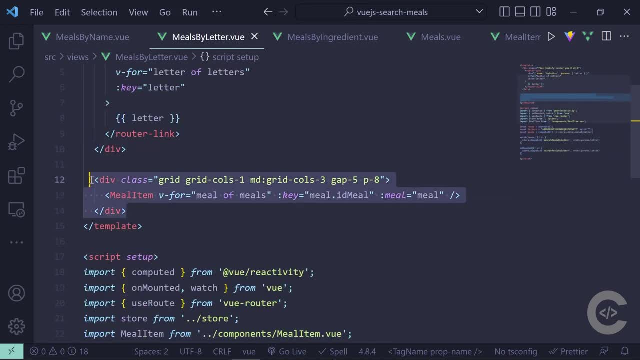 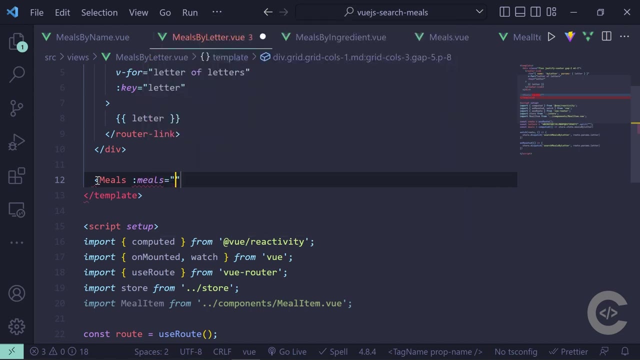 of different video so we have meals by letter let's fix that by a letter and we need to change this and use meals component here as well 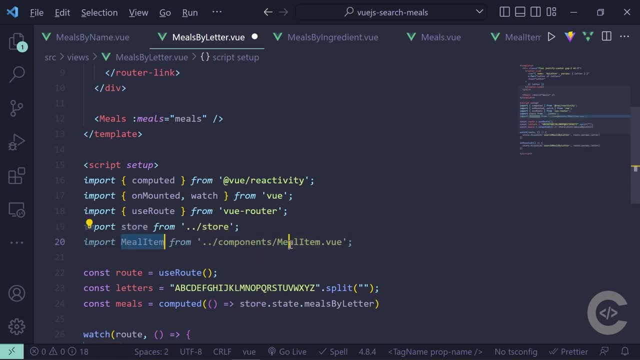 like this and let's import meals 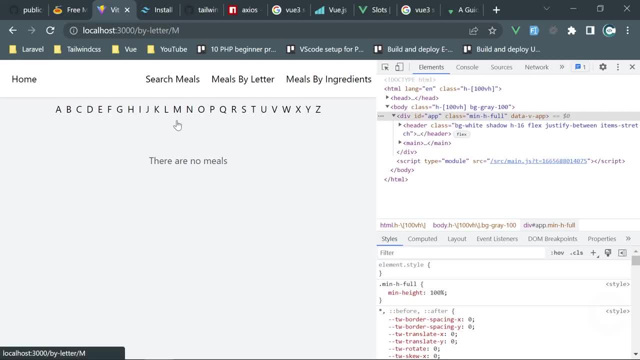 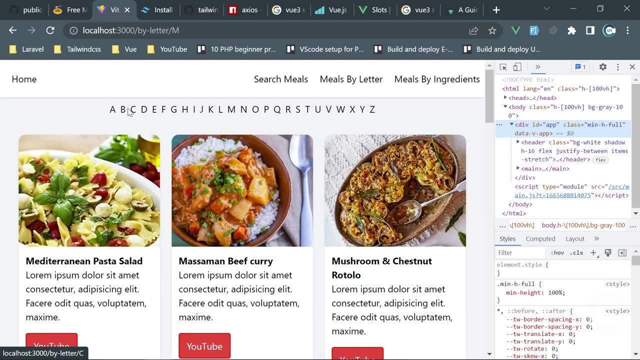 we save this and there are no meals if i click m we see meals with main ingredients starting with m and go into a and we see all of them 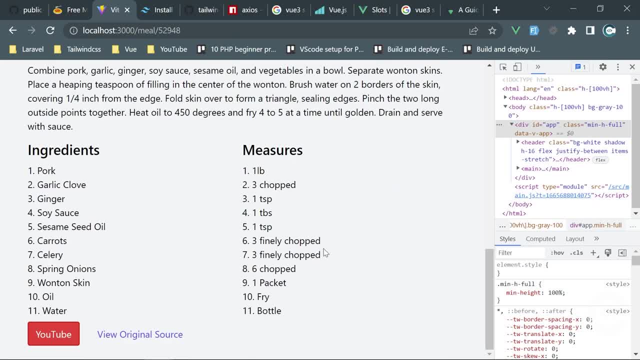 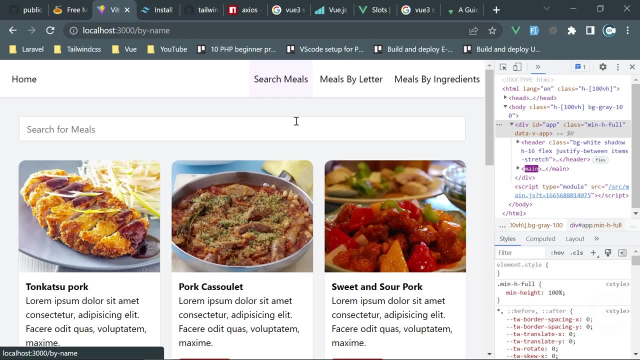 and if we just click inside we see the details page and if we click those links are also working okay so this is the receipt search for meals we have letters and ingredients 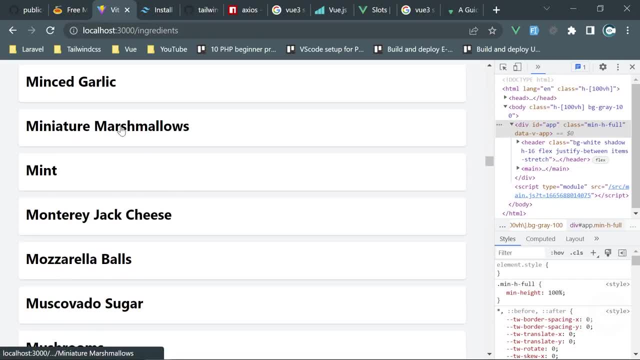 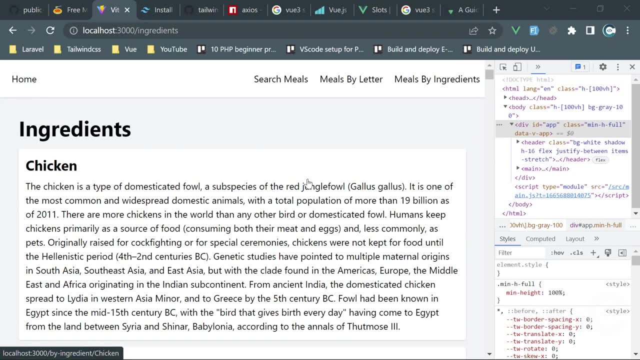 so we have all the ingredients and and we just click on them and just display them okay let's i'm gonna do one very minor thing and 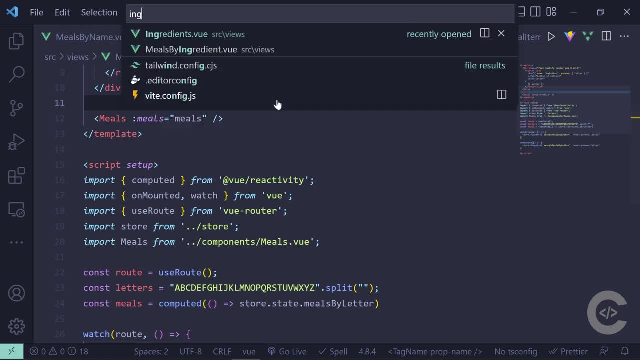 then i think we are done so in this ingredients page i'm gonna add an additional search field 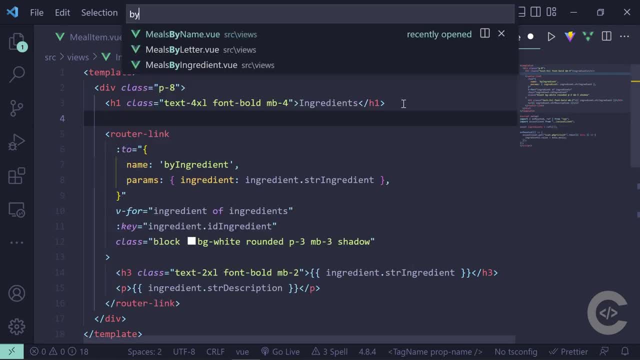 let's copy this from by by name 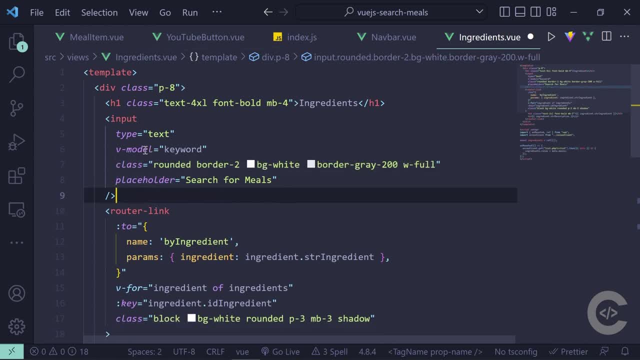 like this and let's remove this change it has a vmodel keyword search for ingredients 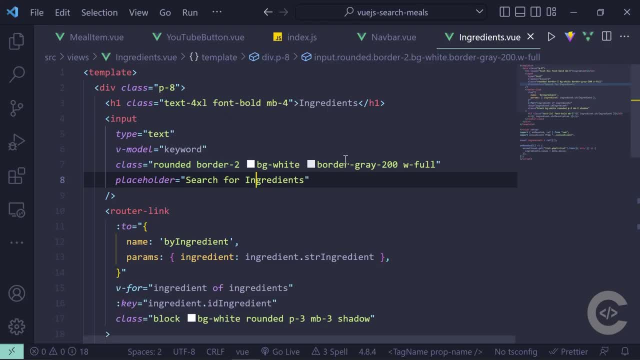 let's save this and let's give this margin bottom of three 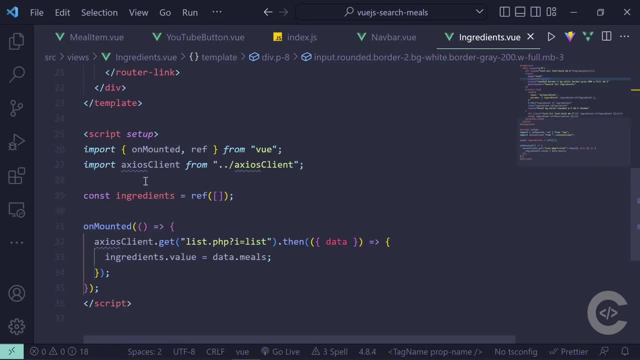 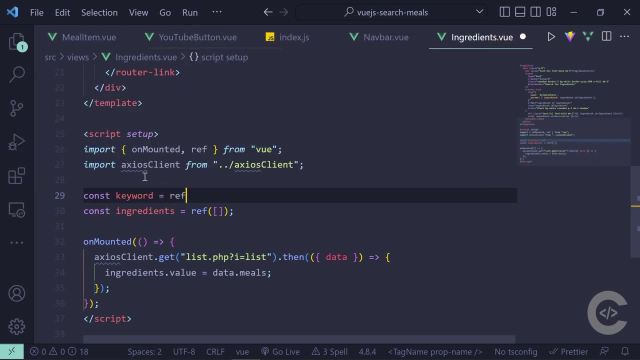 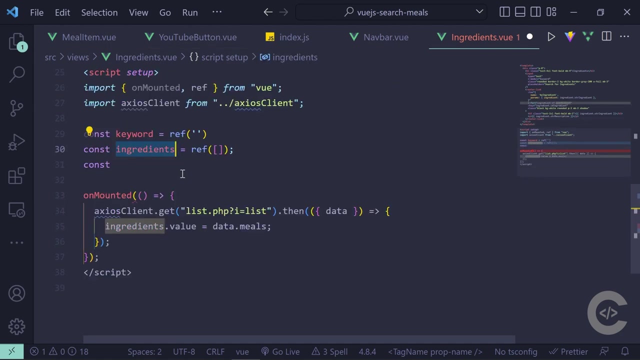 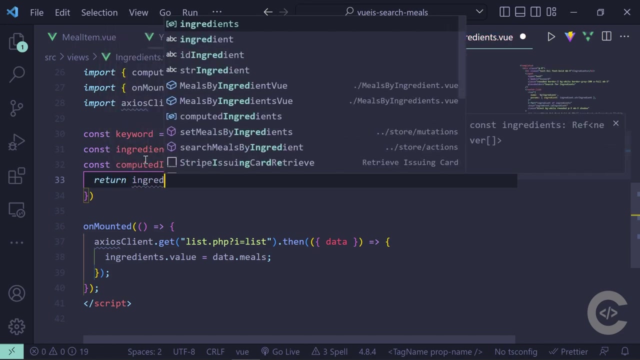 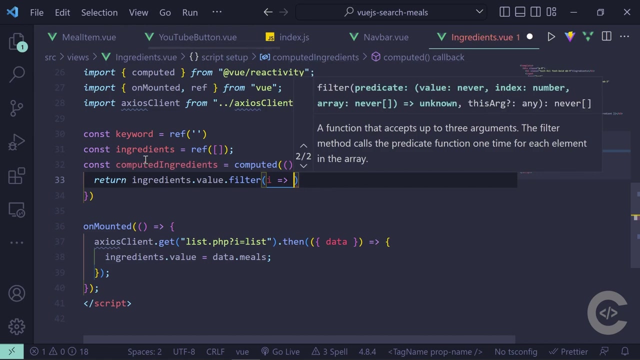 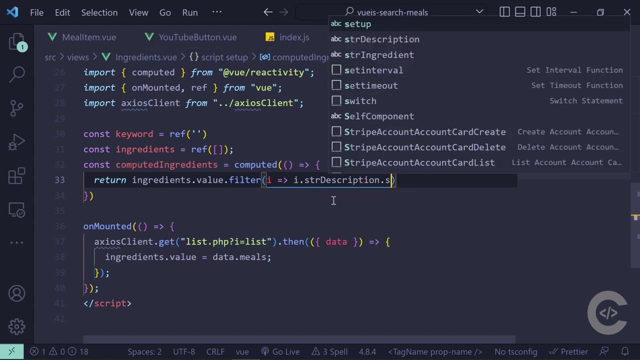 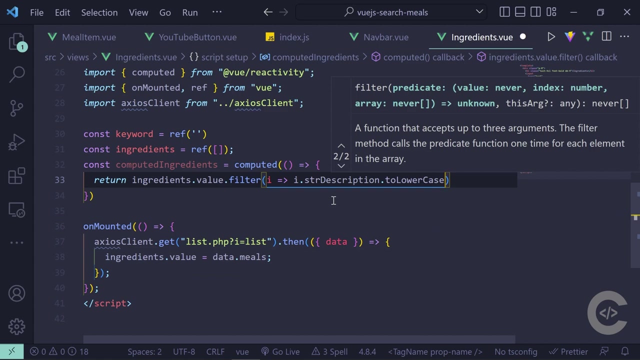 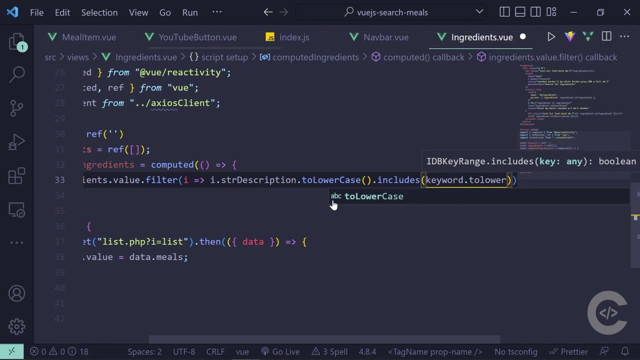 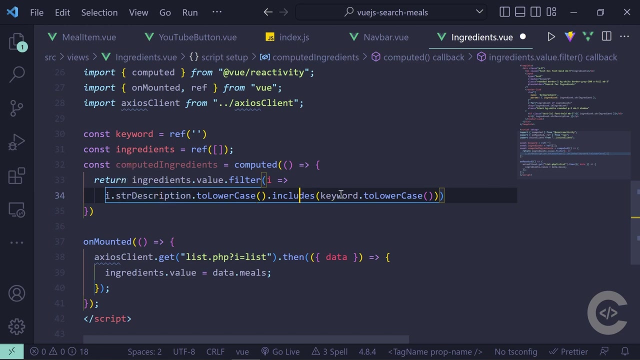 we see that and we have keyword let's declare const ref const keyword corresponds to ref and now i am going to filter and create computed ingredients so const we have the ingredients by the way which is yeah which is okay as it is and i'm going to create like computed ingredients all right that's going to be computed and right here like that so let's go and because I'm not gonna do entire product needs out of this so what from here i'm going to return only those ingredients ingredients dot value filter i whose text or description matches the keyword okay if i str description includes we can run to str um to lower lowercase str description to lowercase if that includes uh keyword dot to lowercase to lower case if that is if this is the case let's move this down if ingredients ingredient description to lowercase includes keyword to lowercase or if str ingredient to a lowercase includes keyword lowercase then we return only those 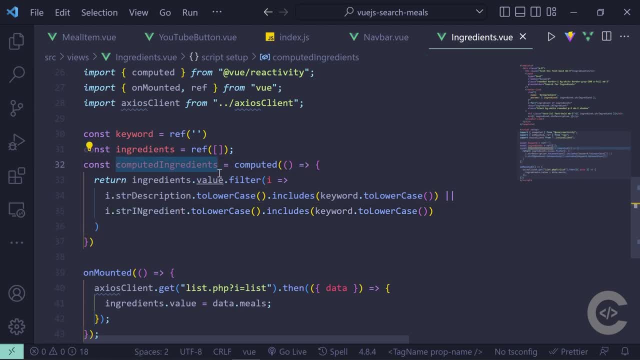 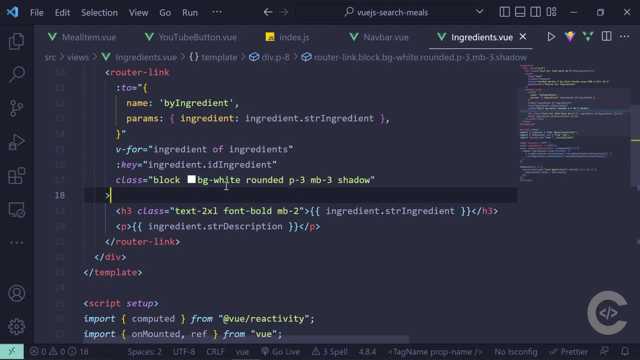 ingredients from here and now we can use computed excuse me i literally lost my voice so right here we need computed ingredients 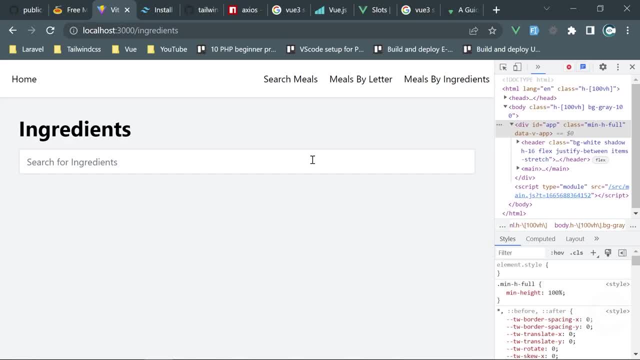 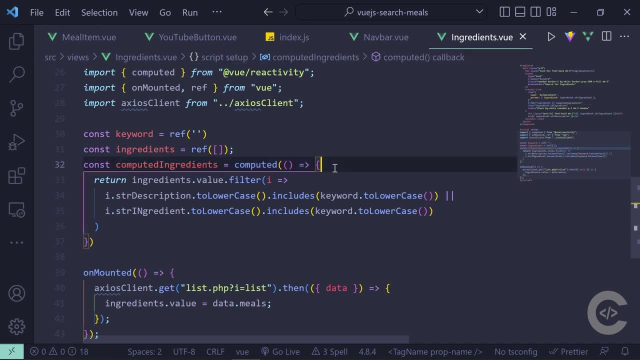 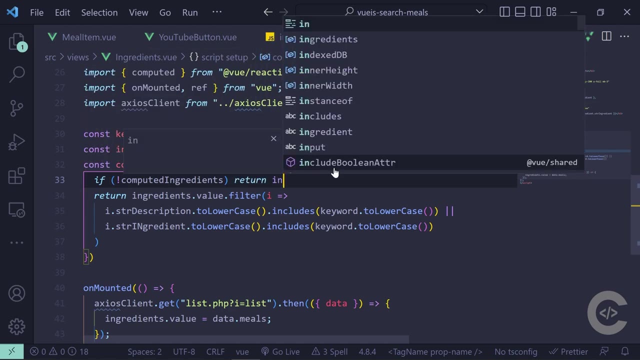 and additional check will be if that does not exist we will return ingredients 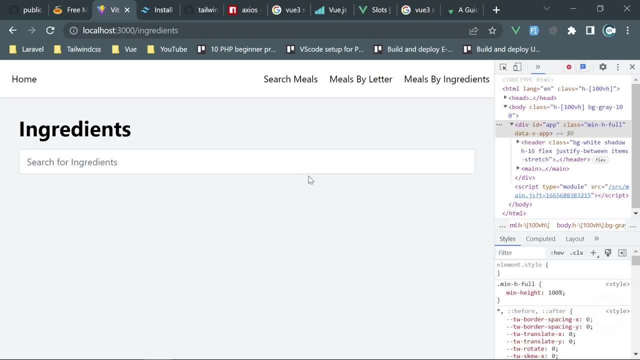 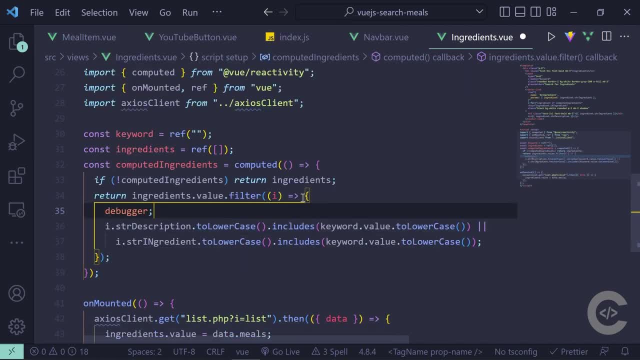 what is i and what it contains okay 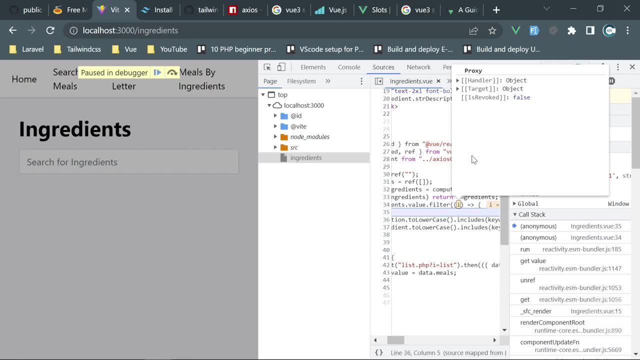 that is str in description str ingredient str description 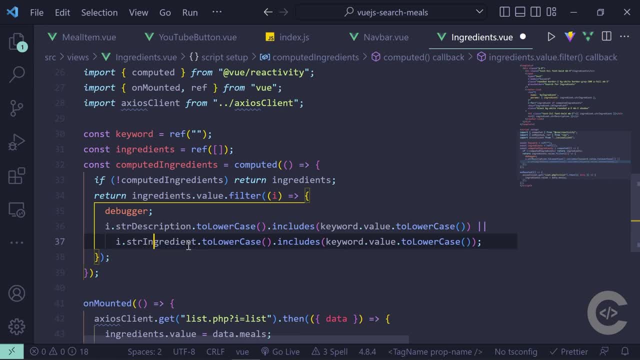 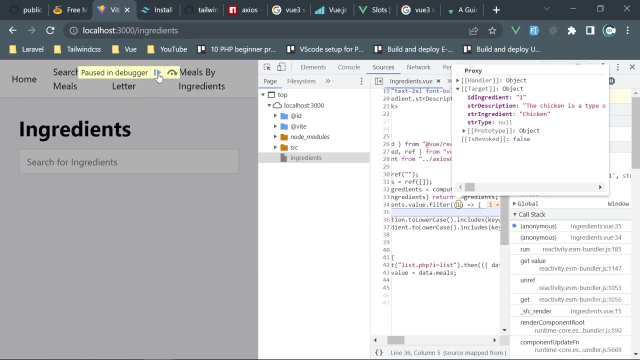 here i have typo okay and we can return we have an error 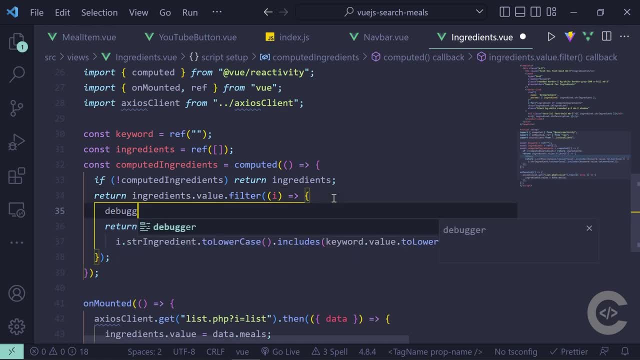 it complains about this str description um it complains about this str description 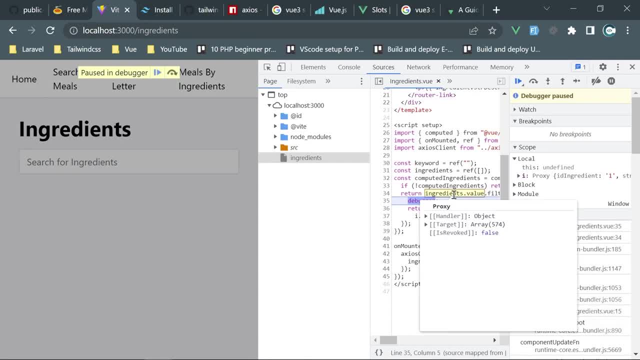 so let's see it exists 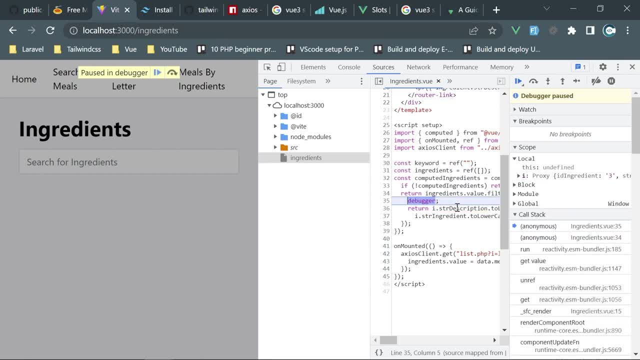 exists yeah for some of them it might not exist 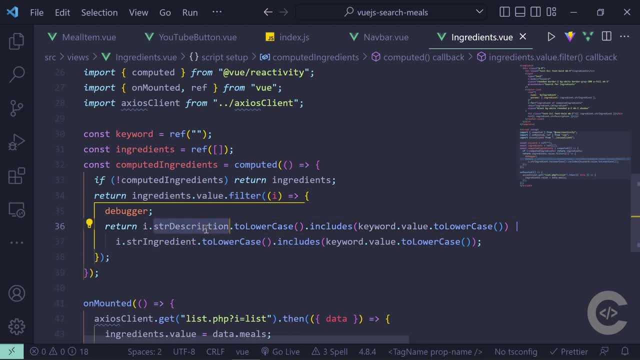 yeah it might be null even now 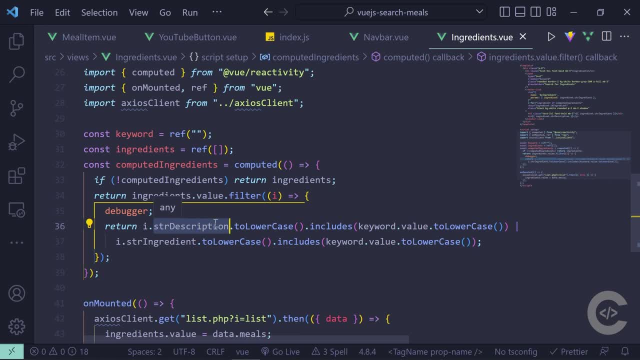 in this case in this case we might assume that if this is null 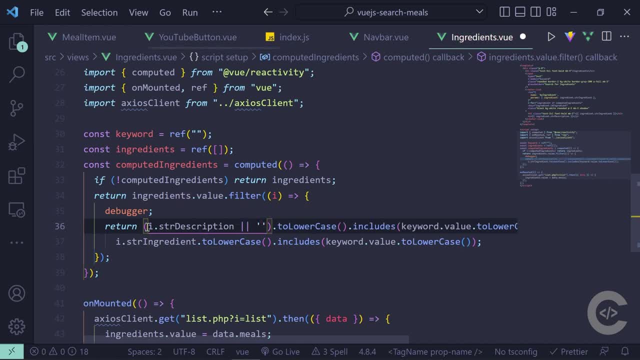 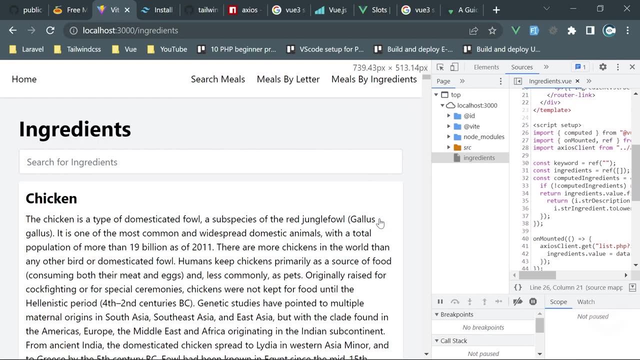 it may stand still for example so 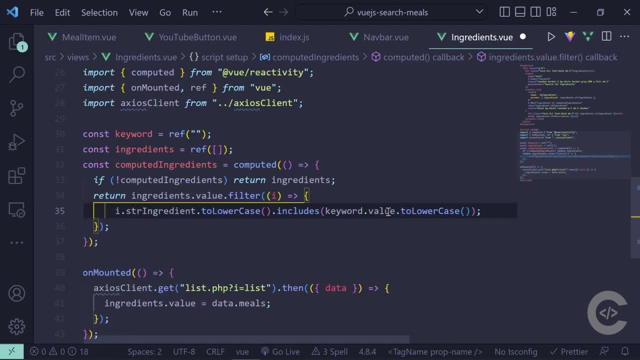 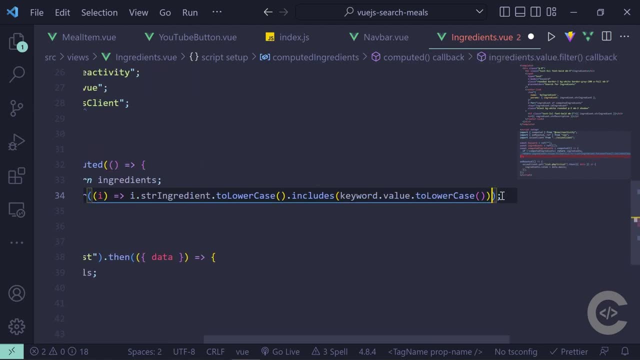 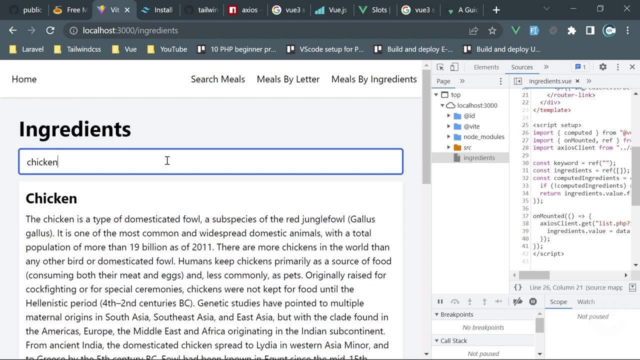 i i i i kiss kiss kiss kiss kiss kiss kiss this in a single line so we just reload the page and we see chicken so we can search for chicken 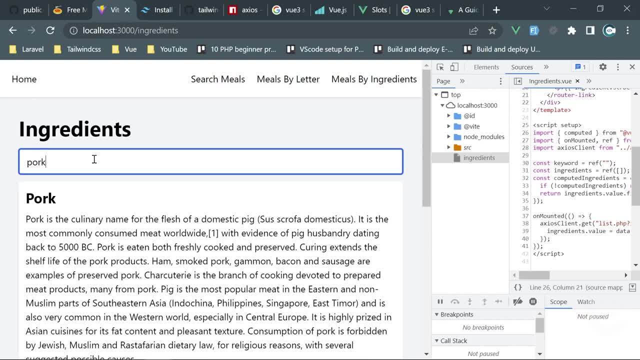 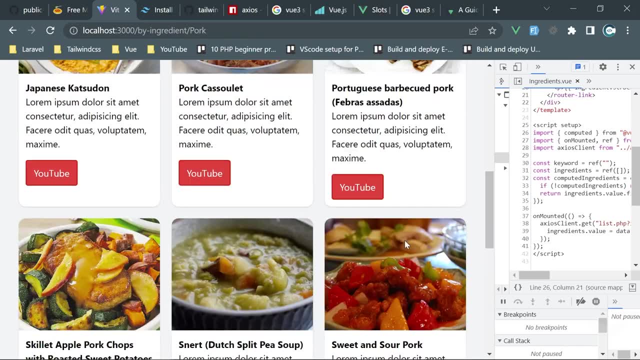 okay here we have it so let's search for pork here we have it and then we click on pork and then we find all the ingredients for this pork okay i made few improvements in this project 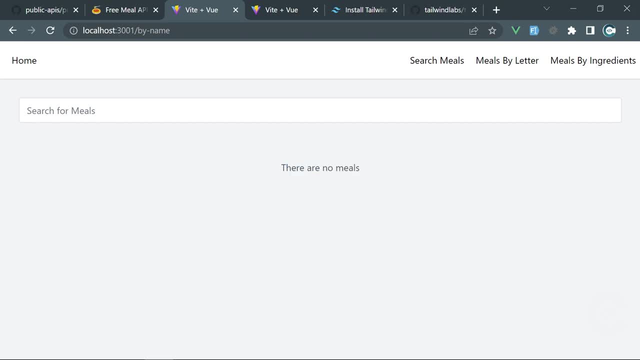 and this is how it was looking when we stopped on the home page basically everything was empty 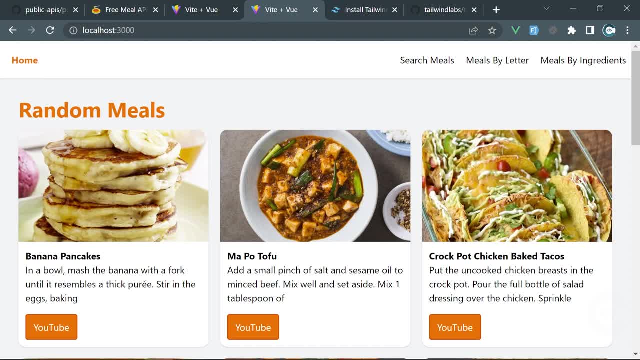 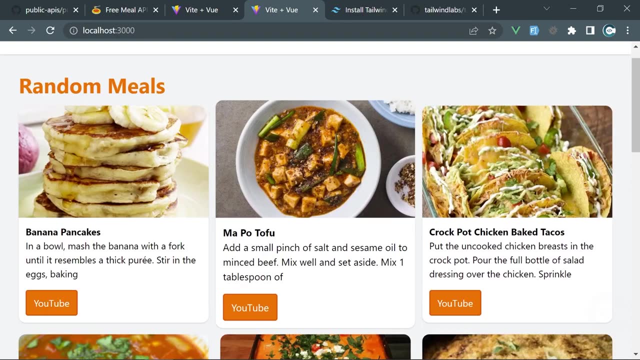 and this is the new version so the most changes basically i made was css related i added either html related or css related i added titles to every page and i made everything basically orange because this is the color i think suits to this type of website and we can go we can open now the the 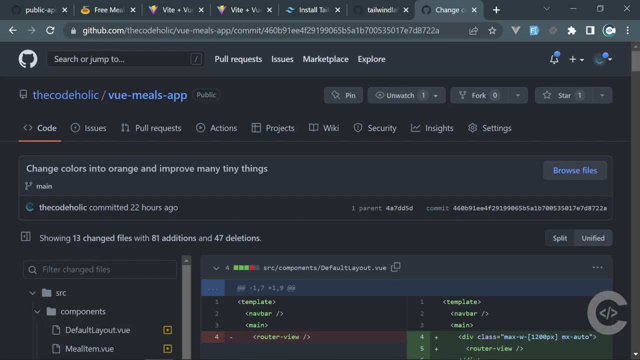 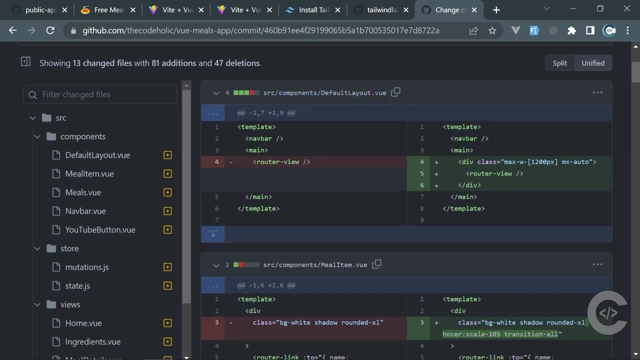 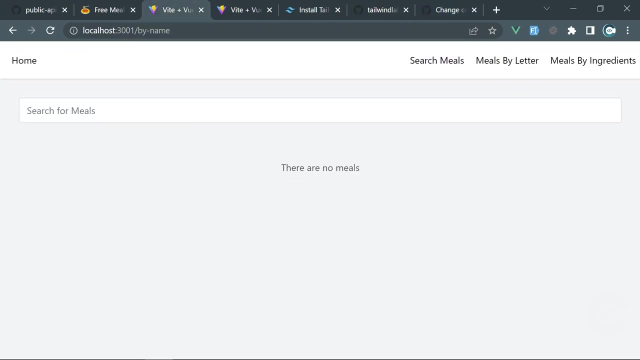 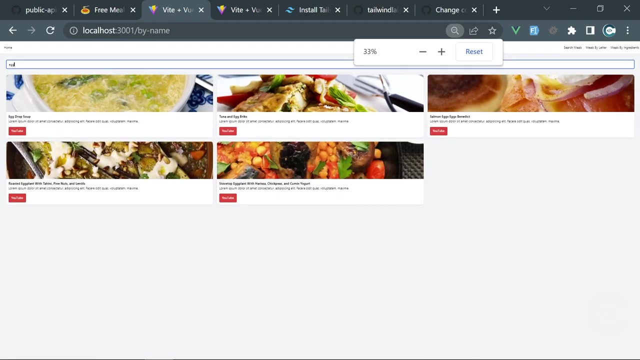 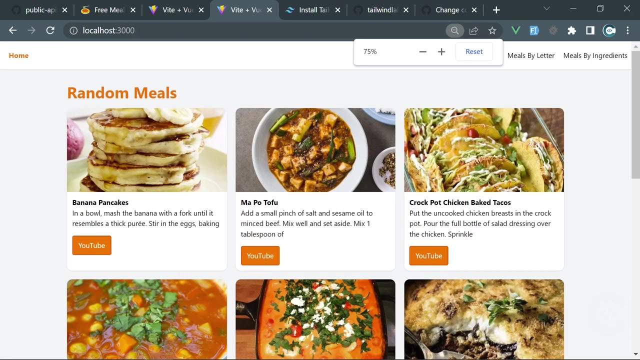 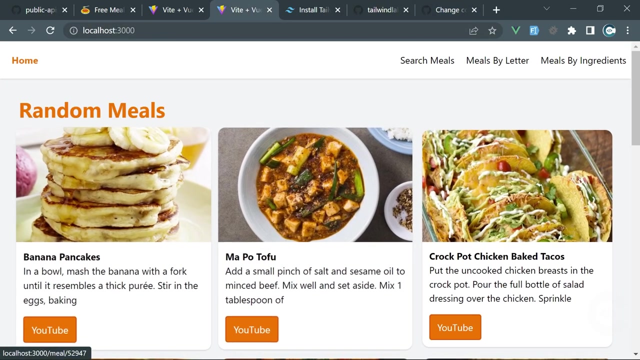 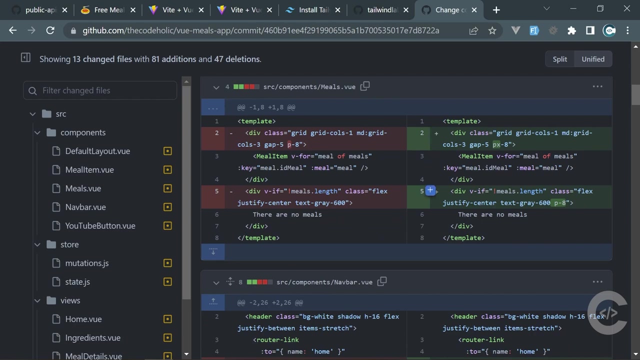 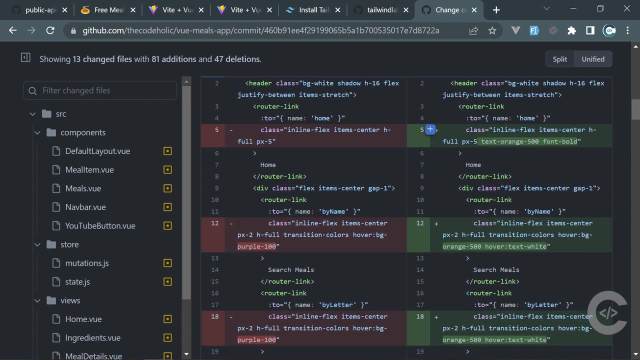 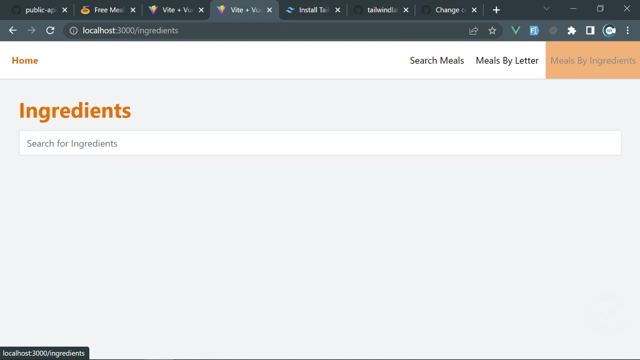 vs code and basically go through those changes or actually i'm going to show these changes on the github repository okay on the comments basically the main router view which was in default layout i restricted its width so in an old version basically that was stretched on a full width even if you zoom out we see the search bar and if you search something that was stretched on a full width it was not nice on our version we have it inside a container okay this is how it looks like which i think is much better the second version basically is that on image hover we have this nice effect on card hover we also have increased some or increased or reduced some paddings so those are very minimalistic and small changes and change the colors into orange 500 in almost all places where i was using the color even the input fields are now changed and i also removed descriptions from these ingredients let's go through these changes 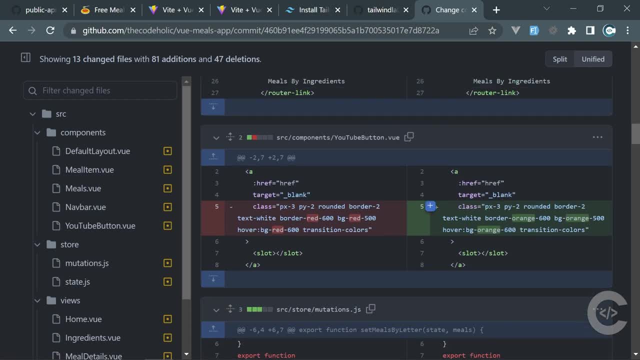 okay those the purple color was hover purple color was changed 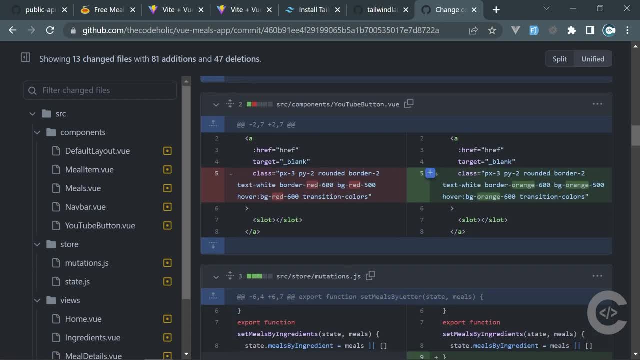 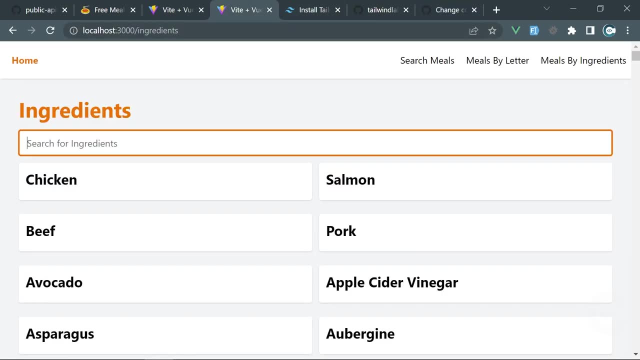 and here we have this youtube button which was changed into orange and down below uh we i basically set the ingredients so whenever we have these ingredients i whenever we click on 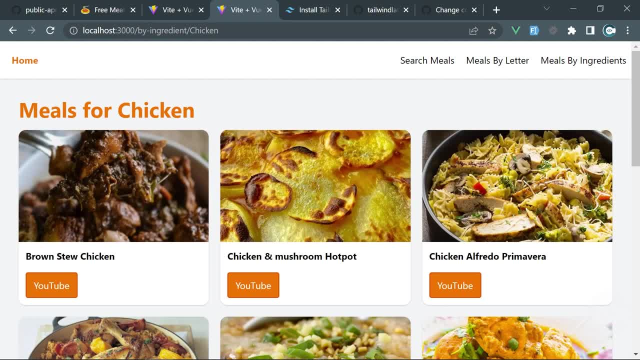 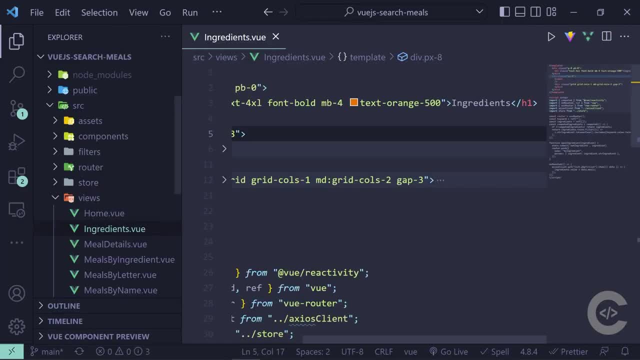 this ingredient i set the ingredient in the view x and on the second page i use that okay this is something i want to show you in vs code so if we go now in ingredients page and scroll down below 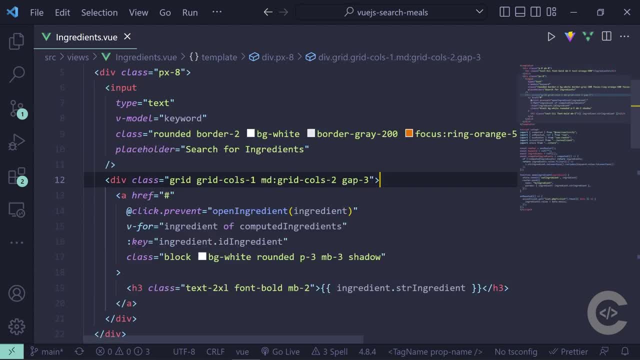 whenever right here on the ingredient we had a router link and that router link basically okay let's check it in github repository where is that 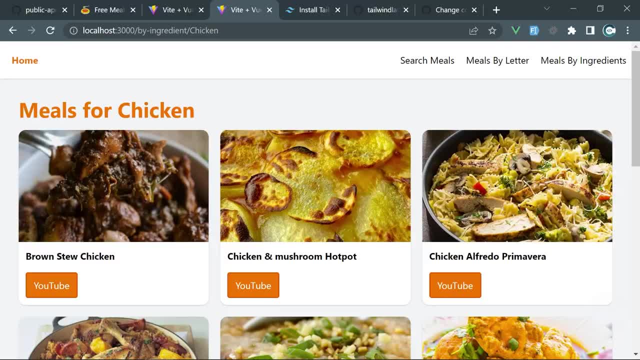 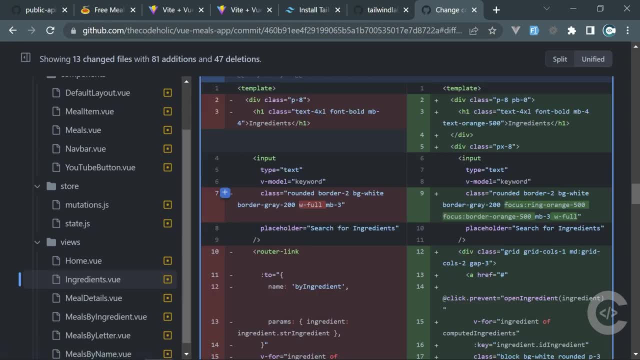 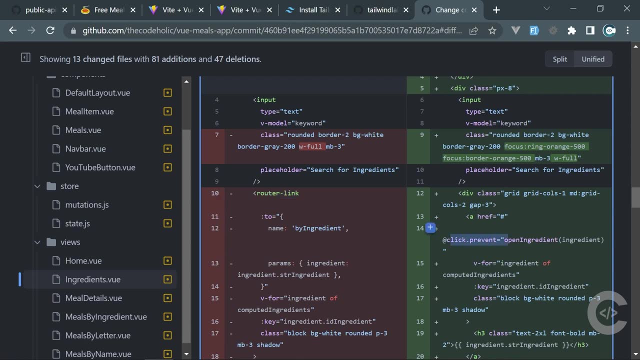 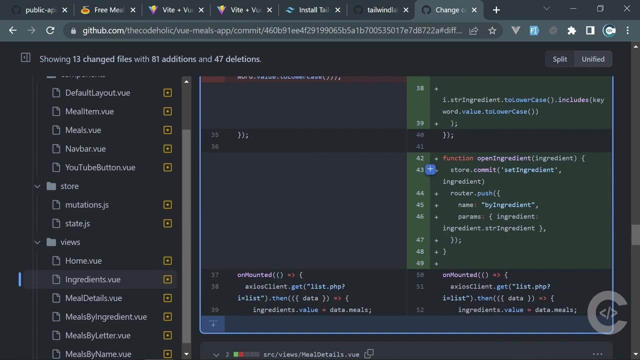 here it is all right so if we click on the left side ingredients so previously where it is previously we had router link with two but now i removed that and we have now click open ingredient okay if you scroll down below we have this open ingredient which will commit 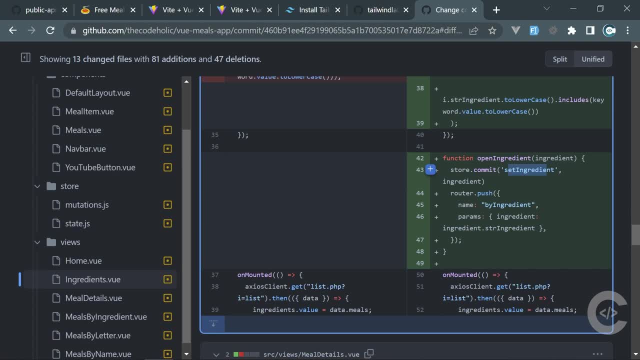 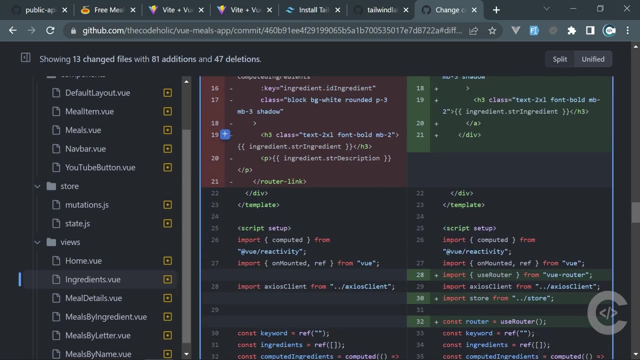 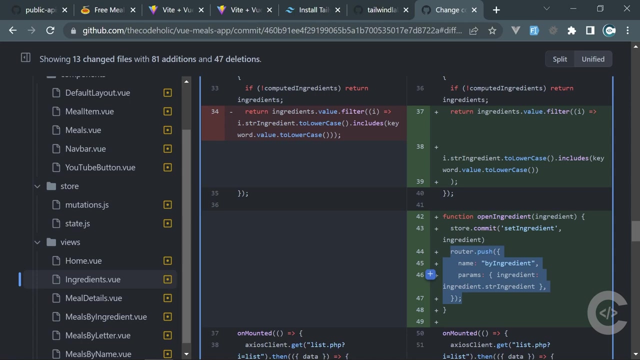 inside the store set ingredient the set ingredient was also added in this picture the store and when the set ingredient is called it's going to also call router push and it's going to update the url like the previously router link was only updating the url but now using javascript we are first committing this in the store saving this in the state and then updating the url and if we now check state right there we have ingredient which is an object and if we check 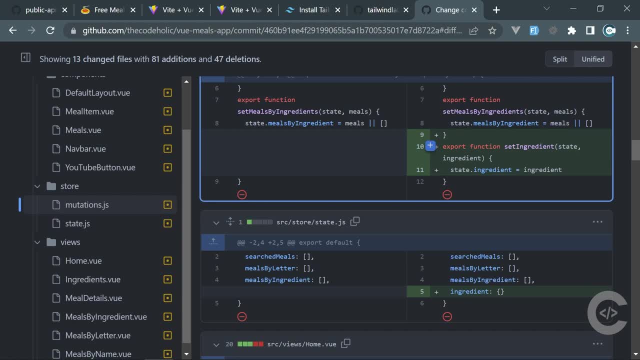 mutations we have right here set ingredient okay which accepts the current ingredient and assigns 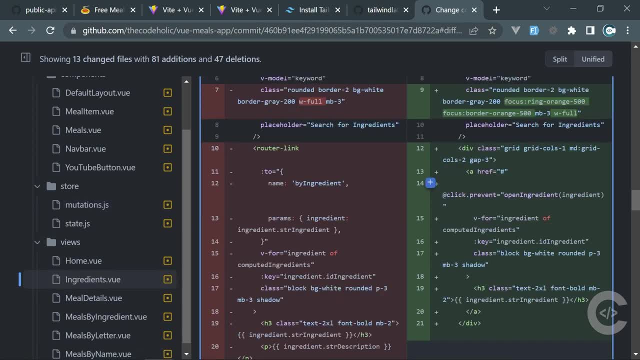 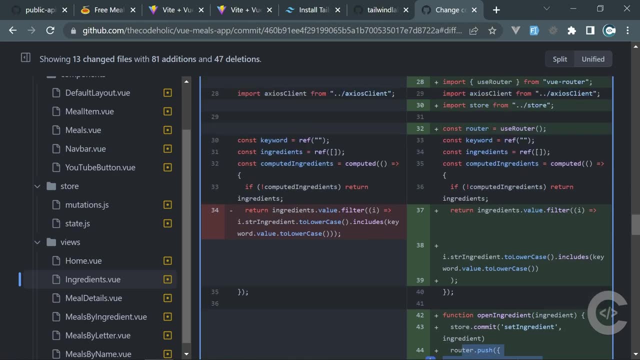 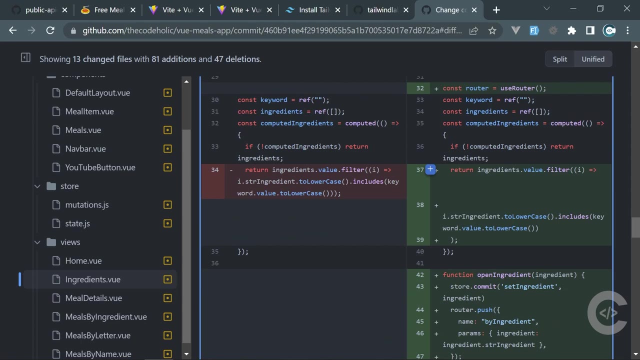 this into ingredient and again if we check ingredients page right here we have the current row we use the current router because we use router push right here and we used also store right here and from the store we basically where it is 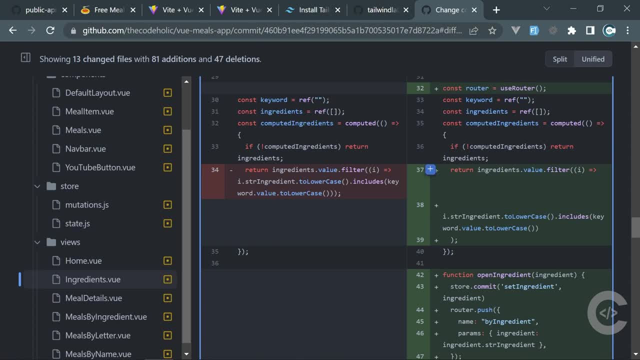 this this is let me zoom out slightly 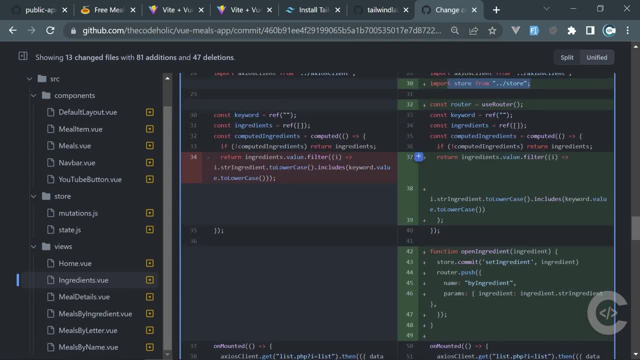 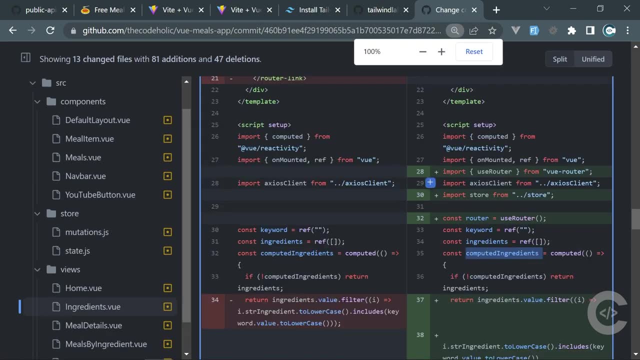 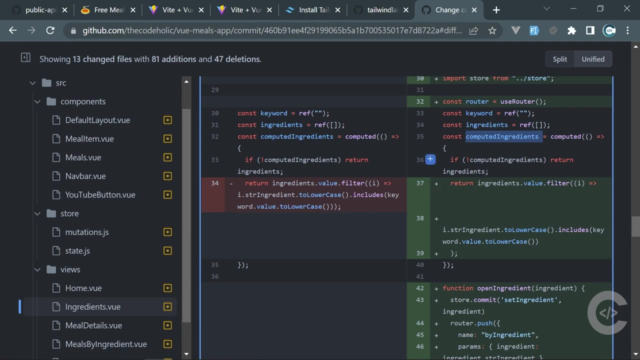 ingredients yeah computing computed ingredient okay this is it so for computed hold on where is the computed property now these computed ingredients are for search but where is the 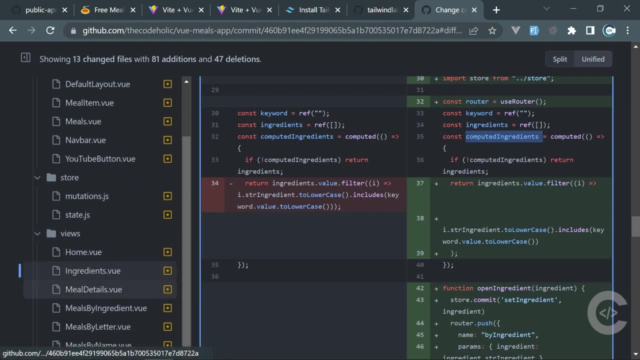 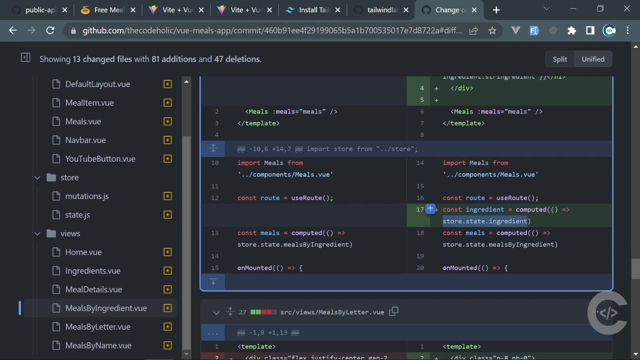 current ingredient oh i'm sorry i'm sorry that is in meals by ingredient sorry so right here we have this ingredient this ingredient which comes from store state ingredient and now this ingredient is used meals 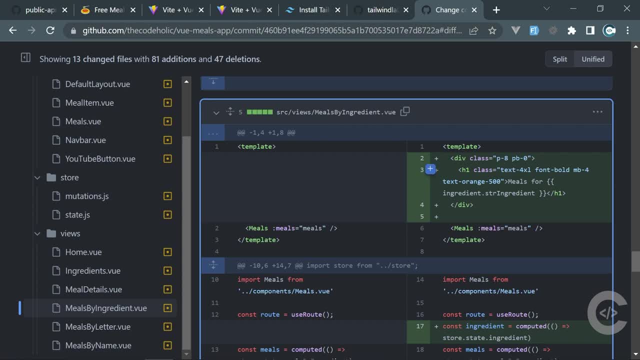 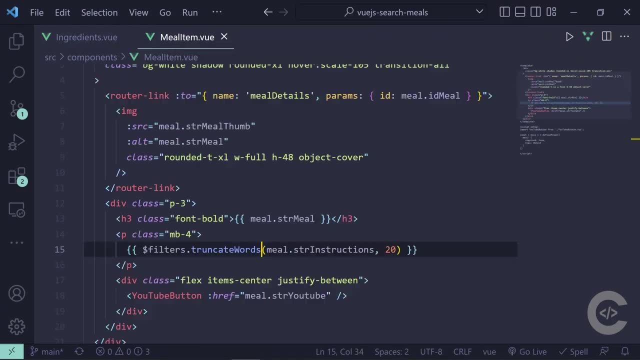 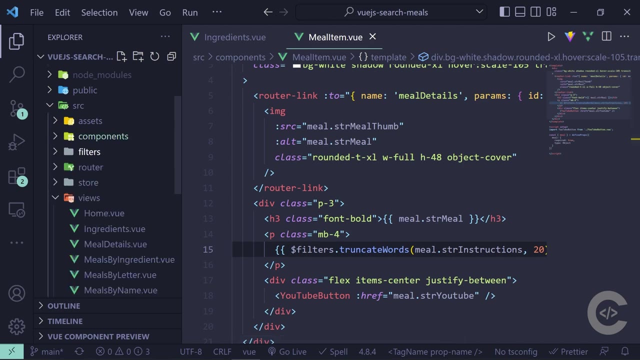 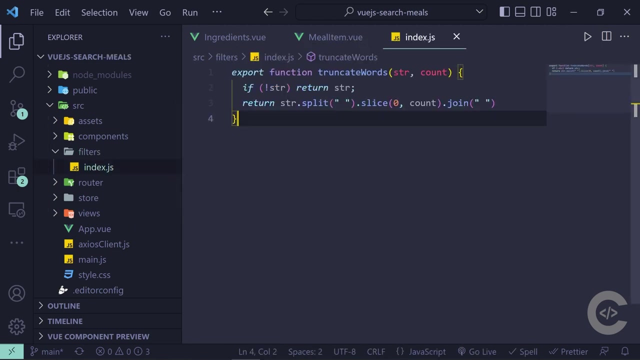 for ingredient right here okay now every page has a title this is one interesting thing second interesting thing is that if we open meal item we are using right here lorem ipsum description and i created filters for that so the single filter basically i created filters folder inside the source and right here we have this new filter export function and i created filters for that so 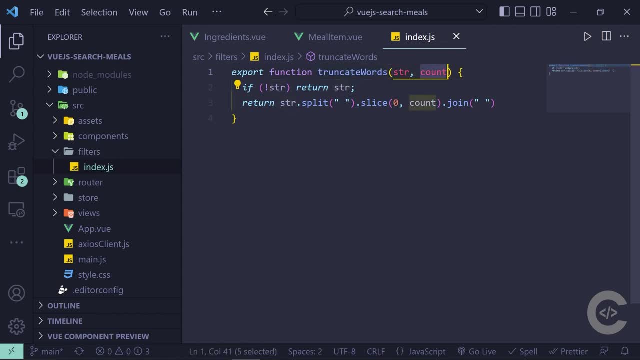 truncate words it accepts string and count how many words needs to be truncated if the string doesn't exist we return string if it exists we split it using space then we take out the count number of words and then join with space again and finally this can return number of first number of words 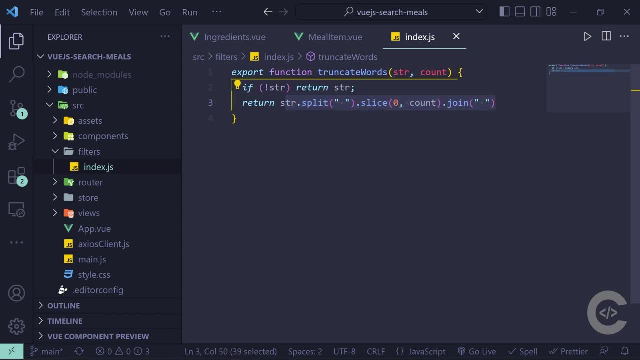 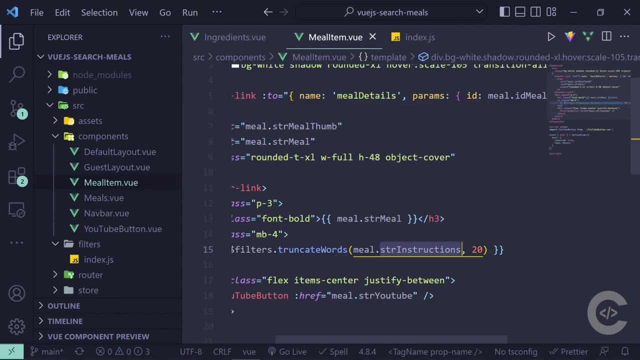 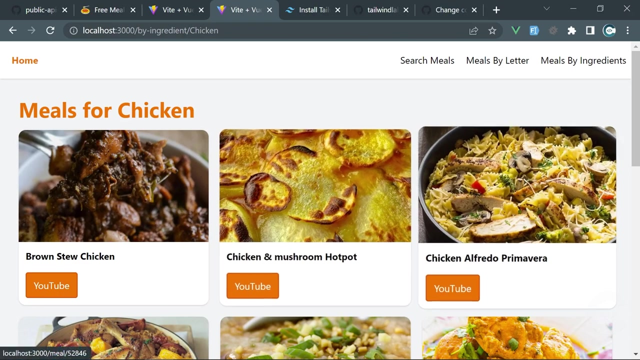 basically without this truncating the description instructions we are too large and if we basically go now in the meal item we are using meal str instructions if we reduce this into 10 then we have all right here reduced by the way those meals don't have this instruction if we go in the home page 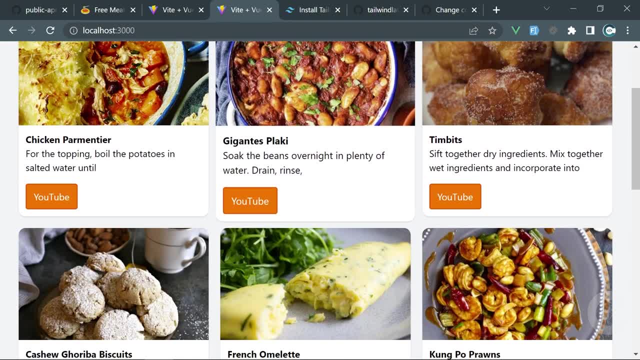 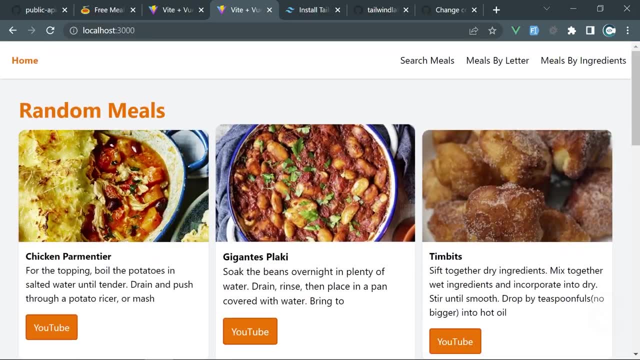 that is something else we did we didn't have home page before we see now 10 words in the description description okay let's change this into 20 and now we have 20 okay this is the home page which we also implemented let's open 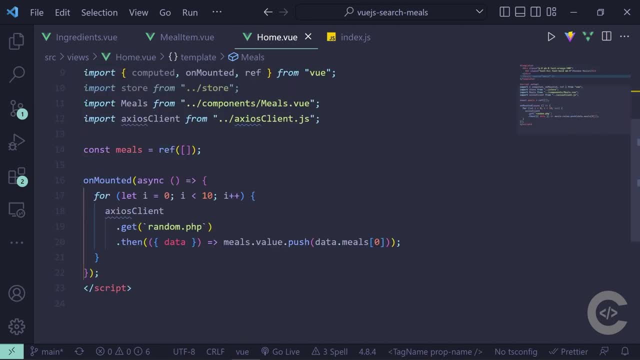 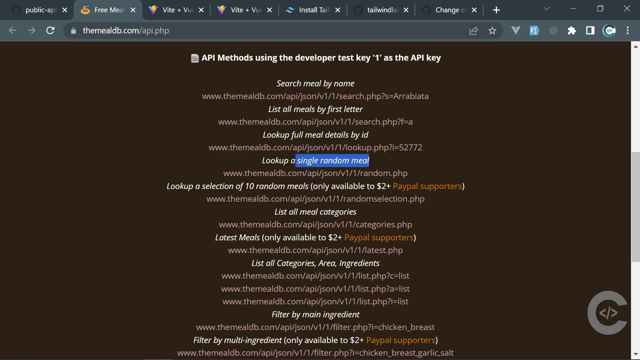 home page and we see that we have 10 words in the description description home page it was previously empty but right here the API basically has an end point to get a single random meal if you want to get the 10 random meals 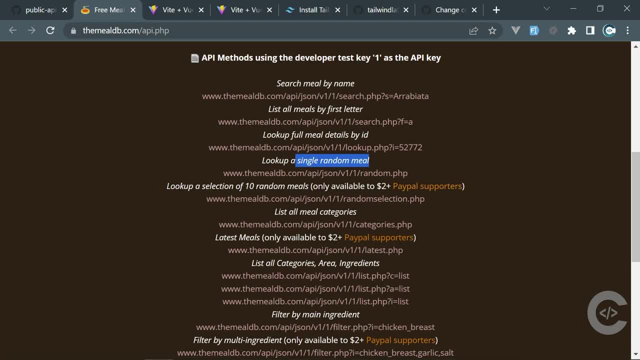 it was only available for two dollar plus people supporters okay so in this 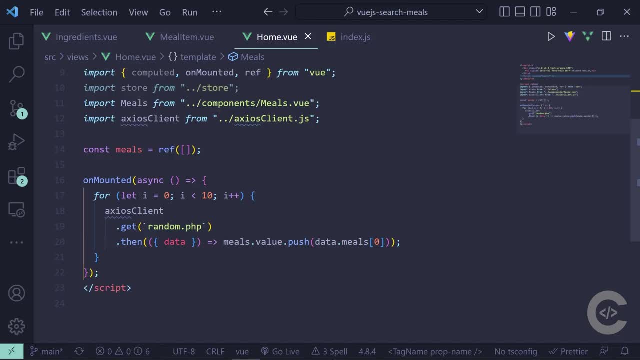 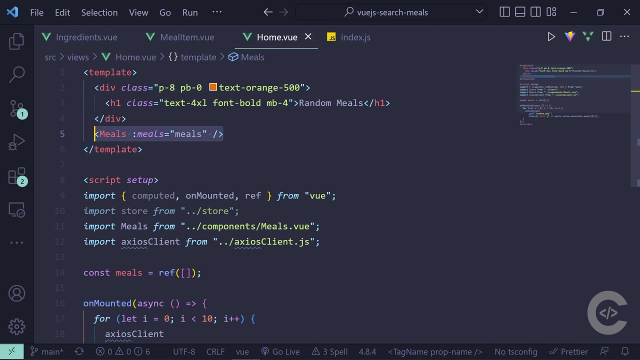 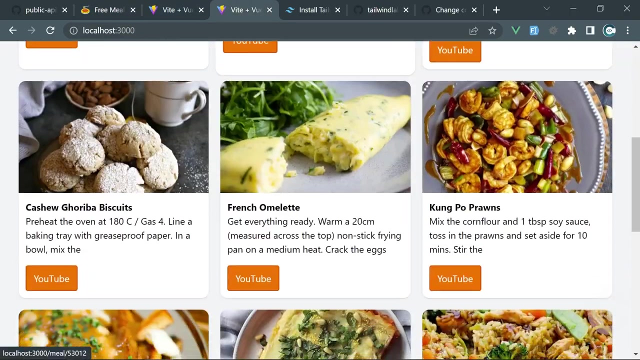 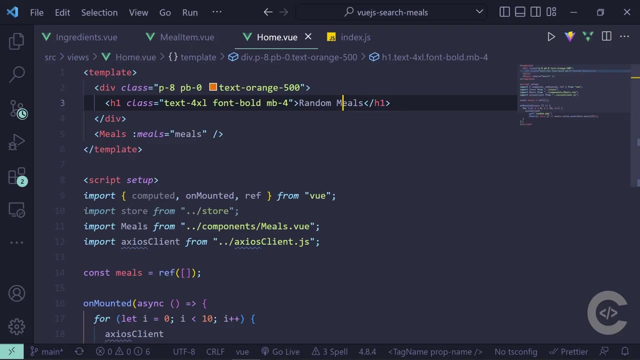 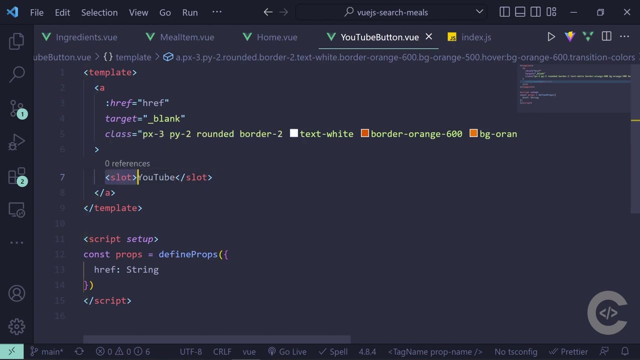 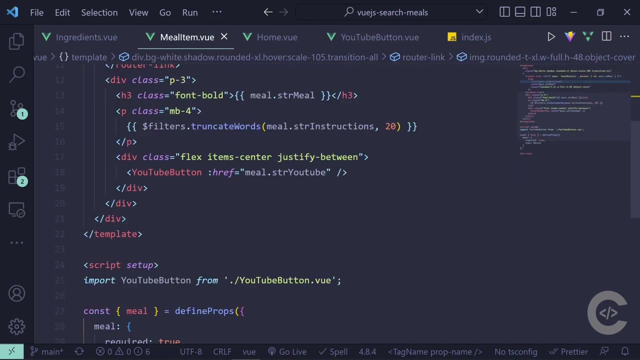 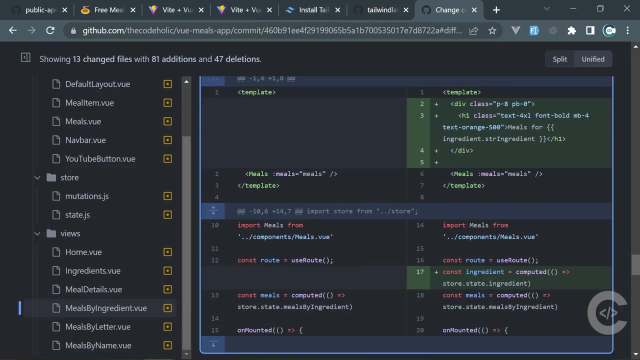 case I took this URL and just made requests 10 times so right here from zero to ten we are iterating we are making requests to this random PHP we are getting data and the data returns meals and there is a zero element inside there so we take this zero element and push inside meals so we have meals right here meals.value push received element and finally we have meals component right here and the title random meals with orange so this is how our new home page looks like which is nice and I also changed the YouTube's default I remembered how actually it was I didn't it didn't become necessary to Google for that so you just need to put the default text for a slot right here and if you don't provide this text it's going to take this one so in this case if we go in the meal item we don't provide the text for the YouTube button however if we provide that right here text for example it's going to appear right here okay so those were all the changes I made in this project we can check the repository again here it is scroll down below we talked about current ingredient those were 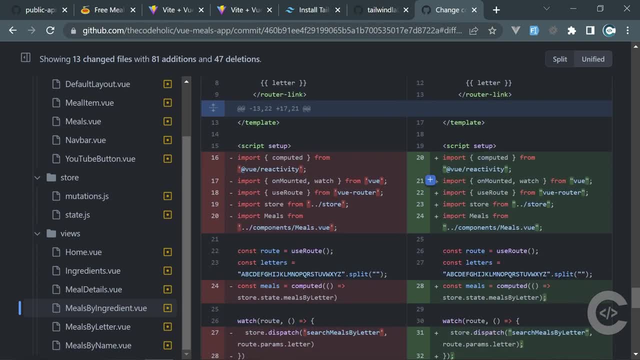 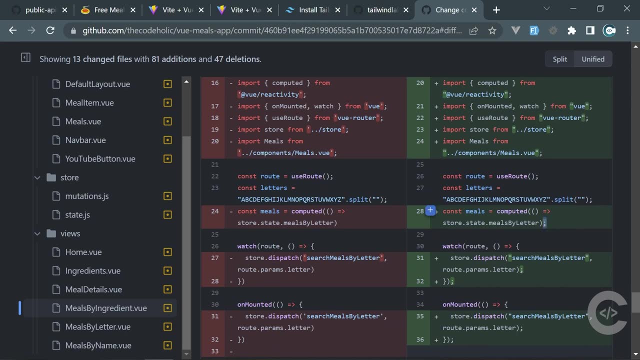 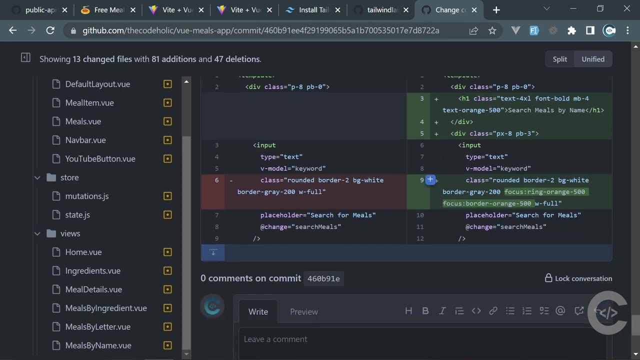 related to only title was changed some CSS stuff we have probably we have code formatting running because semicolons are added and the single quotes are changed into two double quotes nothing big deal search means by name we have that and yeah I think that's all what we changed in this specific commit but I 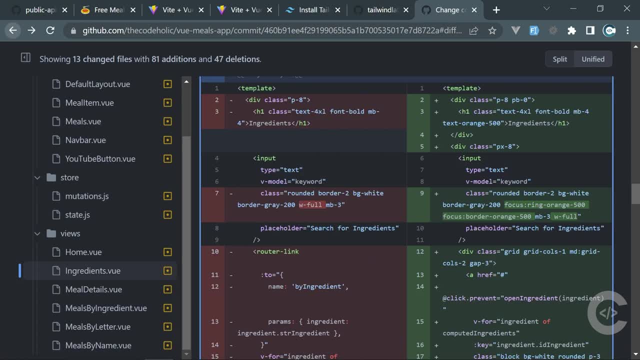 made a few more uh small changes in next comments if we go back 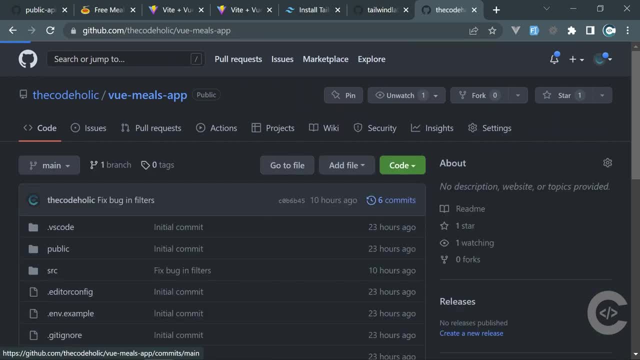 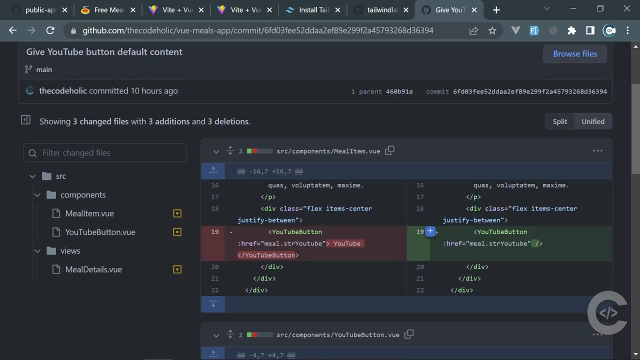 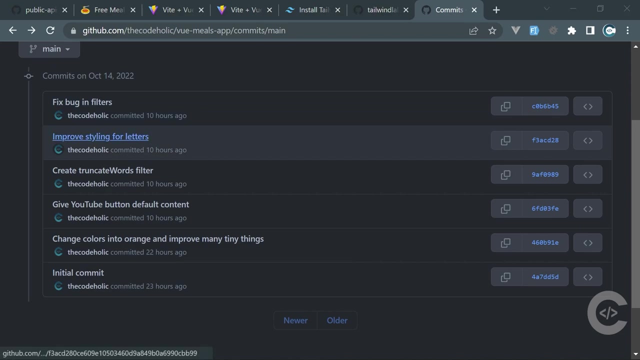 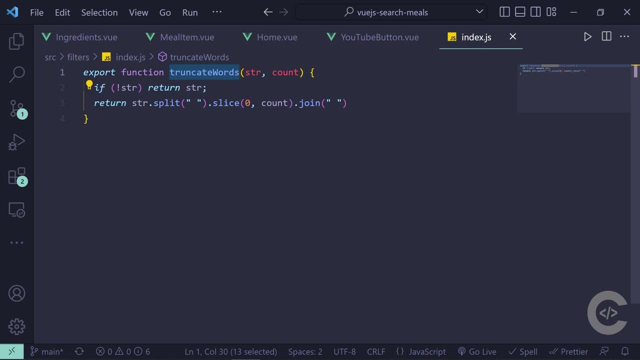 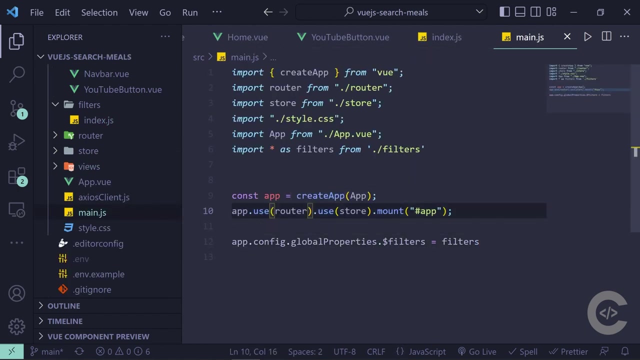 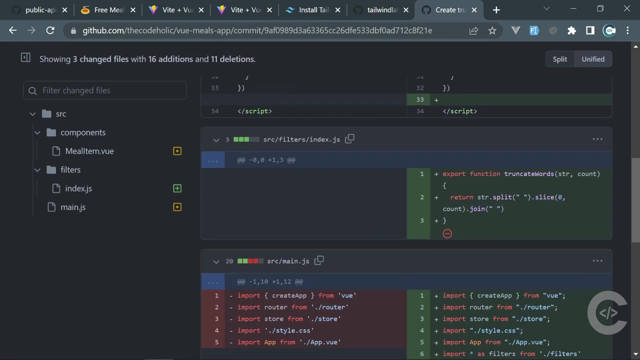 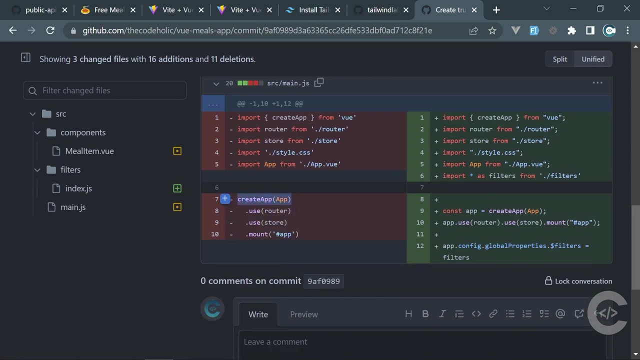 uh actually let's click right here and click on comments so that was the biggest change then give YouTube default content so this is simple change I explained already uh create truncate words filter which I also explained by the way I haven't explained how this filter is used so we create that function export function truncate words but we need to use that index filters index so this is done inside main.js so right here okay let's check this in the comment I think it's going to give us better view because we see the previous version as well okay down below we created this and the down below in the main.js we this is the old version okay okay so we were creating the app and then using rotor using store 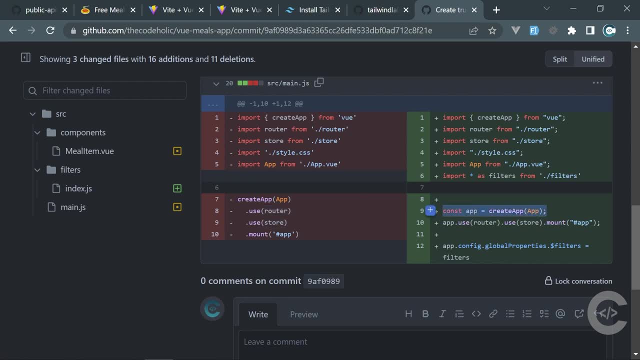 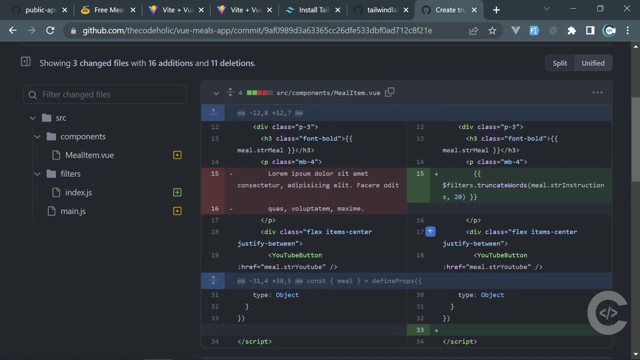 now when we create the app we save it in a variable up we use the router and use the like we were using before but upconfig global properties dot filters becomes everything imported from these filters okay that filters will become an object which will contain this truncate words method inside there so we assign upconfig global properties filters equal object and that's that's how these filters work and we are using dollar filter truncate words right here 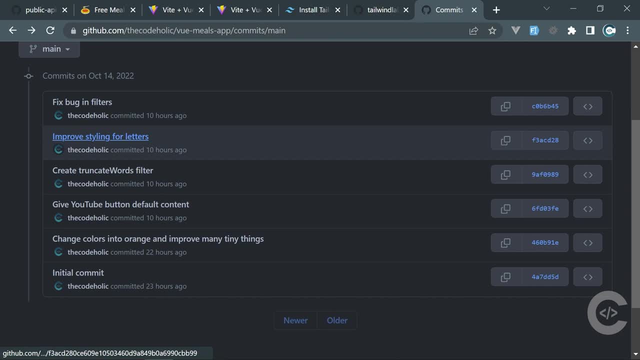 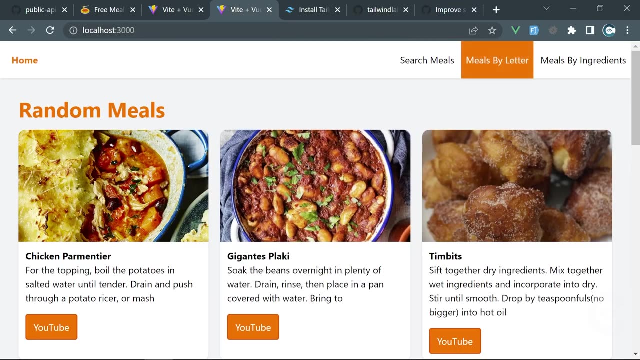 all right and the last commit is improved styling for letters yes i slightly improved the improved the styling for letters we can check this even right here so i added the hover effect the letters 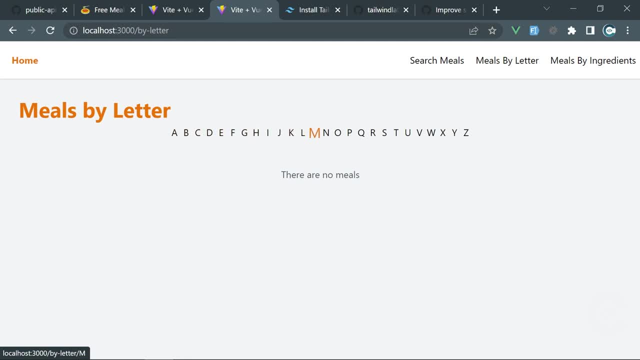 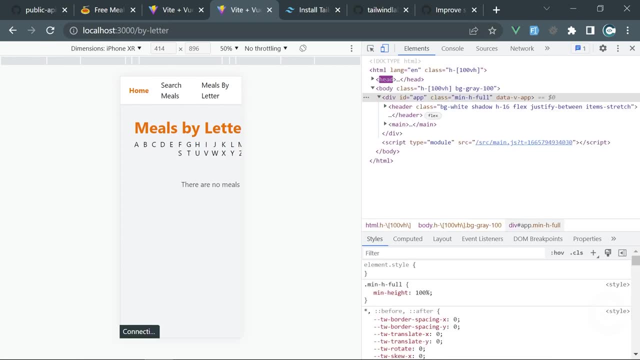 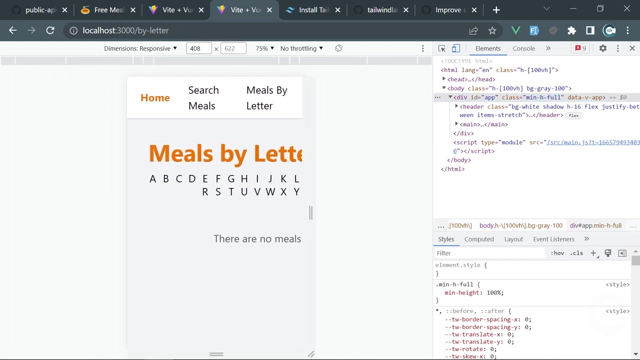 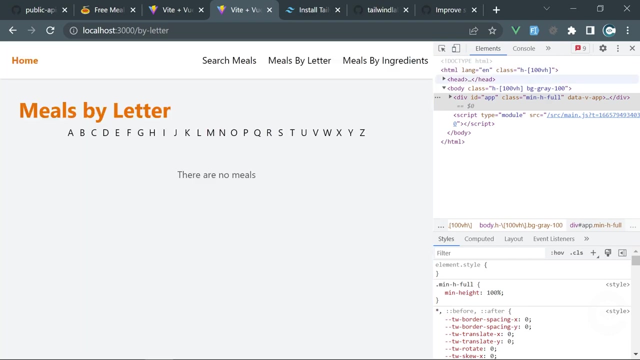 basically increase and i think this is nice as well and also unresponsive um it should look like nice okay it doesn't look like as as i expected to be honest okay something something is wrong at the moment unresponsive